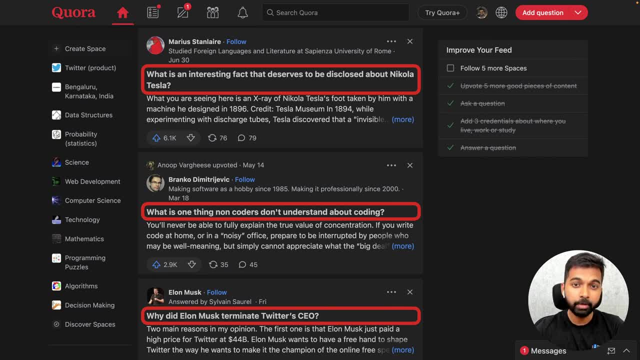 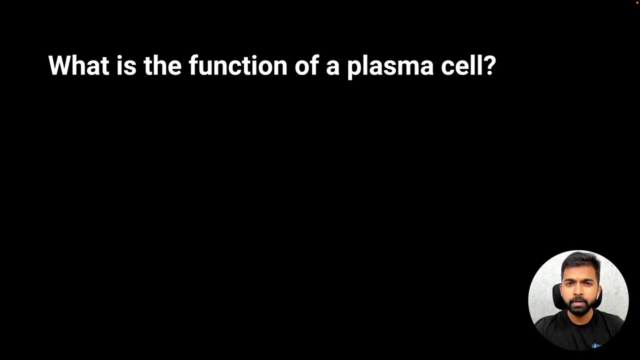 questions. Some questions may be problematic because they may be touching on sensitive topics, They may be hurting people's sentiments, they may be racist, sexist or just inappropriate in some form or another. For example, the question what is the function of a plasma cell is a good question. 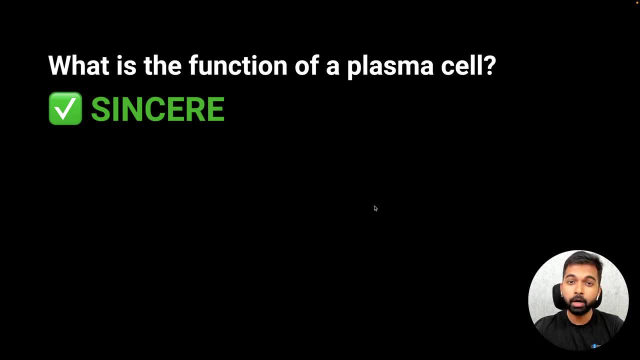 And Quora would call it a sincere question, And this is the kind of question Quora would want to include on their website. On the other hand, a question like this- why can't liberals realize that they're stupid- is clearly not really a question. It is more of a statement being. 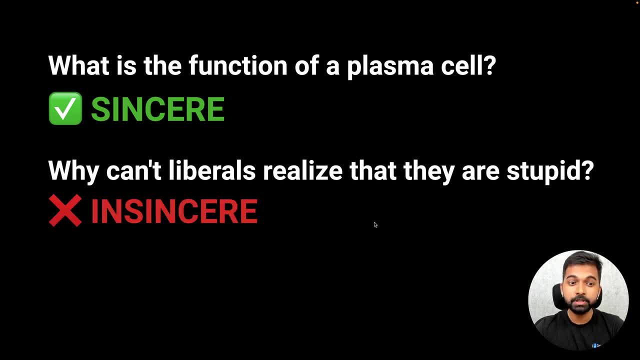 made against a particular group of people, And this is the kind of question that Quora labels as insincere, And this is the kind of question that they would like to avoid. Now the only trouble is, with 10s of 1000s of questions submitted every day, Manually reviewing every question can be time. 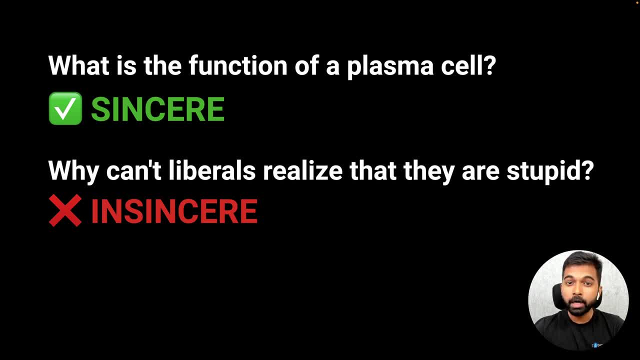 consuming and expensive. So that's why Quora set out to build an automated system which can classify new questions as sincere or insincere. So that's the example of a text classification language problem. in text classification you are given some text and you have to classify it into one or more. 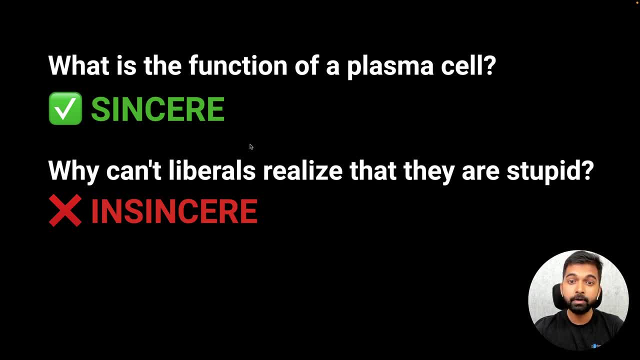 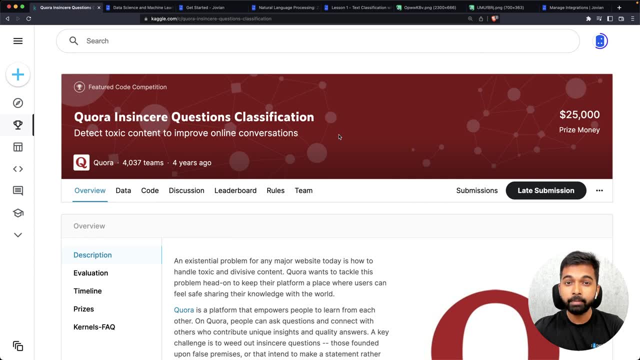 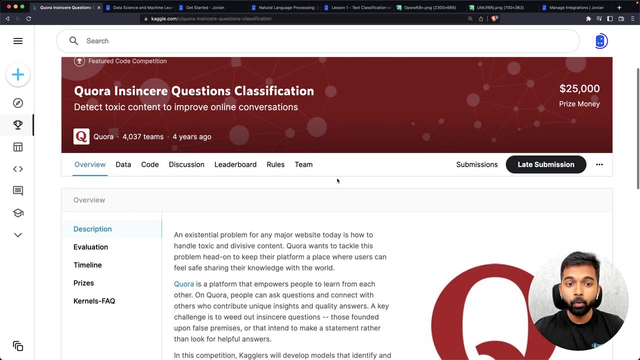 classes in this case, whether the question is sincere or insincere. so this was something that cora actually did, and they crowdsourced the development of this automated system, this text classification system on a website called kaggle, and cora created this competition called the cora. 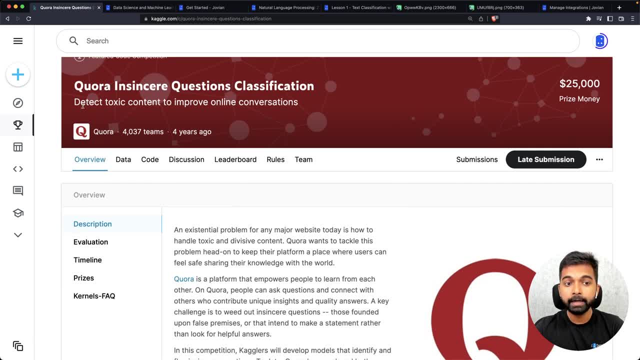 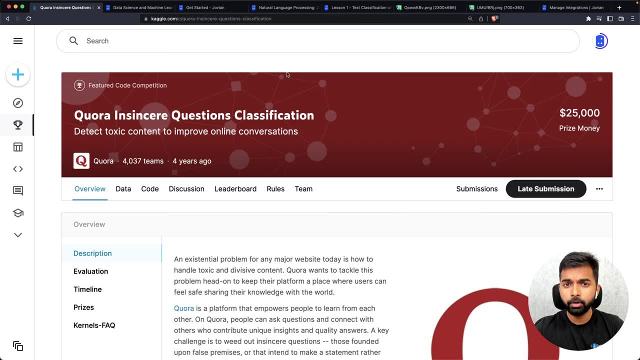 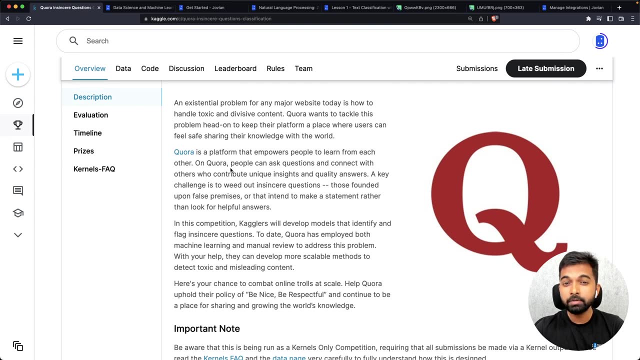 insincere question classification competition to detect content to improve online conversations. now the link to this competition is included below the video and here you can read a little bit about the problem that cora was facing, which we just discussed. cora wants to keep the quality. 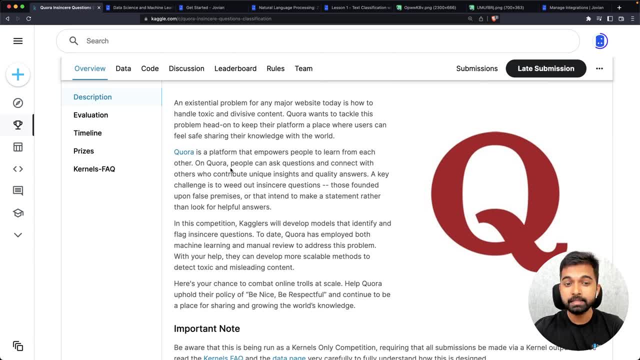 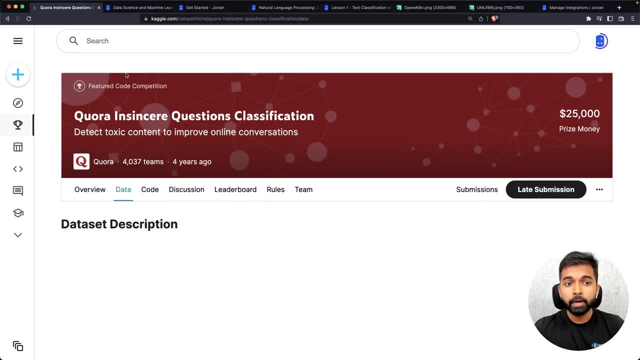 of the questions high and cora wants to avoid any insincere questions. so you can read this description. i encourage you to read it carefully. then you can also head over into the data tab, and in the data tab there is a description of the data that cora has provided for you to. 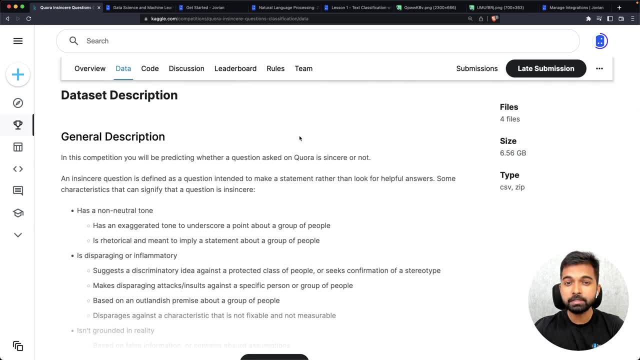 create an automated system now. this data consists of over 1.3 million questions that have been manually tagged by cora's internal team and they want you to use this data of tagged questions to create an automated system that they can use in the future to automatically classify questions as sincere or insincere. now, what makes a question insincere all? 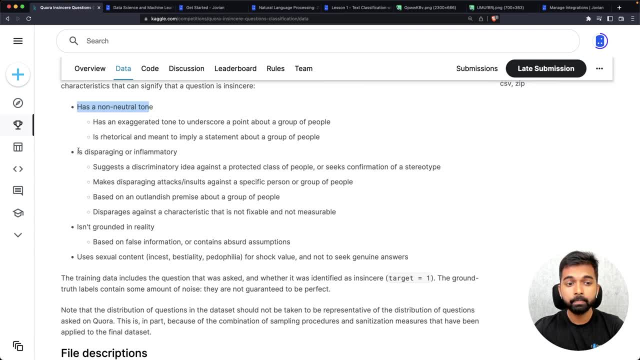 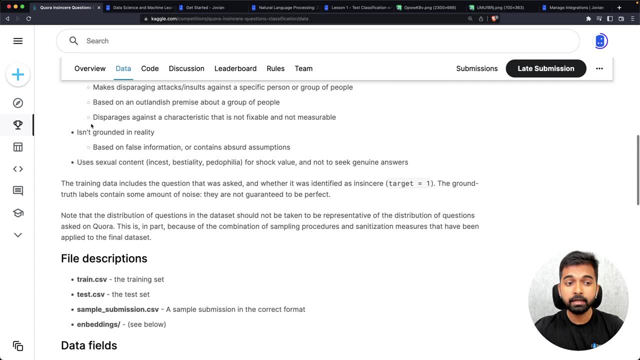 information is provided here if a question has a non-neutral tone, if it is inflammatory or discriminatory or disparaging in terms of the attacks or insults it makes, or if it isn't grounded in reality or if it uses sexual content. so your job is to create an automated system which 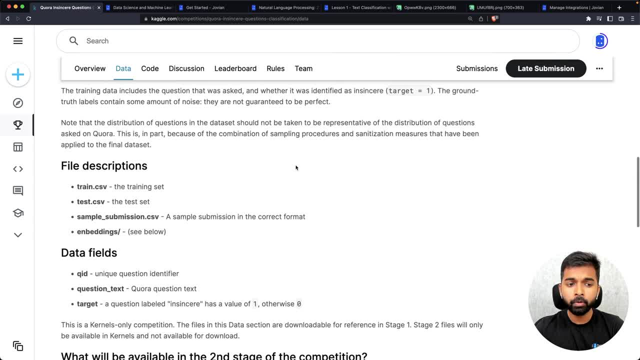 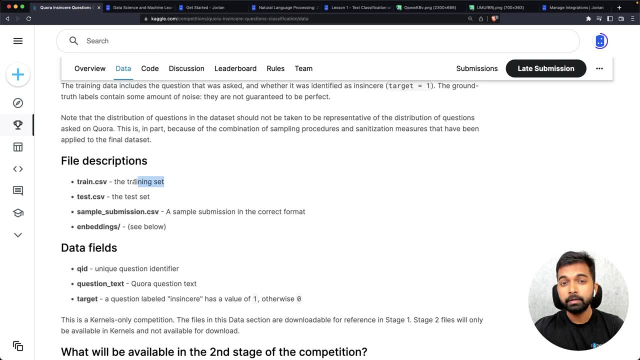 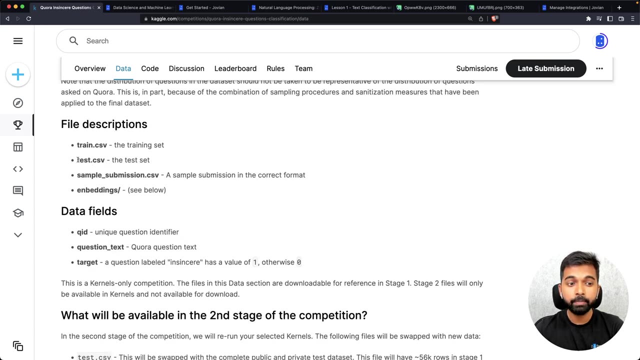 can detect questions like this. so cora has provided three files: traincsv, texttestcsv and sample submissioncsv. the traincsv file contains some data using which you can train your automated system. then you have to make predictions on a test set of questions where you don't know the labels, and your predictions will then have to be submitted. 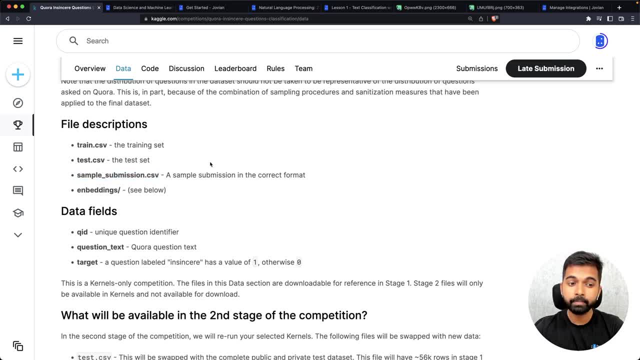 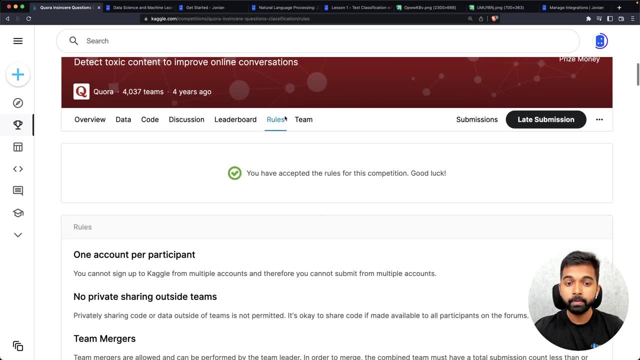 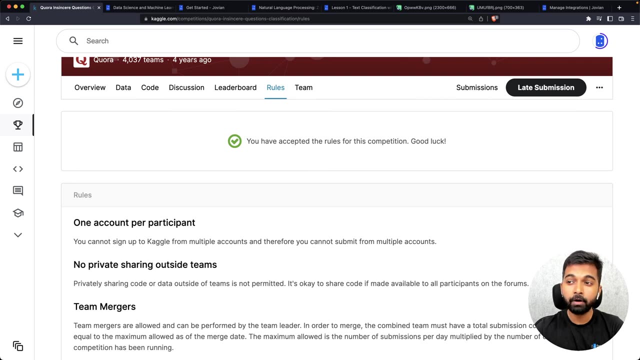 in the format that is indicated in sample submissioncsv. now, in order to download these files, it is very important that you first head over into the rules section of the competition and in the rules section you have to accept the rules of the competition. without accepting the rules, you will not be able to view the data of the competition. 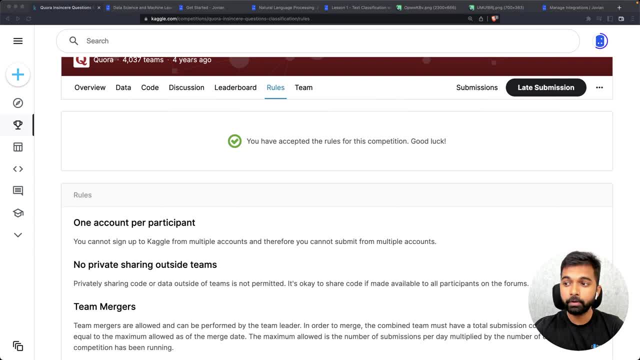 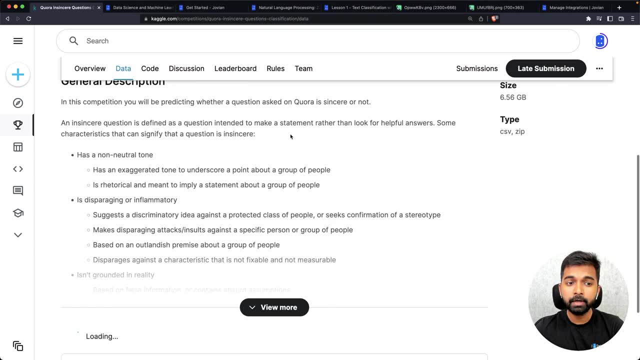 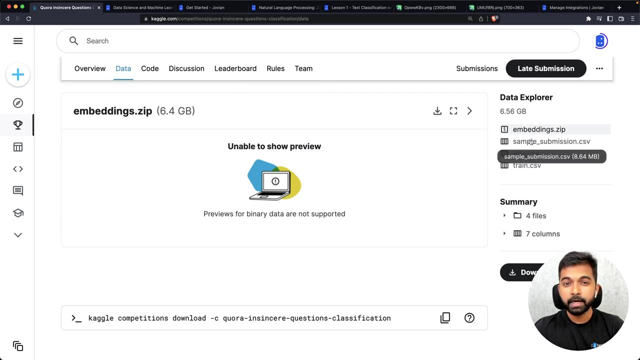 and you will also not be able to download the data of the competition. so do head over to rules on the competition page and accept the rules. then you can come back into the data section and if you scroll down here you will be able to see a data explorer. so you can either download individual files, one by 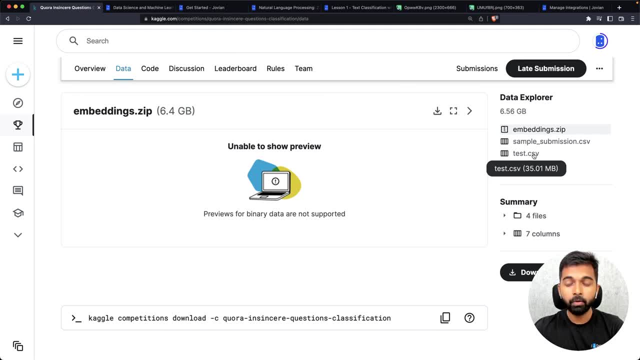 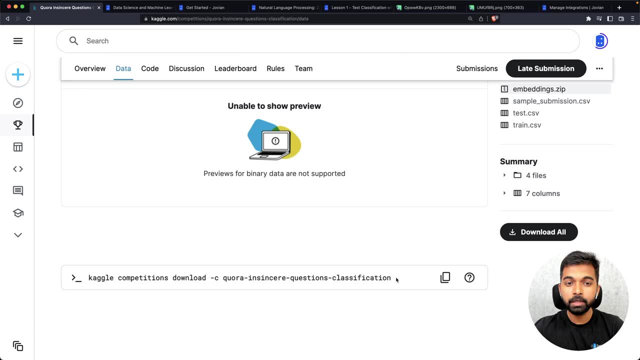 one and then upload it somewhere where you're writing code, or you can use this kaggle command line tool. so kaggle has a command line tool that you can use to automatically download your data. so let's get started by writing some code to process this data and build our automated text classification. 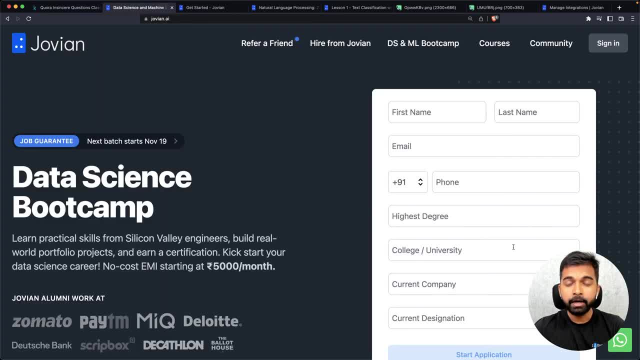 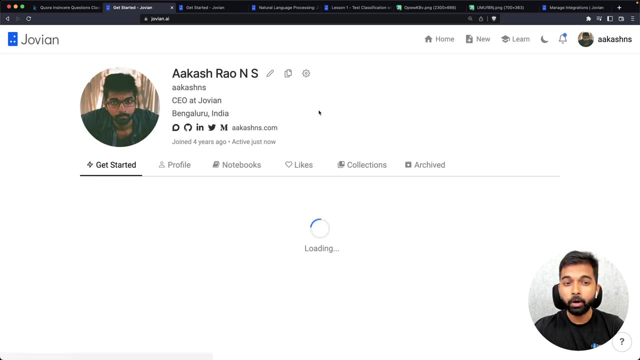 system. so let's head over to wwwjovianai, and jovian is a platform where we run a data science and machine learning bootcamp, so you can check out more information about it here, but for now, you can just sign in and create a free account, or log in. if you already have an account on jovian, you can. 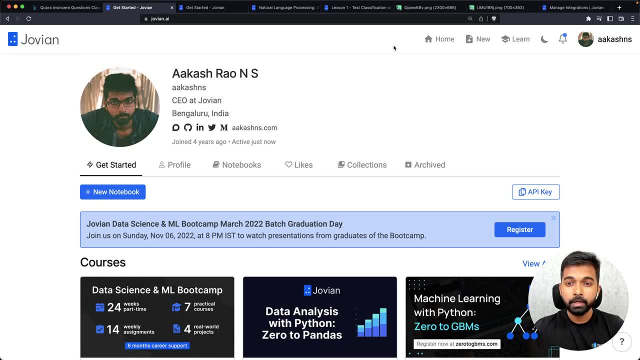 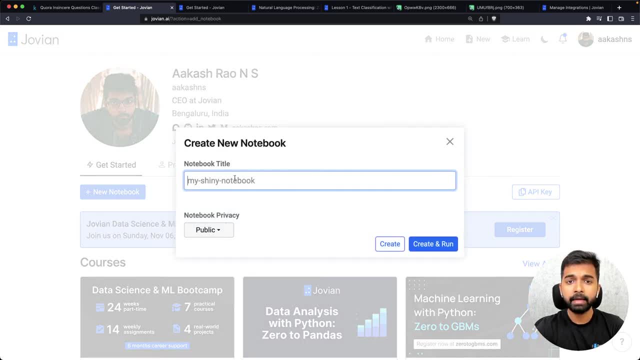 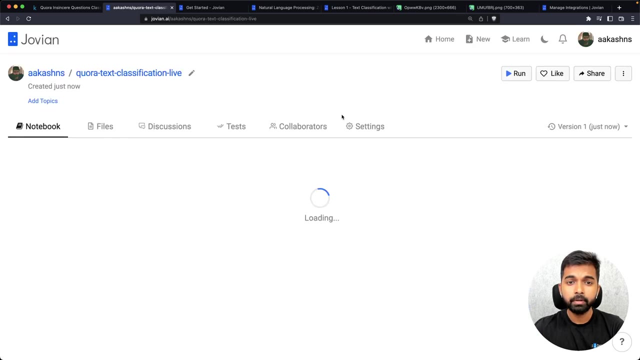 create a new data science platform project. so right at the top, find the new button and click on blank notebook. and now we're going to create a blank notebook and let's just call it cora text classification. i'm going to call it classification live and now i'm going to click create. so now we have created a new project on. 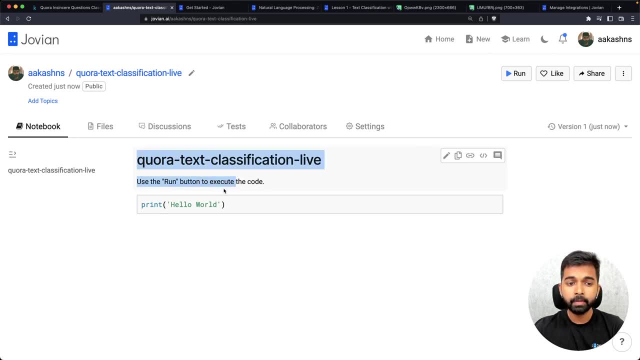 jovian. you can see it has a title here and it has some code here. this project is in the form of a jupyter notebook, which is a common tool used in data science for experimenting with code using an interactive programming environment. now the project has been created, but we also need to run the project so that we can start executing. 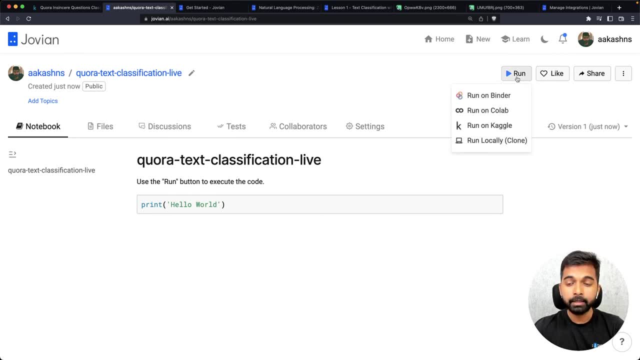 some of the code. so that's where we can click the run button and we have several options to run the code binder is a platform that we offer jovian offers. it provides some compute, but we are going to use a platform called google colab because this is a fairly large data set and we may have high 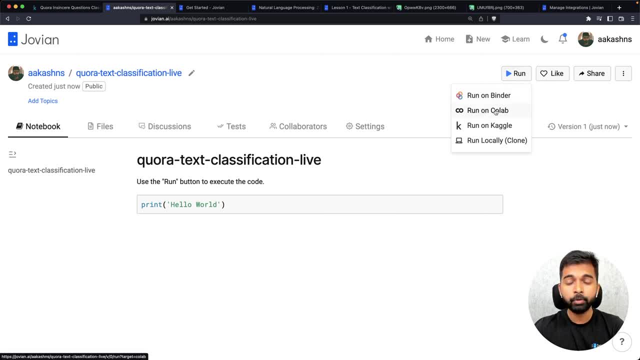 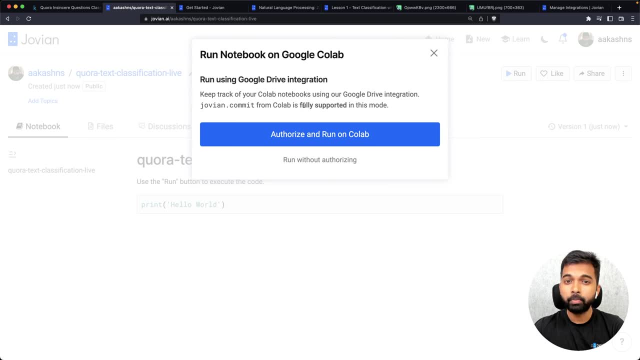 memory or cpu requirements. so i'm going to click run and then i'm going to click run on colab and google. colab is an online jupyter notebook execution environment provided by google and it requires any projects that you want to run to be part of your google drive. so, since we've 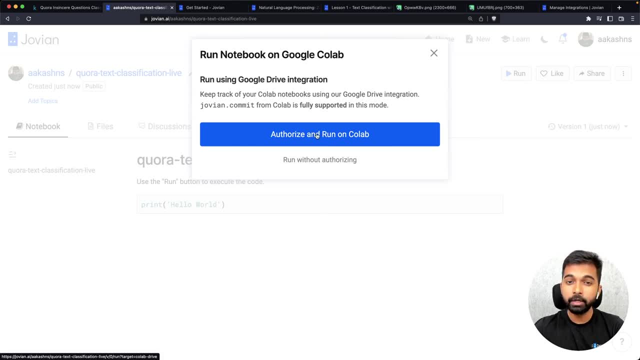 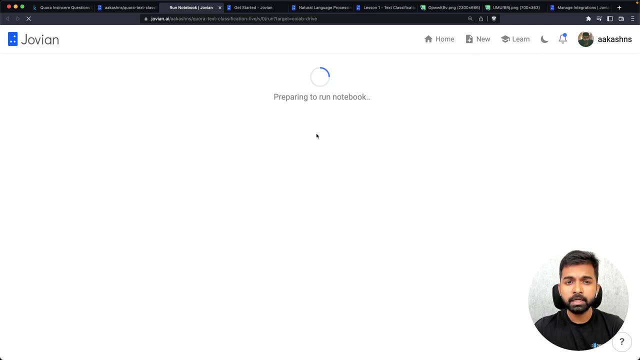 created this project on jovian. you will need to authorize jovian to access your google drive so that we can put this notebook into your google drive and then you can start executing the code. so i'm just going to click authorize and run on colab and then i'm going to select the account. 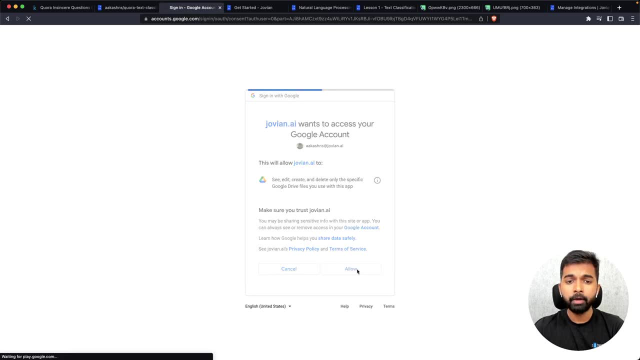 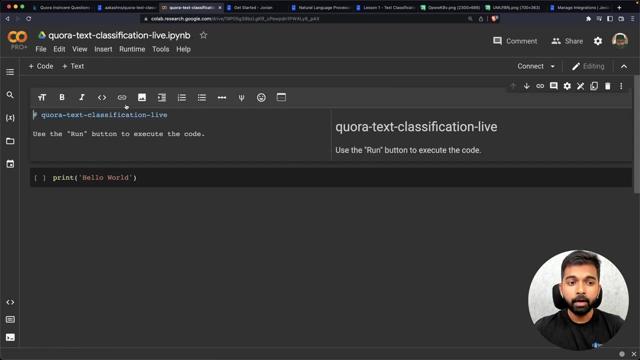 where i want to put this file and i'm going to allow these permissions so that jovian can put this file into my google drive. now we can run the code on google drive, we can make changes to it and then we can save it and bring it back into our jovian project. now let me give this a title. so 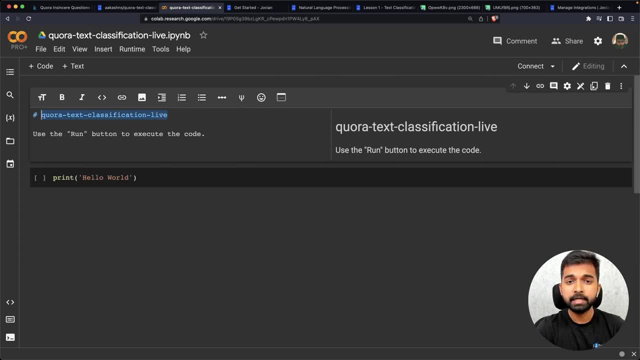 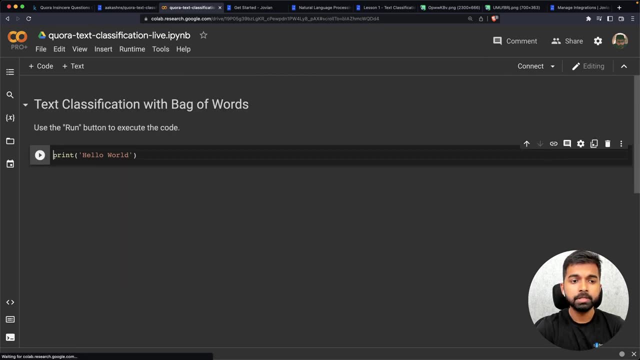 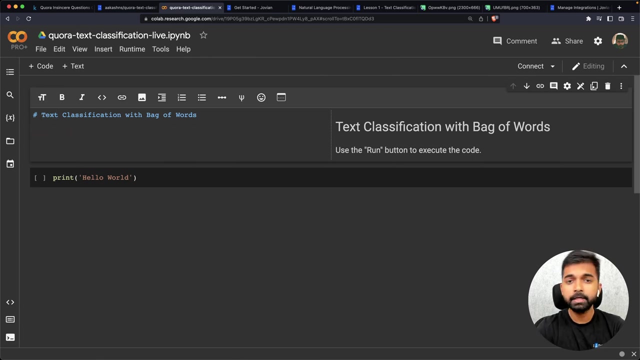 i'm going to click on the first cell and let me call this text classification with bag of words. so now we've given it a title and we are using markdown here, so you can see the hash character here creates a heading and let me get rid of this and let me write out an outline of what. 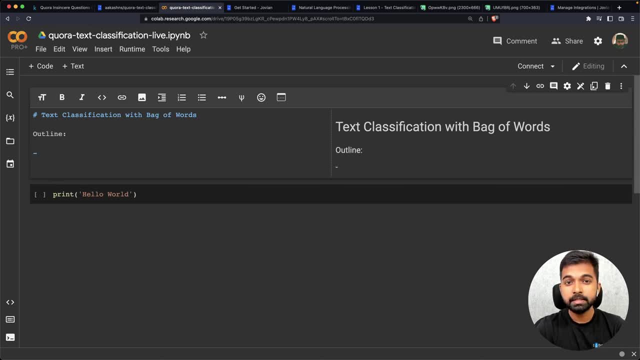 we are going to cover today. so the first thing we're going to do is download and explore the data. we are going to apply text pre-processing techniques, then we are going to implement the bag of words model. this is how we are actually going to build a text classification system. 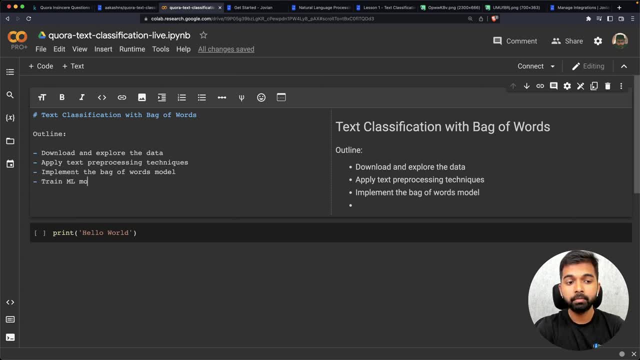 and finally, we are going to train ml models for text classification. now, once we've trained an ml model, we can also then make some predictions on the test data that has been given in the competitions and submit them to kaggle. this is an optional step, but i recommend doing it just to complete the entire cycle. so 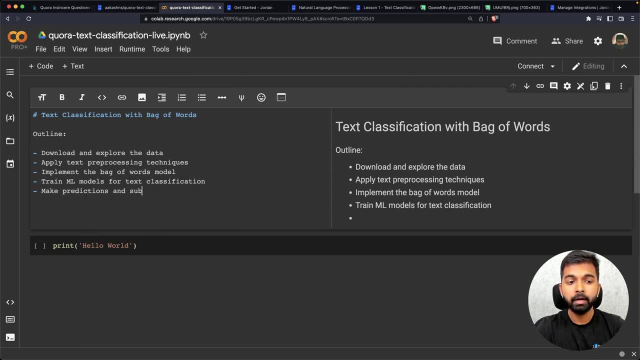 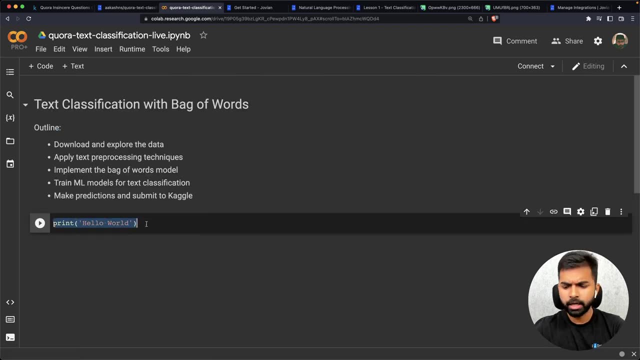 make predictions and submit to kaggle. so now we have an outline and below this outline we have some code. i'm going to remove this code for now, and one of the things that i can do in google colab is create sections that will show up within the test data. 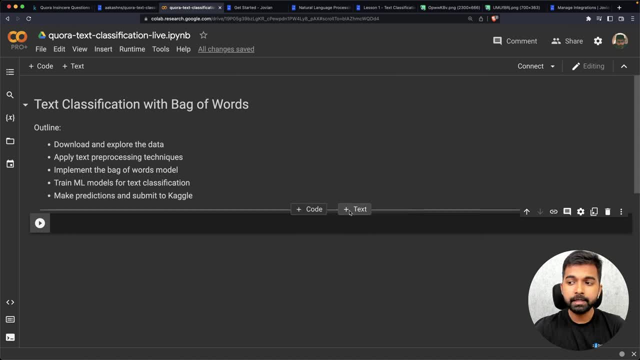 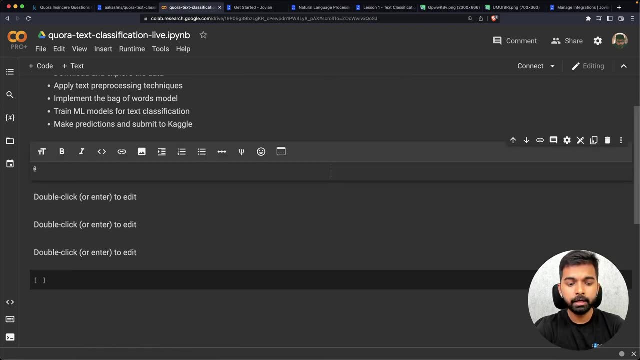 table of contents. So all I need to do here is click the plus text button and then I can create some sections. So here I'm going to double click, here I'm going to create a new heading, So the section is simply going to reflect the outline. 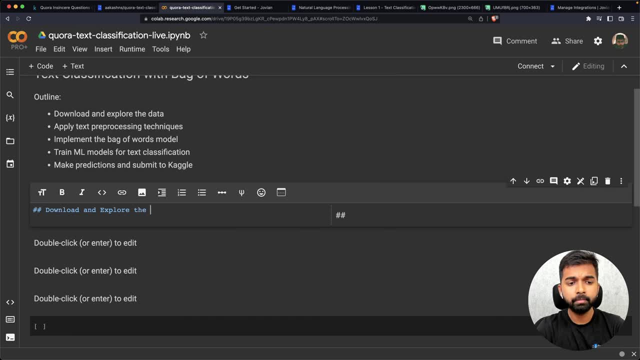 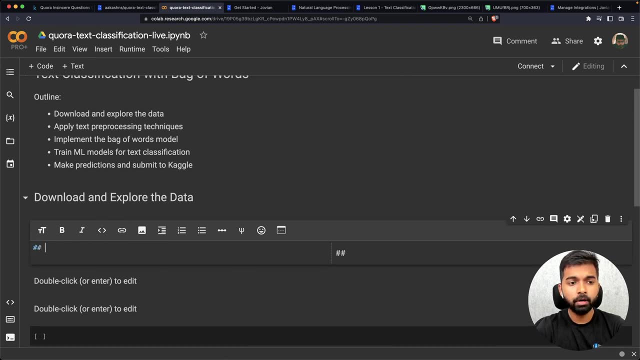 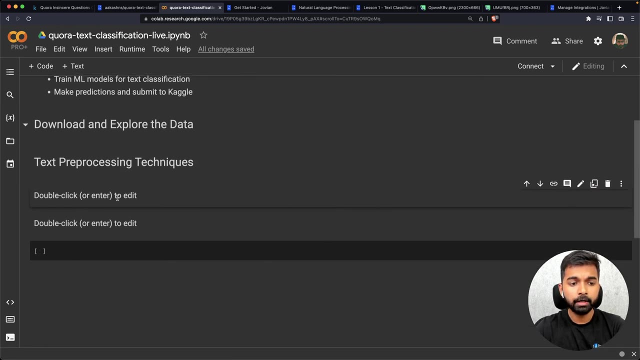 So I'm going to type, download and explore the data. Then I'm going to create another section here. This is called text preprocessing techniques. Then I'm going to create another section here. This is called implement bag of words model. Then let's create another section here: ML models or text classification. 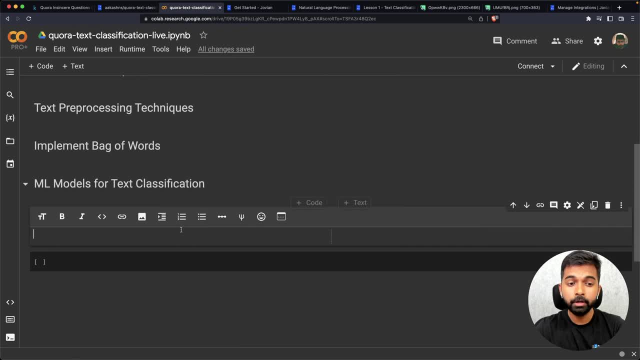 And, by the way, feel free to pause the video at any point and follow along. the best way to learn NLP, or anything in machine learning for that matter, is by just implementing it yourself on a real world problem Like. And finally, we are also going to make predictions and submit to crackle all right now, now that 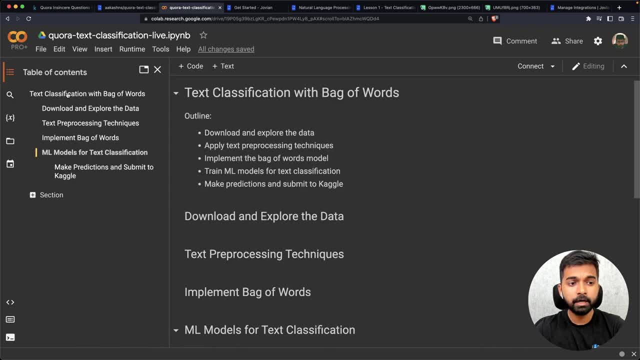 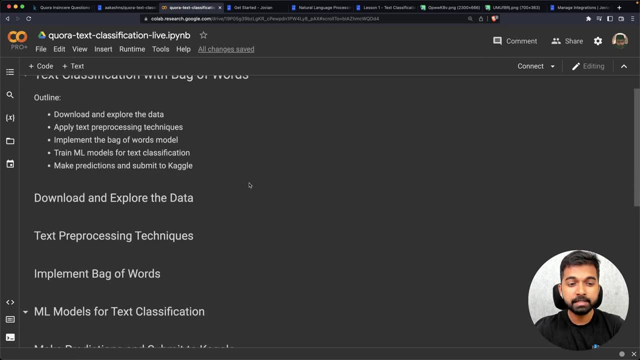 we've created these new cells and we've added these headings. you can see that now we have a nice outline here. that's showing up in the table of contents so I can jump around the notebook as I write a lot of code. now below the download and explore data. 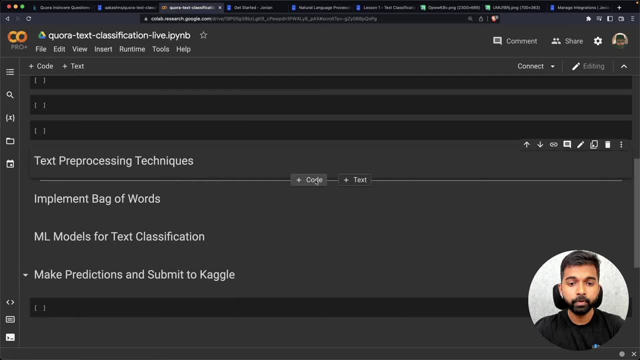 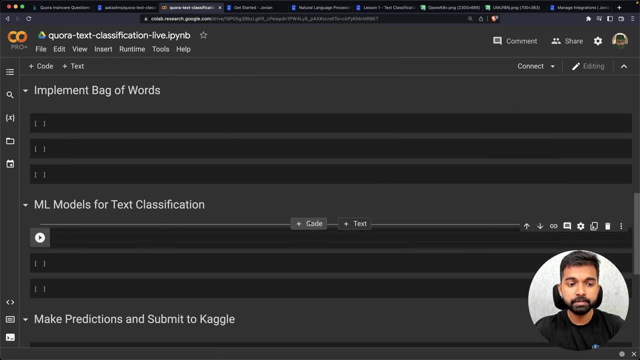 Let's create some code cells. Let's also create some code cells here under text preprocessing Techniques. Let's create some more under bag of words and under ML text classification. Okay, So now down to the first step: downloading and exploring the data. 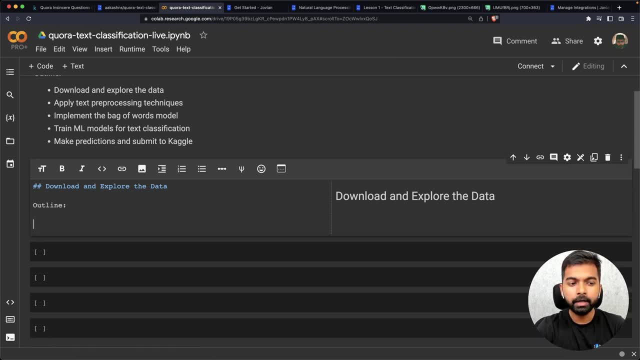 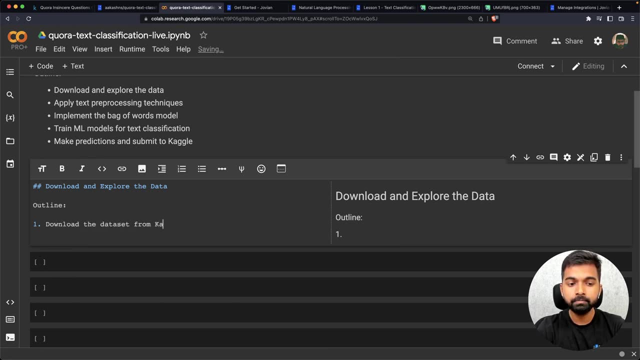 Once again within each section. it's always a good idea to again create an outline. So here's what I'm going to do Now. I'm going to first download the data set from Kaggle to Colab, Then I'm going to explore the data using the pandas. 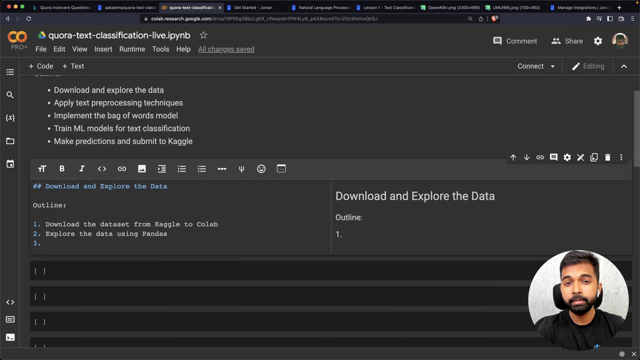 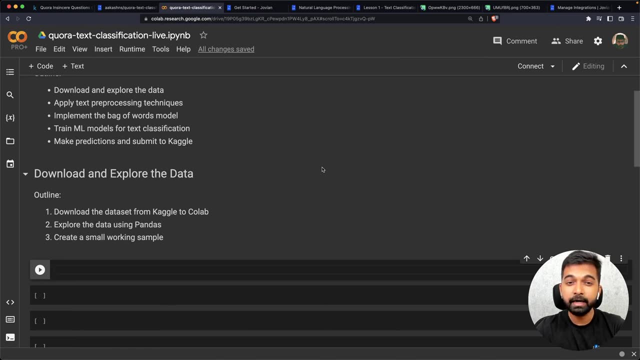 And this library. and finally, I am going to create a working sample because it's going to be a large data set, So I don't want to work with the entire data set. It's always a good idea to work with a small sample of the data while you're just setting. 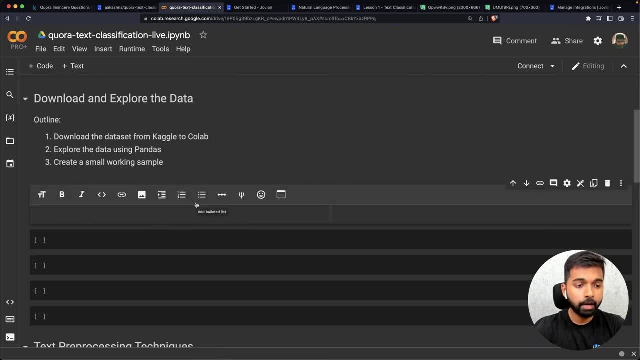 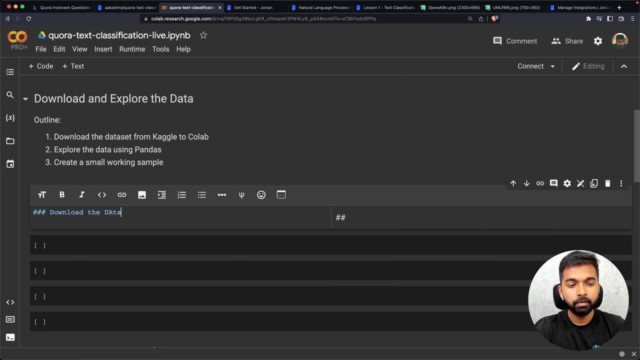 up your notebook Once again. the first step is to download the data to Colab. So I'm now going to create another heading, but download the data to Colab. Okay, And let's start now writing some code to download The data to Colab. 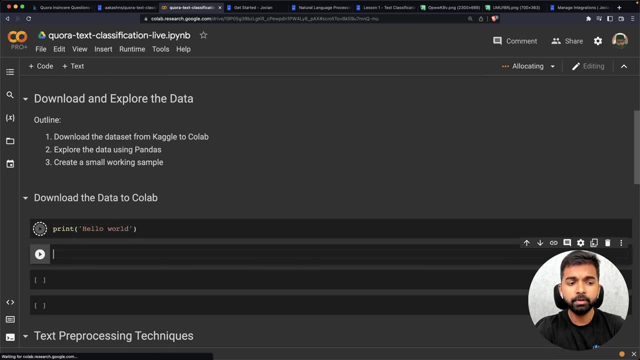 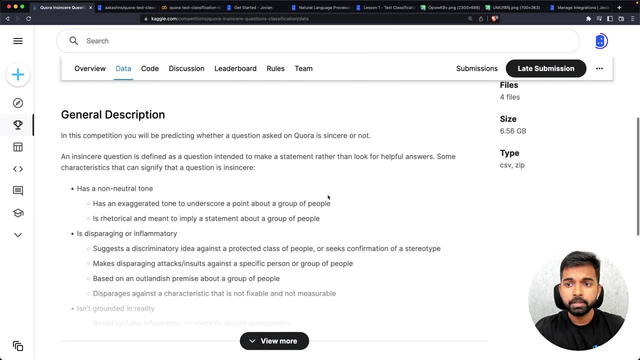 Now inside the code cells here you can write Python code, for example print hello world. But let's see how we can download this competition data set. So now I'm on, now I'm on this competition page and in the competition page I'm on the. 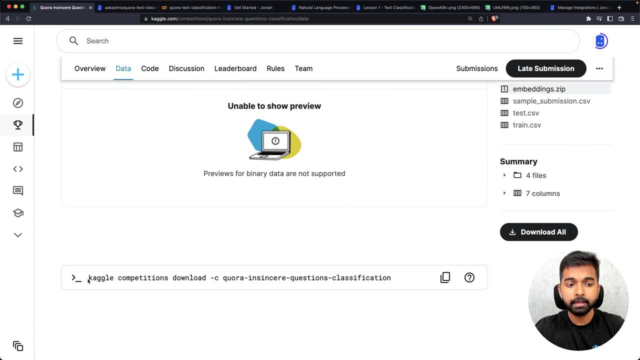 data tab and I go down in the data tab and I can see here that there is this command and this command can be used to download the data set. So I'm just going to copy this command here and I'm going to try to run this command. 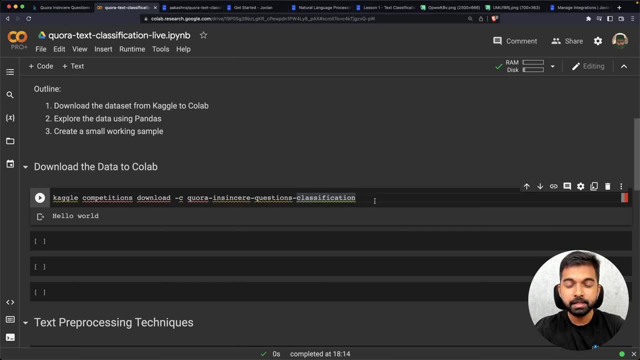 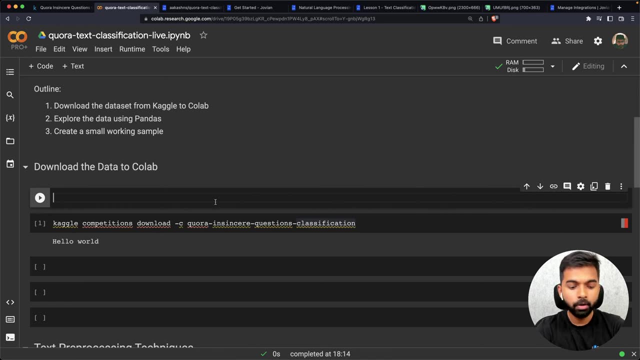 This command is not a Python command. This command is a shell command which has to be run on the terminal. Now, fortunately, Jupyter notebooks, apart from allowing it to run Python code, also allow you to run shell commands. For example, I can run the command LS and it can show me some output. 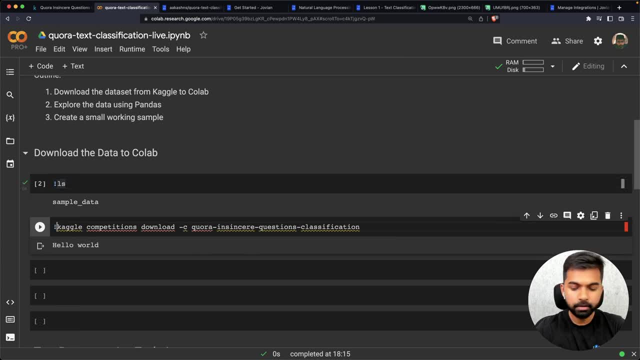 You can see here. So here's what I'm going to do. I'm just going to run. exclamation point. Kaggle competitions. download. and minus C: Cora insincere questions- classification. So this is the ID of the competition. 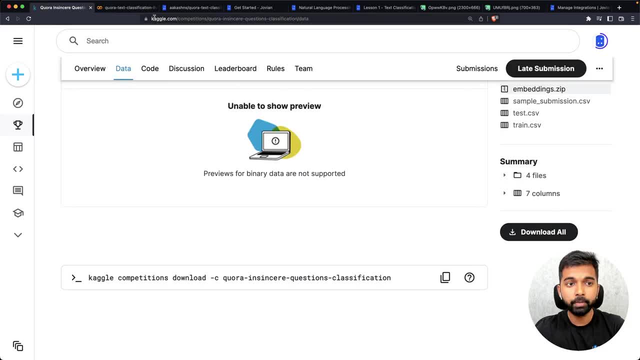 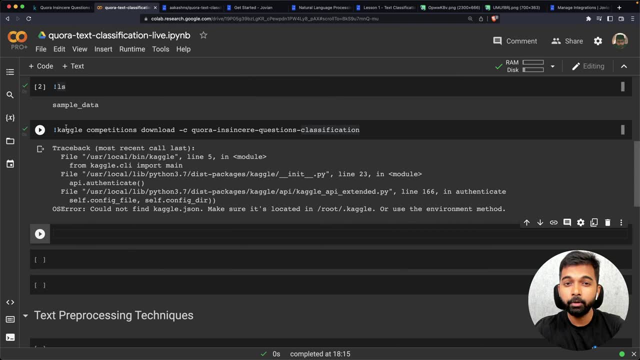 That can also be seen in the URL of the competition. Okay, Let's try to run that. So now we are trying to execute the shell command, which is going to download the data set, but there's a problem. So let's not worry. 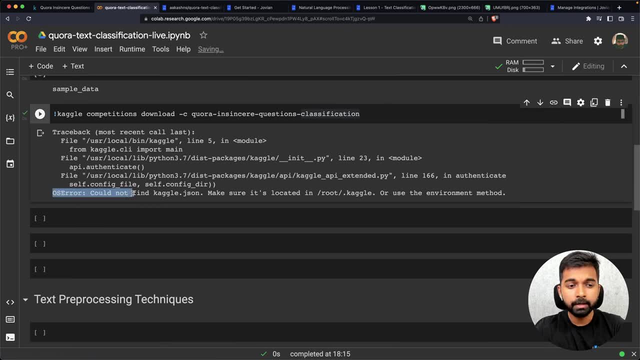 Let's just look at the problem. Normally for a Python error you can look at the last sentence. So it says here: OS error could not find Kaggle dot. Jason, Make sure it is located in slash root slash dot Kaggle or use the environment method. 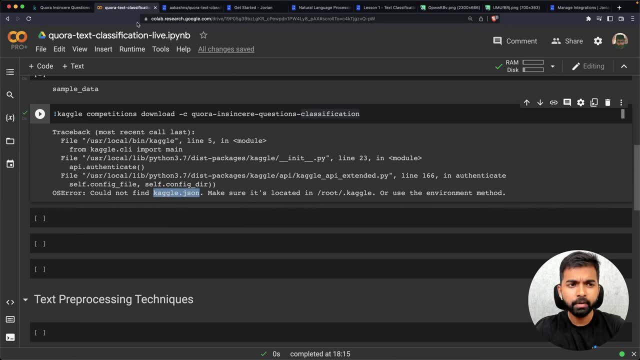 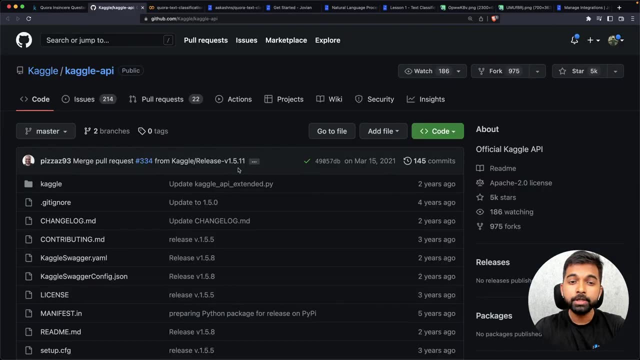 Okay, Look Okay. Looks like we are missing some file called Kaggle dot Jason. No problem, Let's just come back here. And next to this copy command there's also a question mark. So let's just click this question mark, which will take us to the documentation for the Kaggle API. 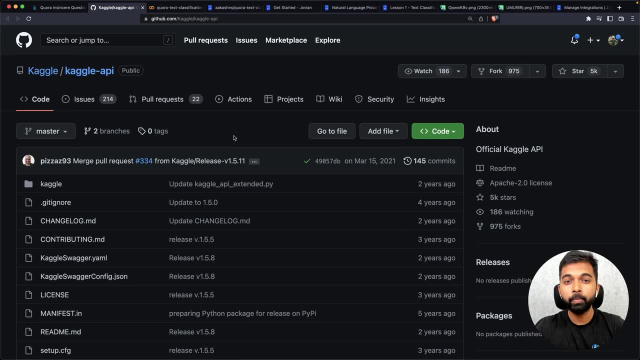 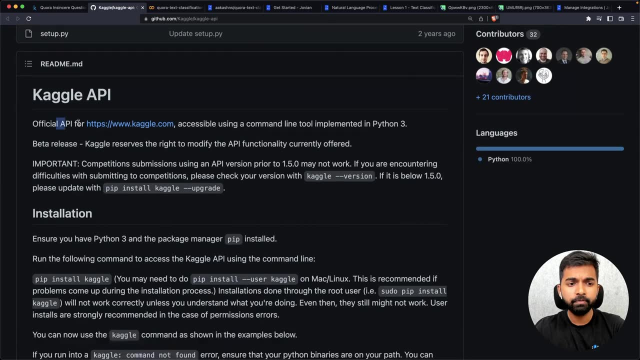 So this is often something you will have to do when you're using any open source tools. You may have to study some documentation. It's not something to worry about. So let's see here. The Kaggle API is the official API for Kagglecom, accessible using a command line tool implemented in Python, three, et cetera. 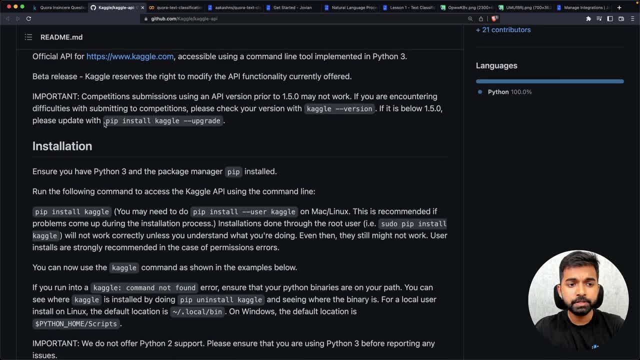 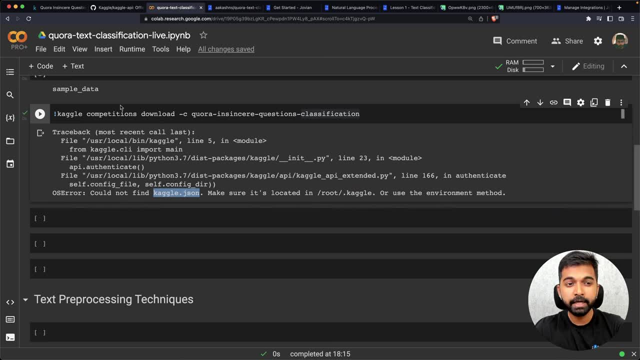 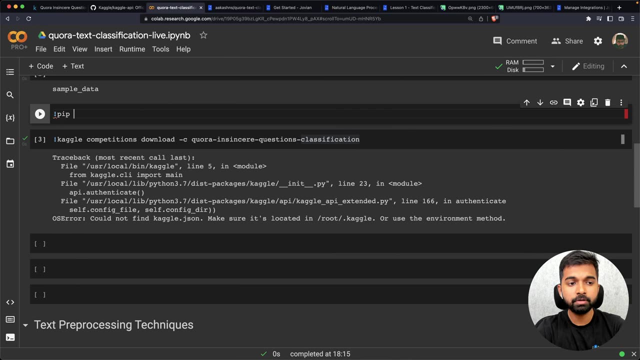 And it says here that you can install it using pip install Kaggle. In our case there was no installation error, Otherwise it would have said Kaggle not found. So it looks like it's already installed on Colab. but in case it was not installed, you can always do a pip install Kaggle and that will install the library. 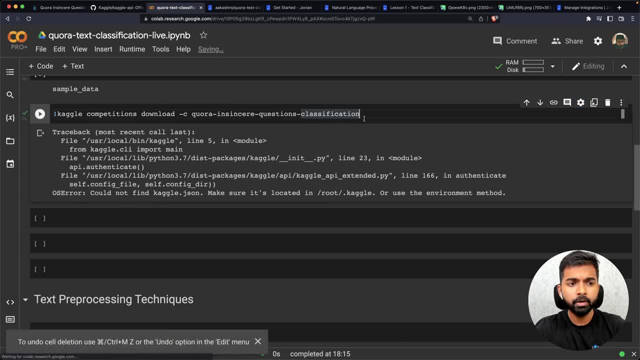 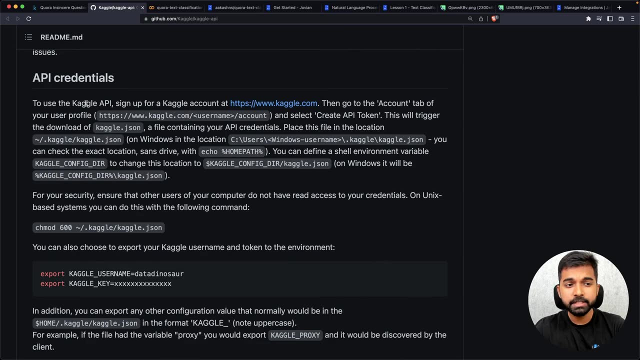 Let's say you are running this code locally on your computer, but we don't need that, All right. Then, after the installation, there is the section called API credentials. So it says that to use the Kaggle API first you need to sign up for an account on Kagglecom. 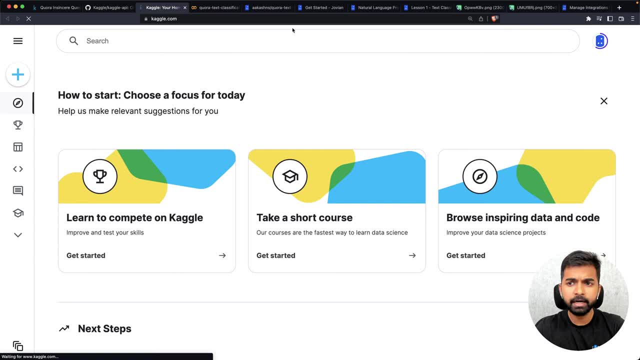 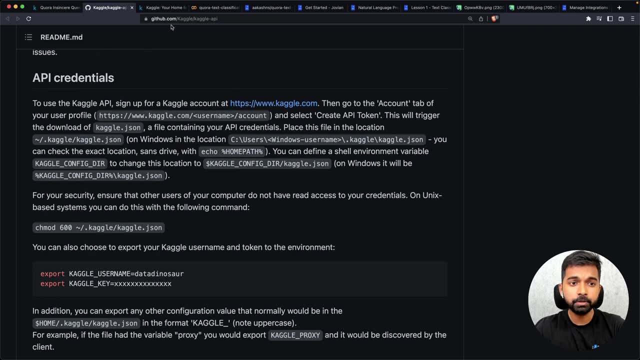 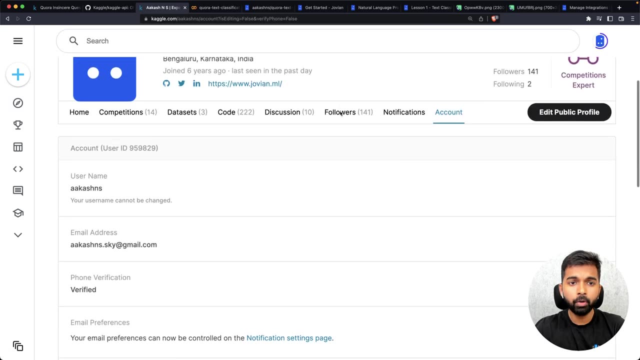 Okay, I already have that. I'm already logged in here on Kaggle. Then you need to go to the account tab of your profile and select the create API token option. So let me go in here and let me click on account. Now let me go down here and there is an option called create new API token. 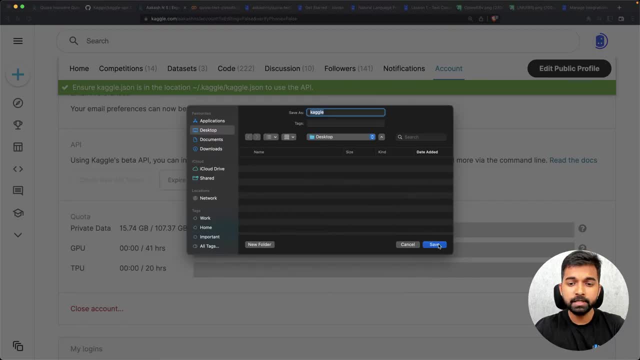 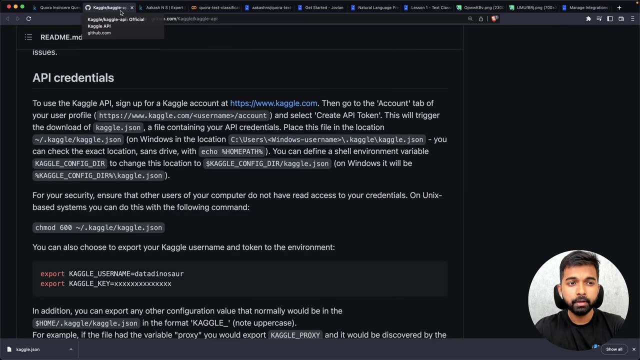 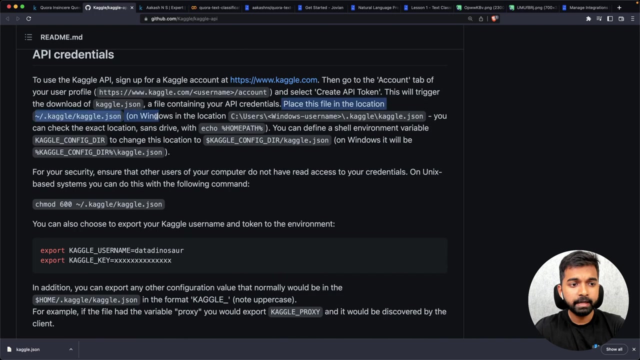 All right, And I'm going to save this Kagglejson file. It looks like it got downloaded Here. I'm going to save it here on my desktop and then it says that, please, this file in Delta slash dot Kaggle, slash, Kagglejson. but remember I am running my code on Google Colab, so it will not serve the purpose if I just put this file on my computer. 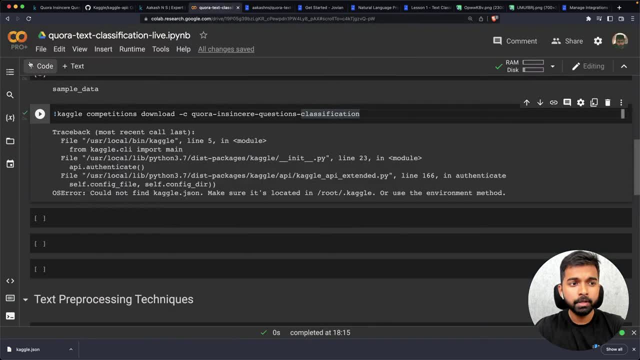 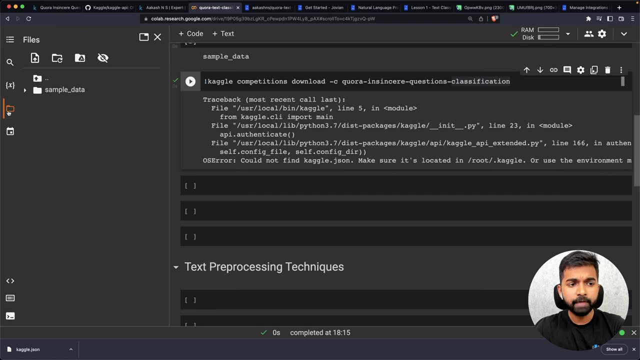 So I will have to upload this file to Google Colab. So in Google Colab I can come in in the left here And here I can see the files tab. so I can open the files tab and there's an upload button here. 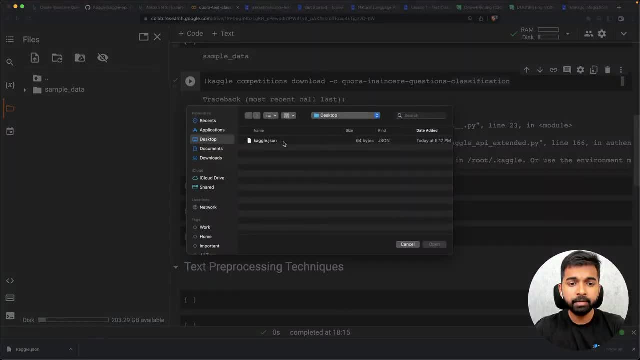 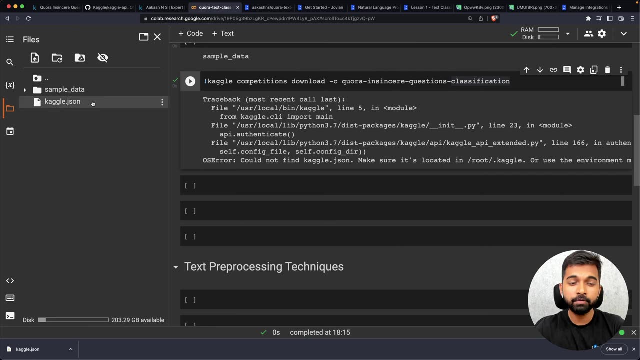 So let me click the upload button and let me grab the Kagglejson file and put it in. Okay, So every time you run a notebook on Colab, you will have to upload the Kagglejson file If you want to download any data on Kaggle. or you don't need to download the Kagglejson file again and again. you only need to download it from Kaggle once, but upload it to Google Colab every time you need to run a notebook. 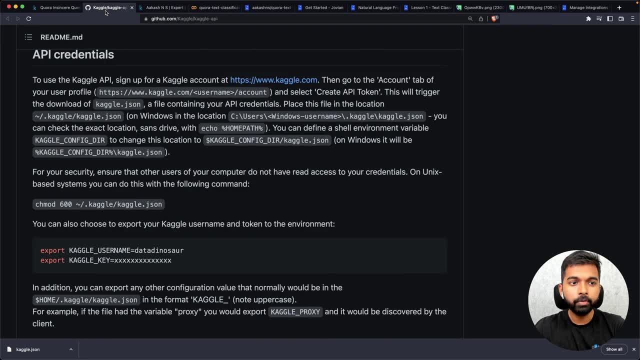 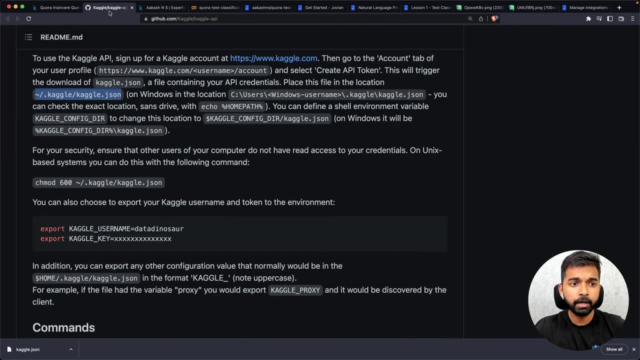 So you'll get the idea. Okay, The last thing. it says: either we can put this file in this location- but we have just put it in the current directory, in the current working directory, Or it says you can define a shell environment variable called Kaggle config directory to change the location of the Kaggle file. JSON file. 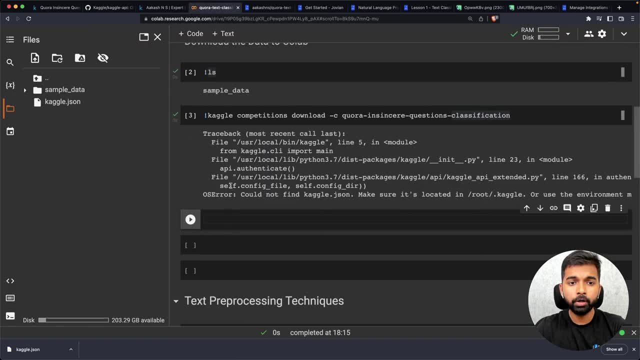 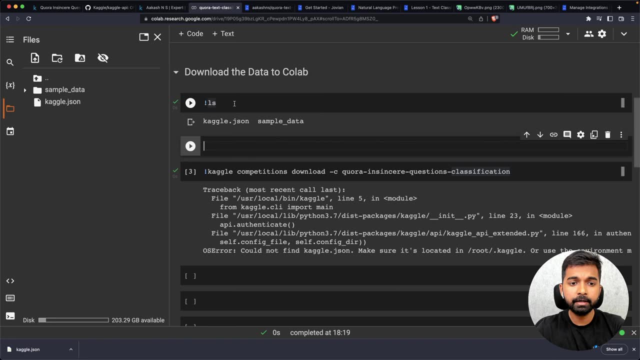 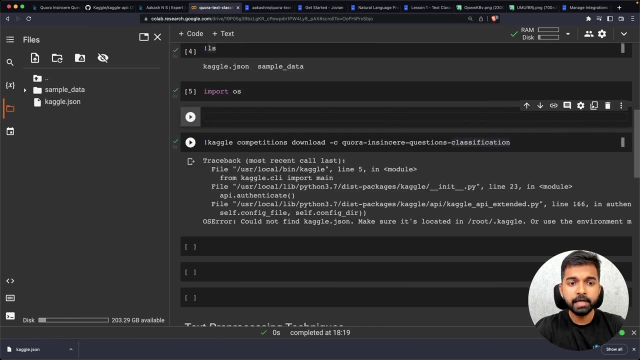 So here's what I'm going to do: I'm going to import the OS module and I'm going to do it above. So now you can see here that we have in the current directory We have a Kagglejson file. So I'm going to import the OS module, import OS and inside OS. 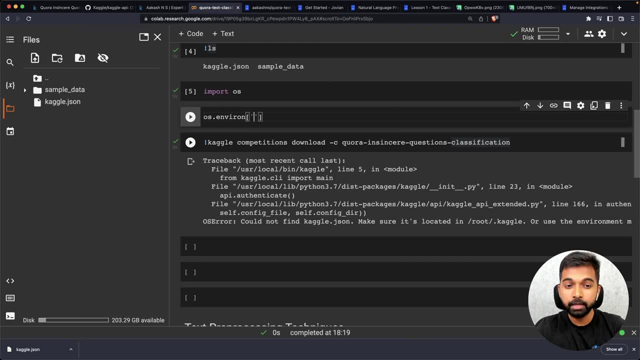 I'm going to set OS dot Environ. So I'm just setting an environment variable, a shell environment variable which will inform the Kaggle API, the Kaggle command line tool, where the config file is located. Okay, So I'm going to say OS dot Environ, Kaggle config dir equals dot. dot simply refers to the current directory. 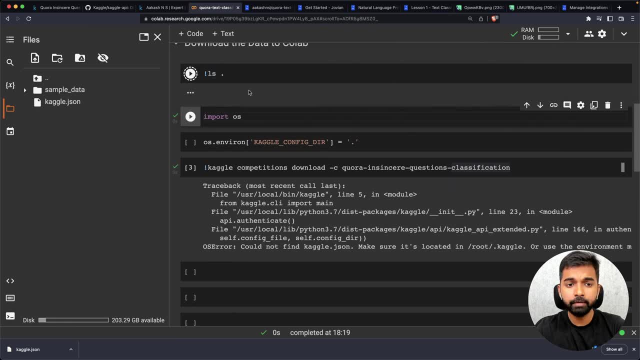 So instead of saying LS, I can say LS, dot, and it will do the same thing. So all I'm doing is I'm configuring that the Kagglejson file is placed in the current directory which is indicated by dot, And now if I run the Kaggle competition download command, it should run properly. 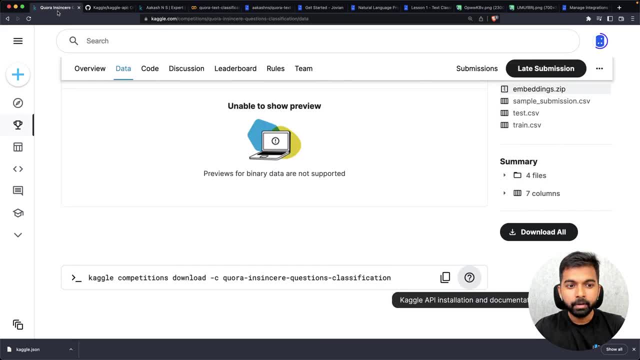 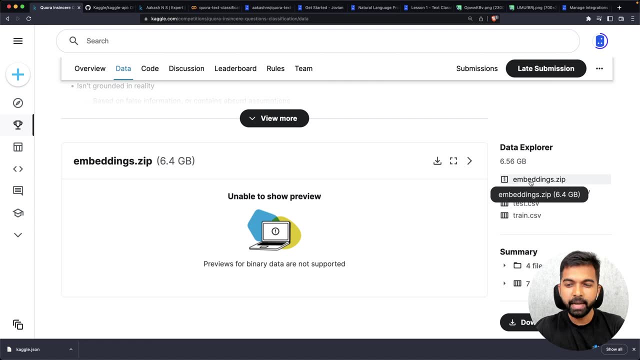 Now one last thing. there seem to be a bunch of files here, So then there seem to be a traincsv file, testcsv file, sample submission, and then embeddingszip file- Okay, Okay. So now I want to download just the file, traincsv. 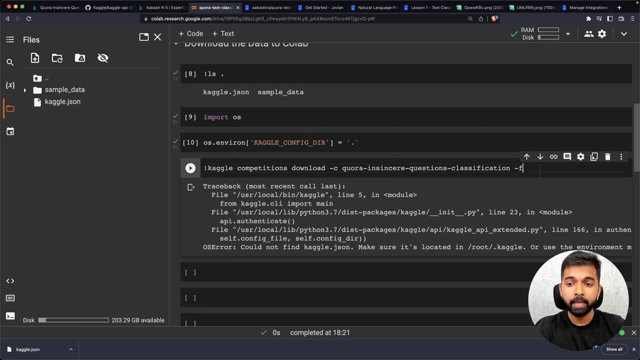 So the way I can indicate that is by typing minus F, traincsv. So that's one thing I'm going to do, And another thing I can do is also put in where I want this data to be downloaded. So I'm just going to download it in the folder, in a folder called data. 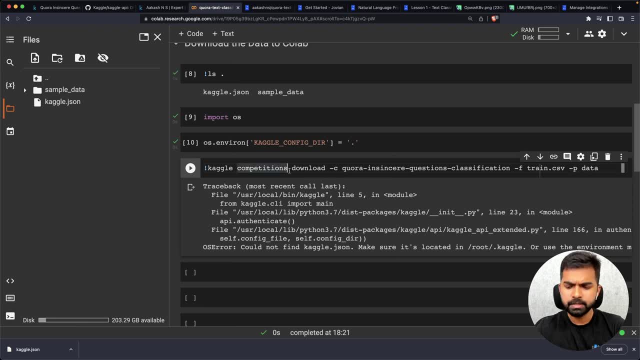 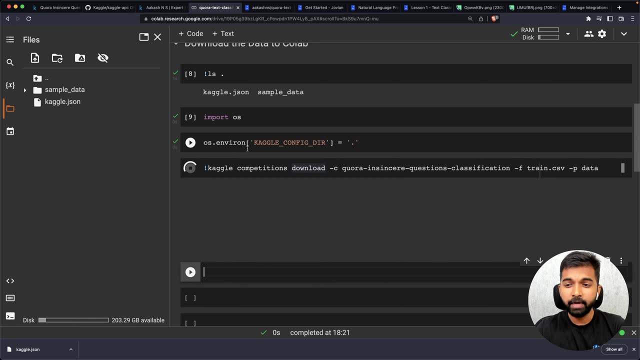 So minus P data, All right. So let me run that. Kaggle: competitions, download minus C, Cora and sincere question: classification: minus F traincsv, minus P data. And where did I find out this? minus F and minus P? Well, all of that is given here. 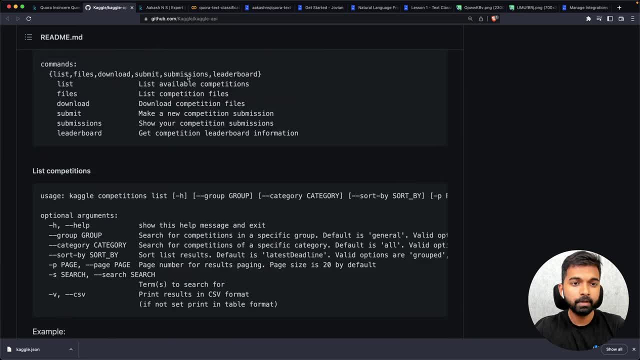 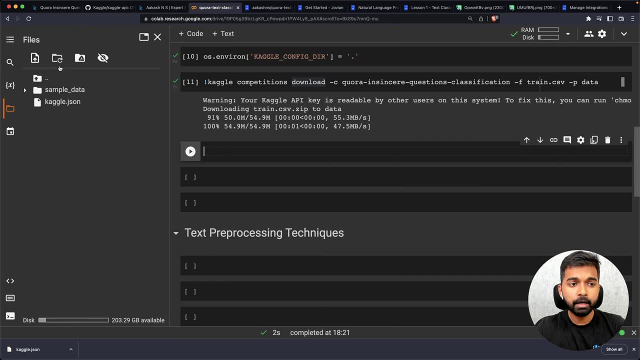 If you just scroll down and check the documentation, so you'll get used to reading documentation. It's not too difficult. It's just something, a list of steps that you have to follow. All right Now, if we click refresh here, you can see that a folder data has been created. 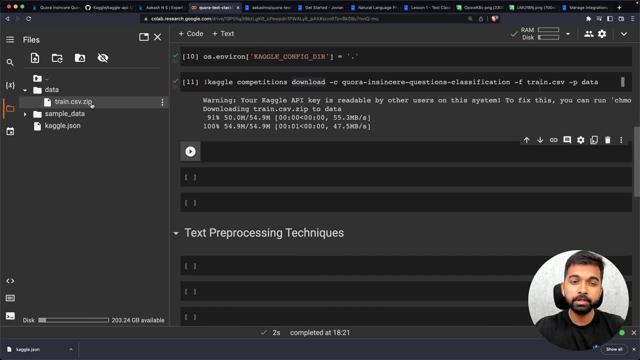 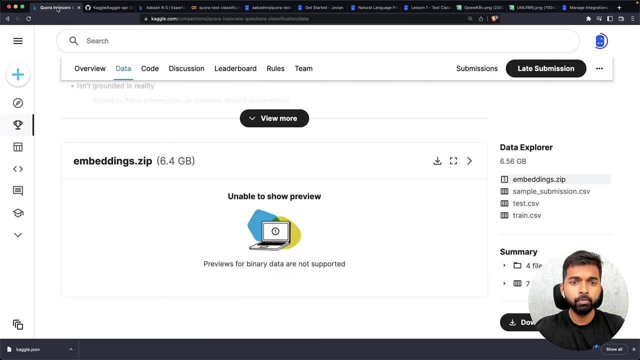 And in that folder, data, a traincsvzip file has been created. Similarly, I can now copy over this command and there are a few more files. So there's a file- testcsv, and sample submissioncsv And sample submissioncsv. Let's download those as well. 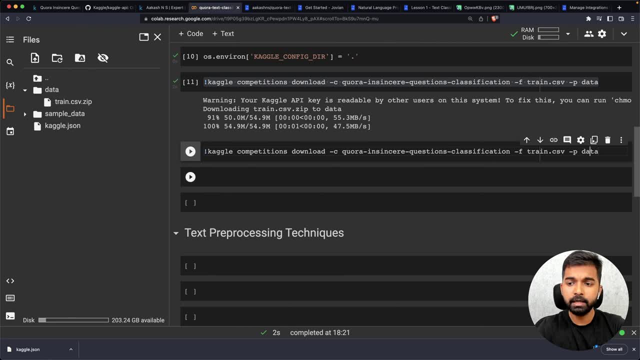 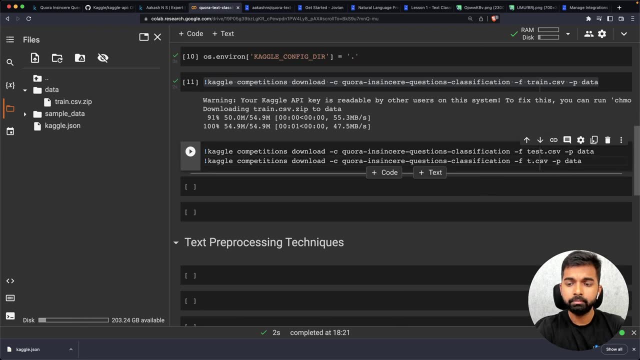 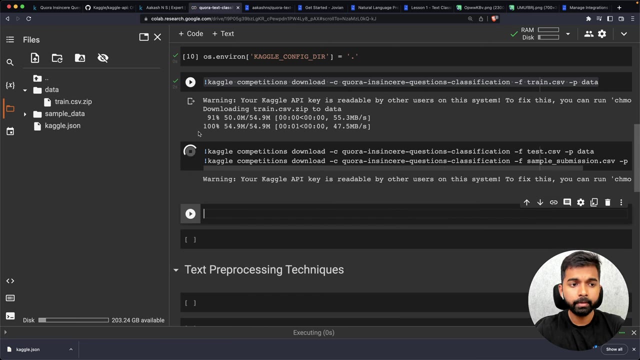 I'm going to come in here, I'm going to say testcsv, and I'm going to come in here and I'm going to say sample submissioncsv. All right, let's run that, And in a moment we should have both the testcsv file and the sample submissioncsv file. 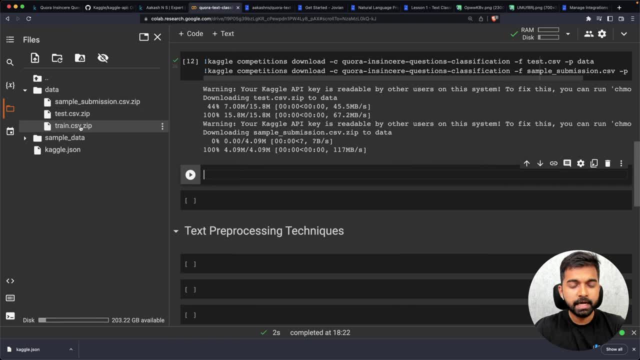 So now, at this point, we can see that Each of these files has been downloaded as a zip file. So if we want, we can unzip these files, but the pandas library that we're going to use for exploring the data can actually work directly with zip files. 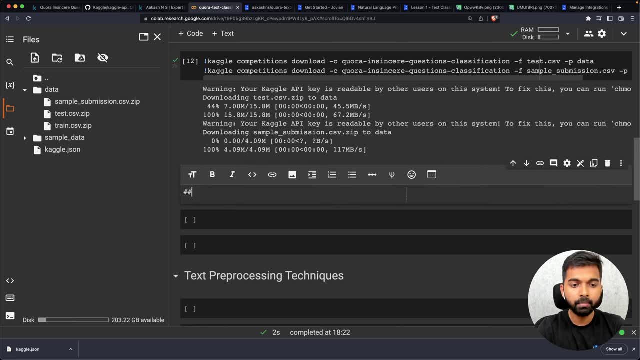 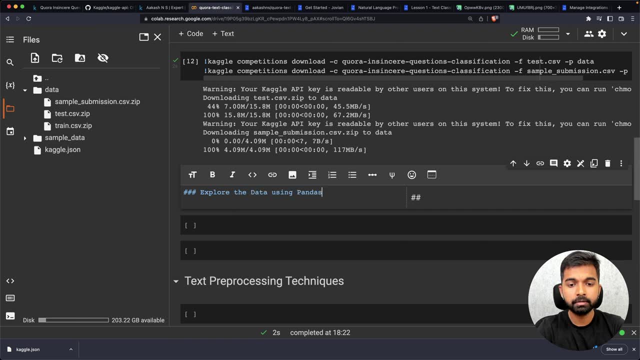 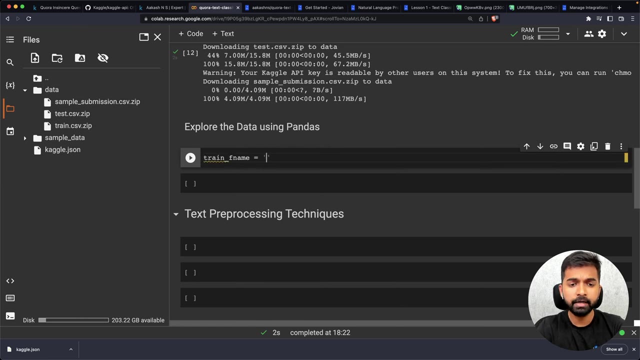 So we don't need to do that. So let's start exploring the data. So the step two is to explore the data using pandas. Okay, So first I'm going to create a few variables: Trainfname, train file name. That is simply. 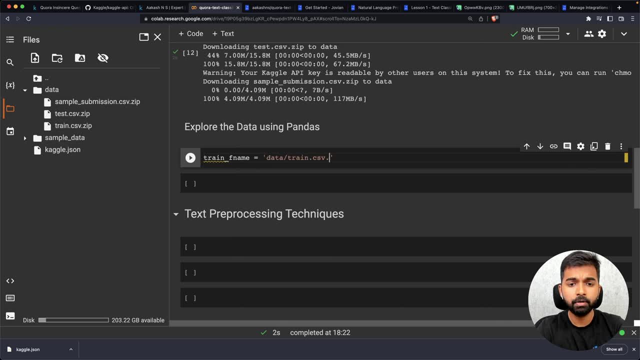 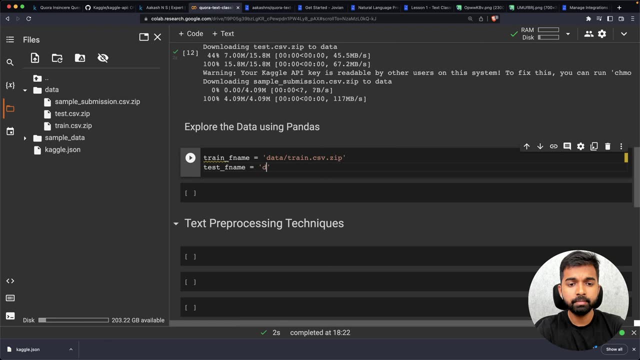 Data slash- traincsvzip. I'm going to create a variable testfname. That is simply data slash- testcsvzip. And finally, I'm going to create a variable called samplefname. So we are now just creating variables. We're not still loading the files. 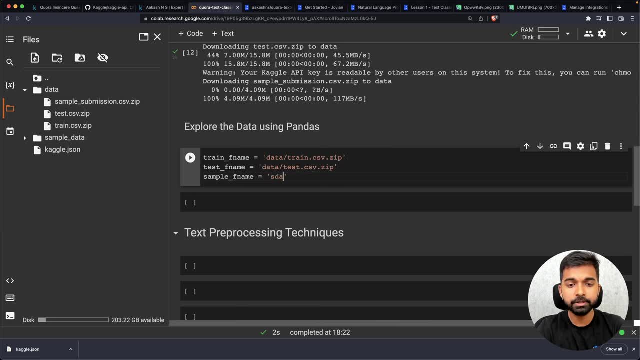 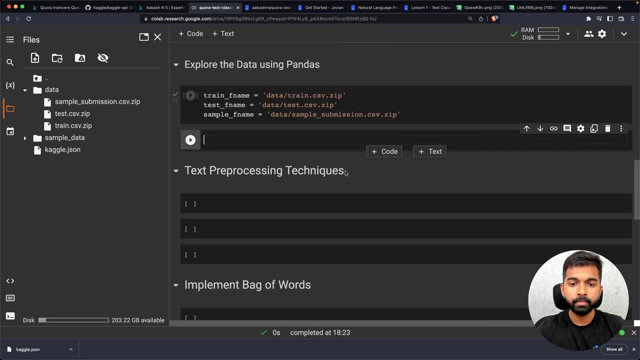 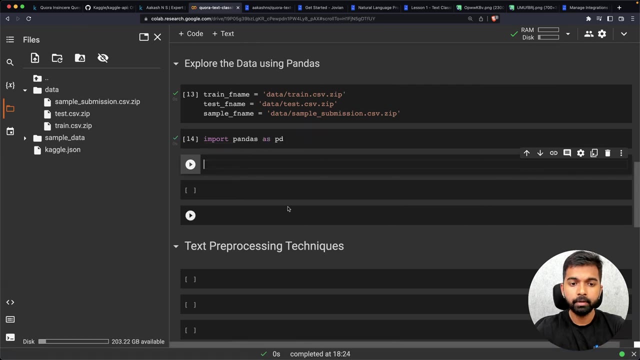 Sample slash or data slash: sample submissioncsvzip. Okay, Now let's import the pandas library. So let's say, import pandas as PD, And now we can create a data frame. So first I'm going to create this data frame called raw DF, because this is going to contain all the raw training data. 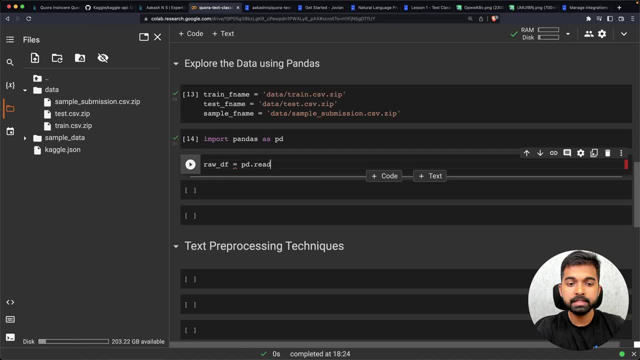 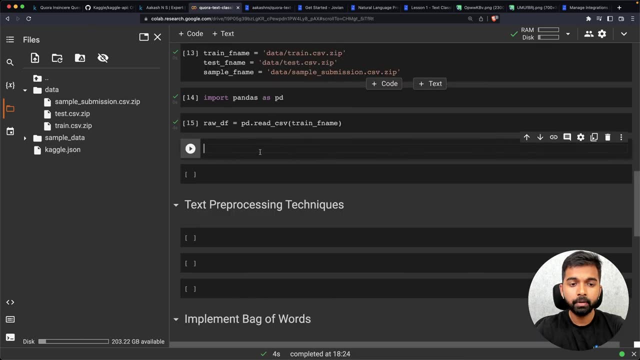 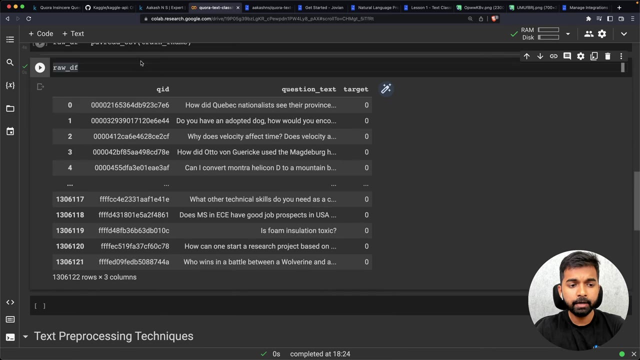 So raw DF is PD dot read CSV, and PD dot read CSV requires a file name, So I'm going to provide train fname. Okay, Let's look at raw DF now. This is coming from the traincsv file, Okay, As mentioned here, and it looks like it contains 1.3 million rows, specifically 1,306,122 rows. 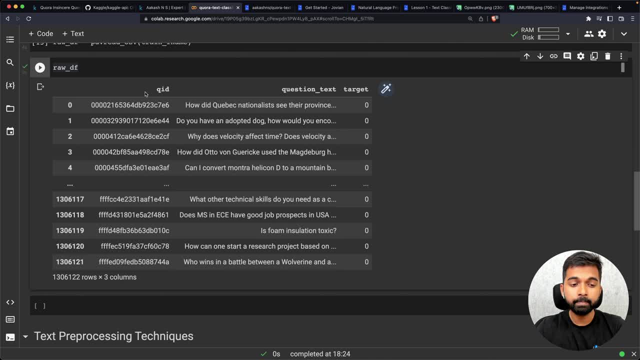 So that's a lot of data that is provided to us for training. And it contains three columns, and the three columns are Q ID or question ID, So Cora has given each question a unique question ID. Then there is a question text. So this is some question text. 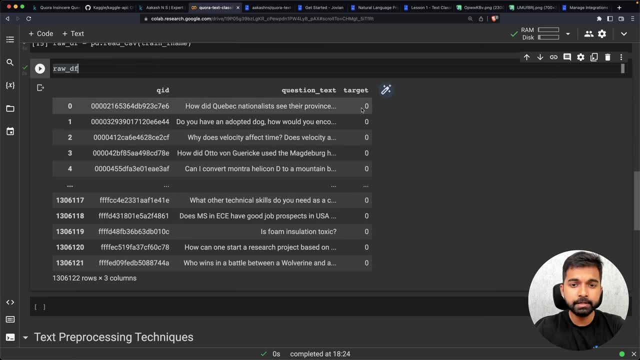 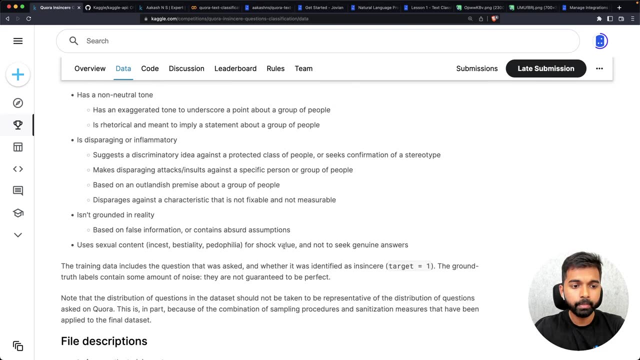 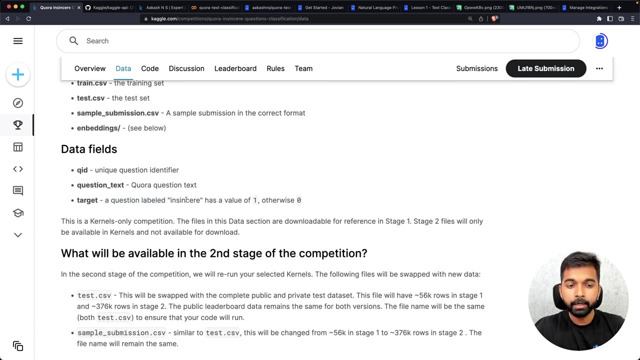 It contains a question ID, It contains a question text and it contains a target. Now, what does this target represent? Looks like it's either Zero or one. Well, if you go down into data and come down here, you can see that the third field target indicates. one indicates that a question is insincere and zero indicates that a question is sincere. 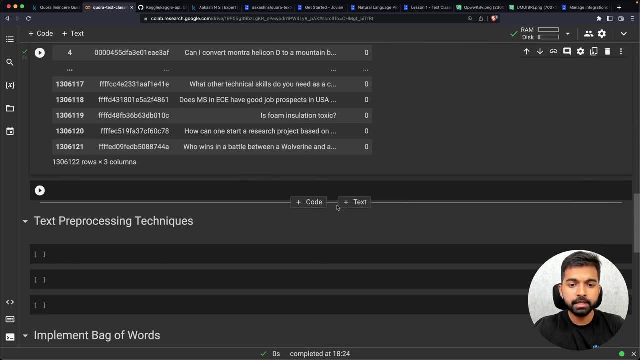 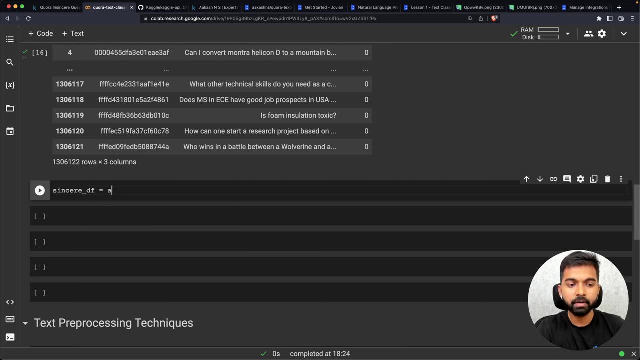 Okay, So let's look at a few sincere and insincere questions. Let's create a sincere DF first, containing the sincere questions. So this would be raw DF and from raw DF. We want to check raw DF. dot Target equals zero. 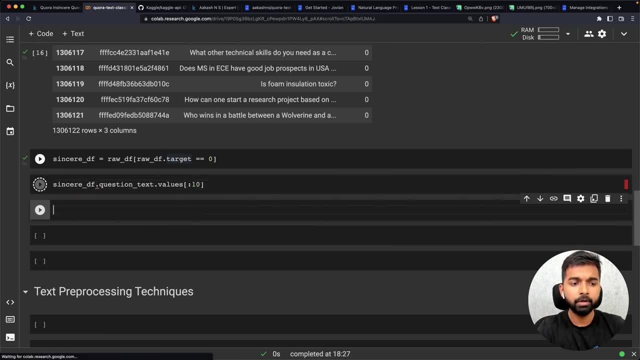 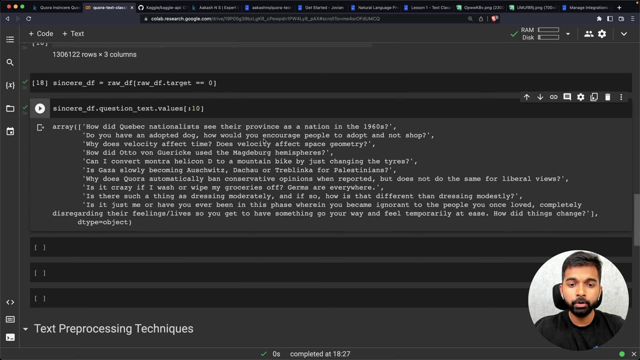 And let's look at sincere DF dot question text: dot values 10.. So here are 10 sincere questions. Do you have an adopted dog? How would you encourage people to adapt, adopt and not shop? How did auto and use the Mandenberg hemisphere, et cetera? 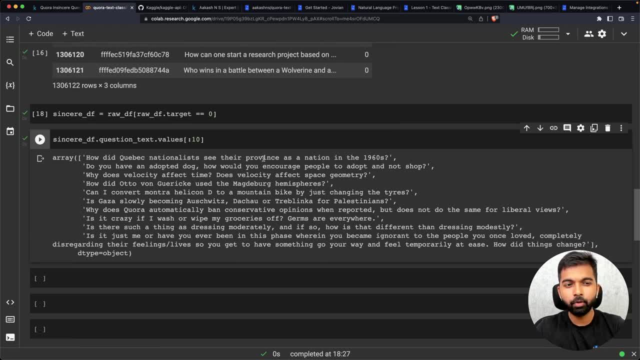 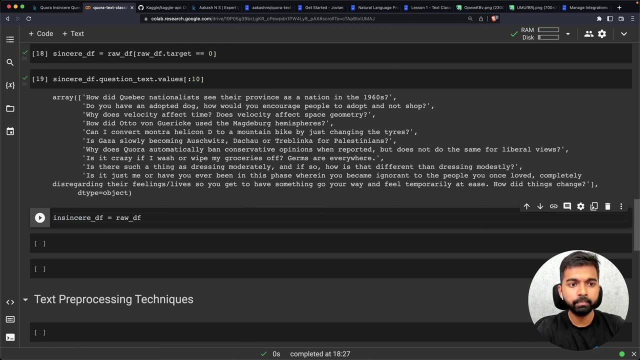 So these all look like fairly decent questions, questions that Cora would want to have, And let's also find insincere questions. So insincere DF equals raw DF. Once again, raw DF dot target equals one and insincere DF dot question text, dot values. 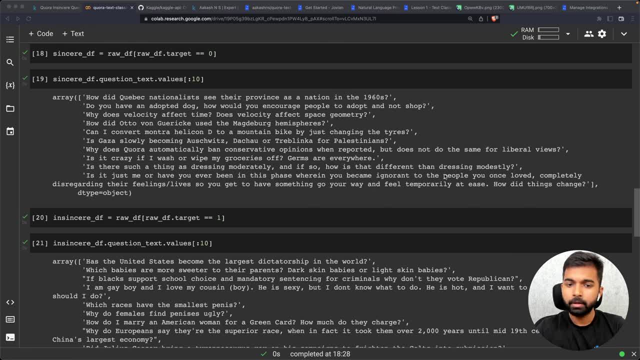 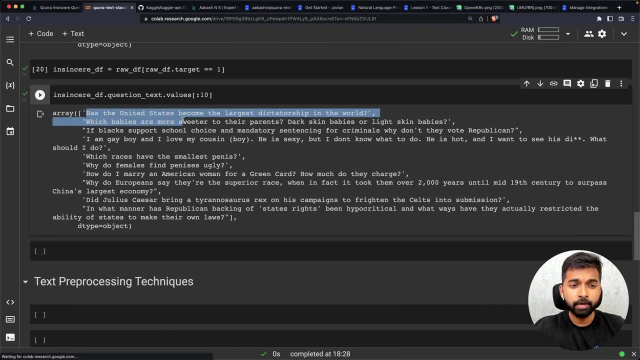 And let's look at that. Okay. So here are some draw, Here are some insincere questions. So it says: has the United States become the largest dictatorship in the world? Clearly this is an implication, not a question. This question looks racist. 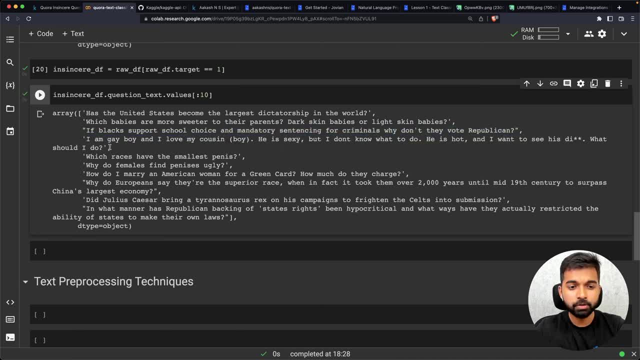 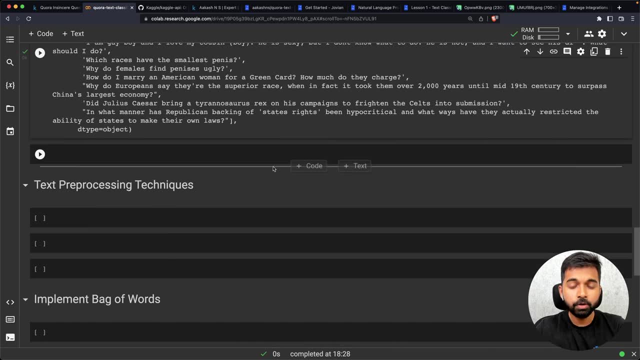 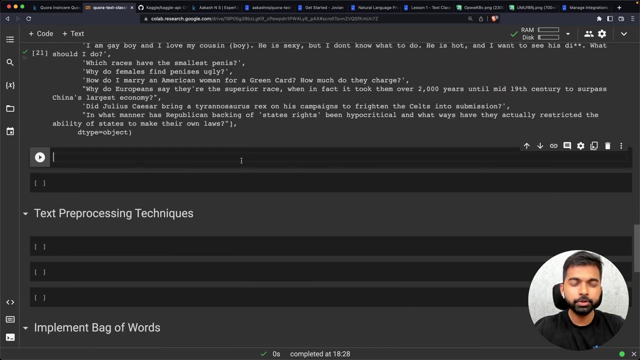 This question looks politically motivated. This question is a quiz homophobic. This question is racist again. So you can see that there are a lot of racist and sexual and content questions. So we obviously want to detect and avoid these kinds of questions. Let's look at, maybe, the distribution of sincere and insincere questions. 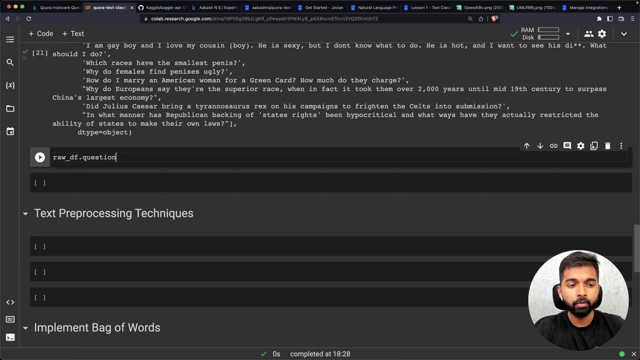 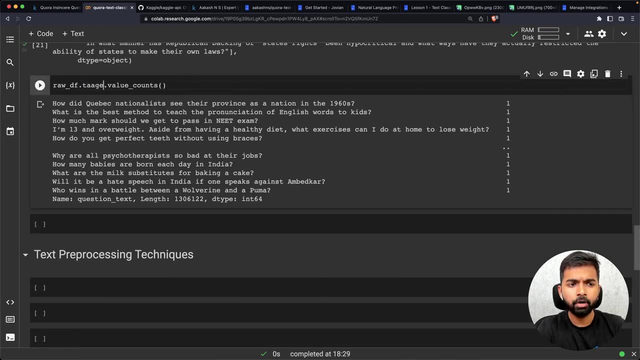 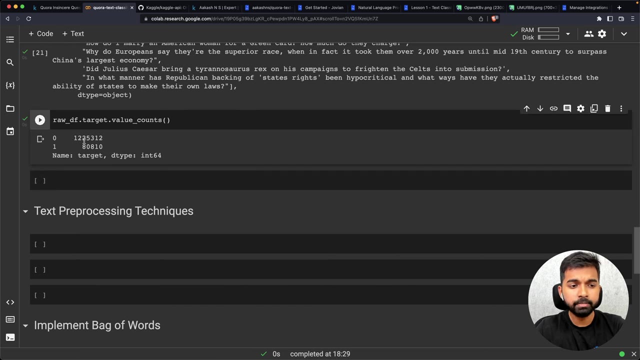 So once again, if I go to raw DF and I look at question text and I just check value counts and okay, I want to do target dot value points, not question text, So you can see that zero occurs 1.22 million times, whereas one occurs only 80,000 times. 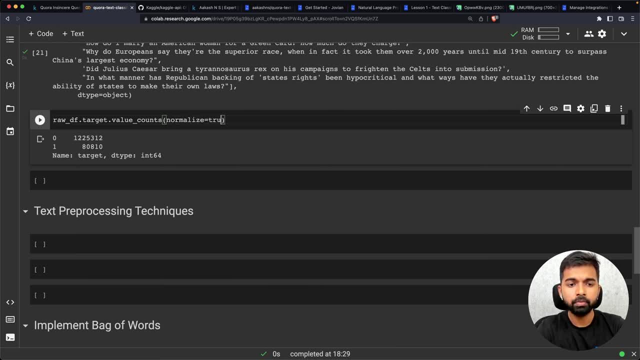 You can also set normalize equals true and just study the fraction. So in this case, about 93% of 94% of questions have the value zero as a target, which means 94% of questions are sincere and only about 6% of questions are insincere. 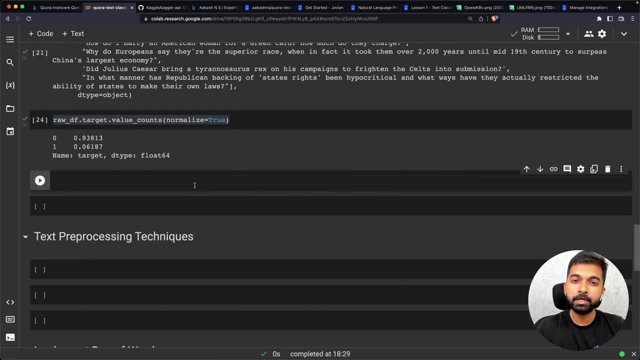 And this is why, whenever you're training a model or some kind of a text classification system, accuracy may not be a good metric to evaluate that system. Because if you always predict zero, if you always detect a question as sincere and predict zero, then you will have 94% accuracy and you may think that's a good accuracy. but you can get. 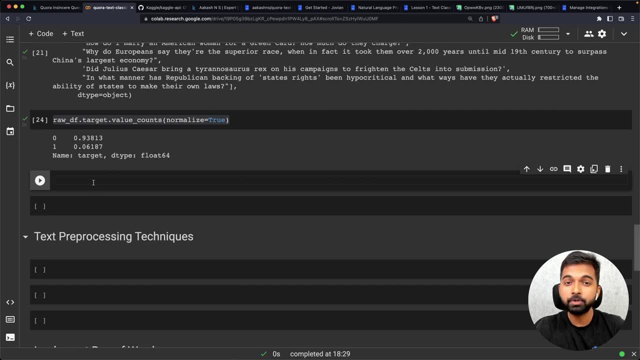 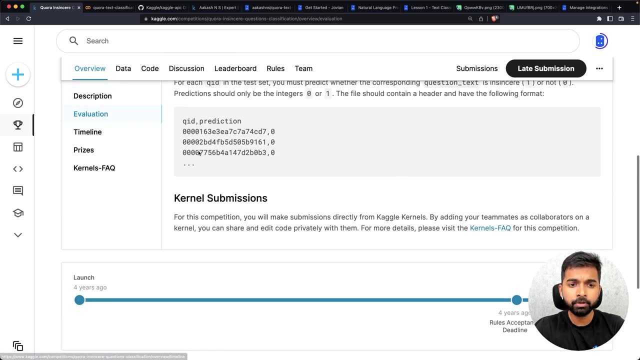 94% accuracy just by predicting zero for everything. So that's not good at all. That is why, if you go back into the competition and check the overview and check the evaluation column, you will see that the submissions made to this competition are evaluated on the F one score. 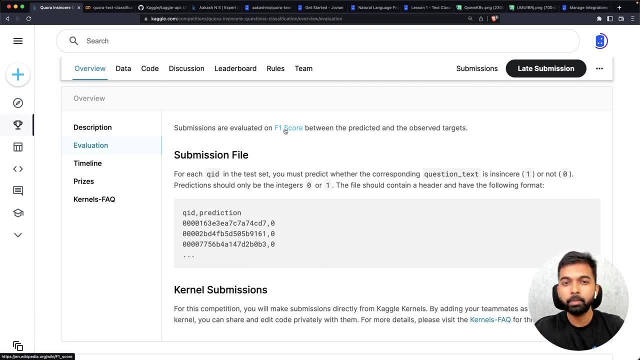 And the F one score is a formula which uses something called precision and recall internally. Now we don't need to worry about all of those things. Um, for now, let's just think about F one score as Cora's way of evaluating your questions. 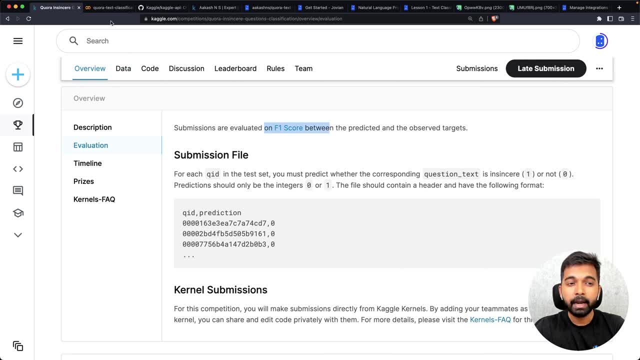 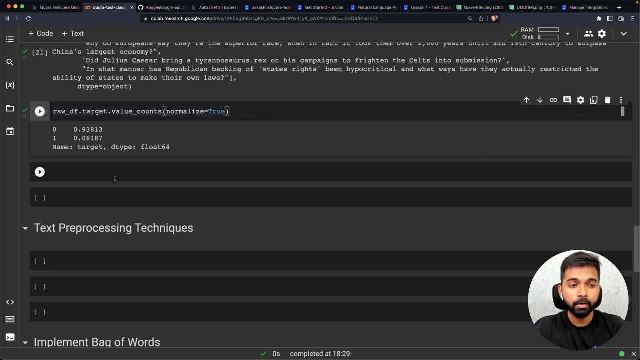 Uh, evaluating your submissions and your predictions, and that is somehow better than accuracy. Okay, Later at some point we will also get into what the F one score and precision recall mean. Okay, So that's a little bit. we've learned about the raw data frame. 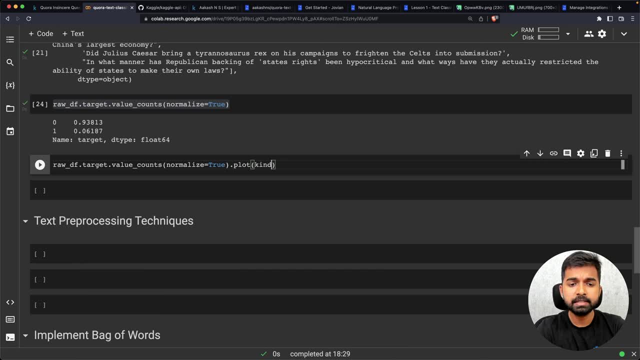 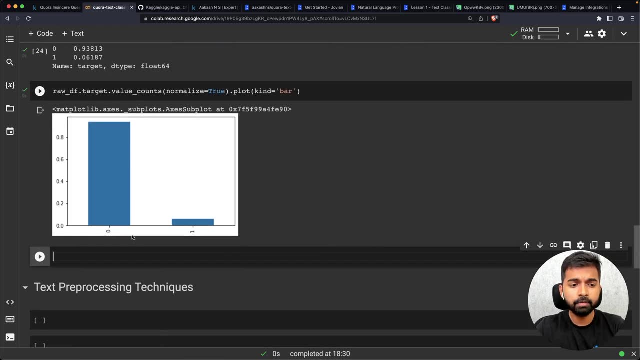 Now, one other thing we can do is we can also plot it as kind equals a bar, So this is also a good way to visualize the data. So here we have, for example: uh, the two classes zero and one. So zero has a fraction of 0.9 and one has a very small fraction. 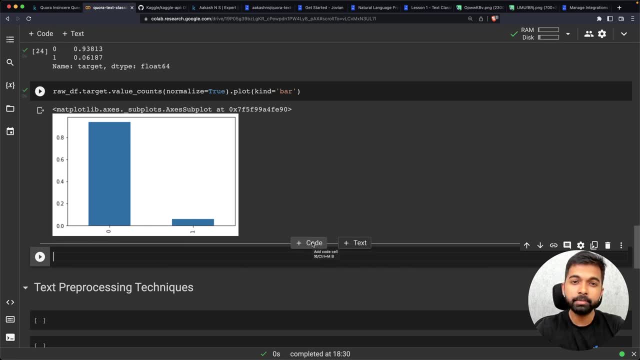 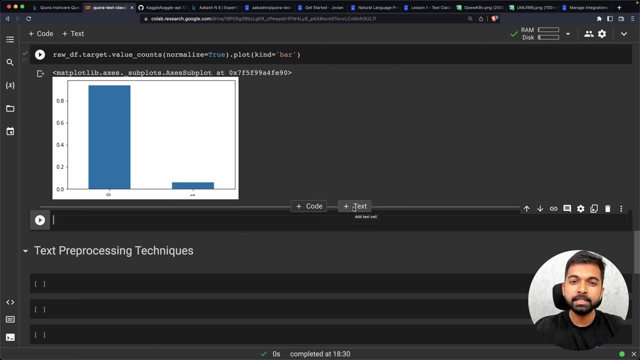 And there is some way we may want to read this class imbalance when we're building a machine learning model. But for now this is enough exploration. I encourage you to explore a little more, find out things like what is the average length of every question? 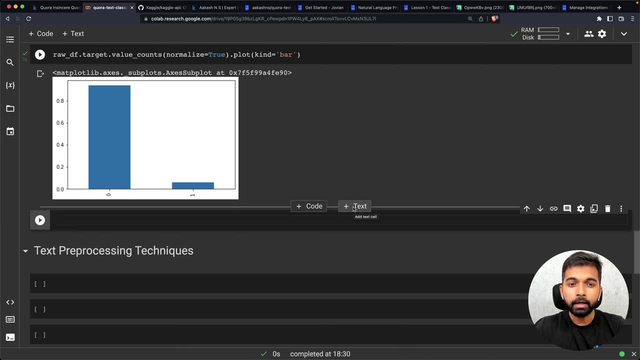 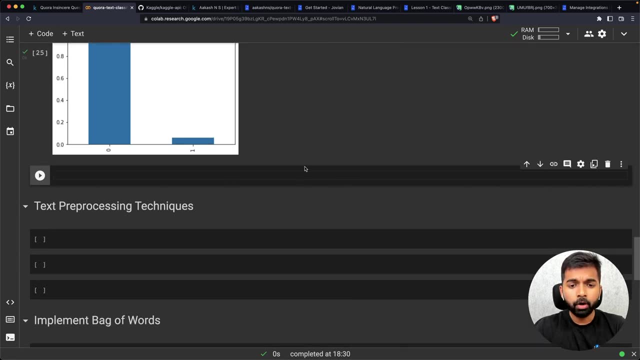 Find out like: um, what is, what are the most common words that are occurring in each question, and things like that. Okay, Now, apart from the raw data frame, which was the train dot CSV file, we also can create a test. 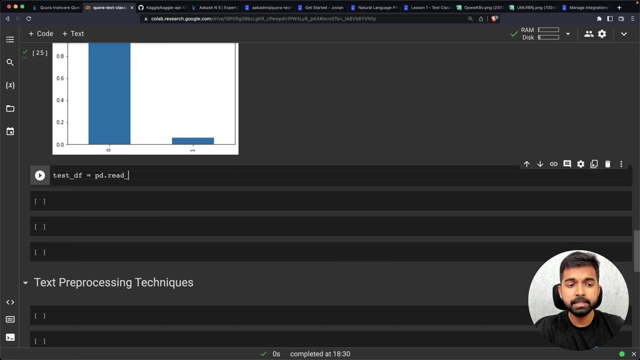 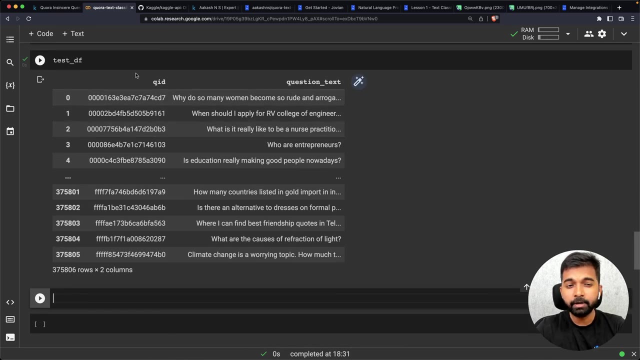 Data frame. So let's get the test data frame, which would be PD, dot, read CSV, And we have the test F name, which contains the file name of the test data frame, And here is a test data frame. And now the test data frame contains a question ID and the test data frame contains a question text. 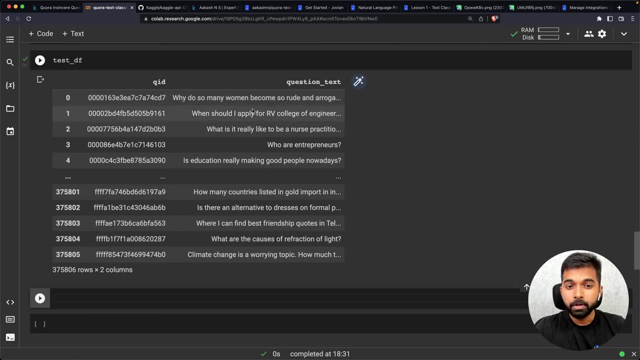 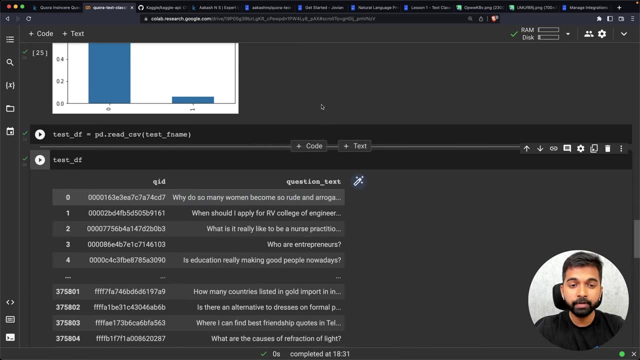 However, it does not contain any target. So what you are supposed to do is read the test data frame And, once you have created An automated system for text classification by processing the training data frame, you have to make some predictions on the test data frame. 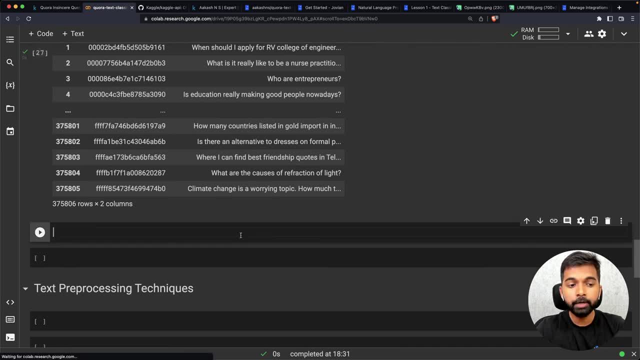 So for each question you need to make a prediction and then you need to create a submission file. So let's create a data frame called sub DF, which is PD, dot, read, CSV, sample submission. Well, what is it called? Let's see. 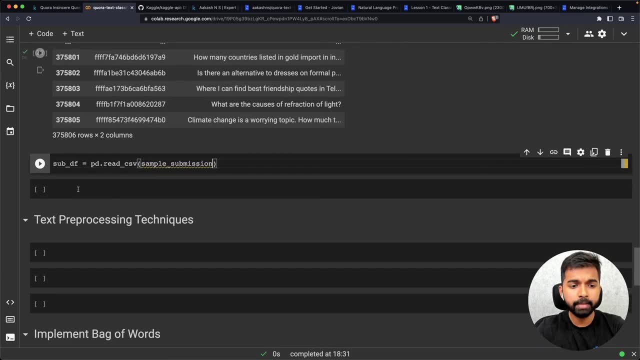 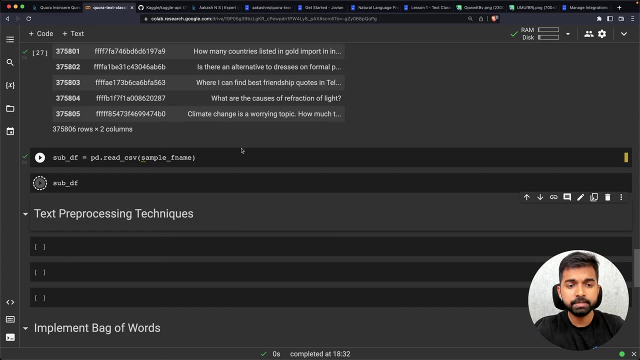 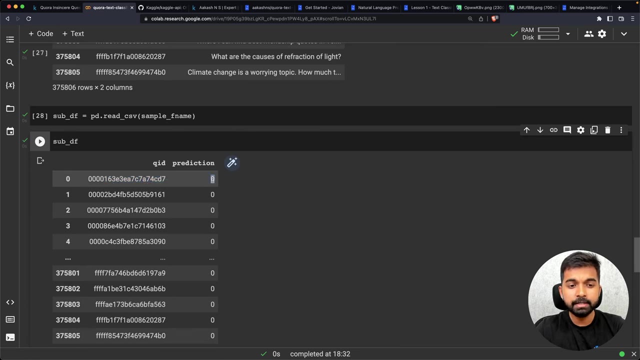 So, um, okay, Sample F name, right? So let's just call it sample F name And let's look at the submission data frame or the submission CSV file. So the submission CSV file contains a question ID, Q ID, and then it contains a prediction. 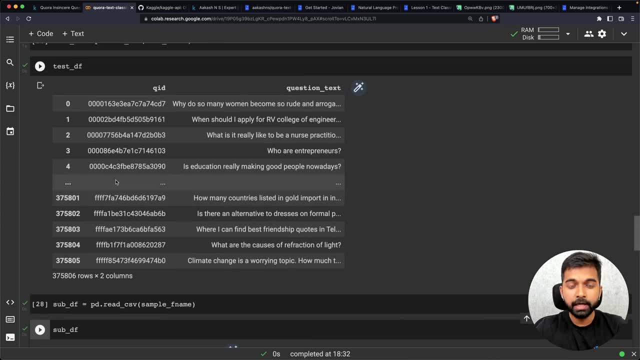 So here's what you have to do. This is a sample submission, but what you have to do is train a machine learning model or build a text classification system using the tagged questions in the or the labeled questions in the training data set, then make predictions for each question within the test data frame. 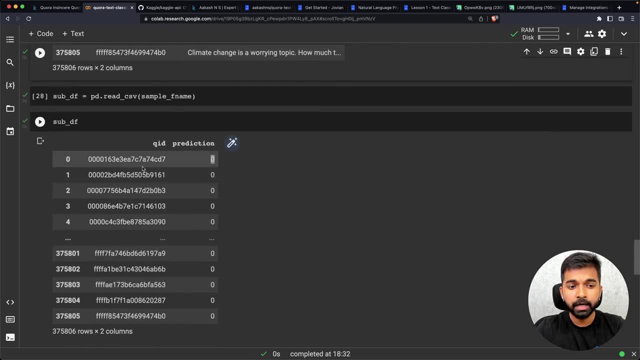 And see that each question has a question ID and you'll find the question IDs from the test data set here in the submission sample file And then, against each question ID, create a prediction, generate a CSV file and submit that CSV file to Kaggle. 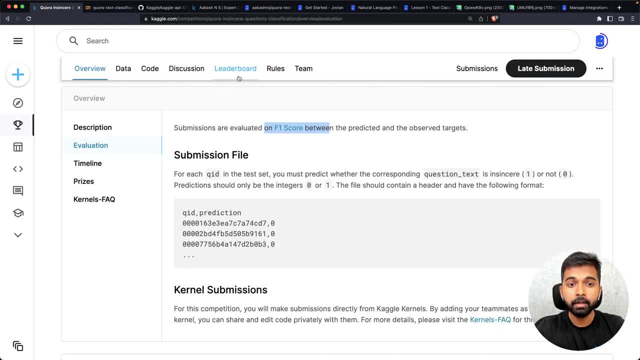 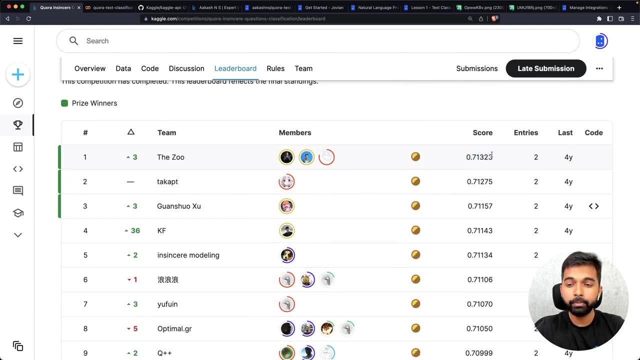 And then you can see where you stand on the leaderboard. You can see where you stand on the leaderboard and your submissions will be evaluated and an F1 score will be computed. So the highest F1 score is 0.71.. So you can make submissions and see where you land. 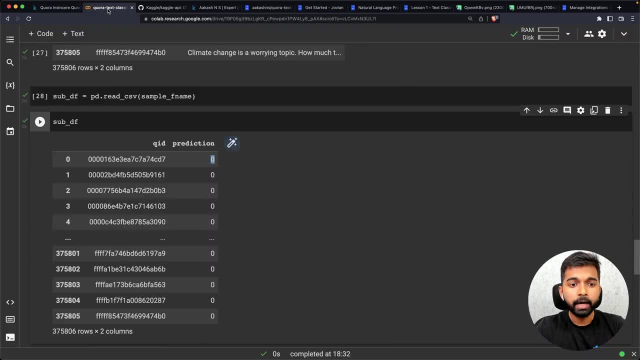 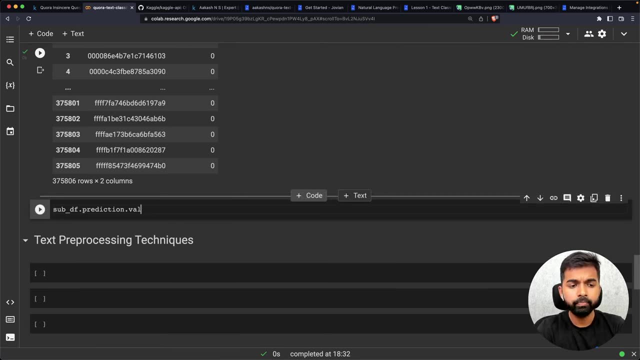 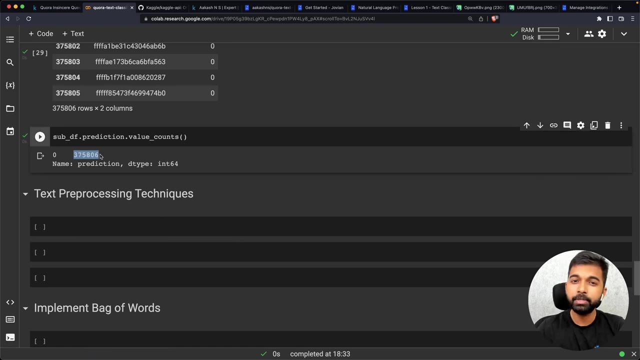 Okay, On the leaderboard, All right. So now we have the submission data frame and the sample submission. If you just study the prediction column value counts, you'll notice that it contains all zeros. It just contains all zeros. Obviously, the submission file that we create should have something other than all zeros. 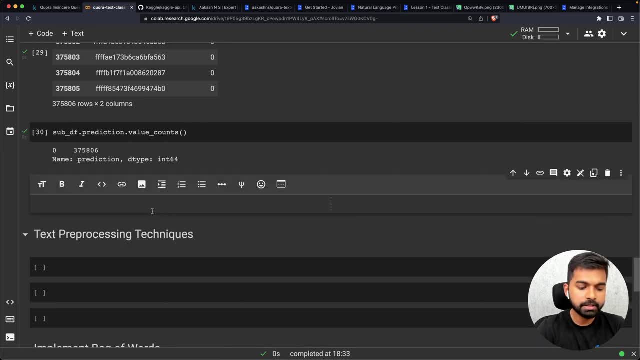 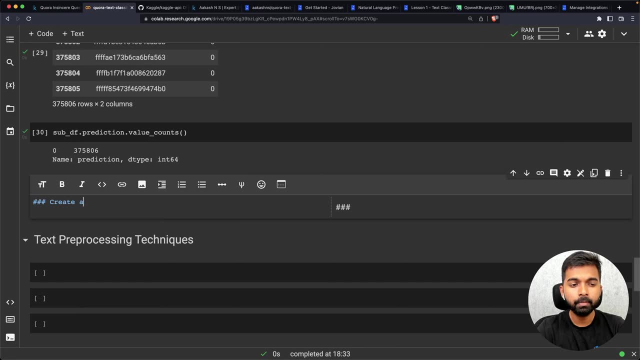 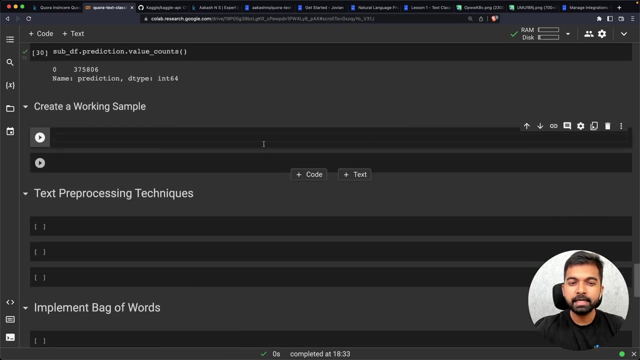 Okay, So that was the second part, which was exploring the data set. Now the final thing we'll do is create a working sample. Okay, So because this contains 1.3 million rows, working with this data set can become a little difficult. 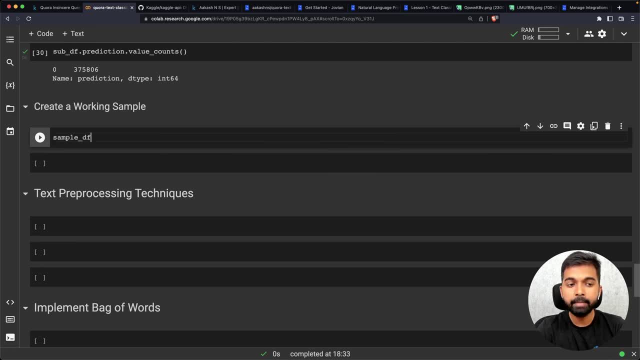 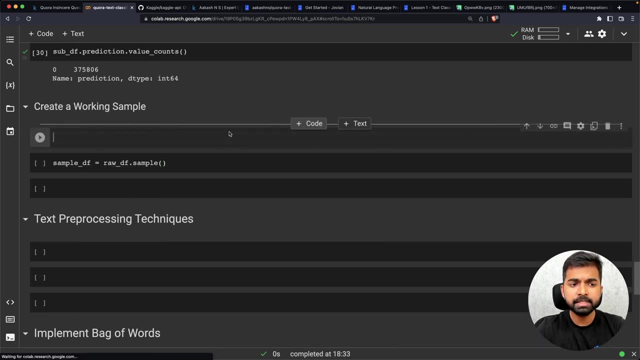 So that's why we're creating a sample data frame. So I'm going to say: sample DF equals raw DF, dot sample And I'm going to give it a sample size which I'm going to keep configurable. Sample size equals a hundred thousand. 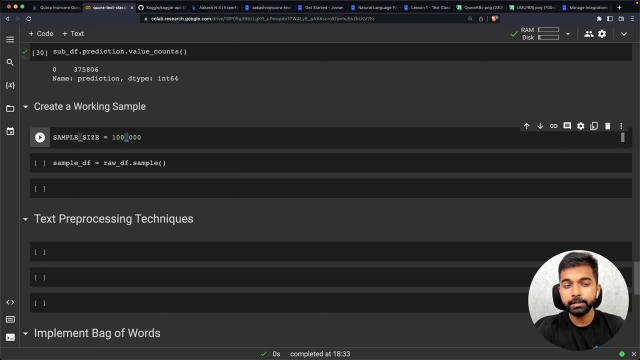 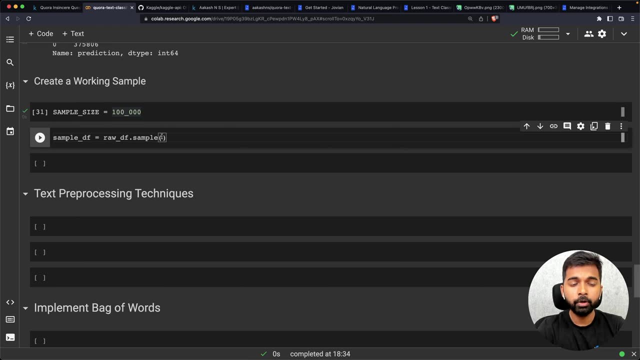 So here's another way to type the number: a hundred thousand. I can type a hundred And then underscore instead of comma. So a hundred underscore thousand, and Python will treat it as the number a hundred thousand. So I'm going to create a sample. 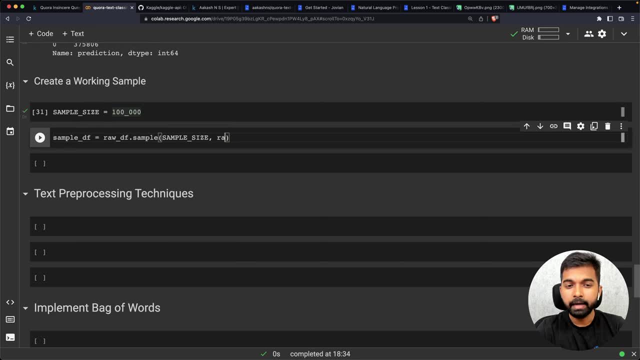 I'm going to create a sample of size, sample size And just so that I get the same sample every time, I'm going to set something called a random state. Okay, No, don't worry, if this doesn't make sense, you can even ignore this. 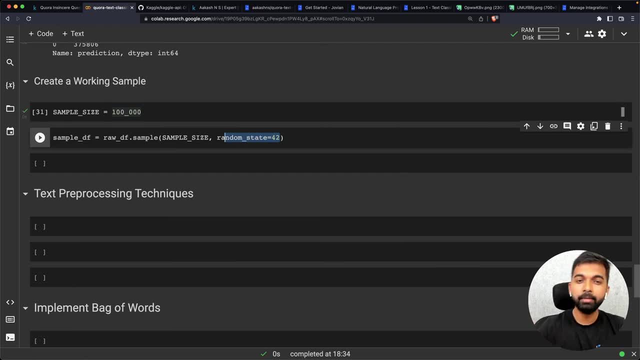 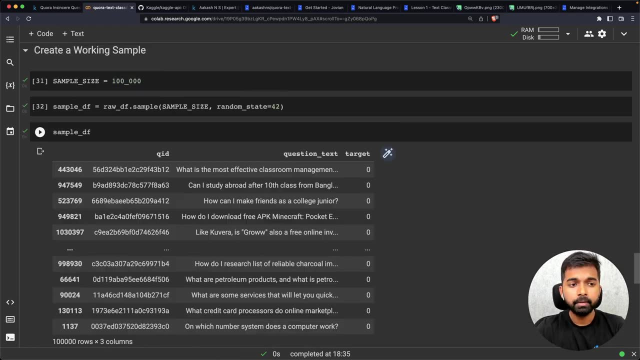 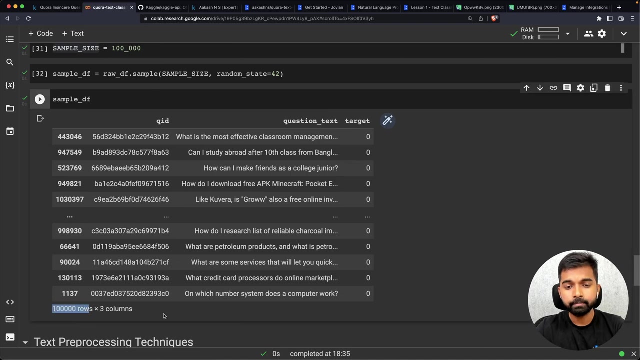 All it does is it makes sure that, as random sample is picked, but each time I run this code, each time I run the notebook, the same sample gets picked. Okay, And let's look at the sample DF. So this is the sample DF, and the sample data frame contains a hundred thousand rows of data that we're going to work with now. 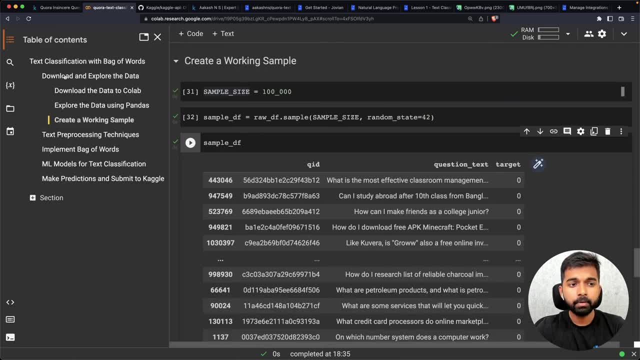 All right. So that was part one which was downloading and exploring the data. We downloaded the data to Google collab. We explored the data using pandas and you can continue exploring And, in case you want to learn pandas and you can check out our course on data analysis and. 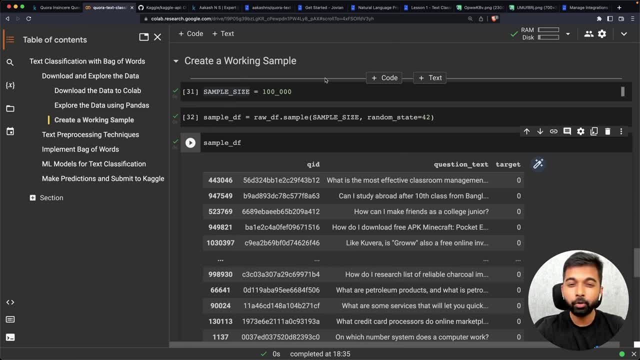 Visualization with Python. It is at the location zero to pandascom And you can also just go to jovianai- sign in and you can find the free course. And finally, after exploring the data, we also created a working sample of the data. 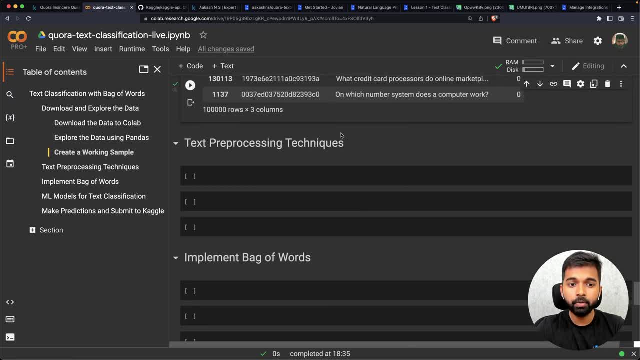 Now this would be a good time to save our work. So I am just going to go in here and click file save, command S, and that is going to save the file for me, And once I save the file, I can come back here. 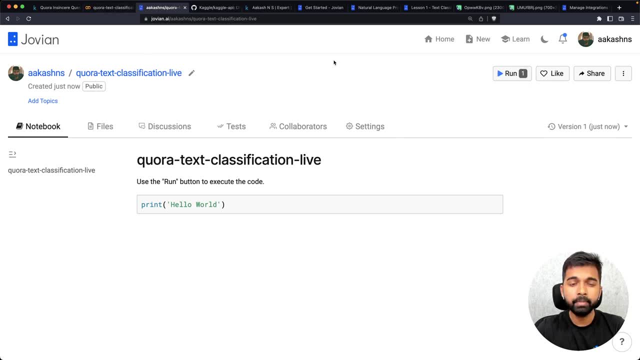 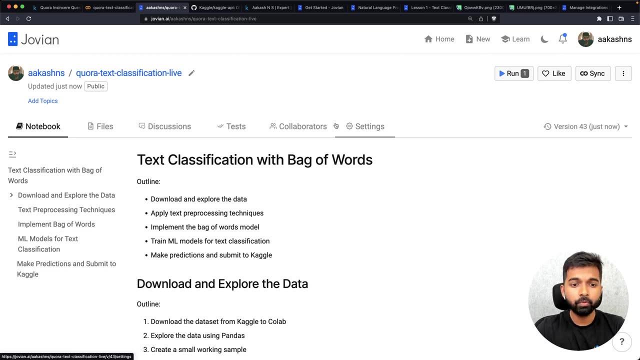 Remember, we created this project on Jovian and then we ran it on Google Colab. So if I come back here and I just reload the page once again, you will notice that the new version has been captured. So every time you save the changes on Colab within your Google drive, 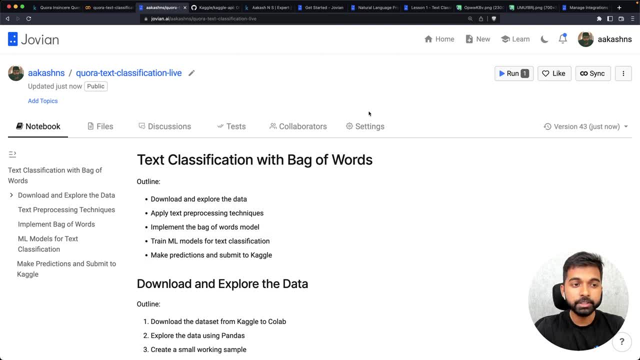 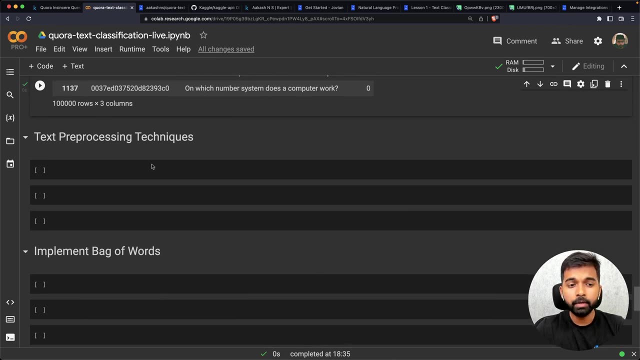 Jovian will automatically pick up the changes and record a new version, Not just now, but Colab also does a lot of auto saving, So all the versions that have been saved in between have also been recorded All right. so now that we have saved our work, we can continue and look. 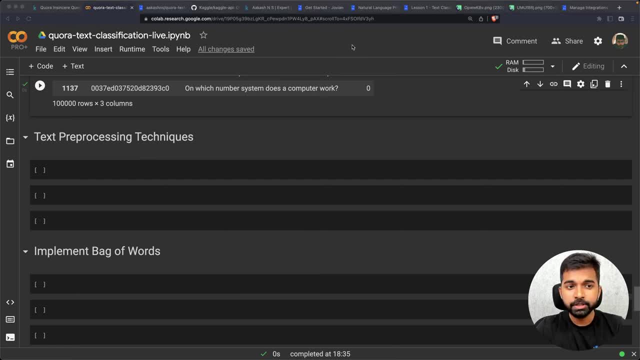 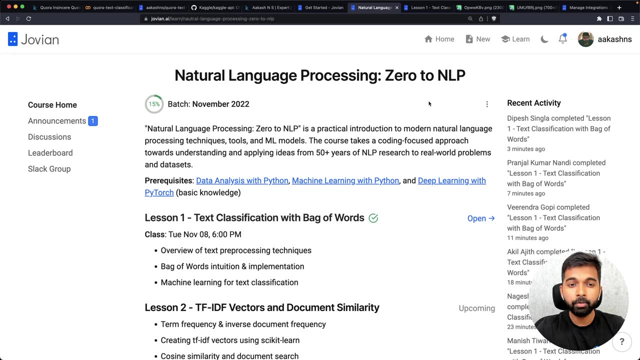 at some text pre-processing techniques. Now, one other thing I want to mention is if you're not enrolled in the course already, please go to zero2nlpcom and click enroll- So you'll see an enroll button here- and enroll into the course, because we are 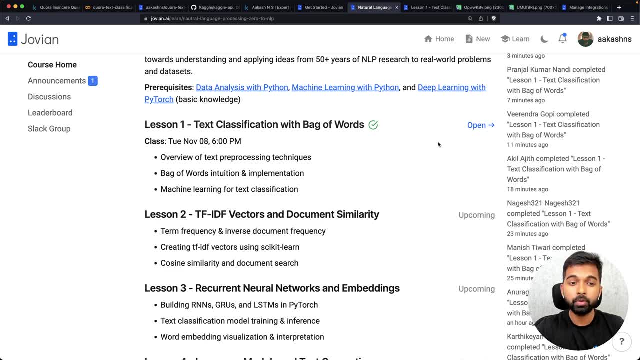 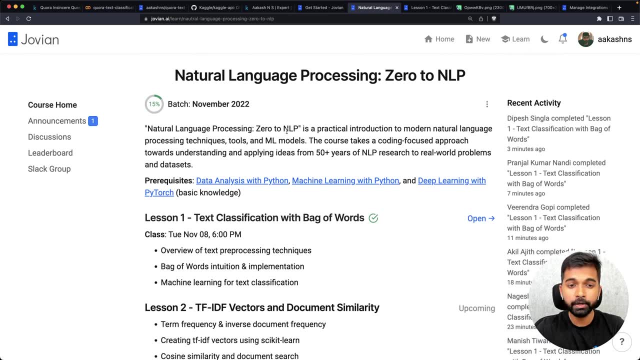 going to have lessons every week And we are also going to have assignments, and to submit these assignments you will need to enroll in the course, and you're also going to build a project and you can also have discussions. So there's a lot here, but do go to zero2nlpcom and enroll into the course. 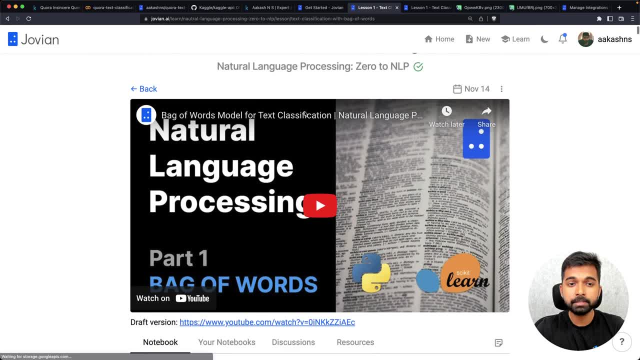 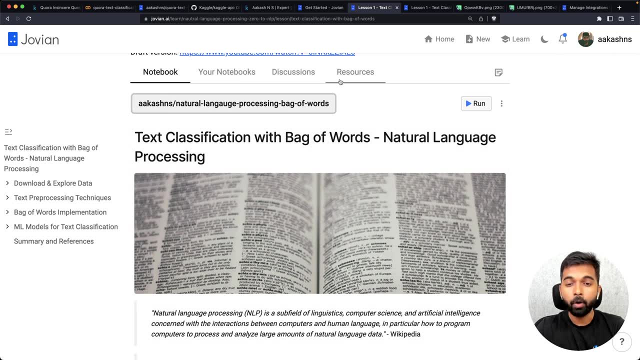 Specifically, we are looking at lesson one, text classification with bag of words, and you'll find the recording here And you will also find the notebook, the code that we're writing today, available here. All the links that we are using today are available in the resources tab and you can. 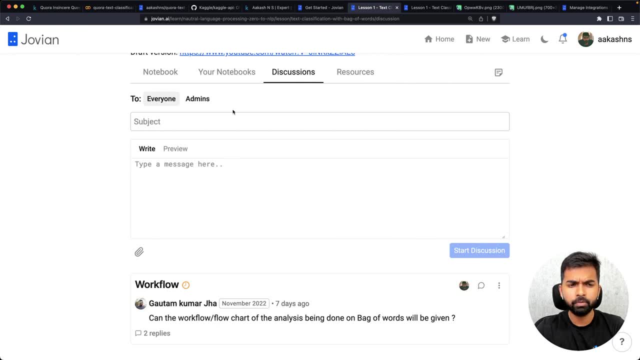 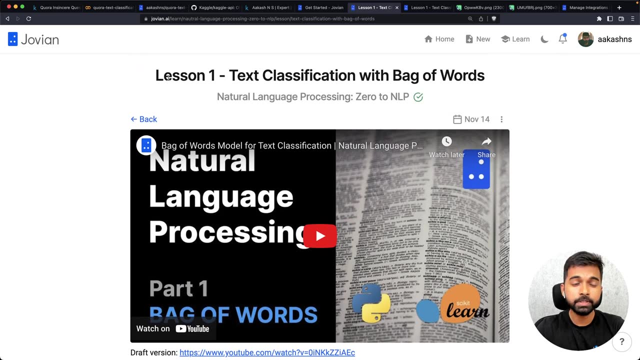 go into the discussions tab and you can ask questions about anything you wish. So do head over to zero2nlpcom and enroll into the course, And Please invite your friends to join the course as well, if you've liked the lesson so far. 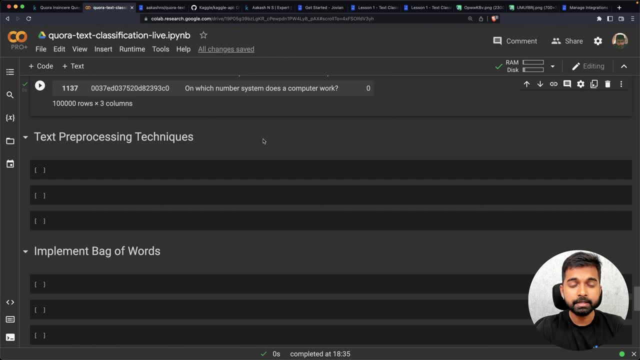 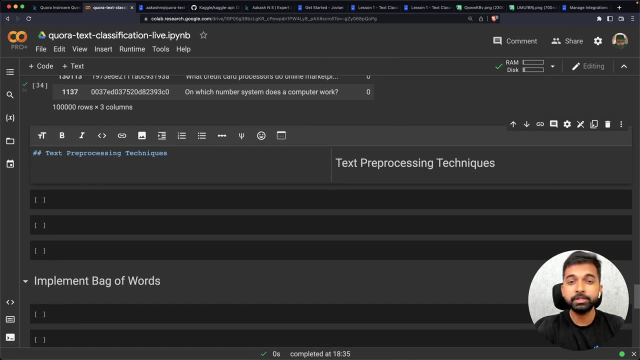 Okay, So coming back to text pre-processing techniques, So now we have looked at, now we have downloaded the data and now we're onto the section, the second section, text pre-processing. So here's what we are going to do in this section. 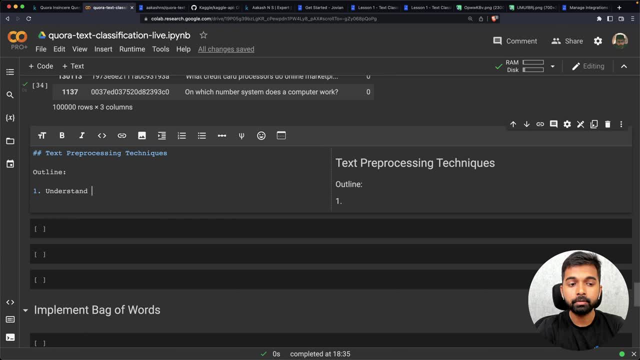 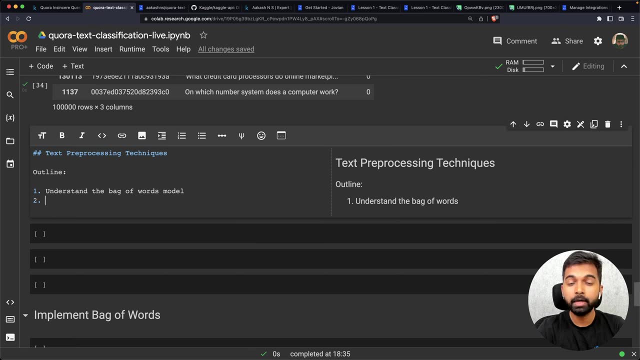 First, we are going to understand the bag of words model. This is a word that we have been throwing around for some time, So we're going to understand how it works. We're going to gain some intuition about it. Next, we're looking at something called tokenization. 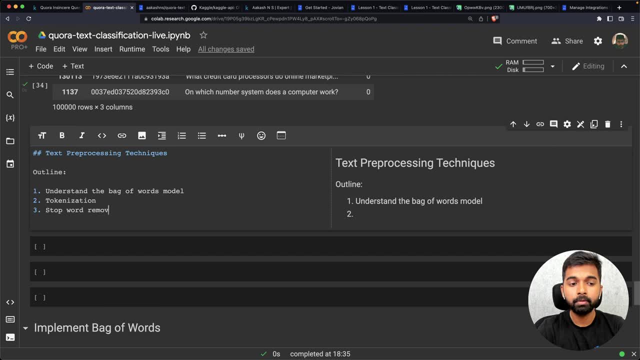 Then we're looking at something called stop- word removal. And then, finally, we are going to look at something called stemming. Okay, Don't worry if these words don't make sense, we're going to look at them in a moment. So here is how the bag of words model works. 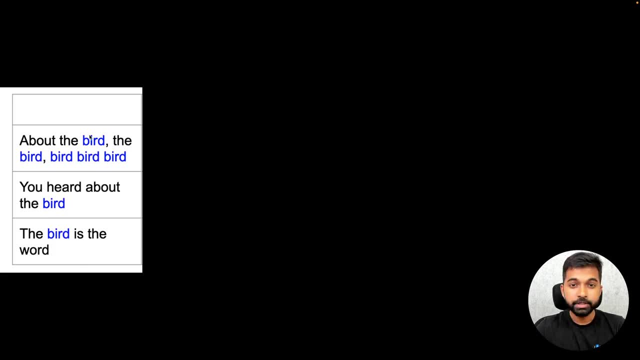 Let's say we have a dataset containing three questions or three sentences. Here is the first sentence. your sentence is about the bird: the bird, bird, bird. It doesn't really make sense. This is a made up example, but just go with it for now. 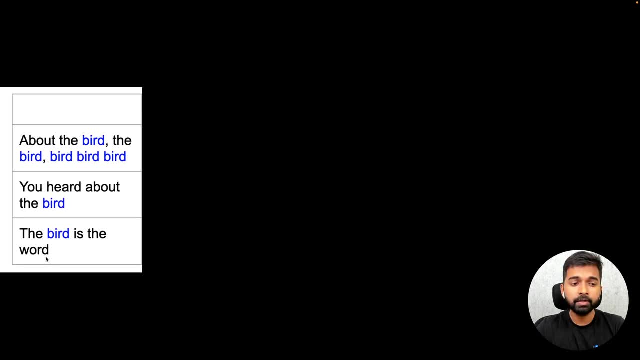 Then the second example in our dataset is: you heard the bird, And the third example is that the bird is the word. So here we have 1.3 million data set. here We have 1.3 million questions in the Cora insincere question classification dataset. 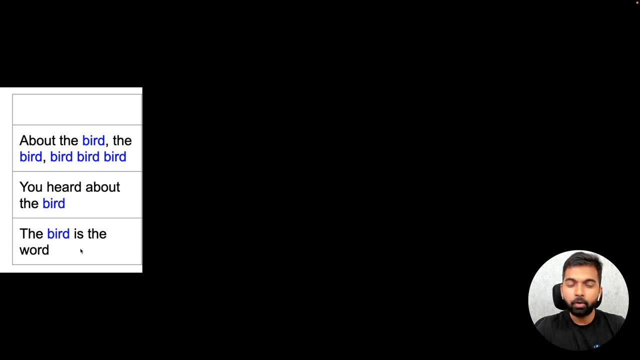 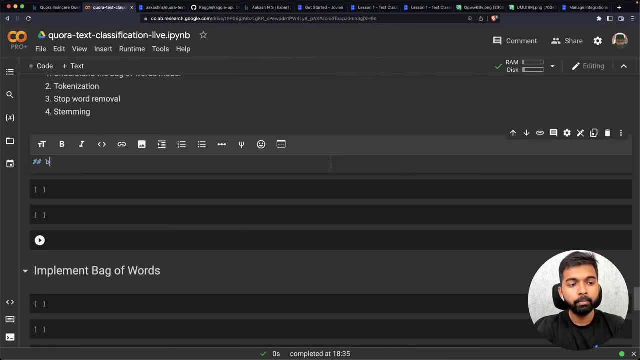 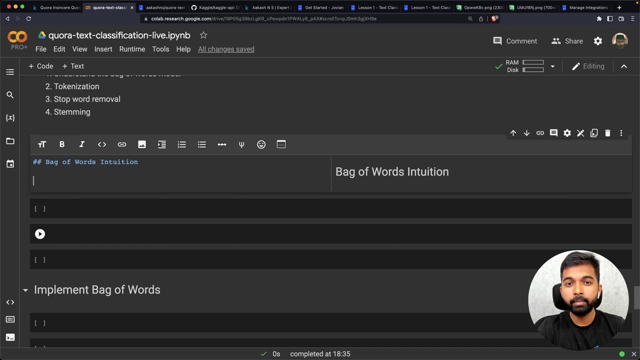 In this sample dataset we have only three, but the concept still applies. So here is how you build a bag of words model. So let's just create a section called bag of words intuition. And here is how you build a bag of words model. 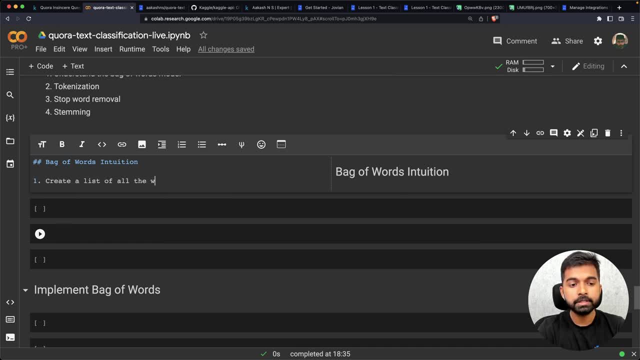 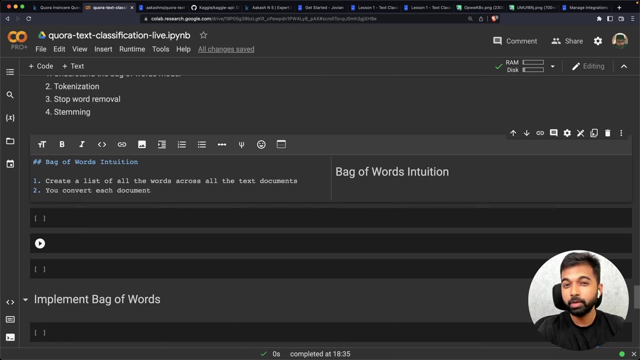 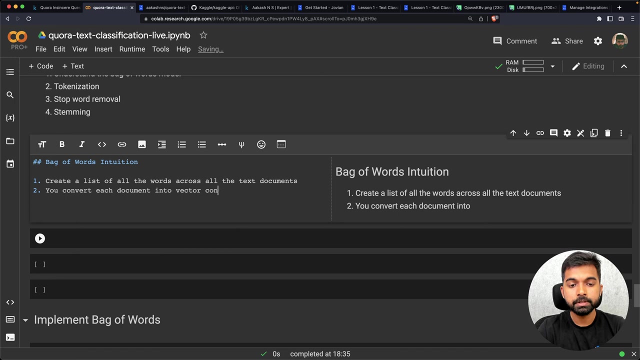 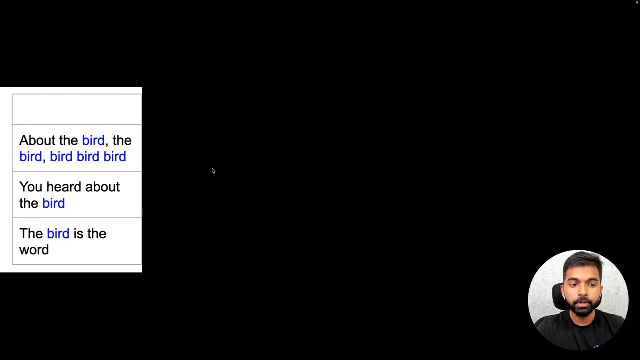 One, you create a list of all the words across all the text documents. Second, you convert each document- or each question in this case- Into a vector containing the counts of each word. Okay, So let's see that in action here. our dataset consists exactly of three documents about the bird: the bird, bird bird. 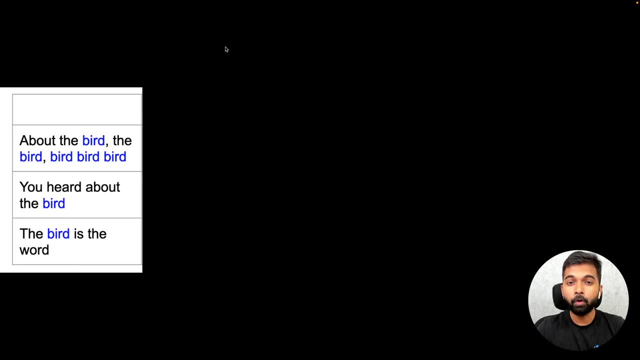 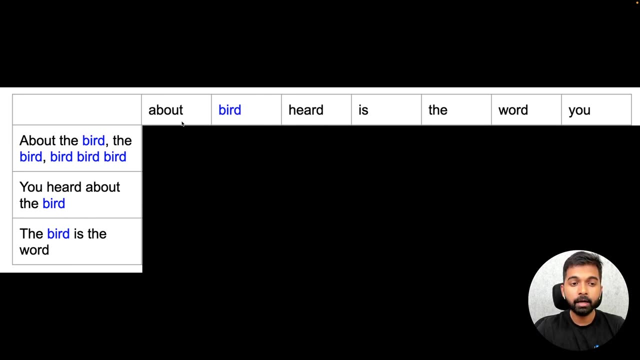 You heard the bird and the bird is the word. Step one is to make a list of all the words present in all the documents together, all the unique words. So here are all the unique boards that are present here about bird Heard is the word you. so these are all the unique words that are present across this dataset. 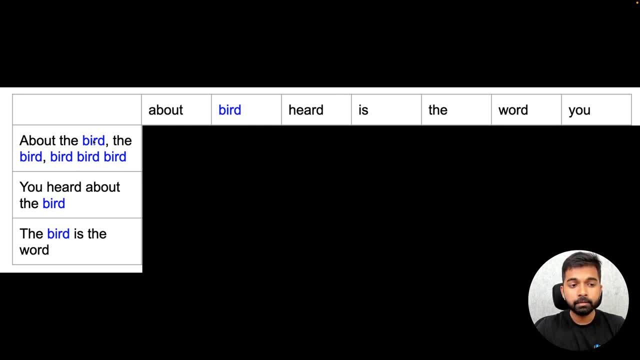 Then we have to convert each of these X documents into a vector. Why a vector? because machine learning algorithms can only understand numbers. computers work with numbers, So we have to turn this text into numbers, so that then we can train machine learning models on it. 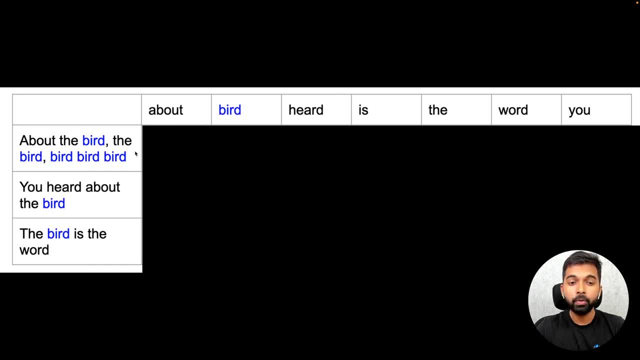 So how do we turn this text about the bird, the bird, bird, bird- into Numbers? Here's how we do it: We count how many times the word about occurs. It occurs once. we count how many times the word bird occurs. 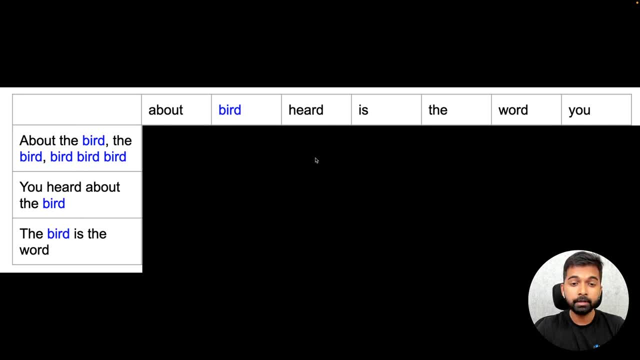 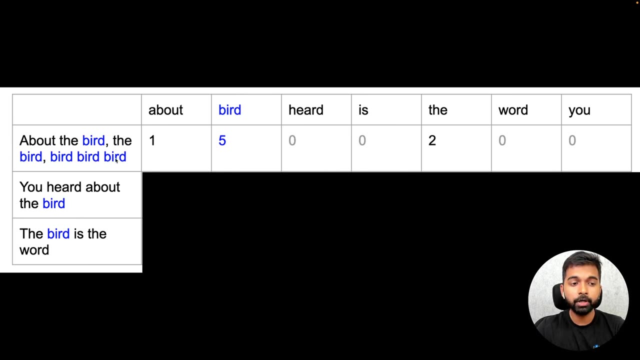 It occurs one, two, three, four, five times. How many times hard occurs. It occurs zero times. is occurs zero times. The occurs one time. word occurs zero times. you occurs zero times, So the occurs two times. So now you see the sentence about the bird, the bird, bird bird gets converted into this vector: 1, 5 0, 0. 2 0, 0. 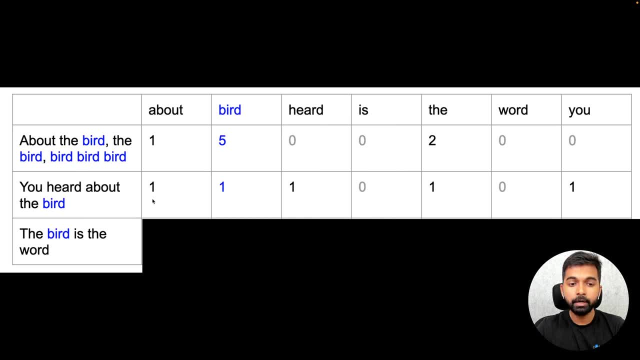 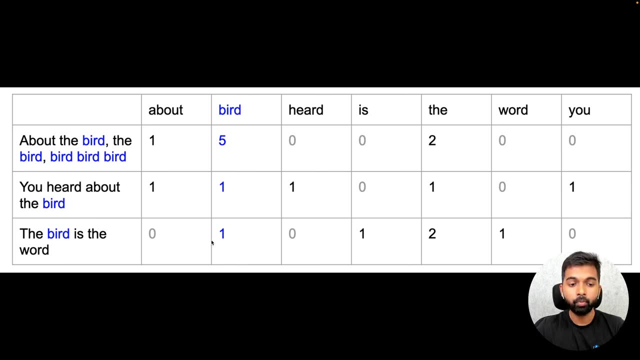 Similarly, you heard the bird gets converted into 1 1, 1, 0, 0, 1 0, 1.. The bird is the word. gets converted into 0 1, 0, 1, 2, 1, 1.. Why? 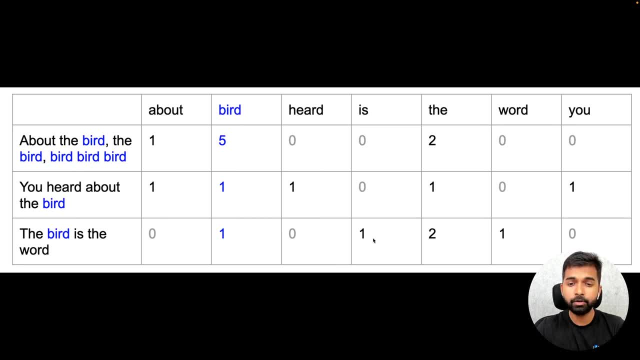 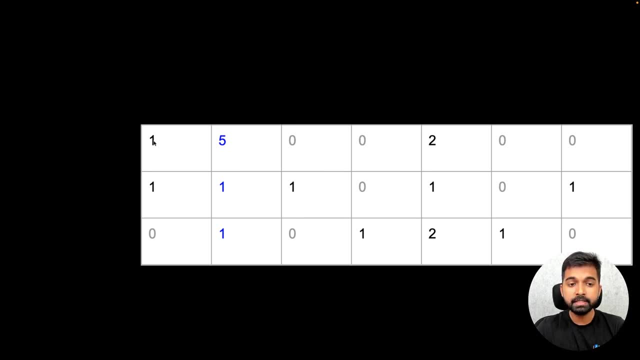 Because it doesn't contain the word about. it contains bird ones. It contains her zero times. It contains the twice is once and word once. So now what we are left with is these vectors. each of the sentences or the documents in the dataset have been converted into vectors. 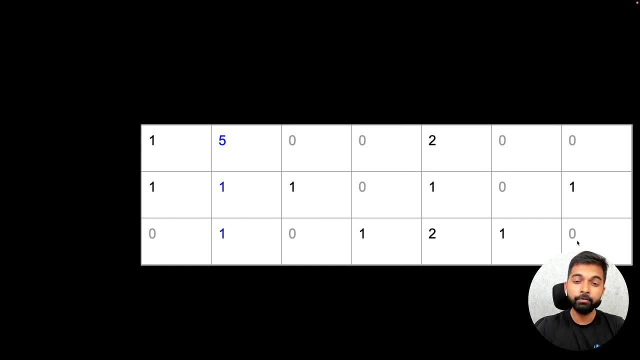 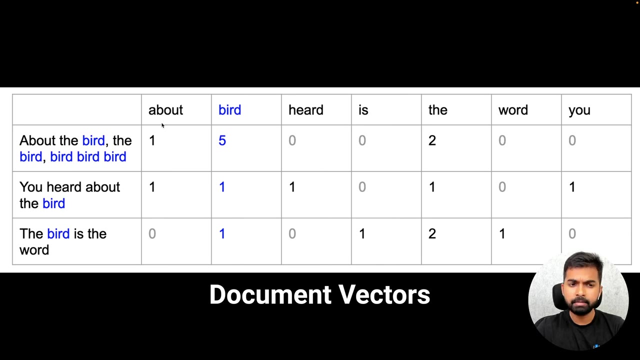 This is the first vector, This is the second vector, This is the third, And if you've done any machine learning, you can now see that this is something that you can feed into a machine learning model. So these are called document vectors, and remember how they are retrieved is by first identifying all the unique words in the dataset and numbering them, and then counting the occurrences of each word in each document to obtain a vector or the document vector. 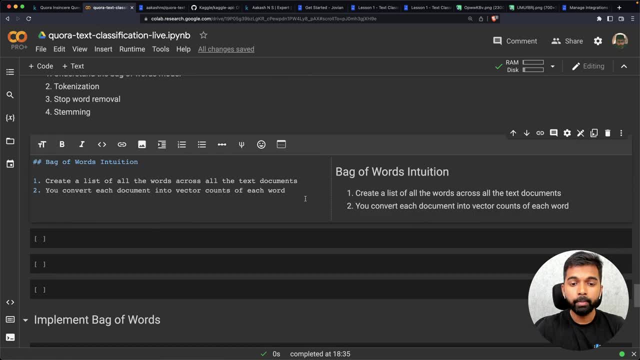 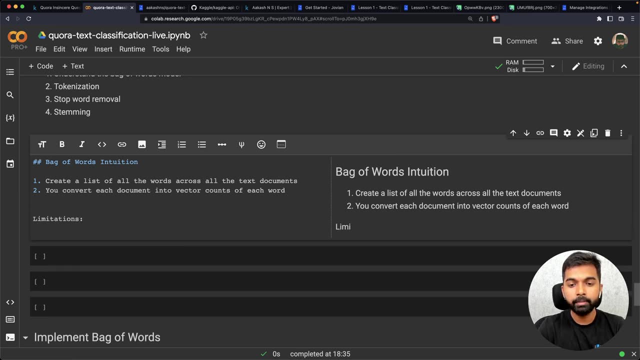 All right. So that is how you build a bag of words model, but there are certain Limitations with directly creating a bag of words model. So here are the limitations. The first is that there may be too many words in the dataset. 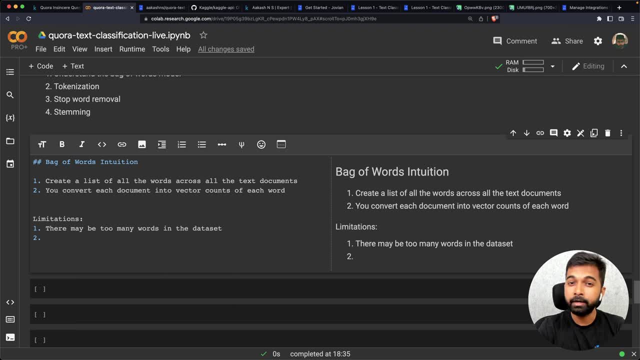 So we have 1.3 million questions in our dataset and it may contain hundreds of thousands of words. So that may make the vectors very large, because each document will be a vector of site, a hundred thousand and that won't even fit in memory. 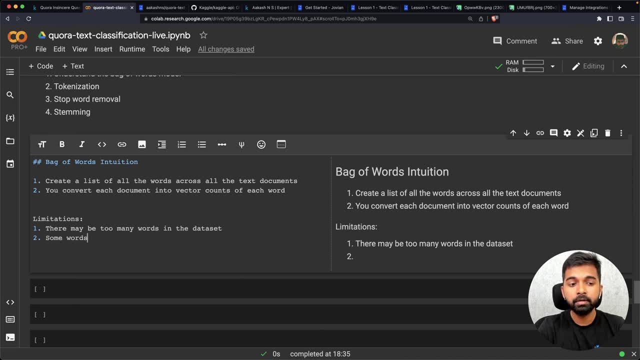 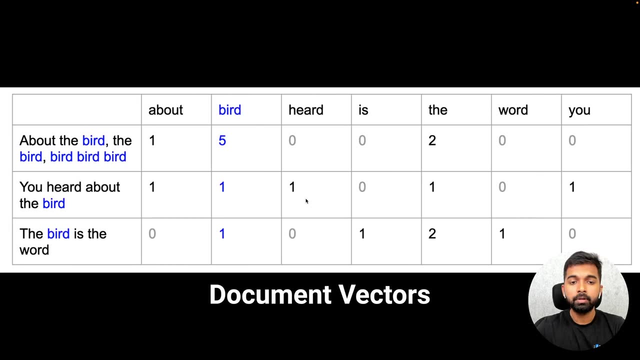 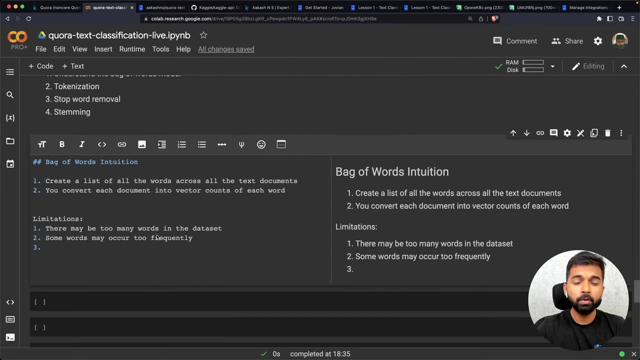 Another limitation is that some words May occur too frequently. So, for example, the word the seems to occur all the time and is also generally having the highest frequency. So we may want to remove these words which occur too frequently. Then some words may occur very rarely or only once, for example some specific technical term that only occurs in one or two. 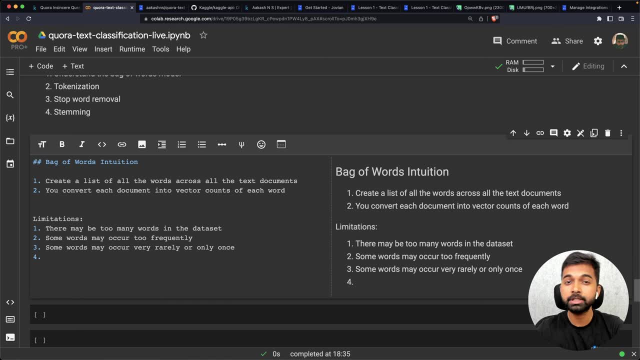 Questions Is very rare, And that may not give us enough information to label a question as sincere or insincere, So we may need to exclude those words as well. Then another thing that we may run into is that a single word may have many forms. 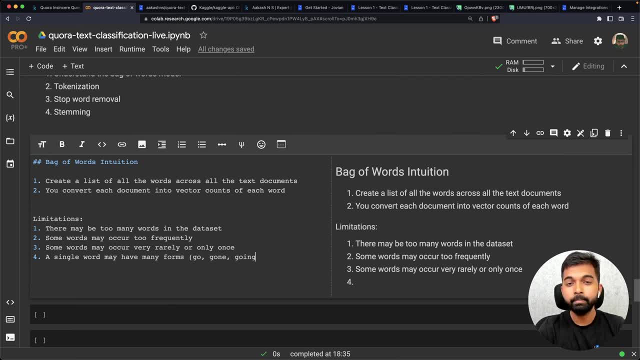 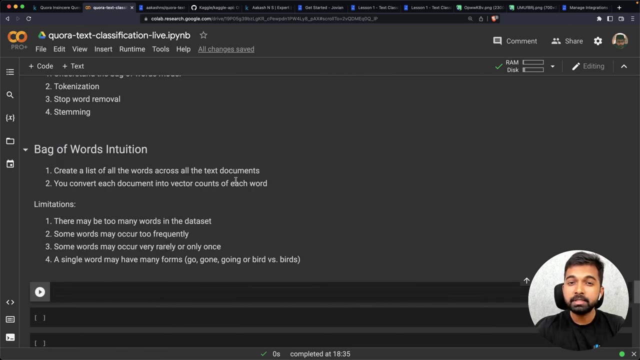 For example, go, gone, going are ultimately all forms of the word go or bird versus birds, Right, So that is something that we may want to count under the same root word, And that is why we perform a several text pre-processing techniques before creating the bag of words model. 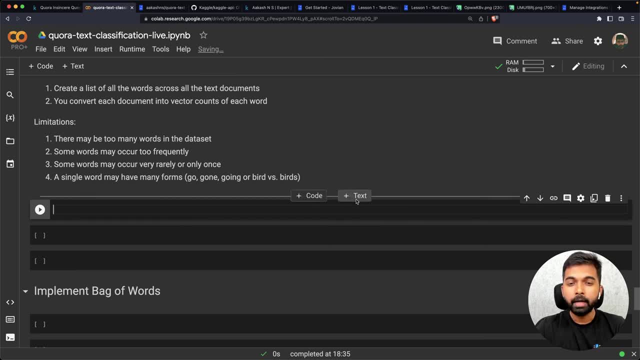 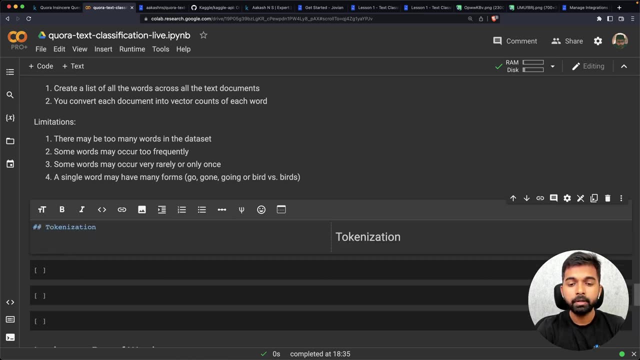 And that's what we are going to look at now, one by one. Now, the first pre-processing technique is something called tokenization. So tokenization is simply the process of splitting a document into words And separators, So it's not just words. 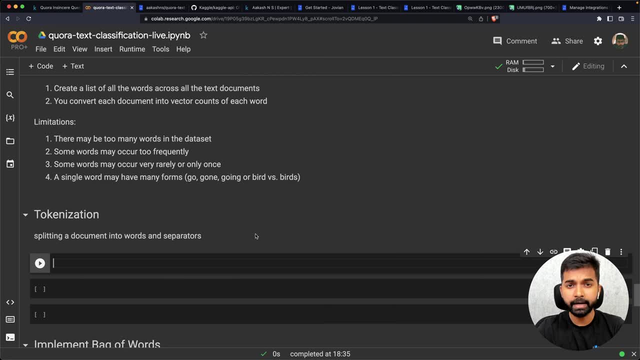 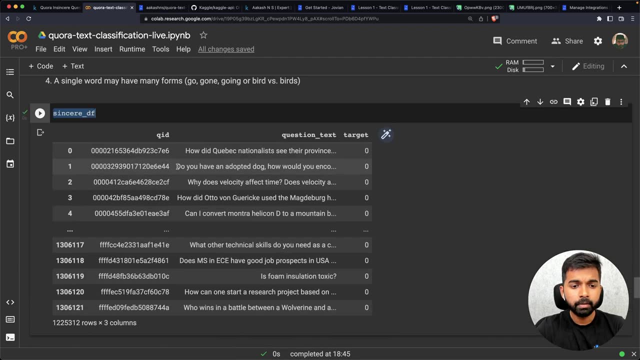 You may want to separate. You may also have to deal with punctuation, things like comma brackets, etc. Let's look at sincere D, F, and from the sincere data frame I'm going to pick a question, This one: do you have an adopted dog? 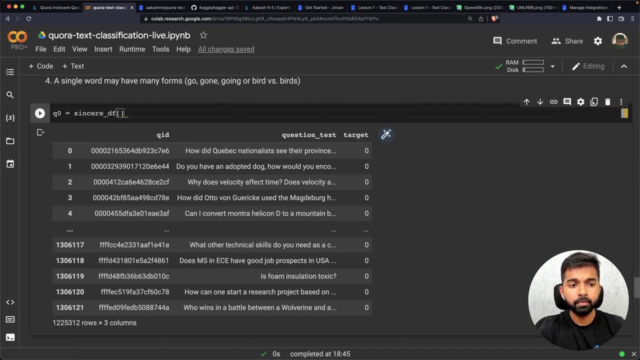 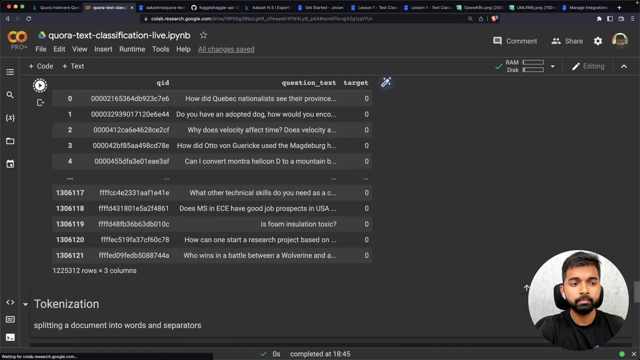 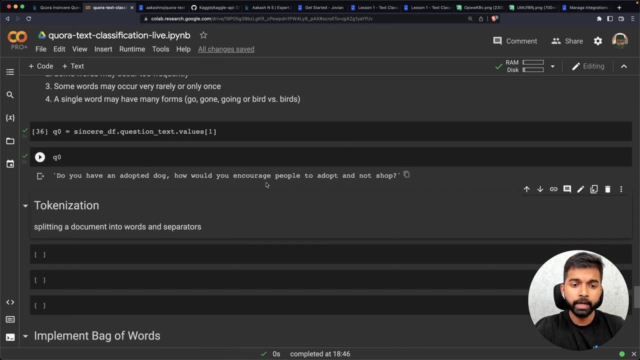 You. zero is sincere. DF one or dot question text: Dot values One. So Q zero is simply the question: Do you have an erupted dog? Would you like to encourage people to adopt and not shop? And let's look at insincerity. 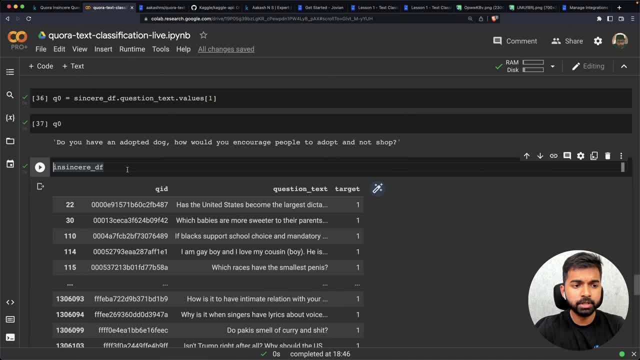 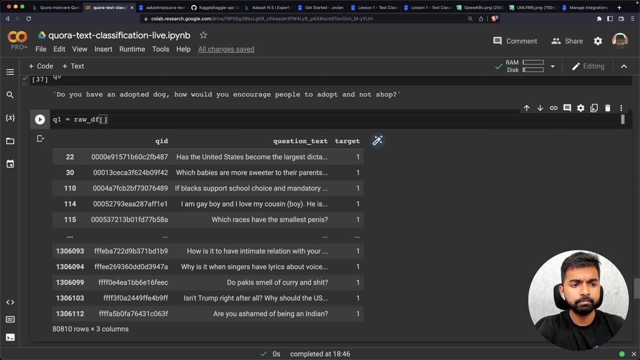 So here's insincere DF, And so I'm going to- I'm just going to pick Q- one equals- let's pick something from Roddy F. So Roddy F or DF dot. Target equals zero dot question text. or target equals one dot question text: one. 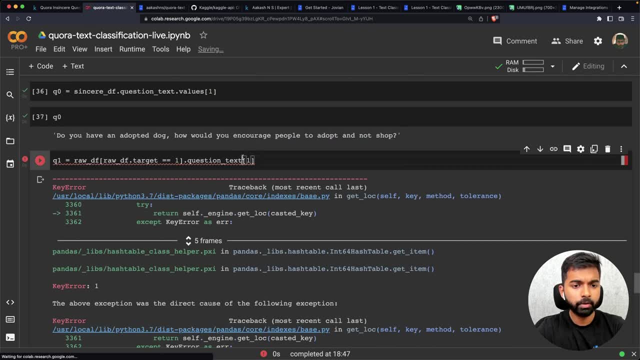 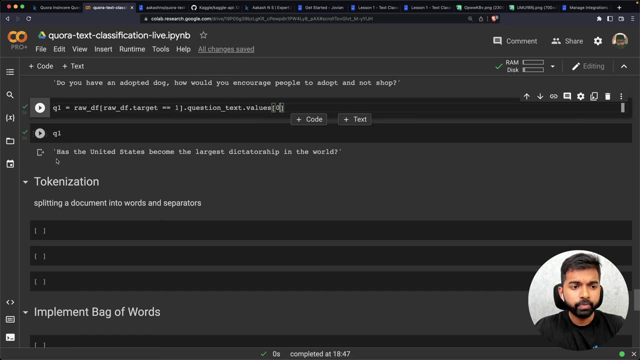 Let's see what that gives us. Okay, Dot values One, Let's try zero. Okay, So let's just go with this one now. Um, so we have one example here. Do you have an adopted dog? How would you like to encourage people to adopt and not shop? 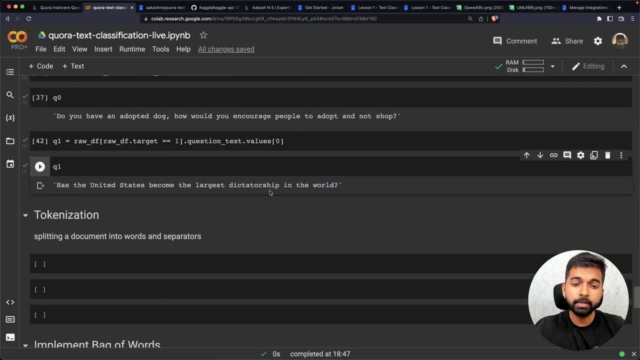 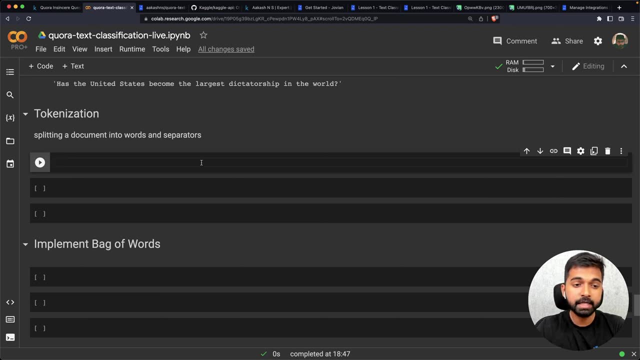 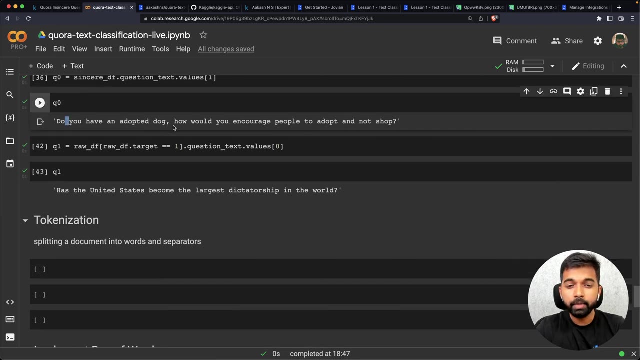 And here is an insincere question: Has the United States become the largest dictator In the world? So the token is: tokenization is simply the process of splitting a documentation, a document into words and separators. So the way we tokenize is either we can just split along the spaces or we can use a tool. 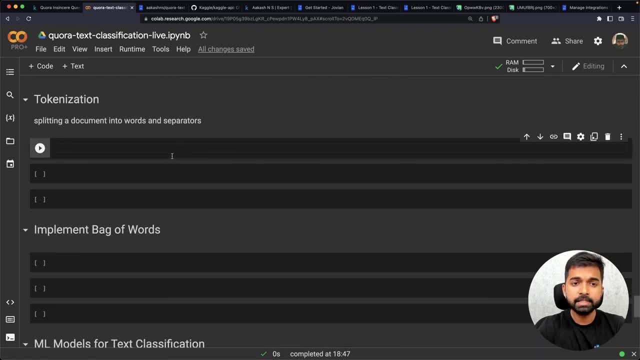 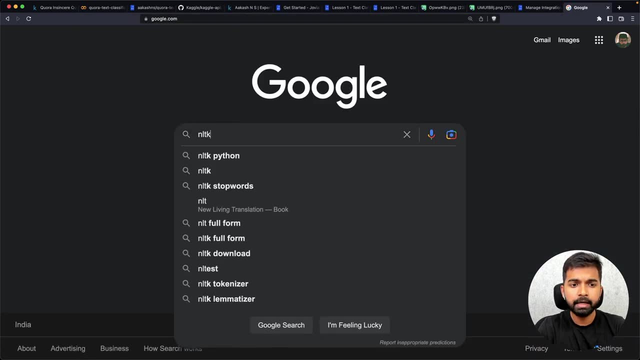 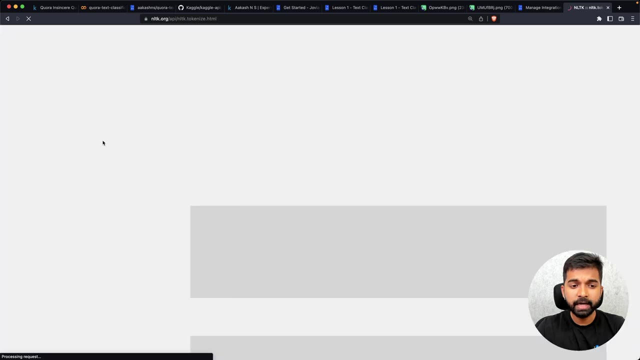 which also detects punctuations properly. So, for example, um, there is this tool called NLTK. So if you just go online and search NLTK, tokenize, So then NLTK has this tokenize package and the way you use it is from the NLTK library. 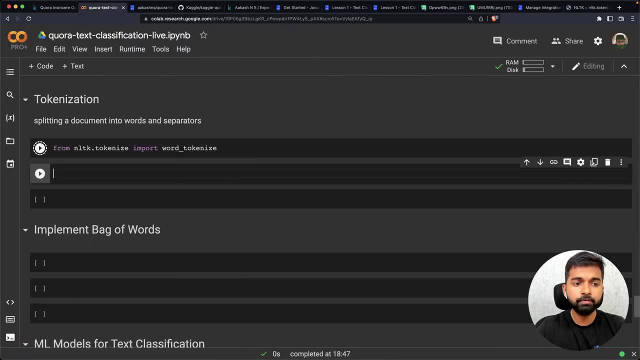 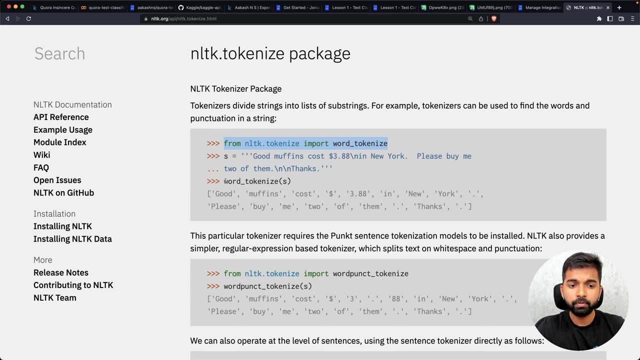 You import word tokenize. I'm just going to go in here and I'm going to say: from NLTKtokenize, import word tokenize. and then you can simply use word tokenize as given here, So word tokenize and give it a string and it's going to tokenize for you. 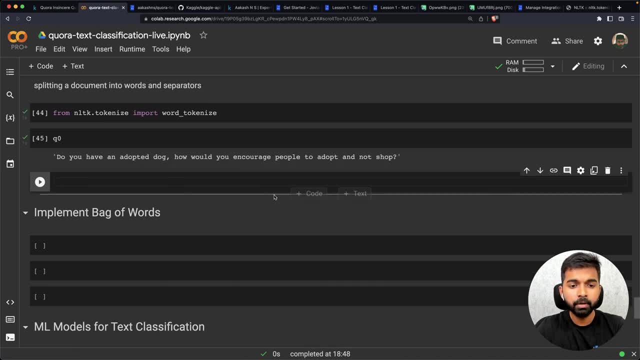 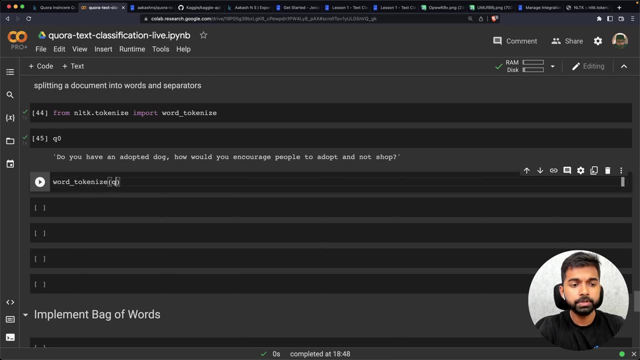 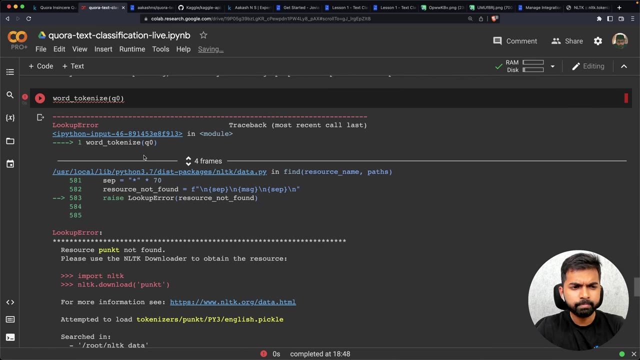 So here's Q0, and let me create a new code cell and let me say word tokenize Q0.. And when we try to tokenize we are going to get an error and let's not panic here. So it says: resource punked: dot not found. 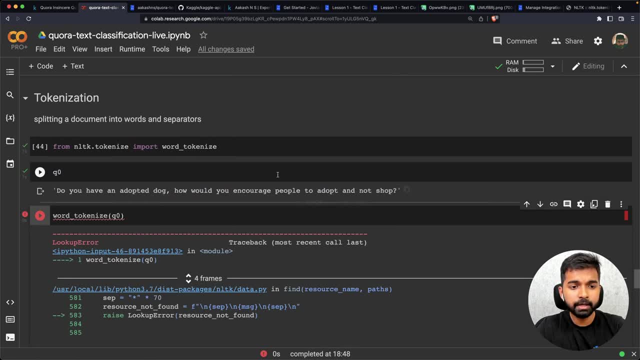 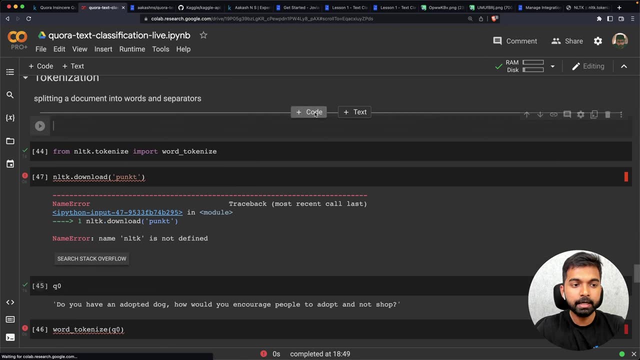 So we may just want to download punked. So let's go up here and let's run that code: NLTK dot. download punked. Okay, Let's also import NLTK. So that requires import NLTK. So this is a common practice. that happens when you write some code and it doesn't run. 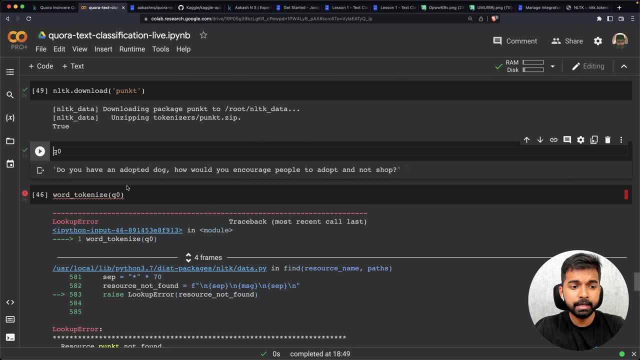 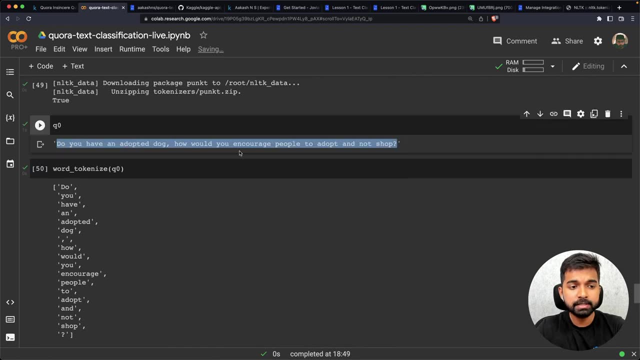 You may have to go out and fix it. Okay, Now It's fixed. So now the data is now the. it's a dictionary of punctuation, Essentially it is. it is downloaded And now you can see we've split this sentence. 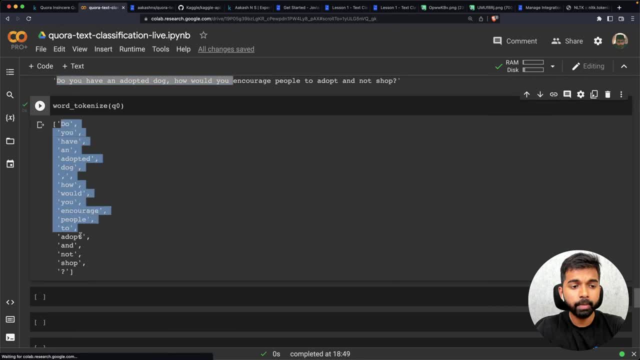 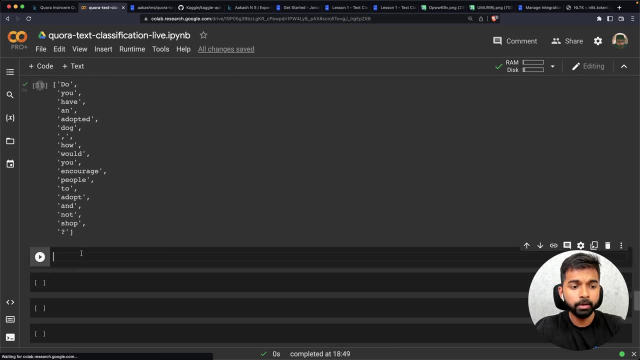 Do you have an adopted dog comma, et cetera, into a bunch of tokens? So here you can see that comma is created as a token, Um, and then question mark becomes a separate token. You can also try it with your own example. 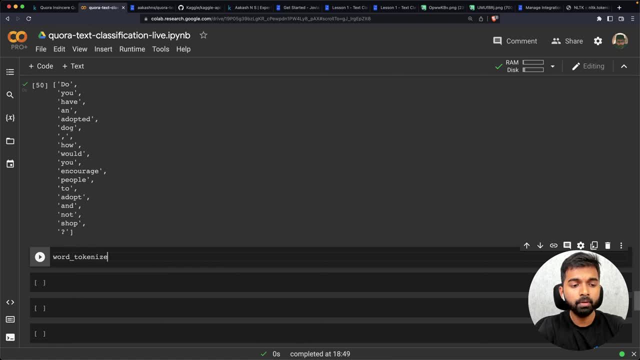 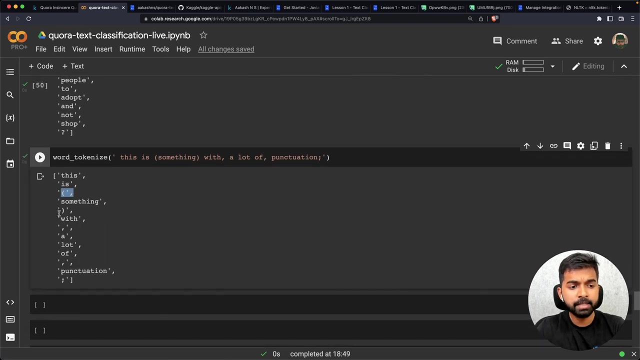 So word tokenize and you can say something like this is Something with a lot of punctuation, right, And you can see what it does with brackets and commas. So you can see your brackets get separated out, commas get separated out, semi-colons get separated out. 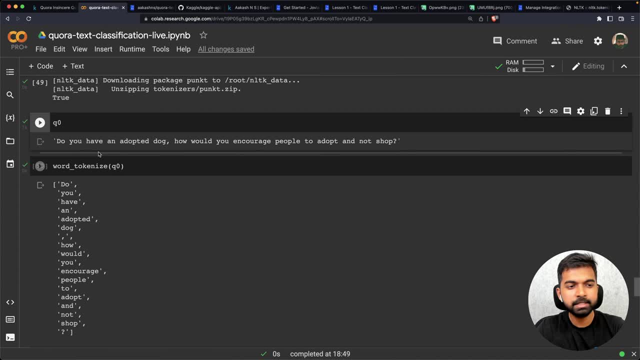 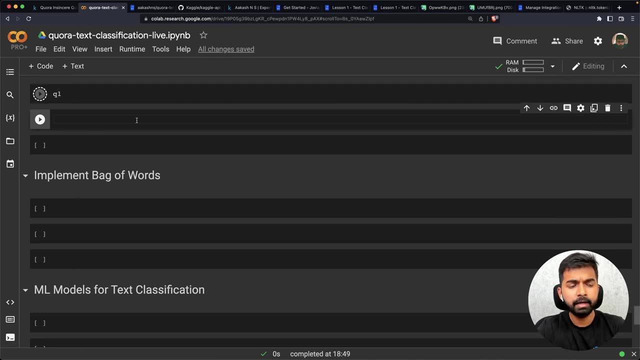 So that's where it's smart, And so in that fashion, you can also try to write your own tokenizer, but you should probably just use the NLTK tokenizer. Okay, Let's also maybe tokenize Q1.. Let's see if there are any interesting tokenization. 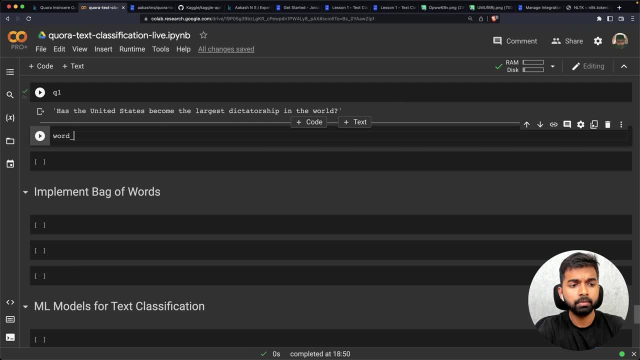 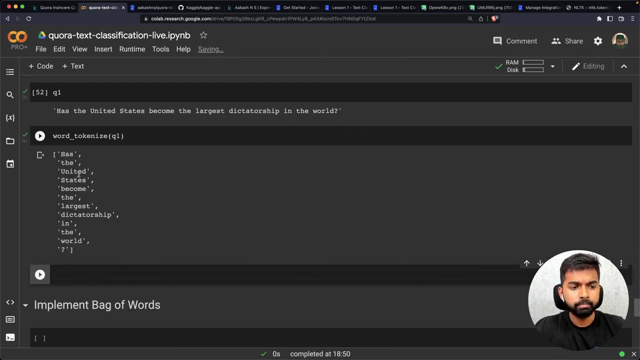 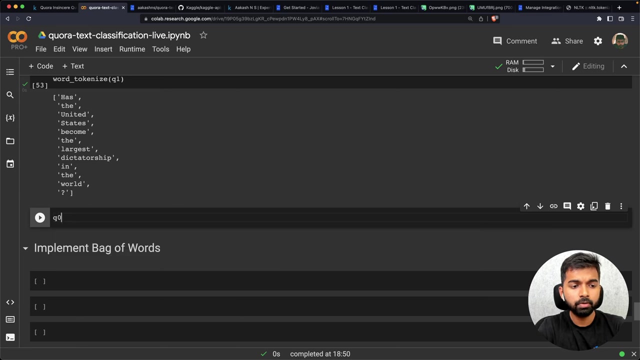 Okay, Is there? Yep? So here it's fairly straightforward. This is a very simple, this is a very simple question and it is tokenized properly. Okay, So I'm just going to store these results. So I'm going to say Q, zero underscore T, okay, 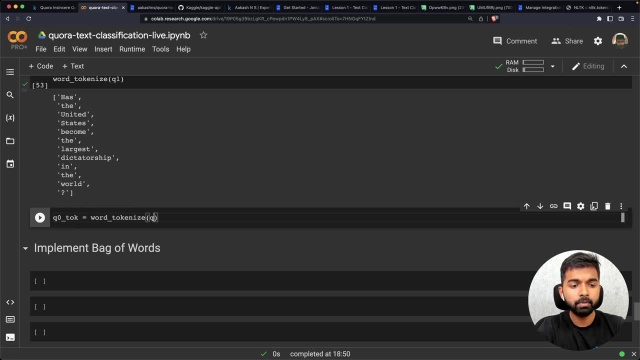 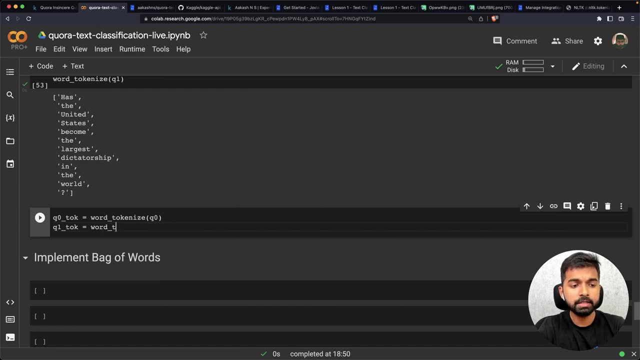 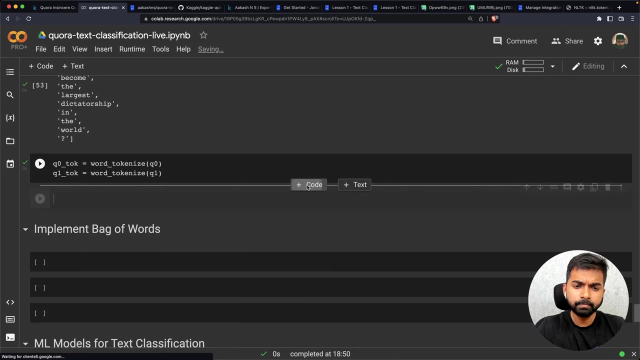 Equals word tokenize Q zero And Q one. underscore T: okay, Equals word tokenize Q one. And then we're going to use it in the next steps. Now I encourage you to experiment this with this a little bit. try some more tokenizations. 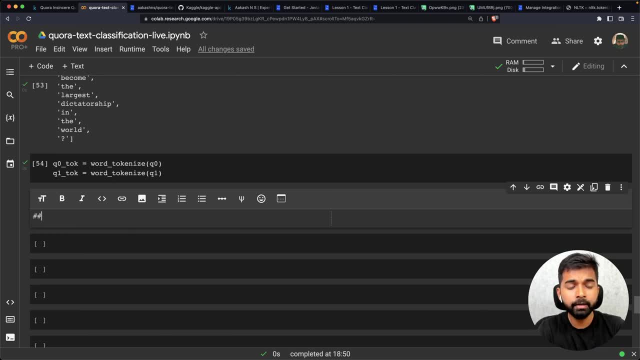 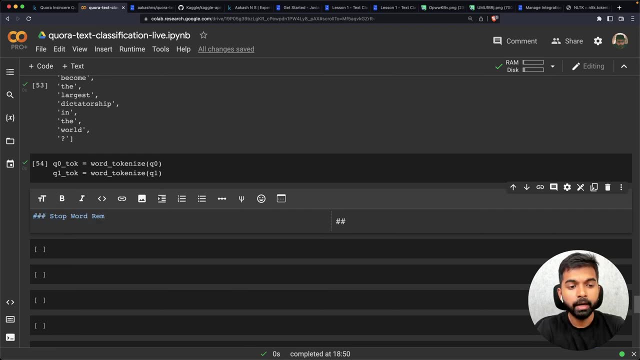 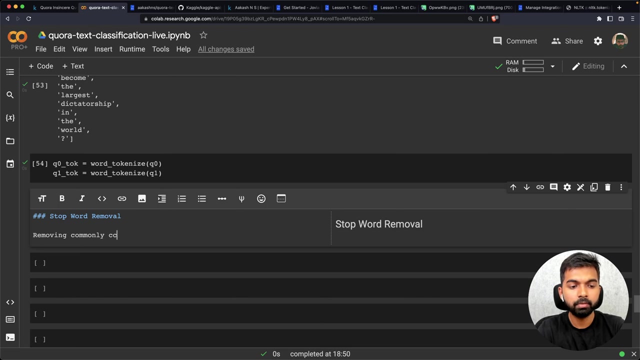 try picking up some different questions which are a little more complicated, but we are going to now move on to the next step, which is stop word removal. And what is stop word removal? It is simply The process of removing commonly occurring words, right? 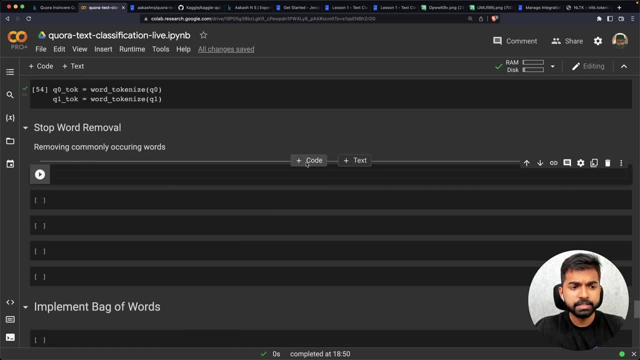 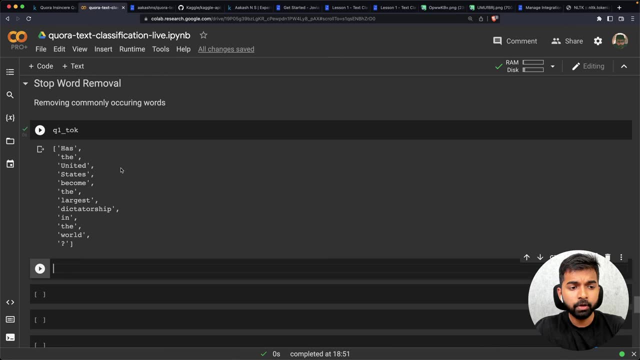 That's all we're going to do here. So let's see, let's try Q, one underscore E, okay, So here you have all these questions, Like you have all these words, like the in, et cetera, that offer that occurred too many times. 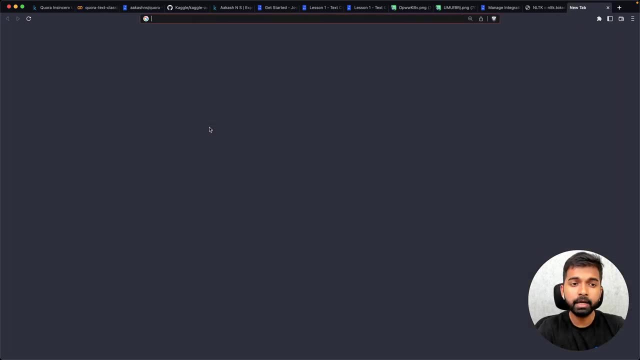 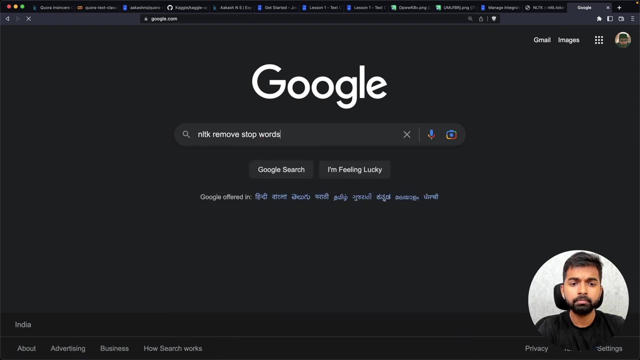 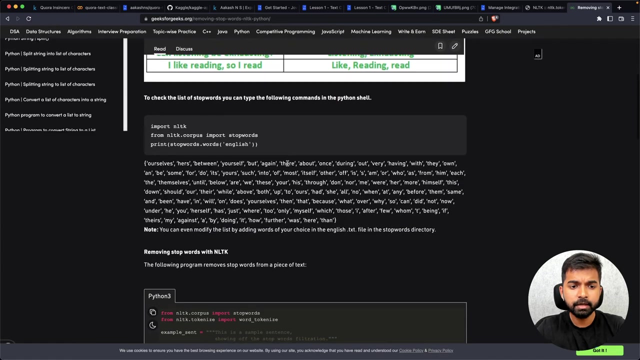 And the way you can remove this is, once again, using the NLTK library. So I'm going to go online And I'm going to search NLTK- remove stop words- And once again there seems to be some documentation available. Let's go in here and let's see how this is done. 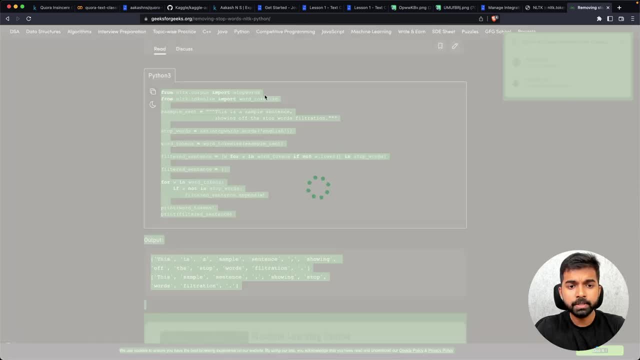 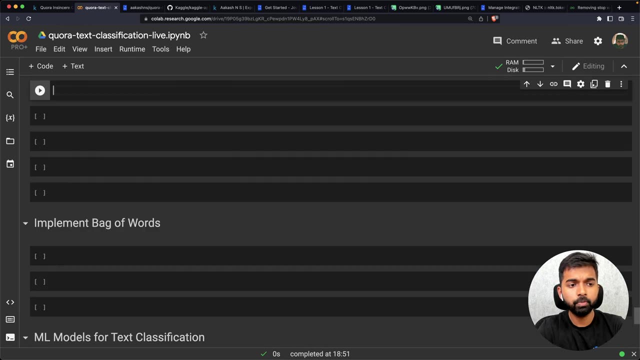 So here is how it's done. So you say from NLTK dot corpus: improve import, stop words. So I'm going to come back here and I'm going to say: from NLTK dot corp, oops, I'm going to say from NLTK dot corpus. 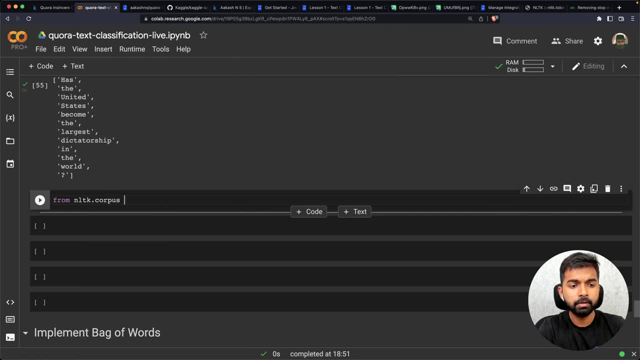 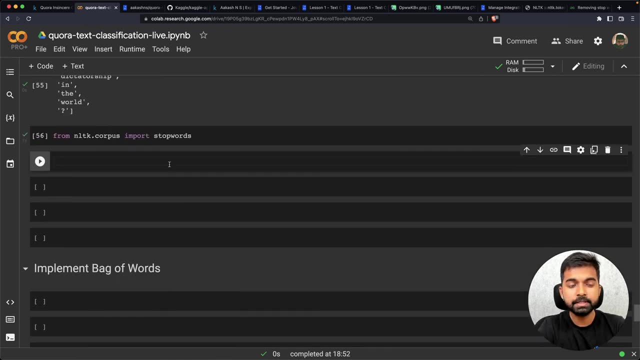 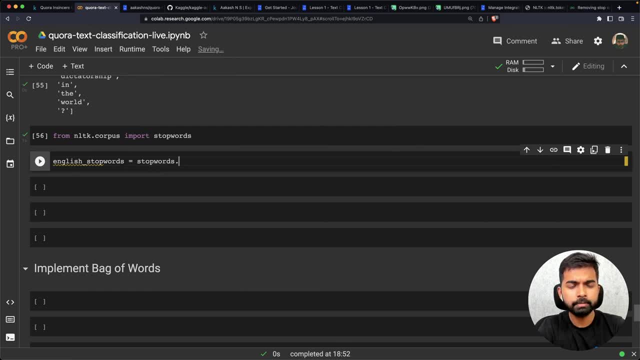 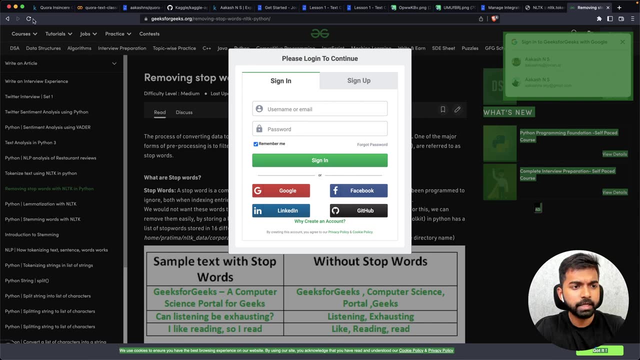 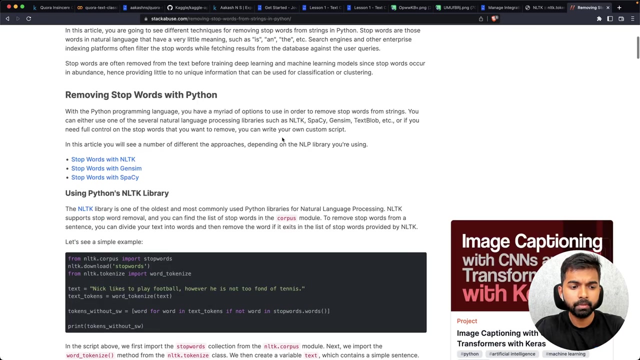 English stop words equals stop words, dot I. let's see here how it's done. Okay, Looks like this requires a login, So I'm going to search somewhere else. Yeah, now we want to say something like stop words, dot words. 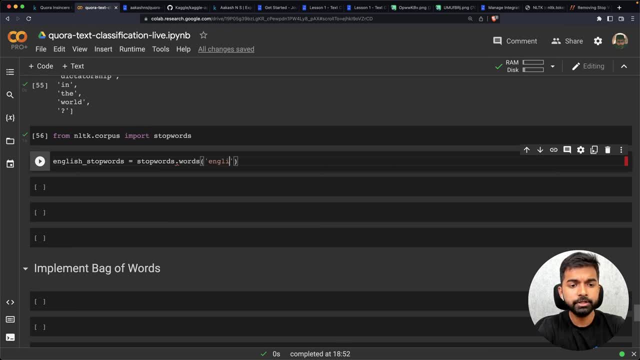 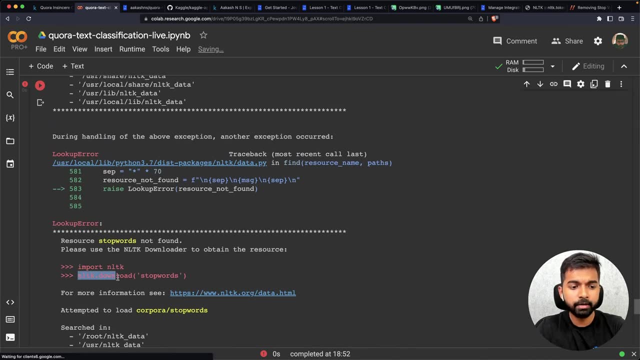 So I'm going to say stop words, dot words, English. So now this is going to give me the full list of English stop words. Okay, Once again there seems to be an error, So it looks like we may need to download a set of stop words as well. 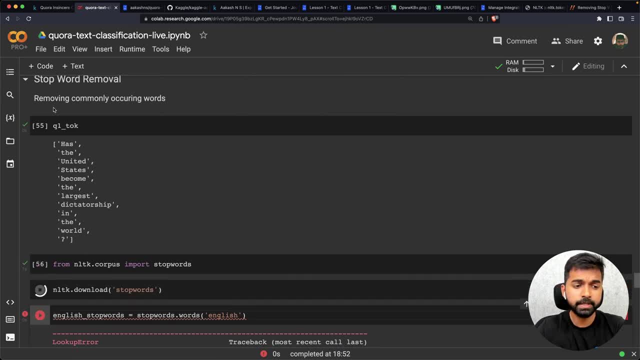 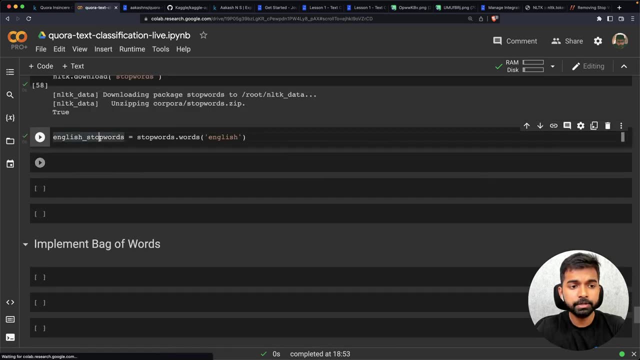 Again, something that will naturally happen when you write the code, and you can just fix it by writing this download statement. So now the stop word database has been downloaded, and now we are looked at the English stop words, And now we have a list of the stop words in the English language. 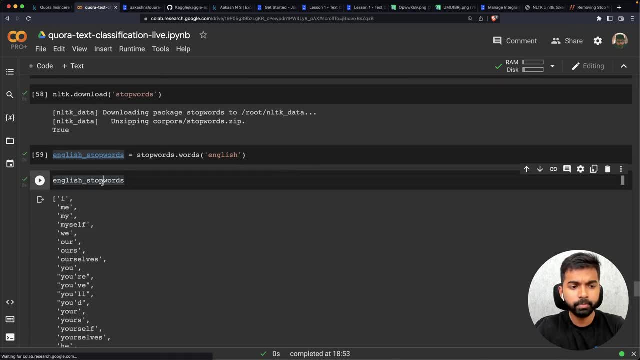 So here is a full list of stop words in the English language. I'll show you a quick trick on how to print it nicely. You can just say comma as a string, dot, join and give it a list of words, and that's going to print it a slightly nicer. 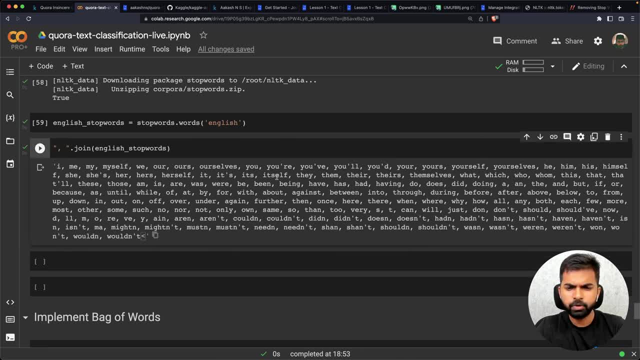 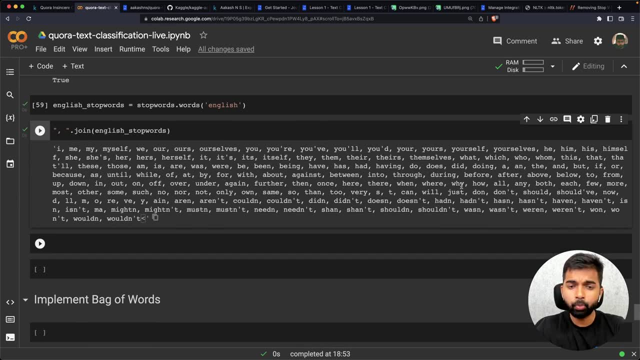 So here is the full list of words. I, me, myself. you can see Hey and the, the articles pronouns. a lot of those things are present here. Now, one thing you'll notice is words like not, couldn't, didn't, et cetera also show up here. 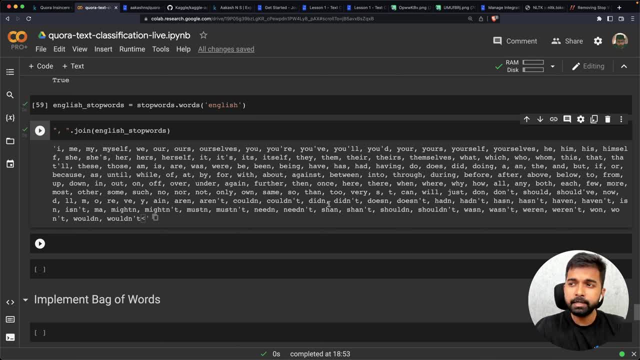 So for the purpose of text classification, sincere and insincere questions- this may not be something we need to worry about. but for the purpose of sentiment analysis, for example, you may want to retain some of these top words like not, et cetera. 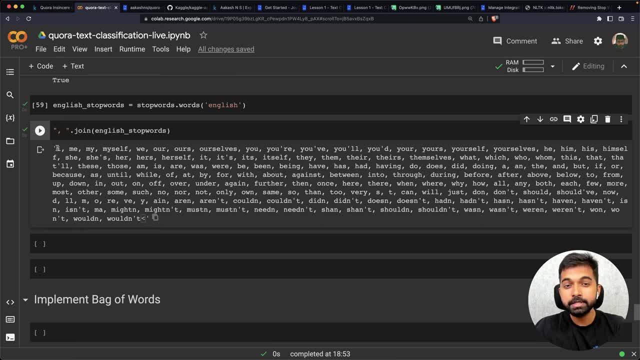 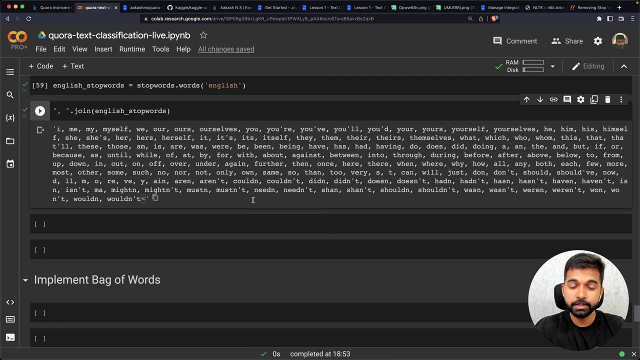 So I would suggest that you look at the stop word list carefully and decide if you want to use all the stop words And if you don't want to use all the stop words, then only pick the words that you actually do want to exclude. 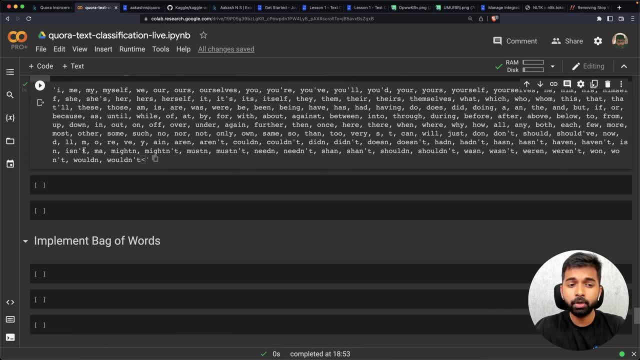 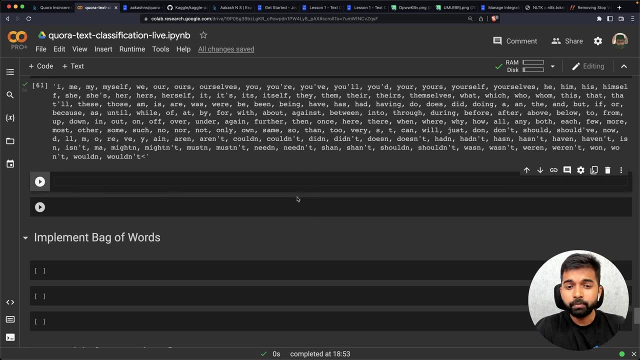 Okay, This is a common error that you can make just going with the given stop word list. So think carefully before using stop words. All right, So now that we have a list of stop words, how do we remove these top words? Well, we can define a simple function for it. 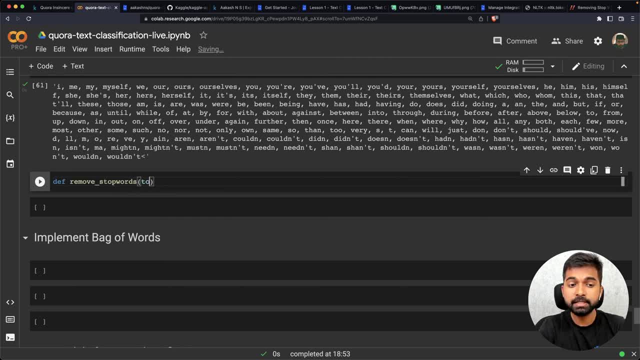 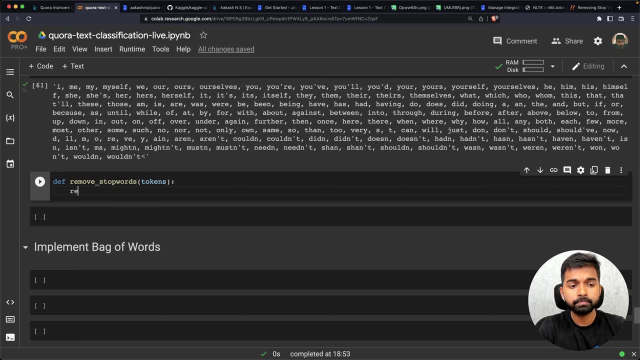 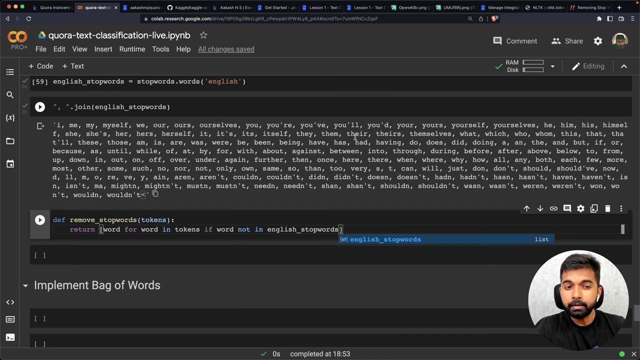 The remove stop words, which takes some text, or which takes a list of tokens. now that we've already tokenized our Questions and we can simply return word or word in tokens If word not in English, stop words, All right. Now one small warning here. look at the stop words here. 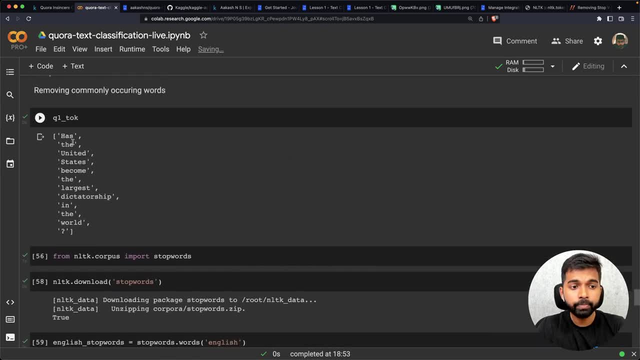 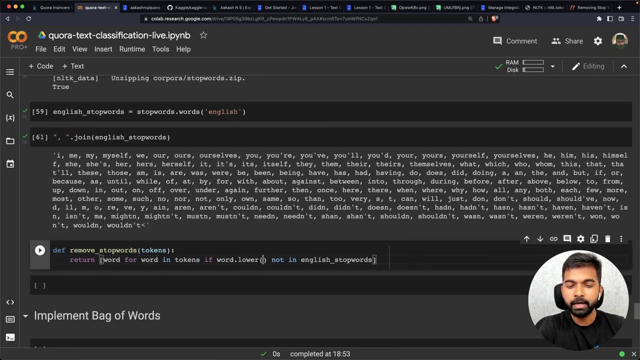 They're all. they're all lowercase. but in our data we may not have all lowercase, So you may want to also add a dot Lowercase. So you may want to also add a dot Lowercase. And that's where it helps to define functions, so that all these small minor things that we 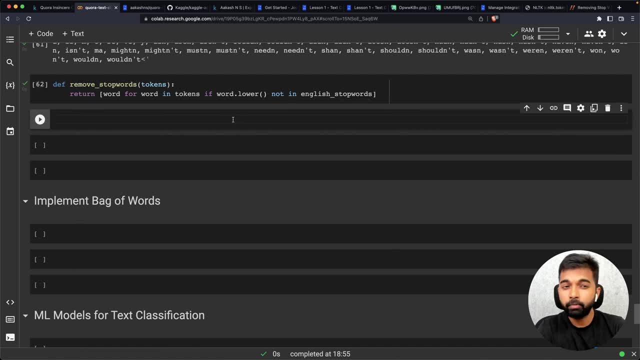 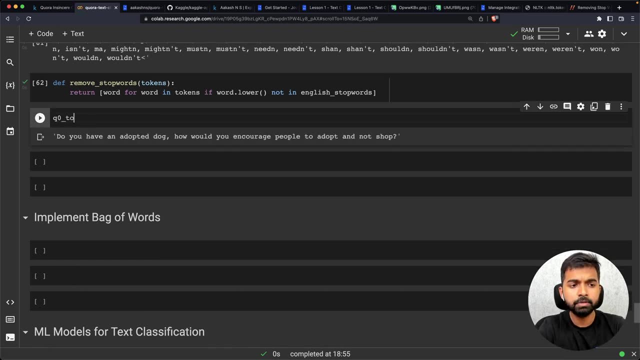 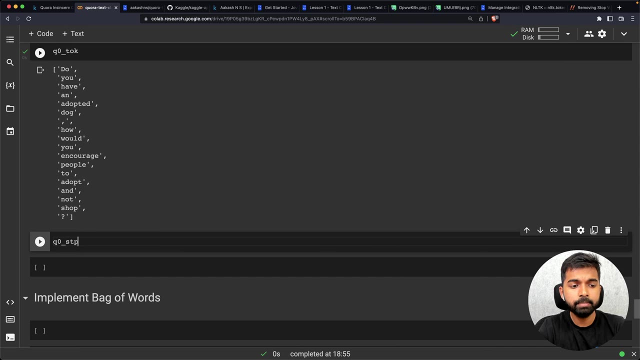 have do not affect us in any way when we are working through the code. All right, So now let's look at Q0 once again. So this is Q0 and this is Q0 tokenized, And let's try to create Q0 underscore STP after removing stop words. 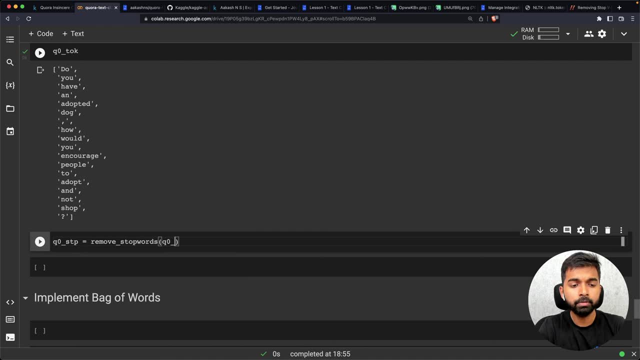 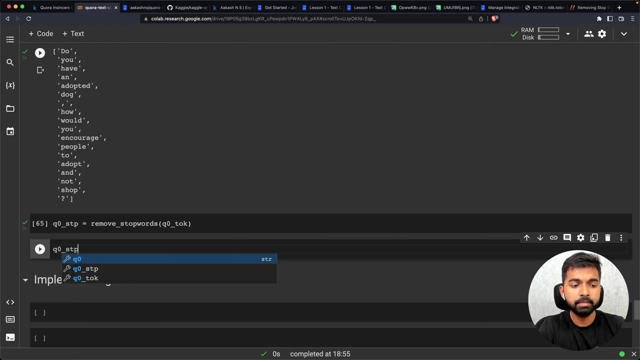 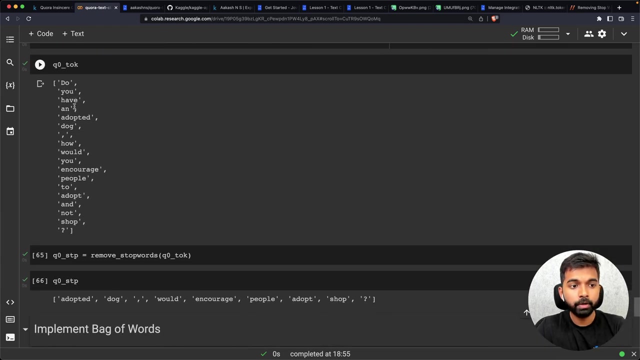 So remove stop words Q0.. Underscore T: okay, And let's check Q0. underscore STP: All right, Looks much smaller. So it looks like the word do the word, you the word have, and all of that is gone. 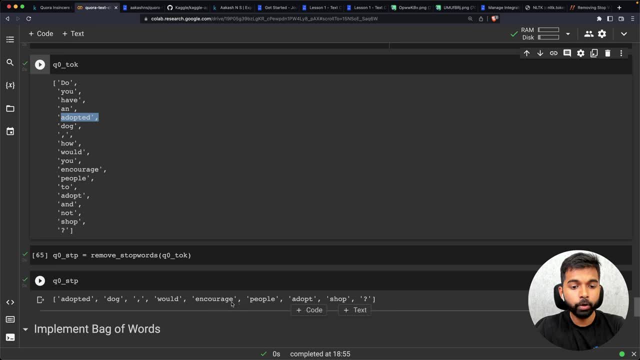 We just have adopted dog comma. I was gone Would encourage people adopt dog shop. So obviously with the sentence is starting to lose meaning already. but we are creating a bag of words. We are not really concerned with order. That is one of the limitations. 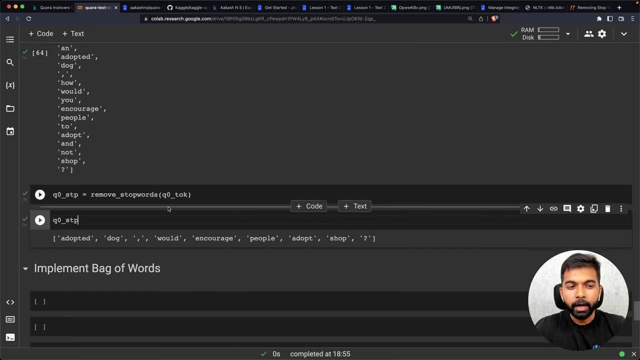 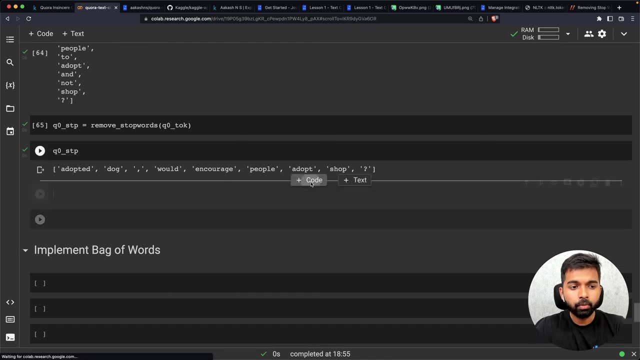 So bag of words, but that's how it is designed So, and we don't want to include the words that are very common, So let's do this again with Q1 as well. So Q1 underscore STP would be: remove, stop words. 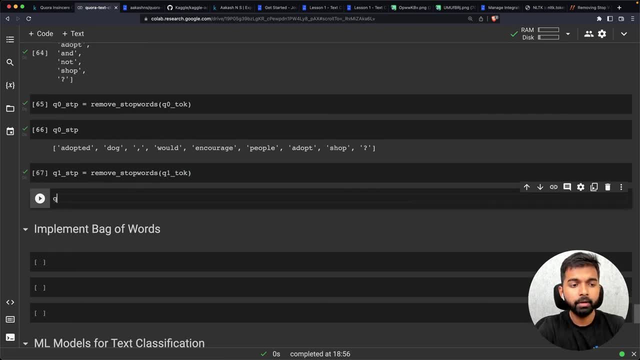 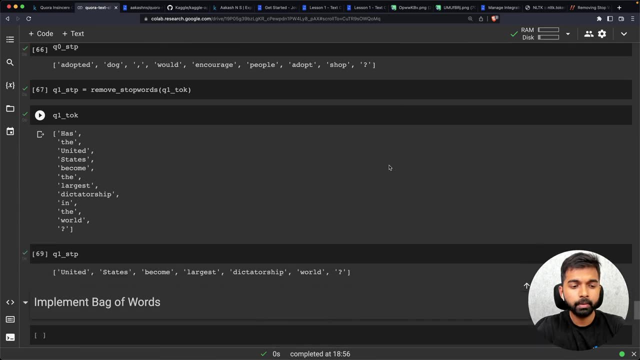 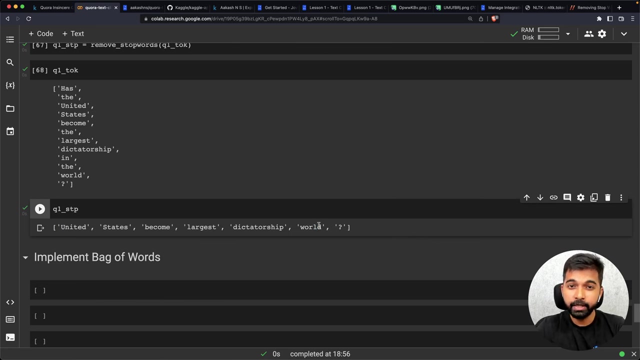 Q1 underscore T- okay, And let's see: Q1 underscore T- okay, And Q1 underscores STP, Yup. So once again you can see that a bunch of the words have gone away. So this is already going to greatly reduce our vocabulary size, because the most common words will be gone. 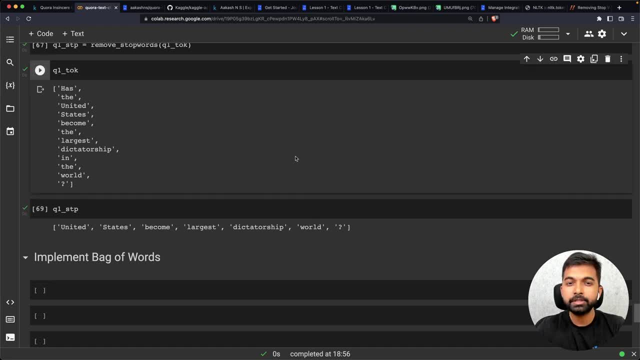 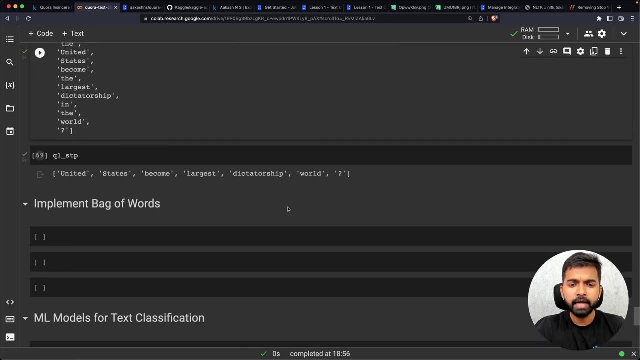 And this is also going to remove the common words which may just have an unfair effect on the machine learning model and may occur in pretty much every question. All right, So that is something that we've done: stop word removal And again, I encourage you to experiment with different stop word lists. 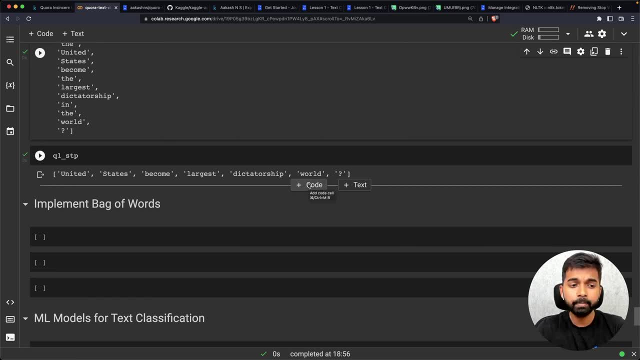 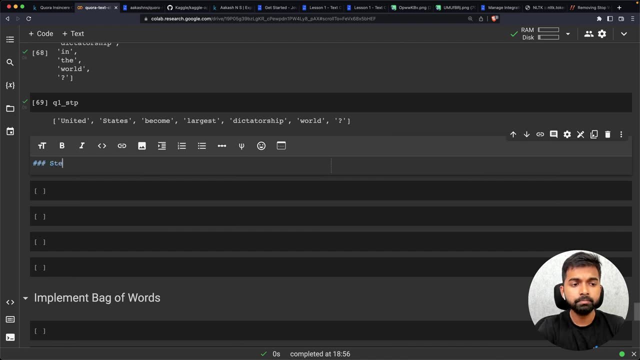 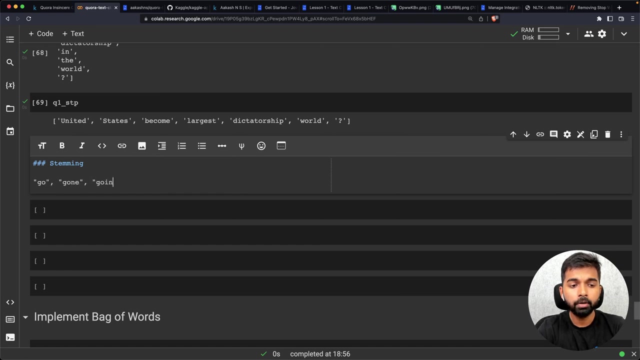 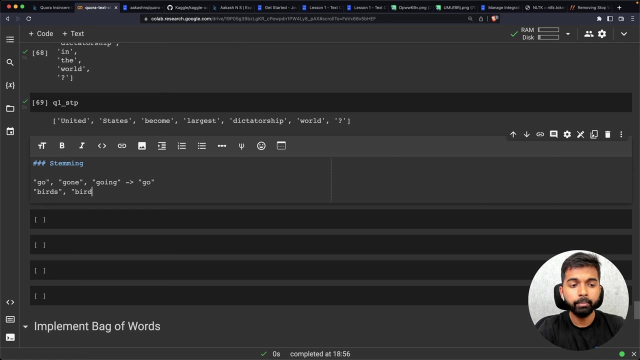 Don't stop here. Just create more code cells and experiment with it. Okay, Next step is something called stemming. So let's talk about stemming Now. stemming is simply the process of turning things like go, gone, going into the root word go. or maybe taking birds and bird and turning them into bird. 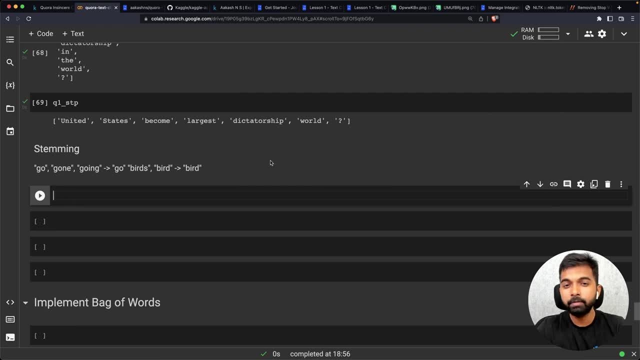 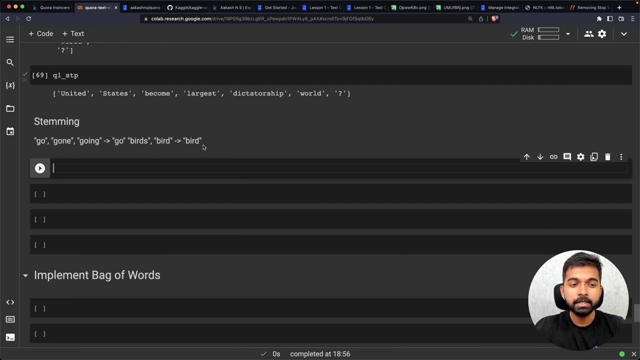 Why do we do this? Because, in terms of counting frequencies, in terms of the meaning, both of these things will have the exact same Effect, essentially, when we're dealing with bag of words. so we may want to reduce the vocabulary, vocabulary size, and increase the frequency of the root word itself. 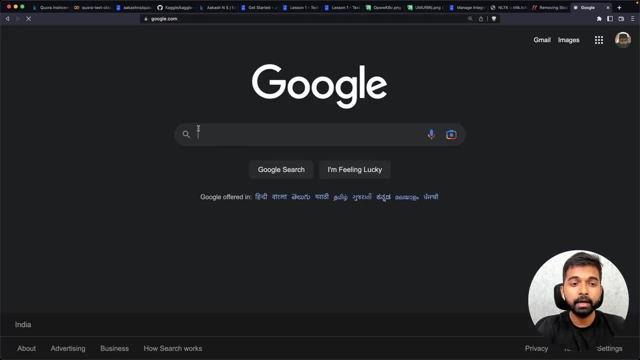 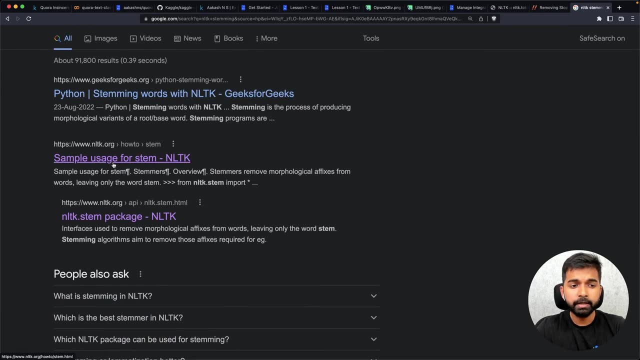 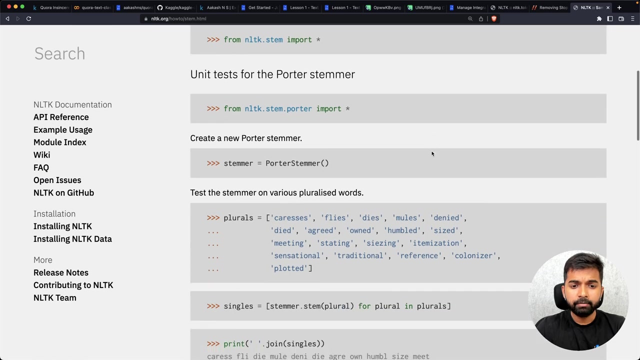 And how do we do that? Once again, we go online and we can use NLTK to do it. So NLTK stemming and when you search you find the NLTK library and here you can see, in NLTK we have several stemmers. 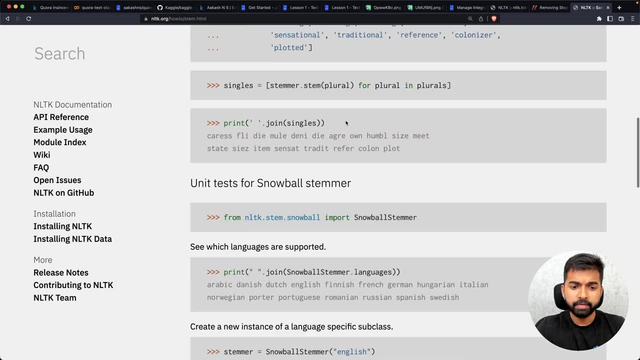 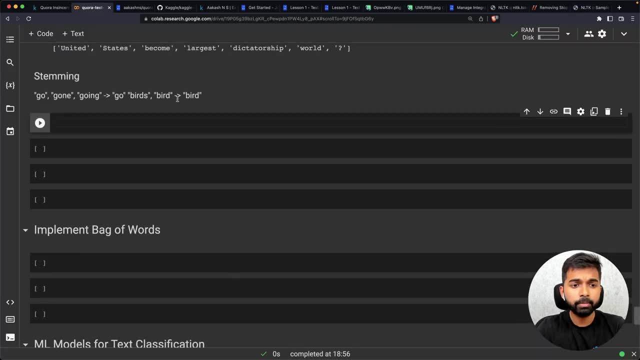 So we have something called a Porter stemmer. We have something called a snowball stemmer. So, just for fun, let me try snowball stemmer. You can try the Porter stemmer as well. I'm going to import the snowball stemmer and then I'm going to create a stemmer. 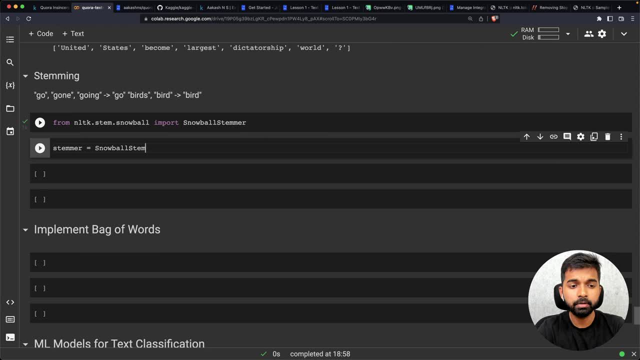 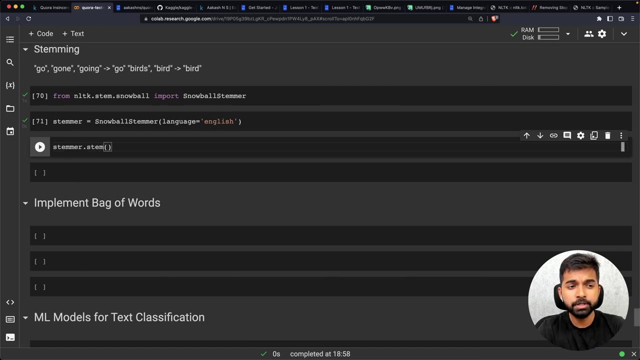 So stemmer equals snowball stemmer, and I'm going to provide a language- English Again. you can study the documentation to see how to use it, or maybe just look at a tutorial, and then you can call stemmerstemmer And give it a word. 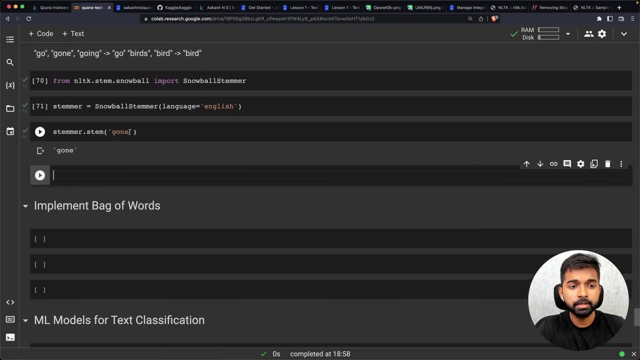 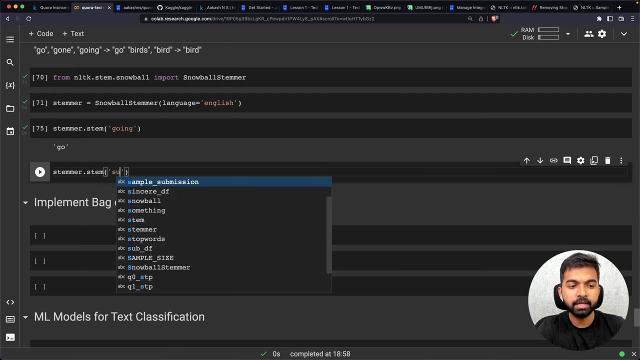 For example: stemmerstem gone, simply returns go. stemmerstem going, also returns go. stemmerstem go, just returns go. So experiment with it, see how stemming works. Let's try stemmerstem, maybe, something like supposedly. 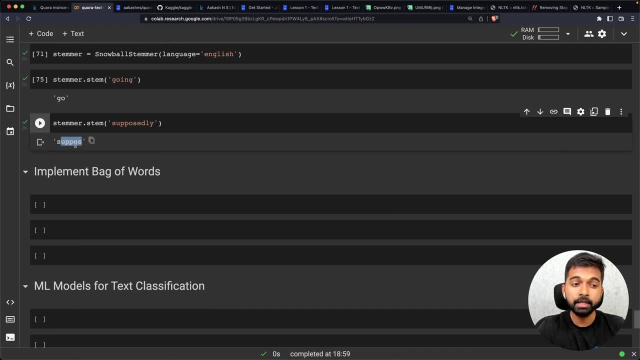 Okay, That's just written: suppose, So it's not always a proper word. Keep that in mind, because you may have something like supposing, suppose Or supposed or something else which may not have this E. So sometimes, after stemming, the words that you get back may not be sensible because they will just be a root of a potential family of words. 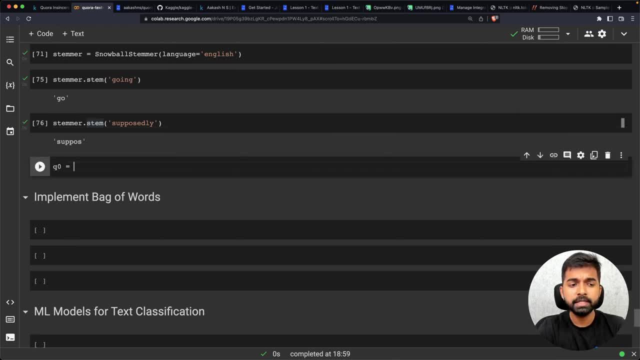 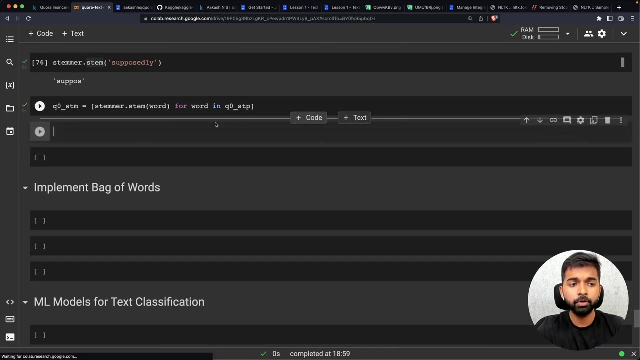 Now how do we create a stemmed version, Let's say, of Q0,? we say Q0 underscore STM equals stemmerstem, word for word in Q0 underscore STP. So since we've already removed stop words, I'm just going to build on that. 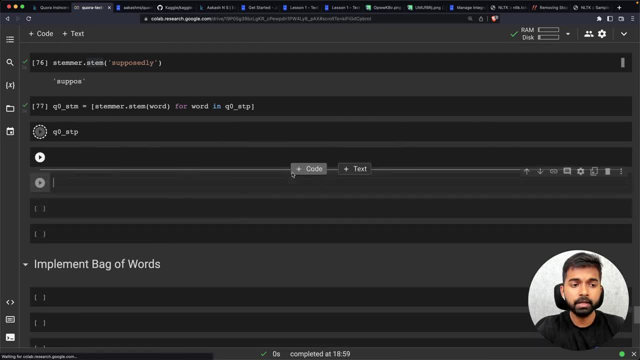 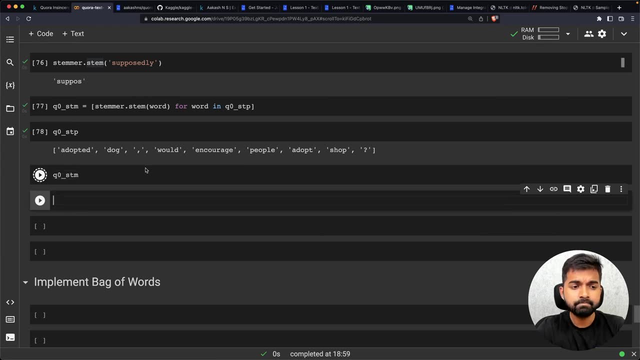 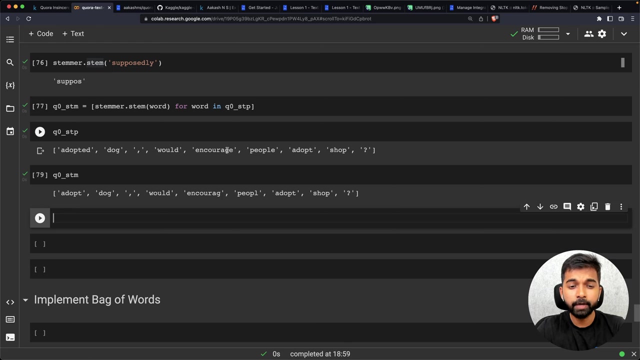 So Q0 underscore STP is this and Q0 underscore STM is smaller. So you can see here, instead of adopted we have adopt, And then instead of encourage, we have encourage without an E, because you can have encouraging. because of certain rules the E here has also been wiped out. 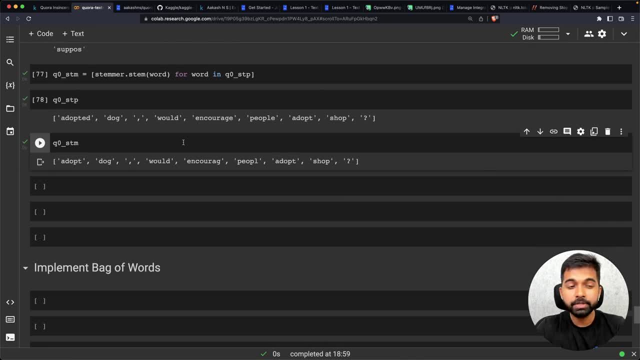 Sometimes it makes sense, Sometimes it doesn't, But the idea is all: Yeah, All of these words get reduced to their root. Let's try that with Q1.. Q1, underscore STM, equals stemmerstem, word for word in Q1, underscore STM. 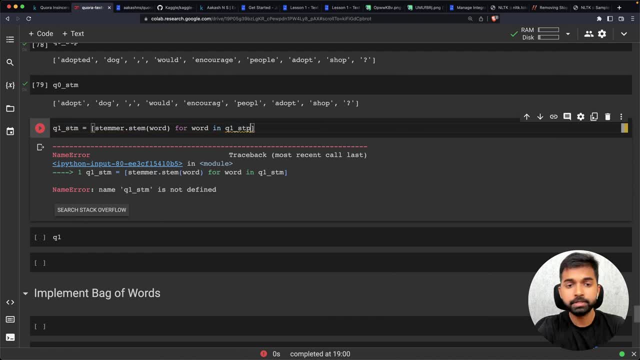 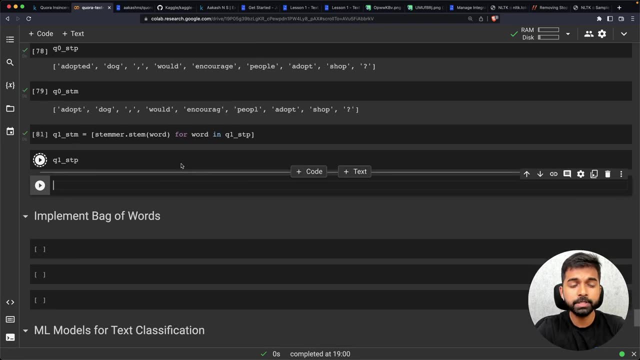 And let's check. Okay, Q1 underscore STP, which was with the stop words removed, And let's check that out as well. So here is Q1 underscore STP with just stop words removed And here is Q1 underscore STM. 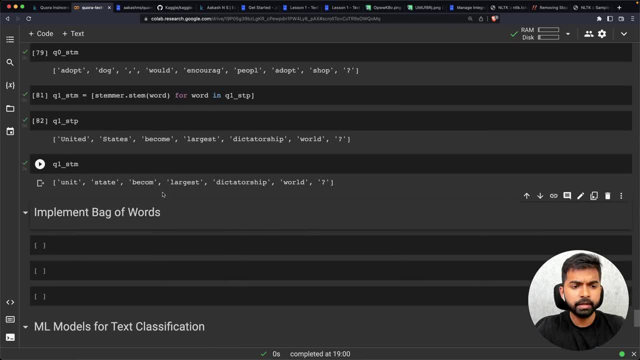 And you can see here that in this case there's not much of a change. Well, United has been changed to unit, something that we may not want, necessarily, but I guess it's okay. States has become, state become has become, just become without an E, and dictatorship has not been reduced. 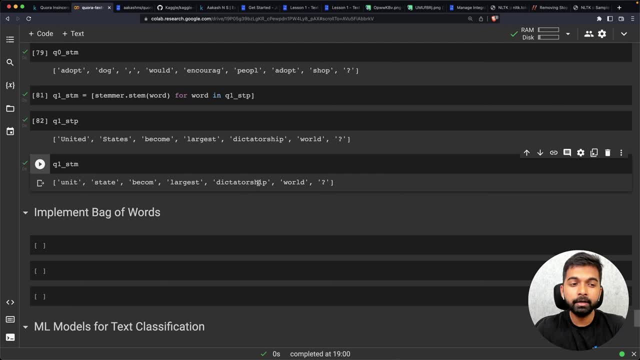 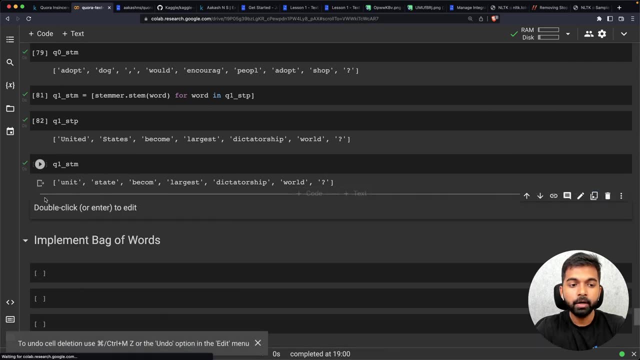 So stemming is done using an algorithm implemented internally, And that's why you may get these edge cases, these funny cases where it may do things that you may not want it to do. Another technique that you should you should check out is lemmatization. 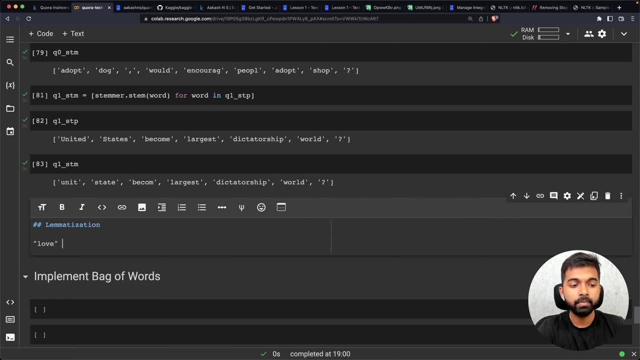 Now, in lemmatization, what is done is, let's say the word love, and you have another word, loving, and you have another word lovable. So the stemming would reduce them all to L O V. lemmatization, on the other hand, would reduce it to a word that actually makes sense. 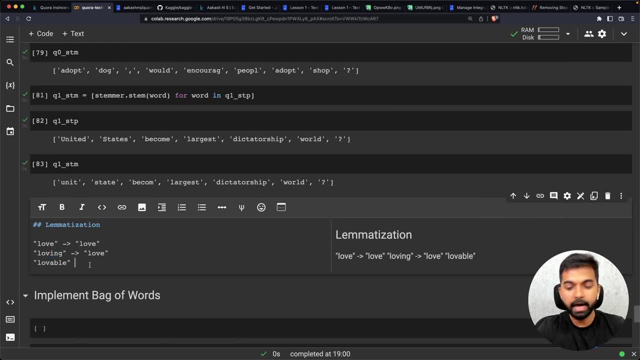 So in this case, lemmatization would remove ING and lemmatization would add the E. and how would it know that it needs To add the E? because lemmatization is going to look at a dictionary. It's going to use a dictionary internally to look up the root form of each of these words. 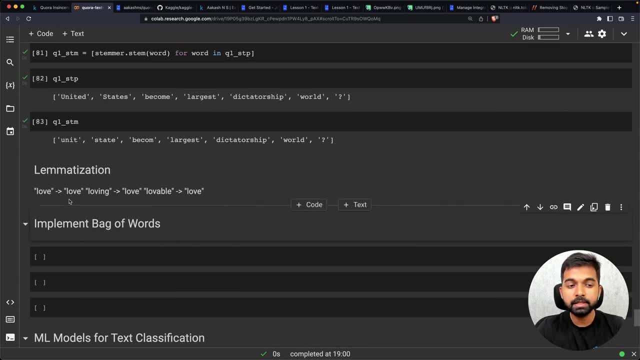 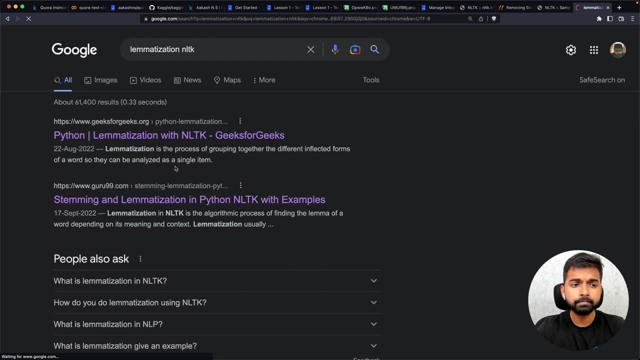 So if you want more human friendly forms of the root words, then you can use lemmatization. And again, you just search lemmatization and LTK and you're probably going to find some tutorial on it. Let's see here. 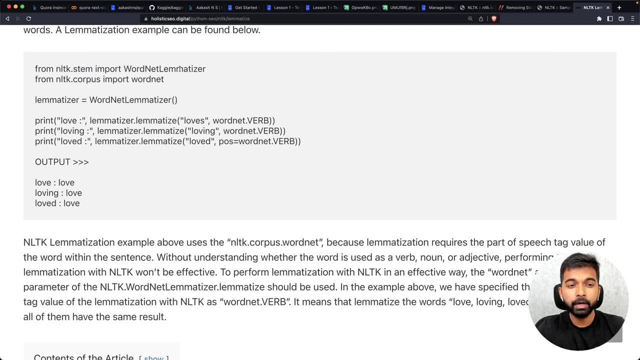 So here is how you use lemmatization in LTK: You Import the word net lemmatizer and then you import this corpus called word net and then you create a lemmatizer and then you call lemmatizer. 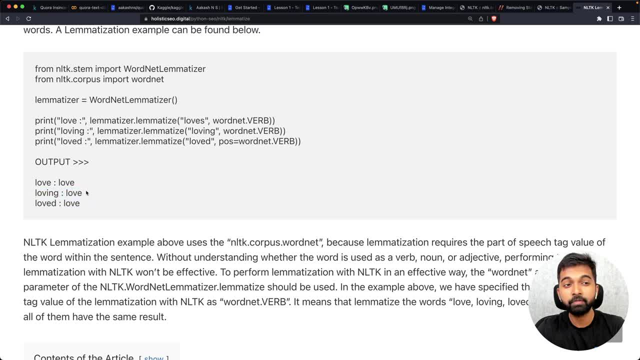 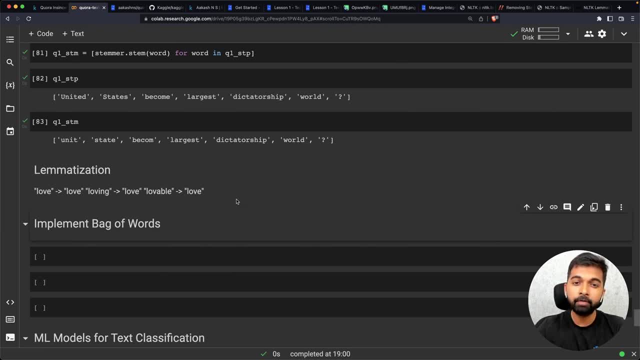 dot, lemmatize, and that's going to give you the root form which is picked from a dictionary. Now I'm leaving this as an exercise for you, And lemmatization is generally not used while building bag of words because it requires looking up a dictionary, which can be fairly slow. 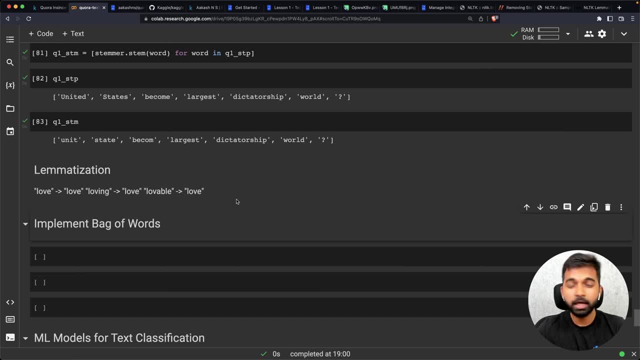 Especially if you have a very large dictionary and it can also take up a lot of memory. So, Because we are going to turn our documents into vectors, Anyway, it doesn't matter whether the short form is something that is just a root of a word or is an actual word from the dictionary. 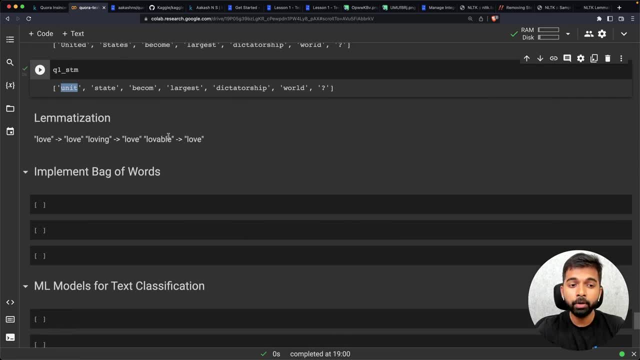 So that's why we're not going to use lemmatization, but in the cases where you want to derive the root word, you can also do that. Apart from all of this, NLTK also allows you to identify parts of speech and do many other things. 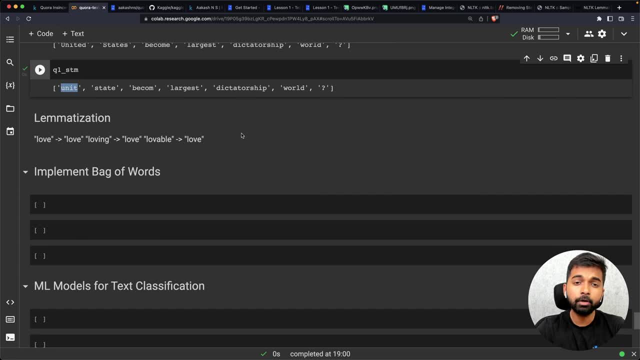 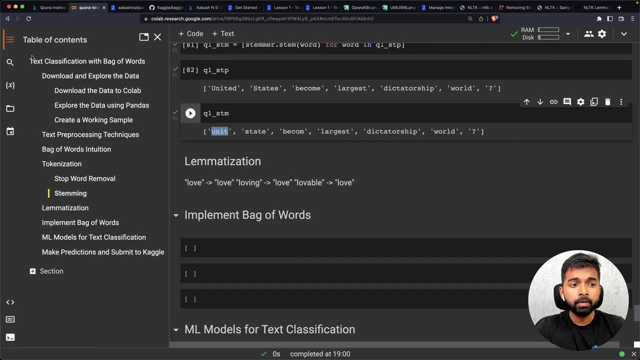 So do check out the NLTK library. You just follow a tutorial, create a notebook on Jovian, experiment with it and you will become a master of NLTK in no Time. So with that we have now completed the second section, which is to perform lemmatization. 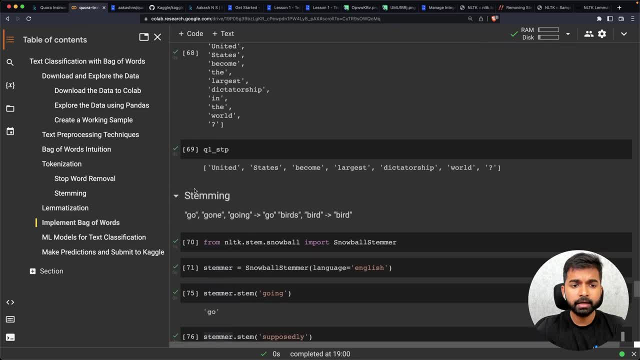 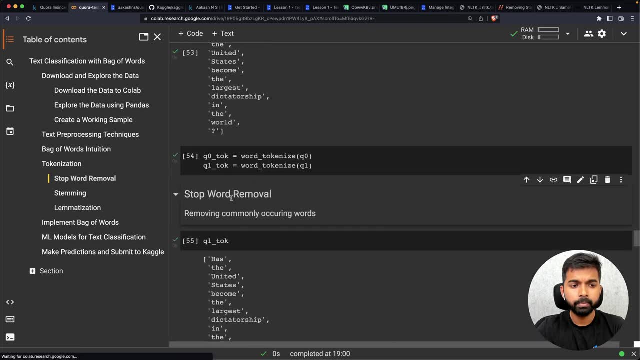 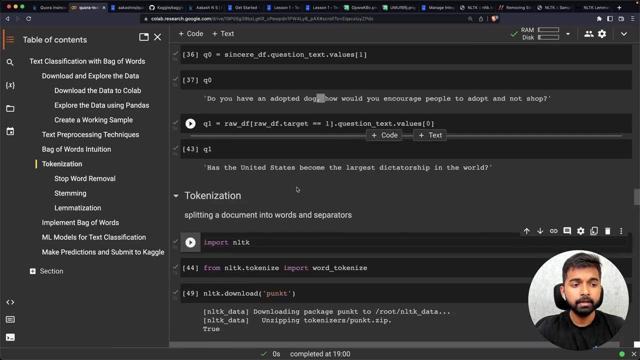 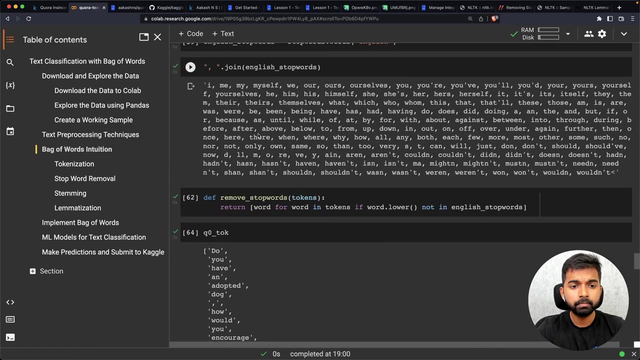 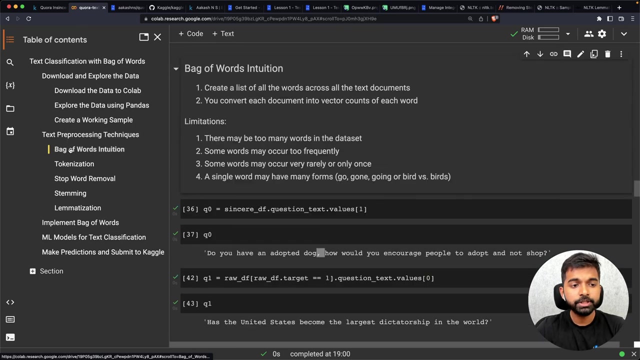 Let's just clean up these headers a little bit so that it's well organized. Yeah, So I'm just using level three headers, putting them under level two headers, so that things are nicely indented in the table of contents. All right, so with that, we have now completed the second section, which is the text pre-processing techniques. 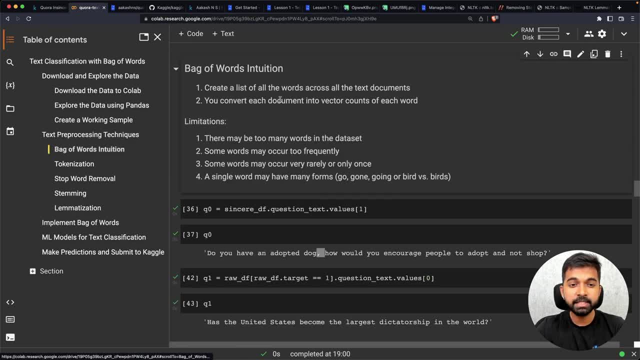 So we wanted to look at the bag of words and intuition. So, basically, how we create bag of words is by listing all the words, then converting each document into a vector using the count of words. But because it has all these limitations- that there may be too many words, some words occur frequently, et cetera- we first tokenize. 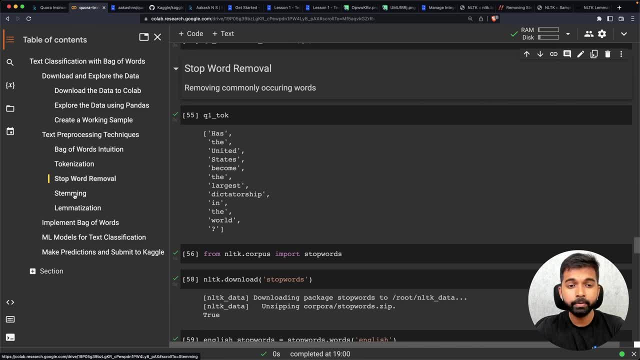 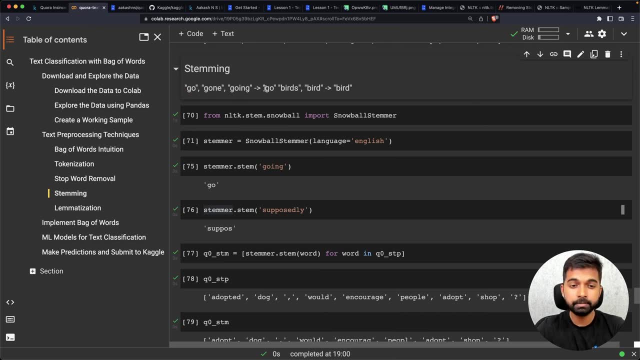 The text, then we remove stop words and then we stem the word. So we go from go, go on going to go, so that that reduces the vocabulary and counts all of these forms as a single word. And optionally, if you want, instead of stemming we can also perform lemmatization. 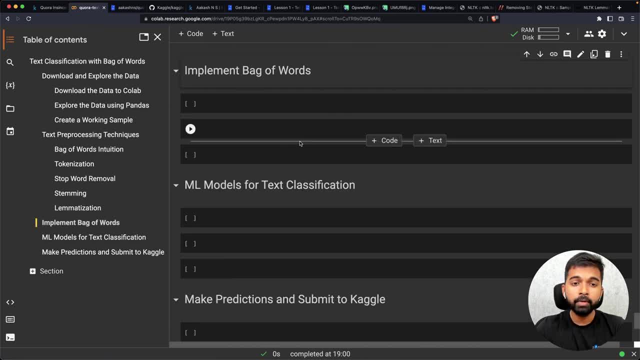 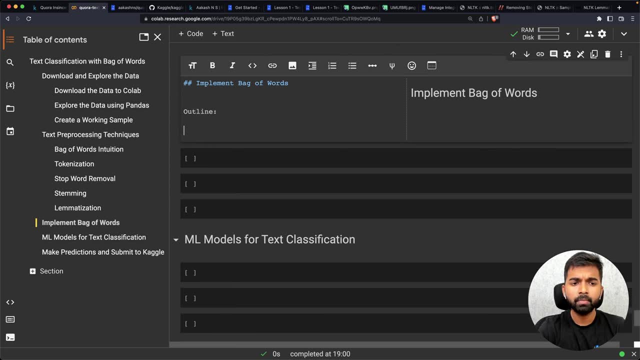 All right. So now we are ready to. so now we are ready to implement the bag of words model. So let's create an outline once again. So here's what We're going to do. first, We're going to create a vocabulary using count vectorizer, and we'll see what that is. 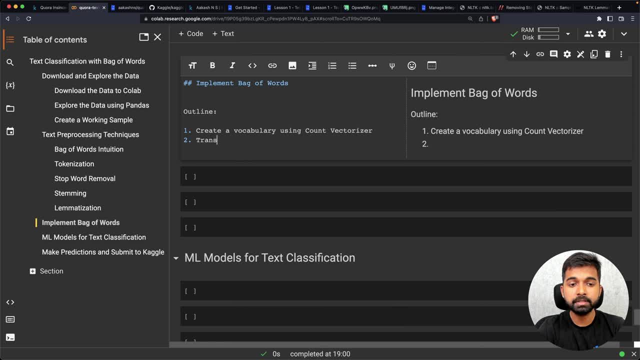 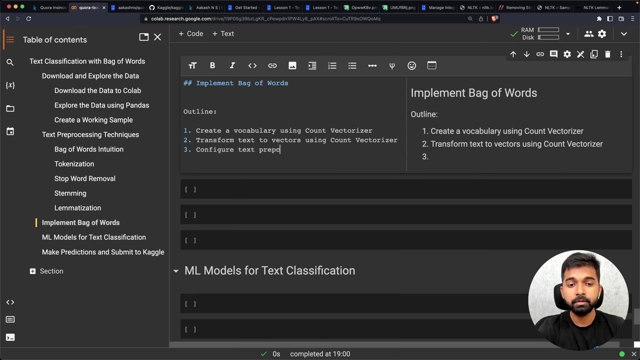 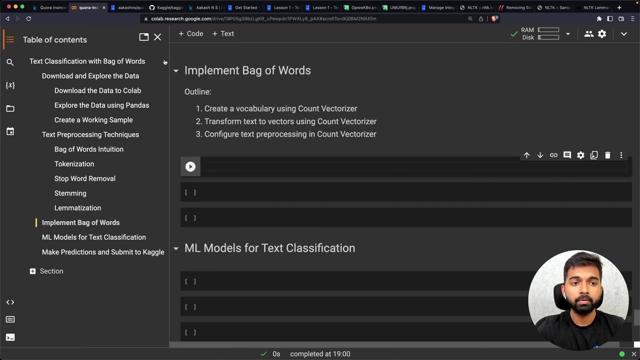 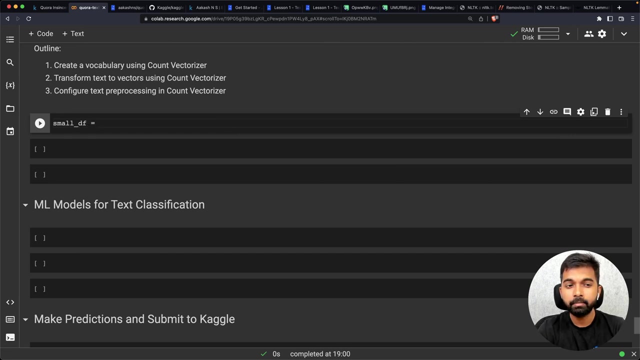 Then we are going to transform text to vectors using count vectorizer And then, finally, we are going to configure text pre-processing In count vectorizer. All right, So here's what I'm going to do. I'm going to create a small sample of just five questions. 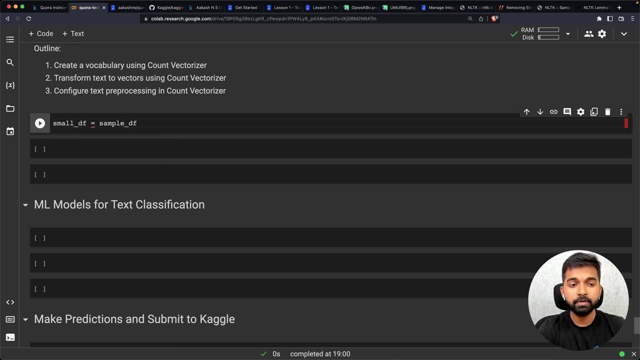 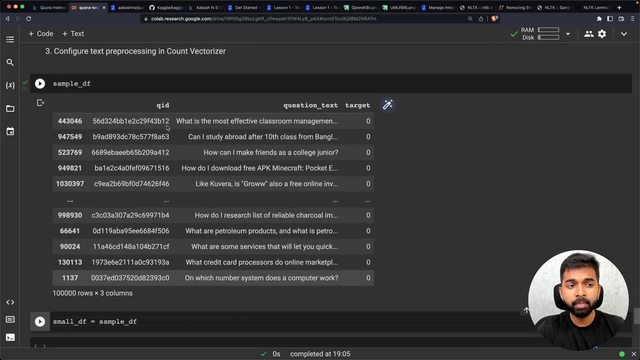 So I'm going to say small DF is sample DF. Remember, sample DF contains 10,000 rows or 10,000 questions. Sorry. So remember, remember sample DF contains 10,000 questions. Okay, Let me say that again. 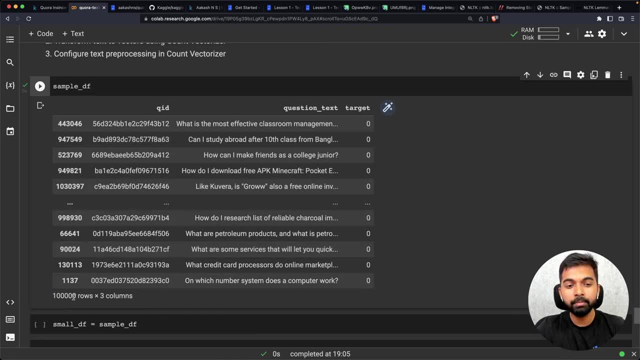 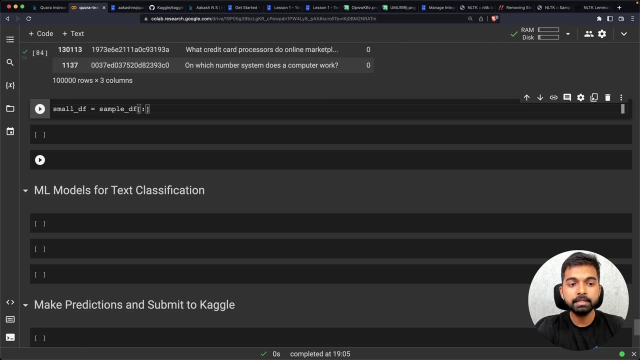 Remember, The sample DF contains a hundred thousand questions out of the 1.3 million. So before we work with the a hundred thousand, let's just work with five questions. So let's create small DF, which contains just the first five questions from sample DF and small DF. 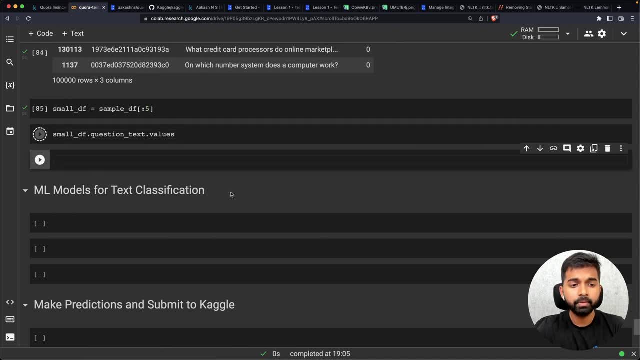 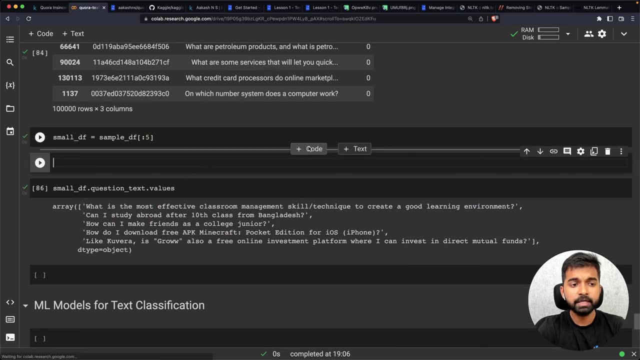 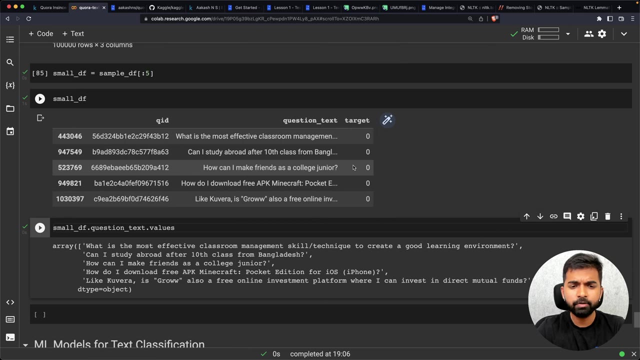 Let's look at the question text values. So these are just the first five questions. And let's look at small DF itself. You can see that all of these questions have the target zero, and that's fine. We're just creating a vocabulary right now. 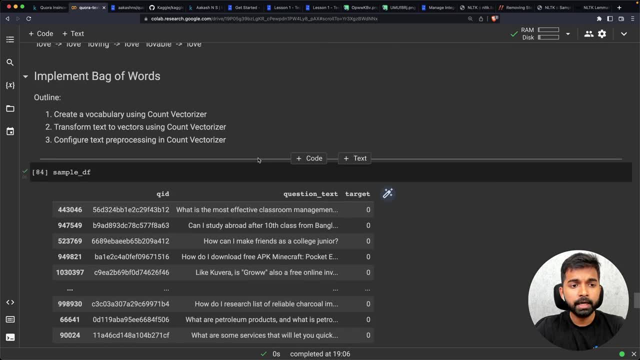 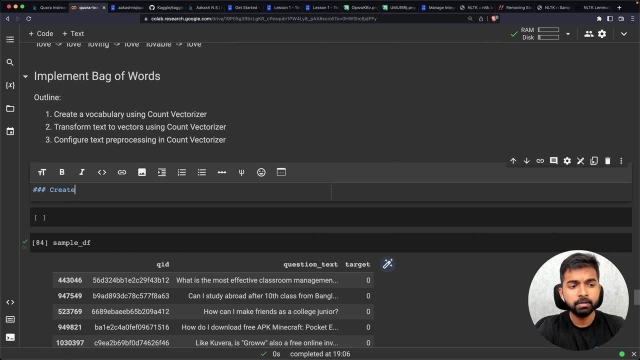 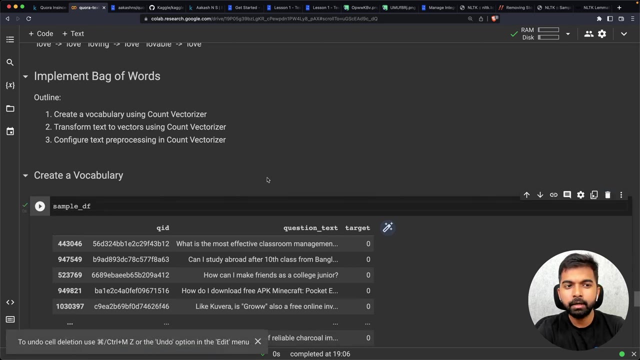 So now we are going to use count vectorizer to create the vocabulary. So let me just create a section here so that our board is a little well organized. So create a vocabulary And count vectorizer is a helper class from the cyclic loan library. 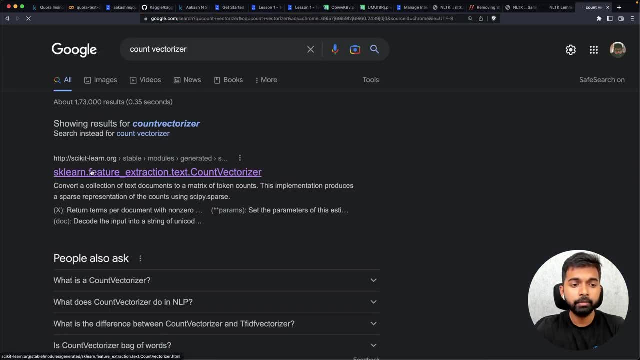 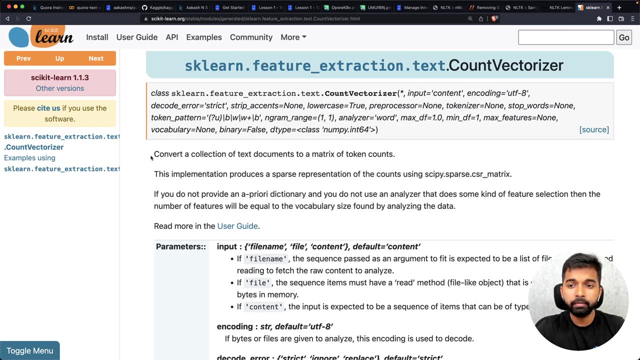 So I'm just going to search count vectorizer. You can see that it is part of the cyclic loan library SK learn. This is where it is located. And what does count vectorizer do? It converts a collection of text documents into a matrix of token counts. 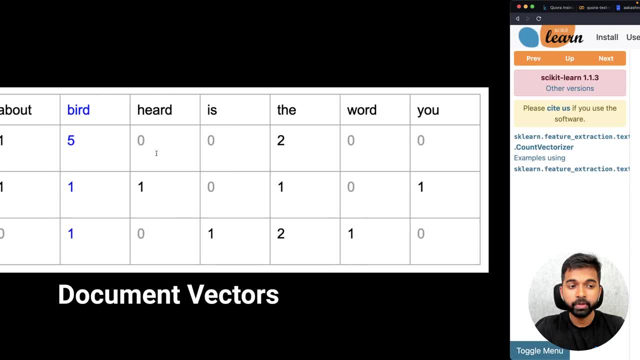 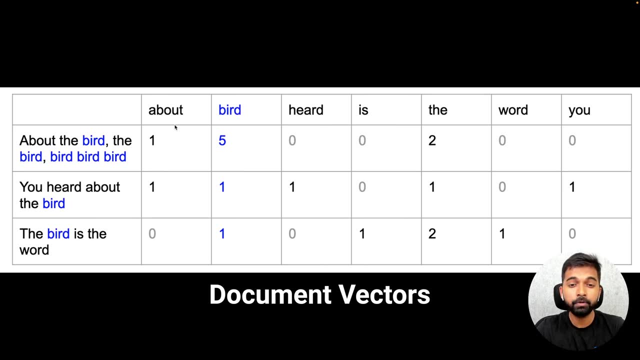 That is just a fancy way of saying that. it creates a bag of words model. So, given a bunch of text, it takes all those text documents, identifies the vocabulary, which is the set of unique words that occur in these documents, and then turns each document into a vector using the counts of those words within those documents. 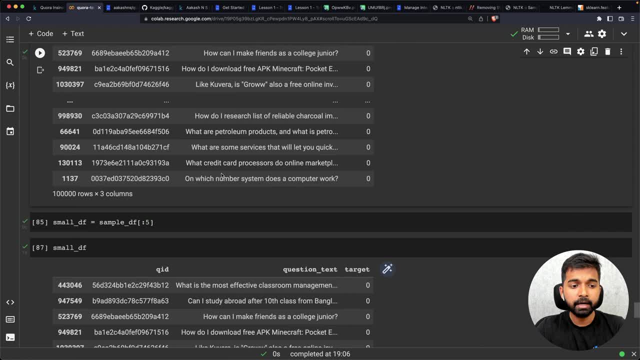 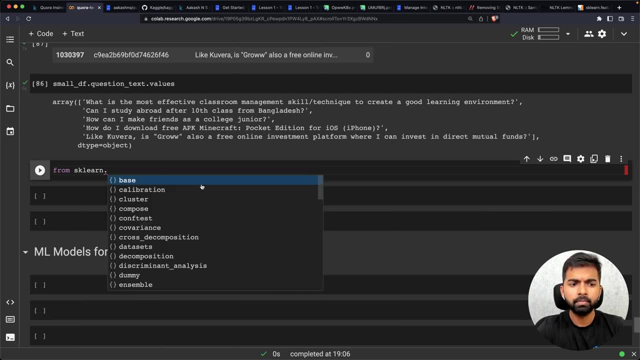 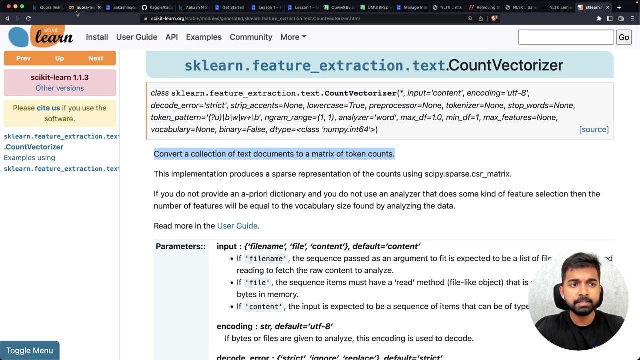 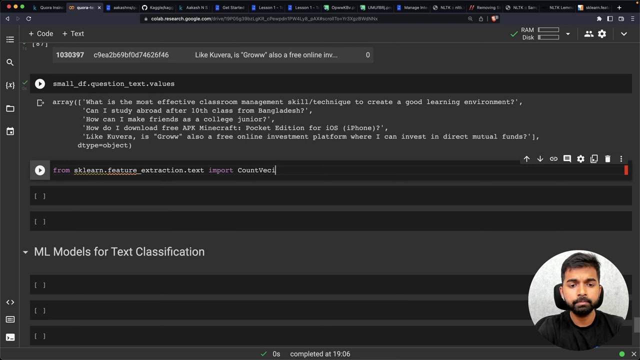 Okay, So let's import count vectorizer. I am going to come down here and I'm going to say import from sklearn. Let's see Feature extractiontxt. So feature extractiontxt, import count vectorizer Done, And let me just create a small vector. Let me call it smallvect is just count vectorizer. 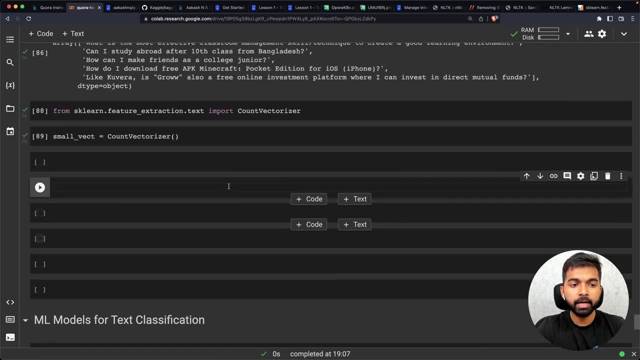 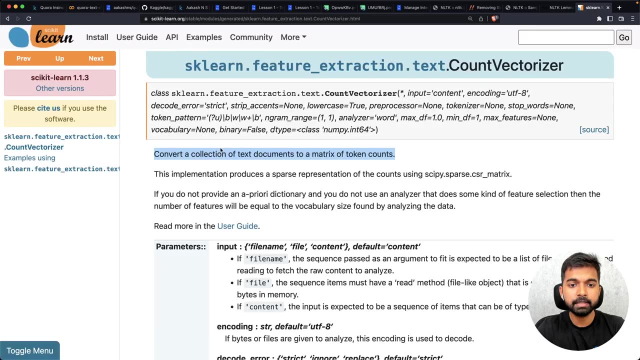 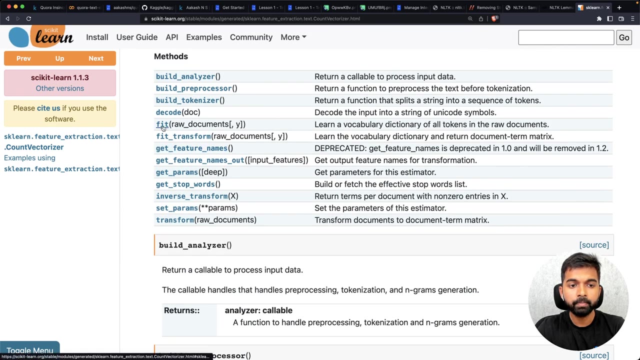 So it can take a lot of parameters, but for now we're not going to take any parameters. And now let us try smallvectfit. If you go into the documentation of count vectorizer here, you can see that once you create a count vectorizer it has this fit function, which. 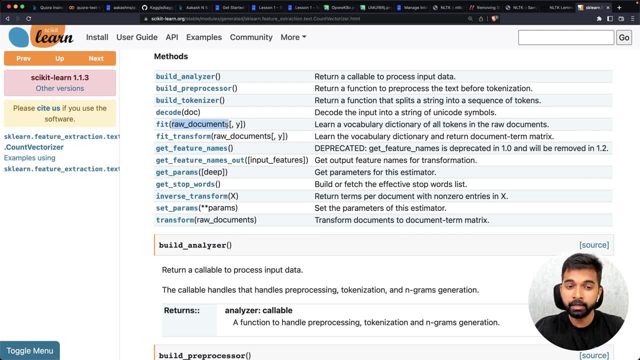 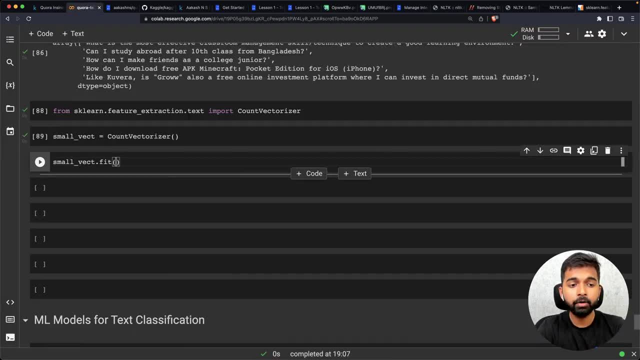 takes a set of raw documents, or a set of questions, in our case, and it learns a vocabulary which is simply the set of all the tokens in those raw documents. So smallvectfit, and let's give it smalldfquestiontext, which is simply these five questions. 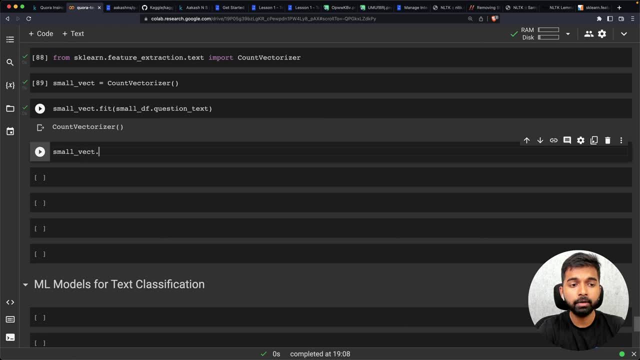 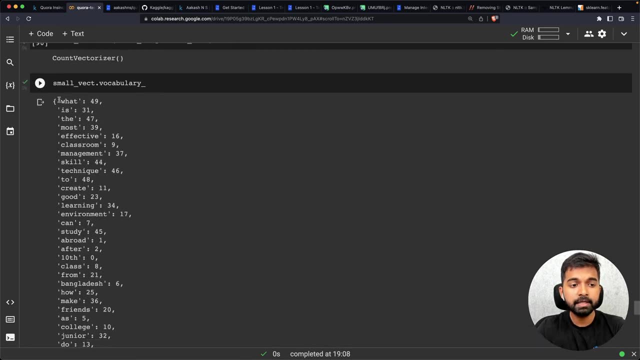 And now it has learned the vocabulary. So now, if you do smallvectvocabulary, underscore again something you can check in the documentation. you can see that these are all the words that it has identified from the five questions. And right now, 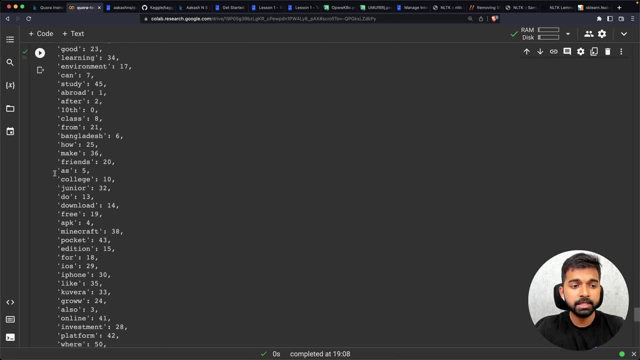 we're not doing any stop word removal, stemming, etc. That's why you see things like a and etc too, And you can see that these numbers start from zero. So the word 10th, as the numbers, hasn't position zero, And similarly the word abroad has a position one. So these words are sorted. 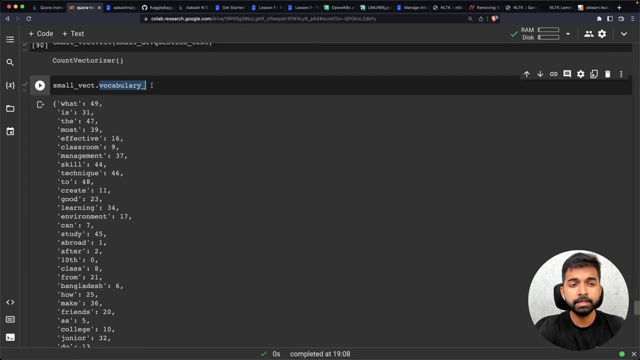 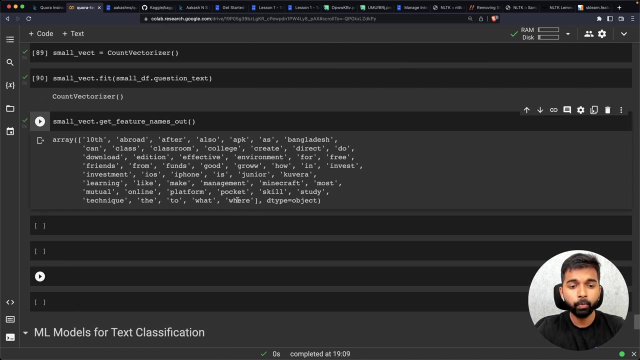 in alphabetical order. If you want to see just a list of words, you can also check dot, get feature names out And that's going to give you the actual list of words that have been picked up in the vocabulary. So, 10th to where these are wrong. 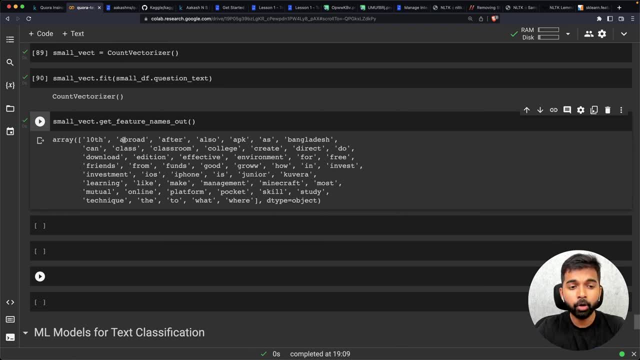 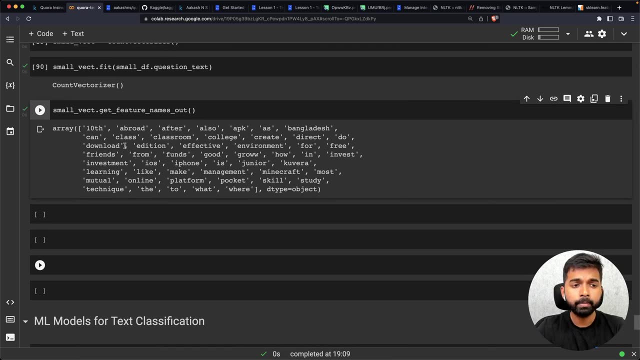 all the words in the vocabulary. 10th would have the position zero abroad, without the position one. after that would have the position two, and so on. All right, So that is how you learn a vocabulary: by building a count vectorizer. Now, so far we've learned the vocabulary, but we have not done the second step. 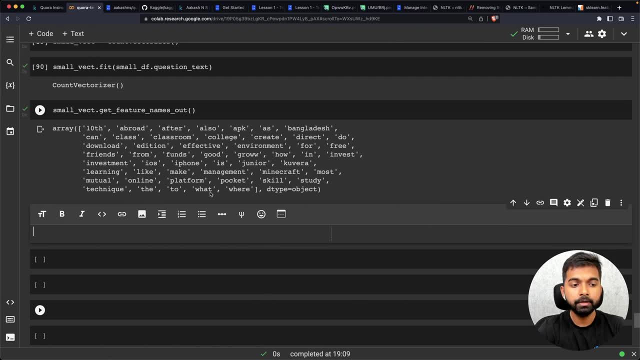 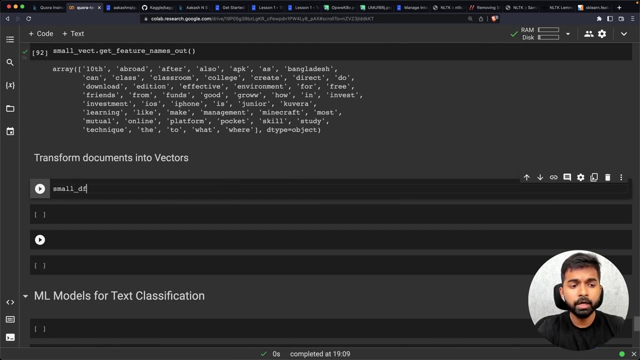 So we've done this step, but we've not done this step. So now let us transform documents into vectors, And again, this is fairly straightforward. So here we have small df, dot, question, text or values. These are all the questions that we have. 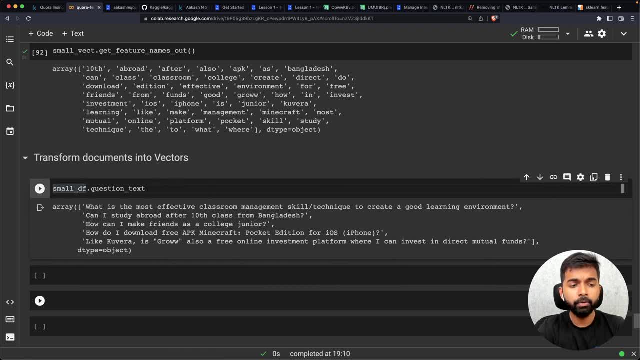 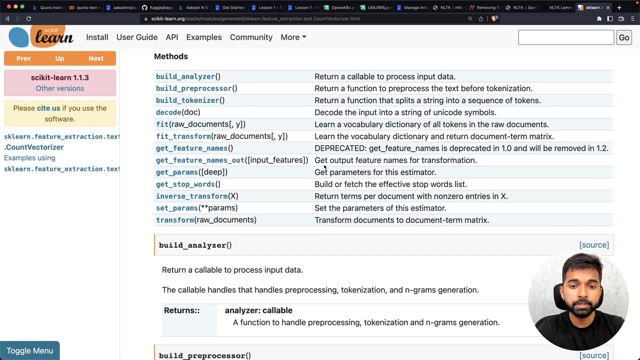 And if I simply pass this into small vec, dot transform. So dot transform is the method available. Again, all of this is documented here. Dot fit is used to learn a vocabulary. dot get feature names out is used to get the output. We. 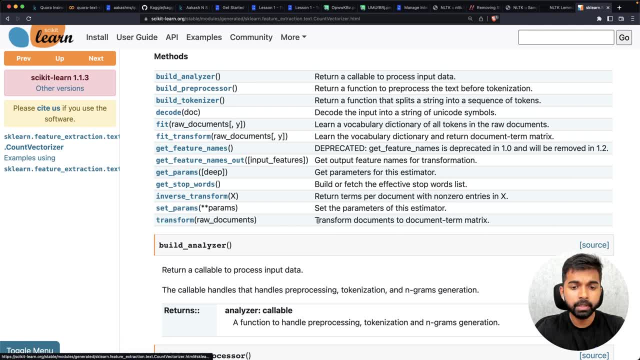 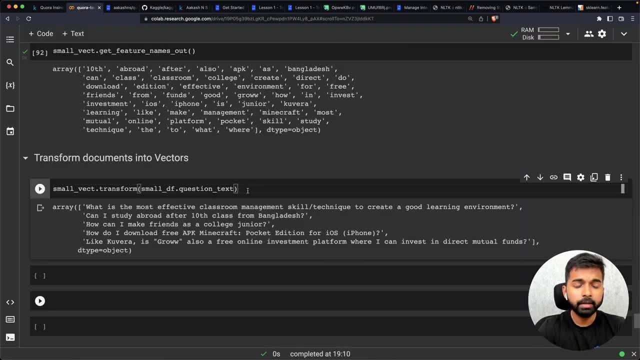 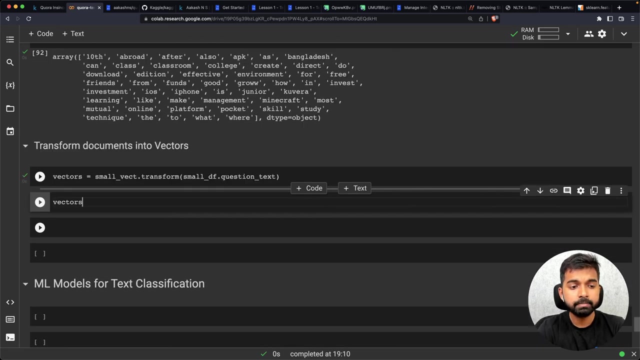 And finally, dot transform is used to transform raw documents to a document term matrix, which is basically the bag of words vectors. All right, So we're going to transform it and store it into this variable called vectors. Okay, And let us check vectors. 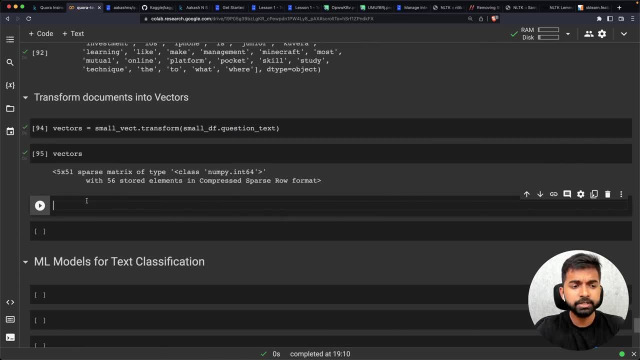 And it says: vectors is a Sparse matrix of type such and such. well, because there are lots of zeros, So because there are 56 entries in a vocabulary and a particular sentence, we only have five or six of them. So most of the vectors will have a lot of zeros. and to store this efficiently, 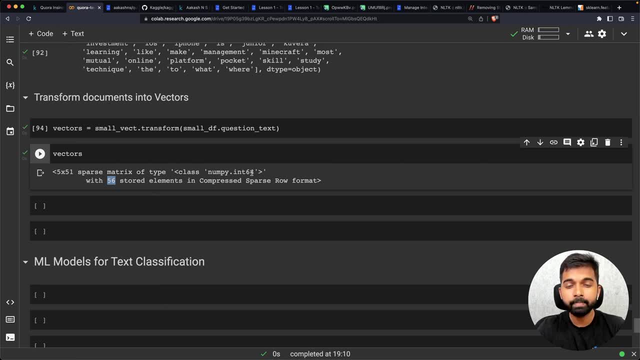 Number internally uses something called a sparse matrix, So that's why you're not seeing the full value here. but if you ever want to see the values inside a star sparse matrix, you can do dot two array. Now, be careful while doing this with a very large sparse. 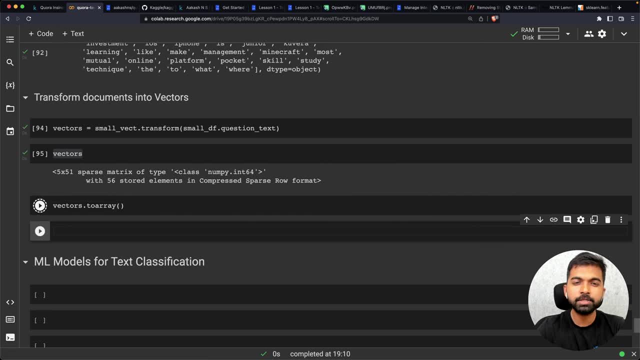 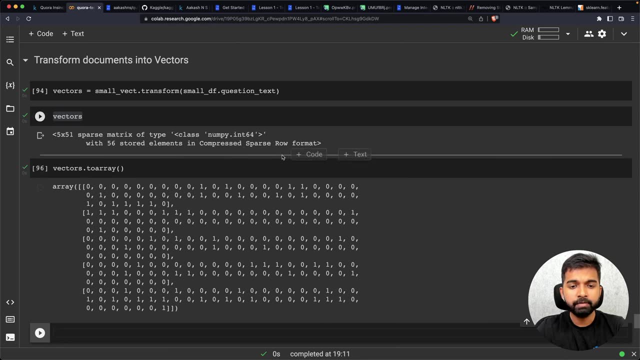 Sparse matrix, Because this can run out of memory. but in this case our sparse matrix itself is quite small, so we can convert it to array. So you can see now that we have in this vectors and we can also check it shape. 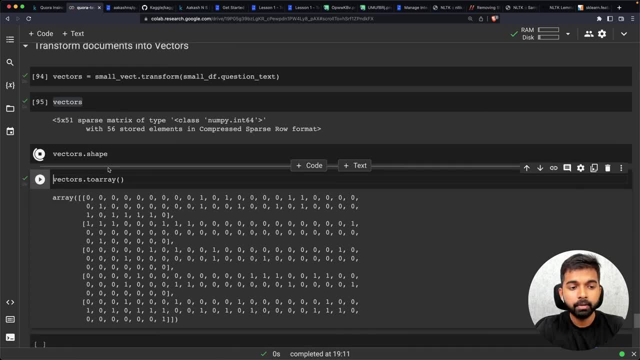 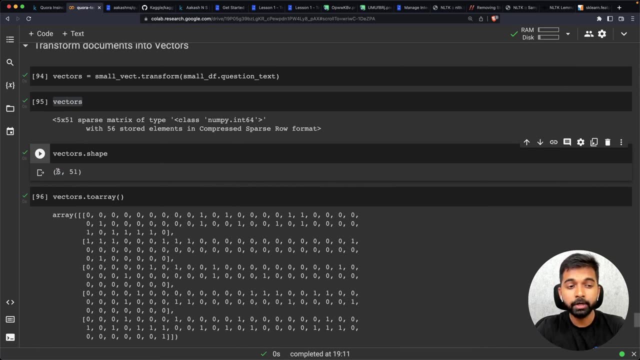 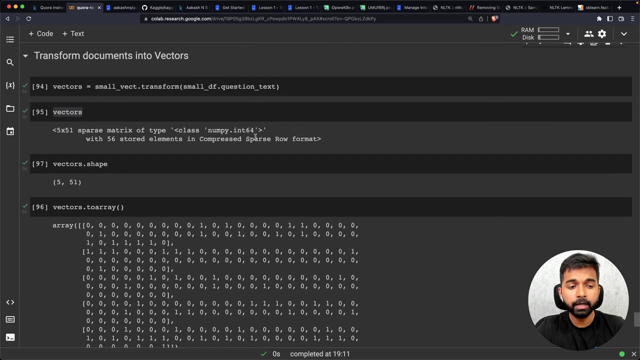 So we can say: vectors dot shape. So it has five rows, one row for each or one vector for each question, And it has 51 columns, because there are 51 entries in our vocabulary, All right, So what does This represent? this represents the first vector, which is this: 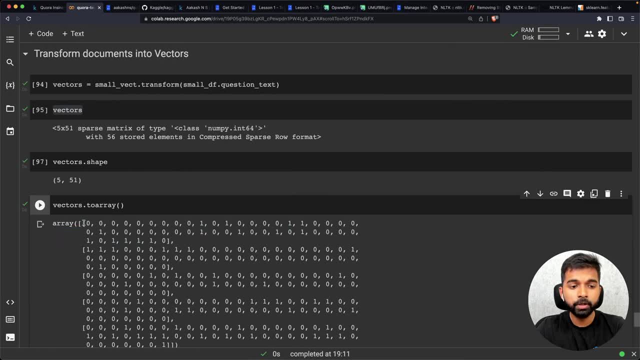 So it represents exactly this. You can verify that if you go in here and check the position, at which you have a one zero one, two zero one, two, three, four, five, six, seven, eight, nine, 10 at the. 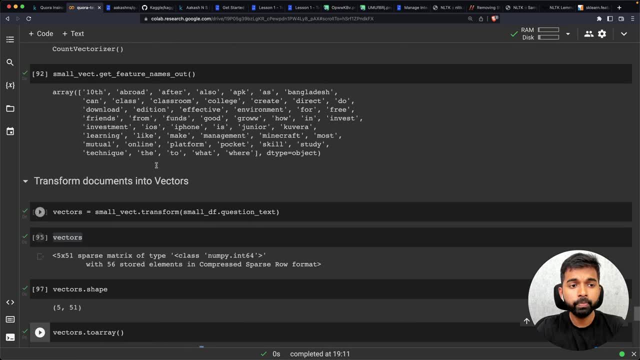 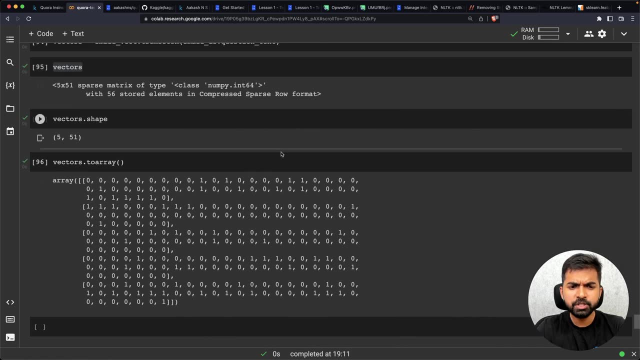 10th position we have a one. What does that correspond to? Zero, one, two, three, four, five, six, seven, eight, nine, 10.. That corresponds to college. And let's just check out the first question. 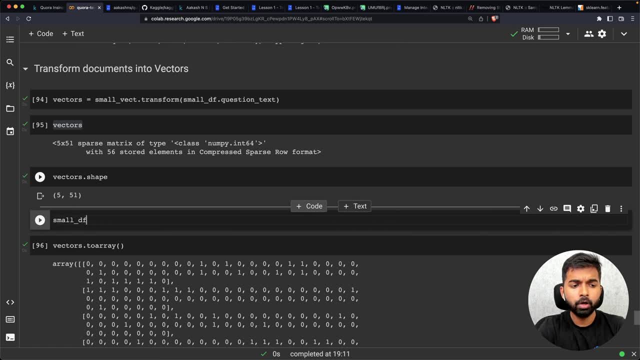 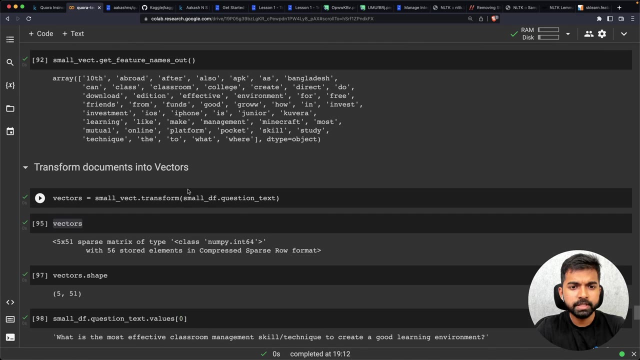 So let us just check Small df dot question X: zero. dot value zero. So it says that, all right, what was this One, two, three create? Yeah, it was probably create right, One, zero. one, two, three, four, five, six, seven, eight, nine, but it was classroom. 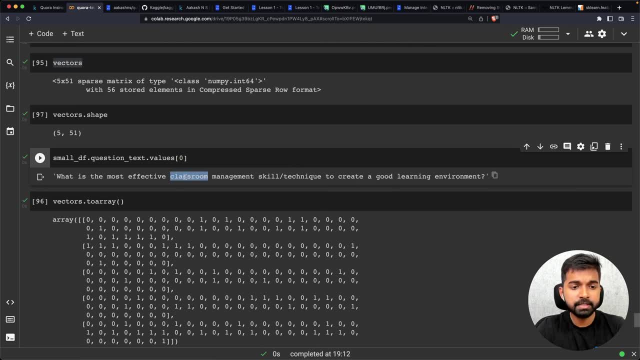 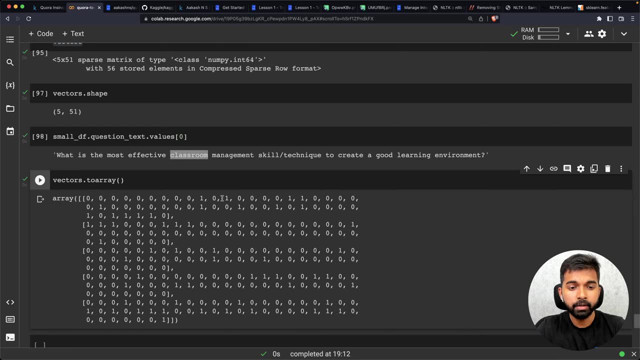 And clearly there's a classroom here. So you can see that this classroom here And you can see that this classroom here, and when there is a classroom here at the position 10, that has a value one. similarly to positions after classroom there is a one. 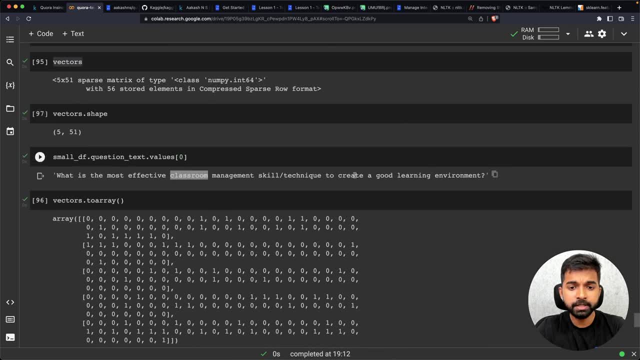 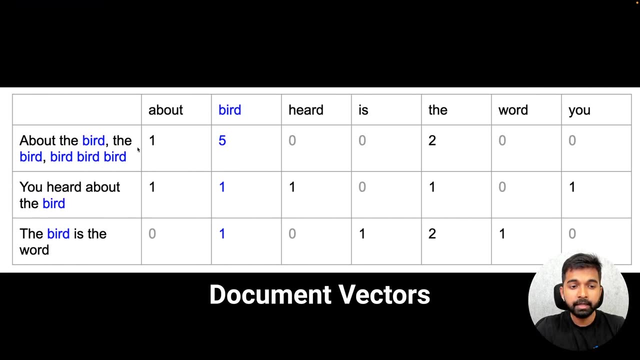 So what occurs after classroom? create and clearly create as present in the world. So we've done exactly this: We started with these, we identified the words and then now we have turned each of these questions into a vector, and the numbers in the vectors indicate simply the counts of those words, those specific 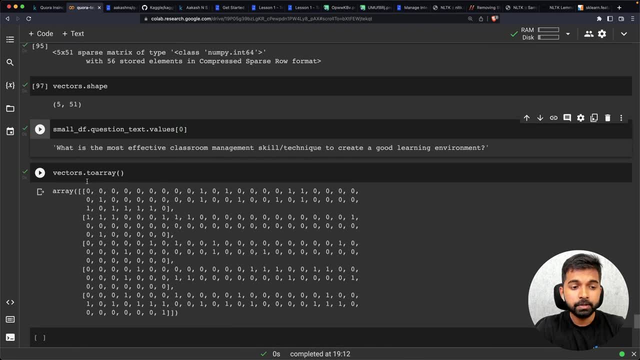 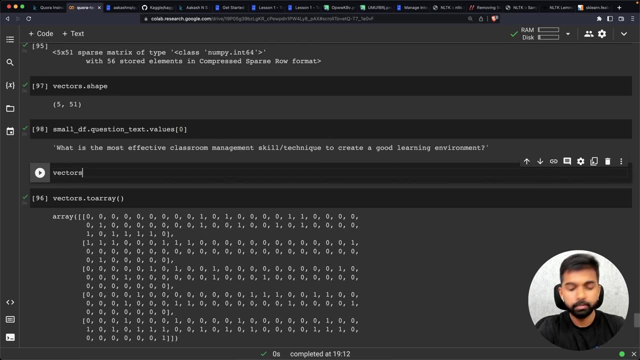 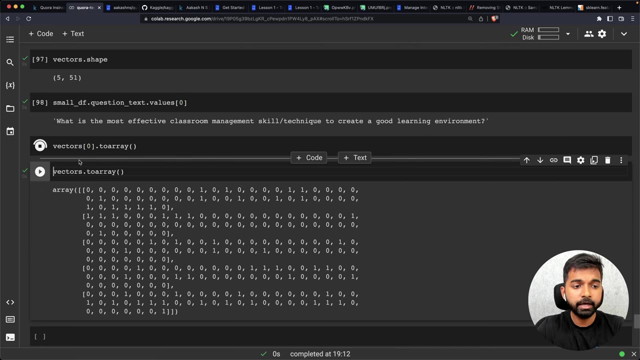 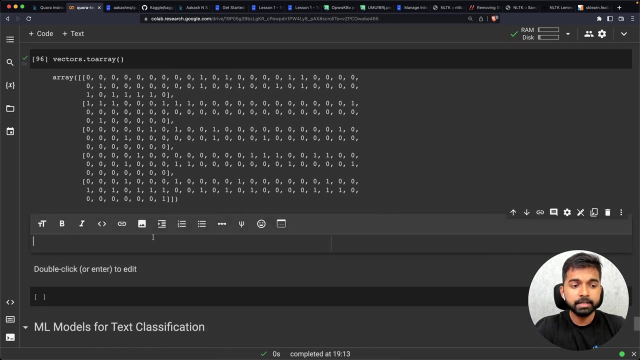 vocabulary words in that question. All right, So that's one vector. You can look at an individual vector as well. You can say vectors zero, dot, two, array, And this is an individual vector here. All right, Perfect. So now that we've done this next step, now let us look at the step of actually 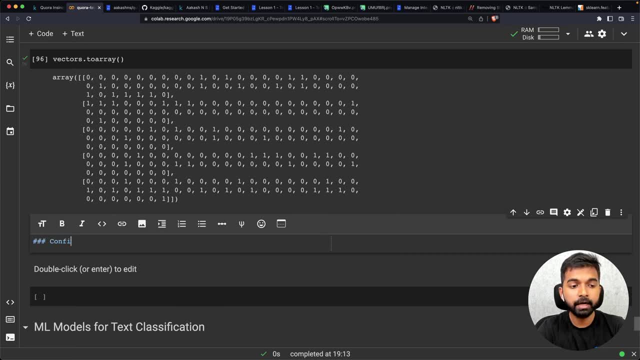 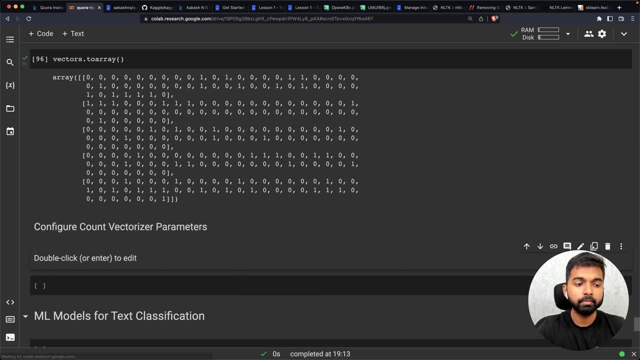 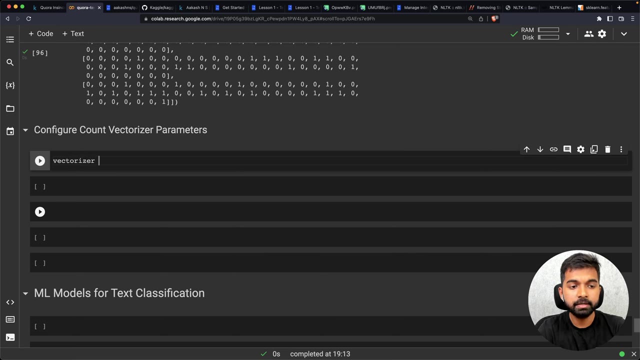 configuring the count vectorizer and using it for the entire data Set. So configure count vectorizer parameters. So let's create another vectorizer. Let's say vectorizer equals count vectorizer. But this time we're going to pass in a few arguments. 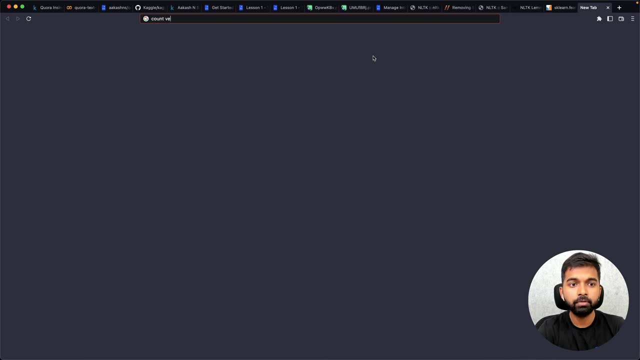 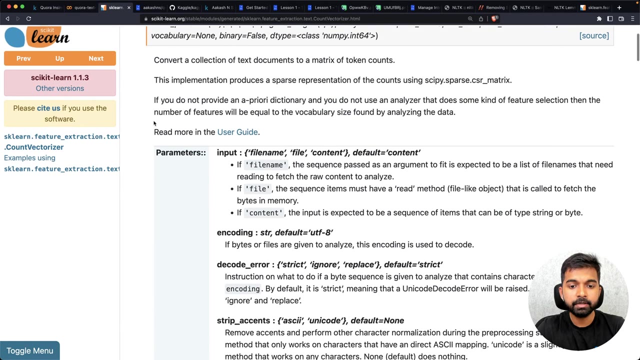 So going back to count vectorizer, So let's once again search count vectorizer. Now, going back back to count vectorizer, you can see that it has a bunch of arguments. The first one is called input, which simply takes what type of input you're passing. 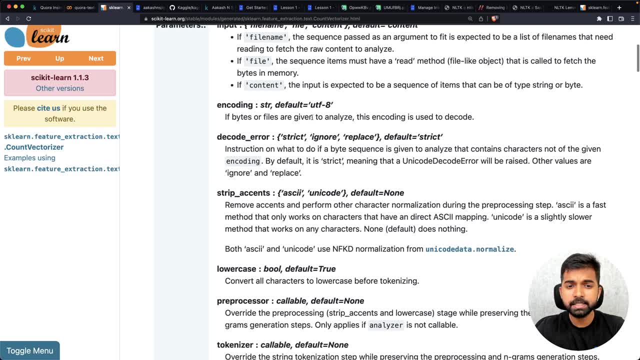 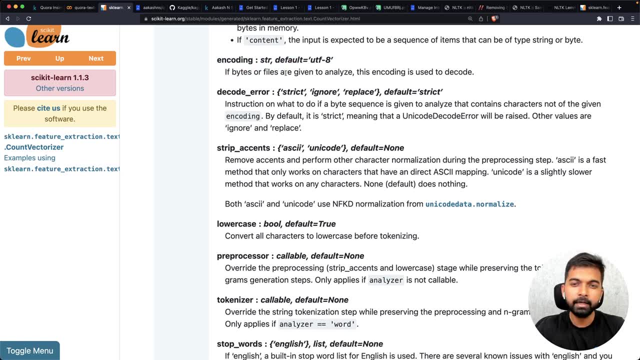 Are you going to pass a file or a file name or some content? Well, we are passing the content directly, So that's okay. We can leave the default value. We need not concern ourselves with the encoding, but if you find any errors in encoding, you can use that. 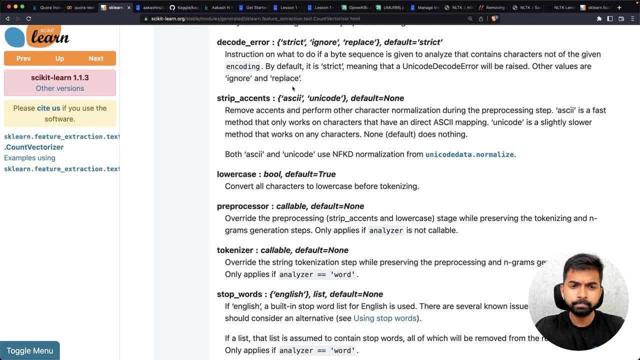 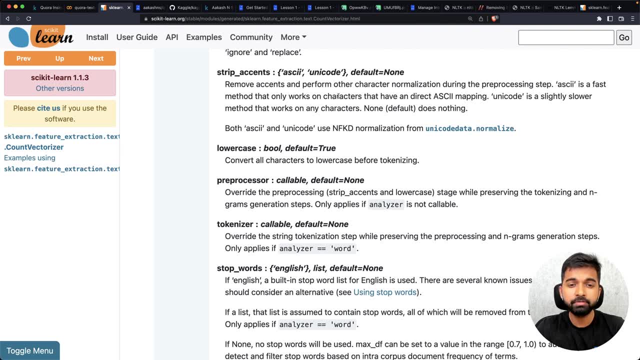 We need not concern ourselves with decoding either. We need not concern ourselves with strip accents again. unless you're working with some European language which may have accents, you need not concern yourself with it. lowercase. Okay, This is something that we may want to set. 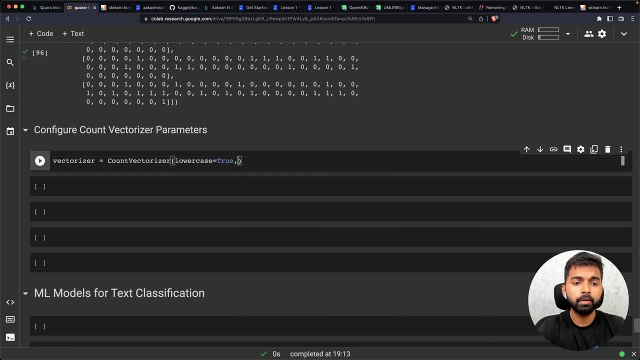 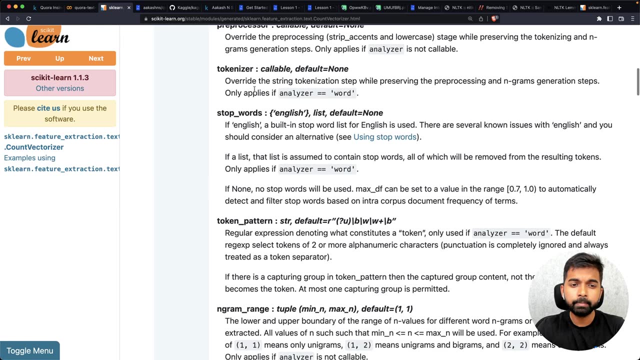 So I'm just going to set lowercase equals, true. What else? What else do we have here? Reprocessor? Well, do we need some kind of preprocessor? Probably not tokenizer, So it has its own tokenizer built in, but you can provide a tokenizer. 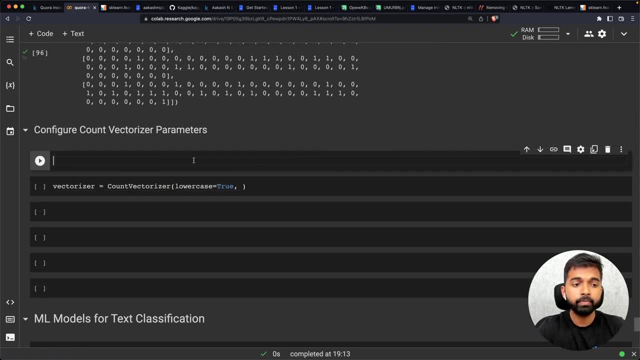 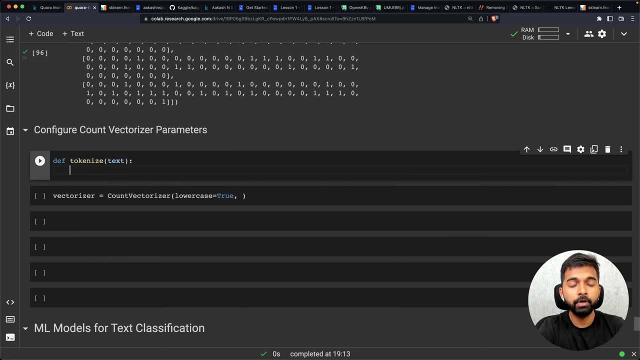 So let's try and provide a tokenizer, Let's define our own tokenizer, So def tokenize, Which takes some text, and in the tokenizer we are also going to perform stop word removal. So remember, we have imported word tokenize, So word tokenize, token, or, or let's just say word tokenize. 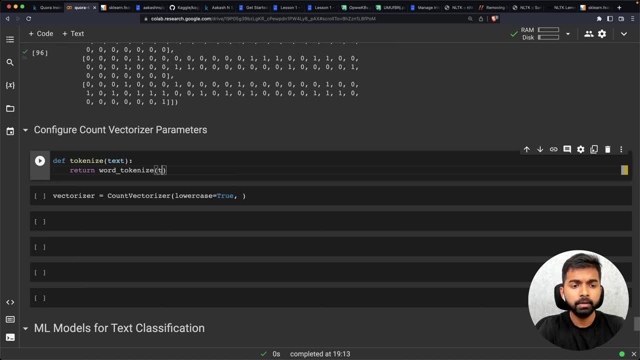 Well, that would just tokenize the text. Yeah, Word tokenize text would just tokenize the text. but we also want to remove stop words. So let's also do that. Let's say Word for word in word: tokenize text If word dot lower, not in English: stop words. 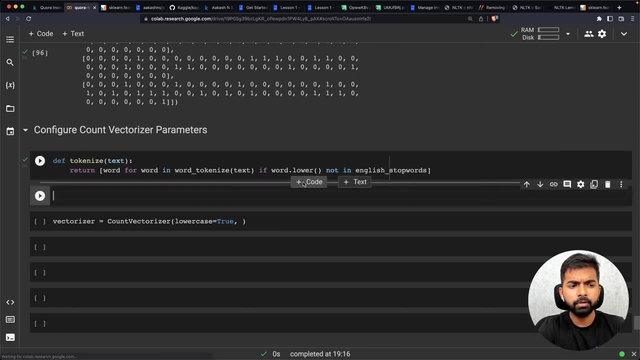 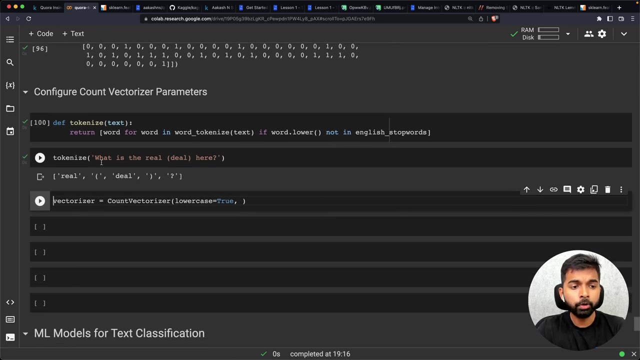 All right. So let's test this function out, Tokenize And let's say what is the real deal here. You can see that it has not only tokenize the text, but it has also checked the English stop words and it has removed the stop words. 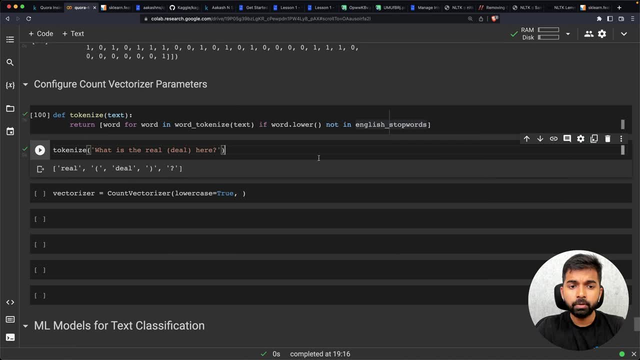 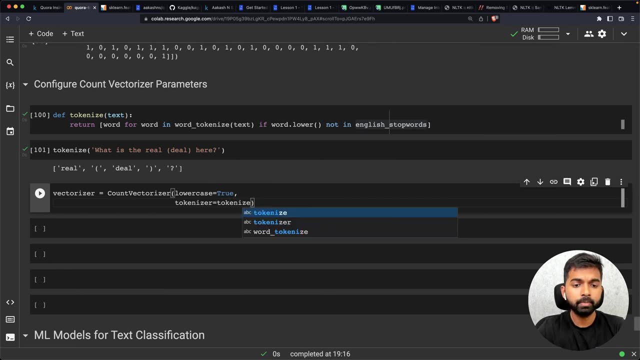 Like what is in the right. So this is the tokenizer that we're going to use. So I'm going to pass a tokenizer and that is just my tokenized function. In Python, you can actually pass a function as an argument. That's very interesting. 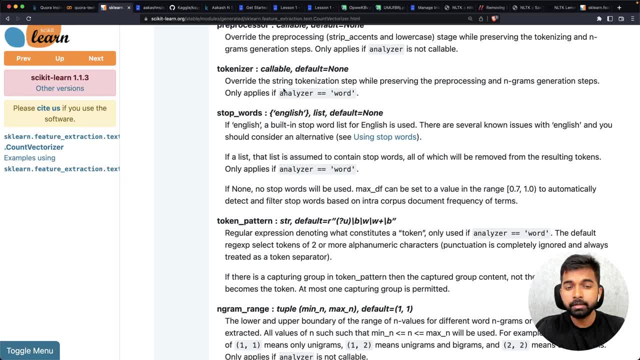 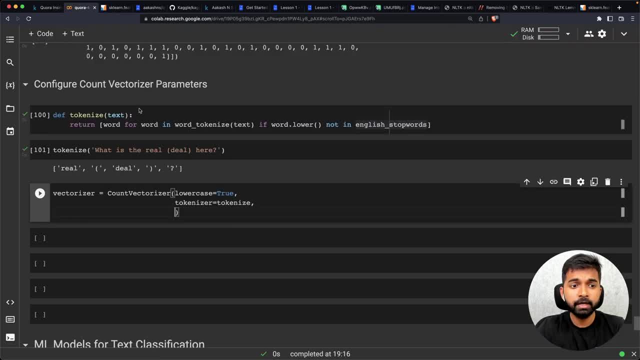 Okay, So now we've provided a custom tokenizer and we've also provided a custom stop word list. So here's something you can do. You can actually provide a stop word list here. So we didn't need to This. we could actually just provide a list of stop words directly. 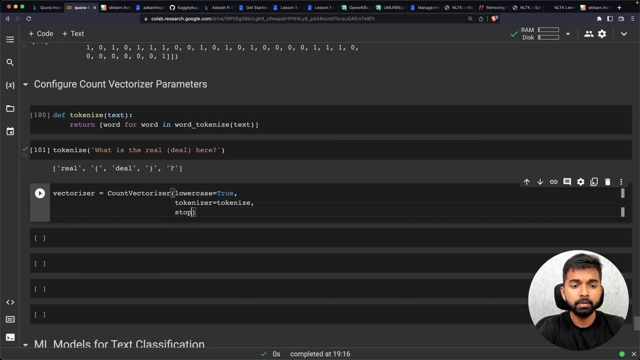 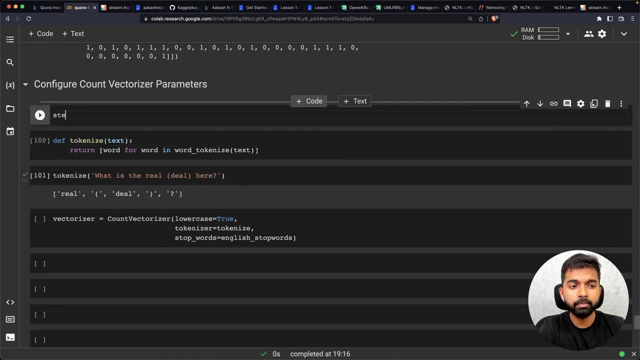 So if we don't need to do this, we can just say: stop words equals English stop words. Now, one thing we do need to do is perform stemming, And that is something we may actually do want to do here, So I'm going to create a new stemmer equals snowball stemmer. 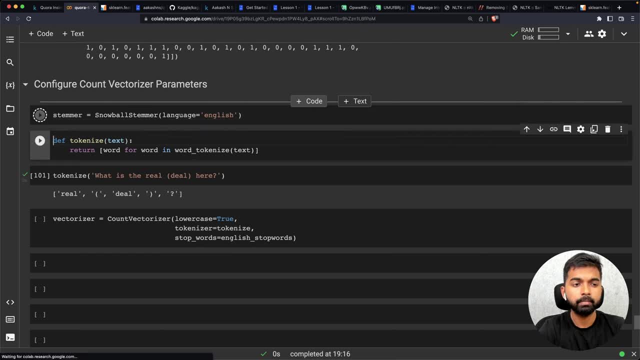 Language: English. Now the stemmer is created and I'm just going to stem this word. So stem stemmer. STEM word or word in word, tokenize, And let me just put in some forms here which may require stemming. You can see, now we are no longer performing stop word removal because we are 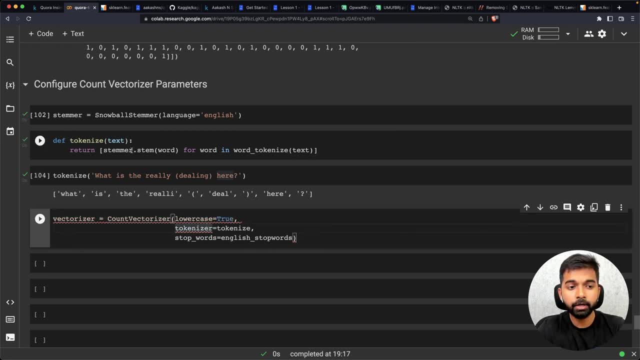 providing a list of stop words here into our vectorizer, So that's not required in our tokenize. However, we are performing stemming using the snowball stemmer for the English language, So you can see that really has been reduced to R-E-A-L-L-I, So that's something that stemmer does and dealing has been reduced to deal. 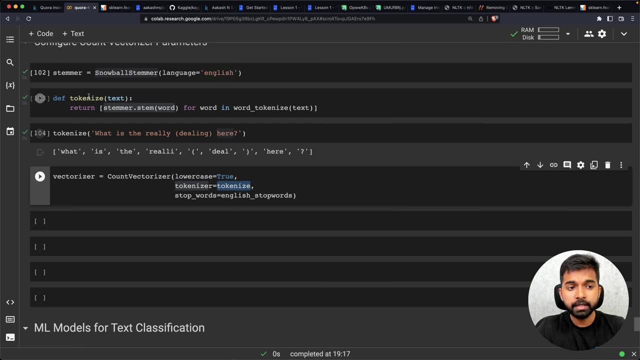 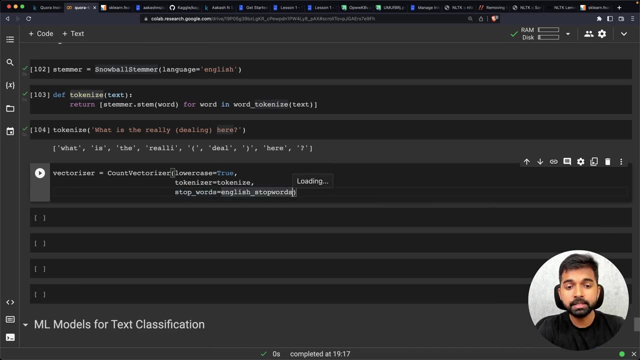 and so on. All right, So now our tokenizer, our tokenize function, which is passes tokenizer, is going to perform tokenization, It is going to perform stemming, and then the stop words are passed in directly. So we don't need to perform stop word removal here, It's done by the count. 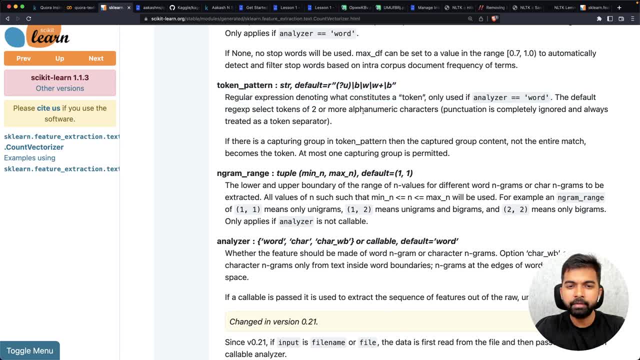 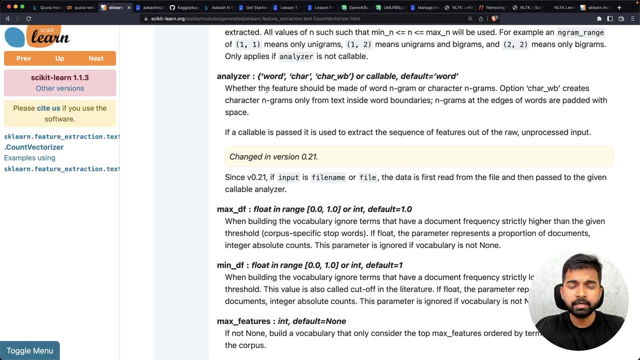 vectorizer, Then token pattern- Well, not relevant here, because we passed a custom tokenizer. Ngram range is not something we need to worry about. Analyzer: again not something we need to worry about. You can check out all the other options, but here is one I'm really interested. 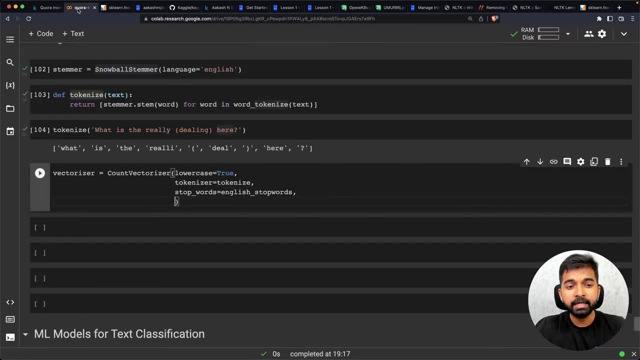 in which is max features. Remember, we said that the vocabulary size may become too large. We may end up with a 100%, Hundreds of thousands of individual unique words. So you can actually perform, you can actually pass max features And if you say max features equals thousand, let's say: 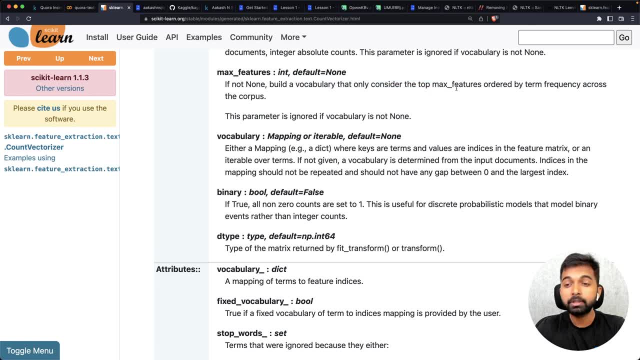 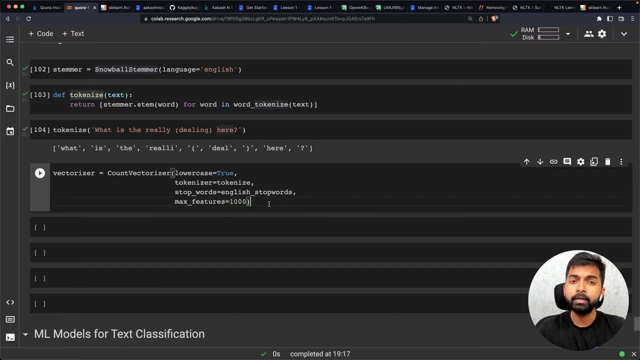 then the vocabulary will only consider the top thousand words or terms in the dictionary occurring in the data set. So now our vocabulary is not going to contain all the words that have been obtained after stemming and stop word removal. It is going to contain only the thousand. 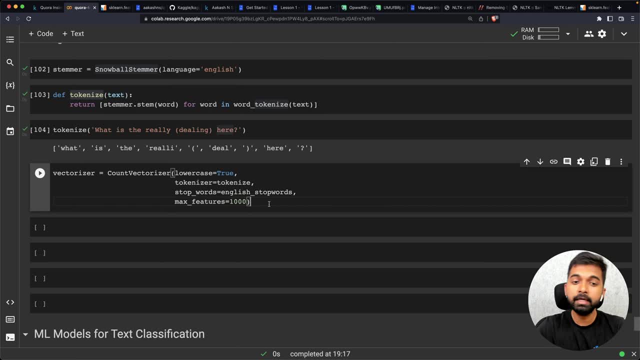 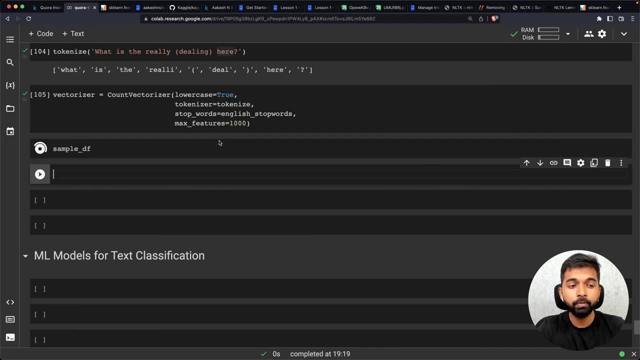 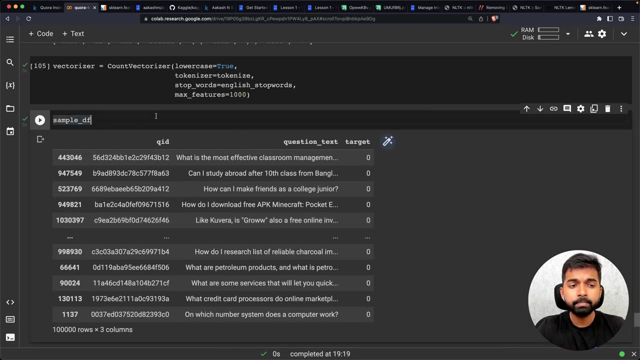 most common words. Now we have a vectorizer and now we have our sample data frame. Remember the 100,000 words that we have picked, the a hundred thousand questions. So now we have a sample data frame containing a hundred thousand questions. So we are going to now first learn the vocabulary. 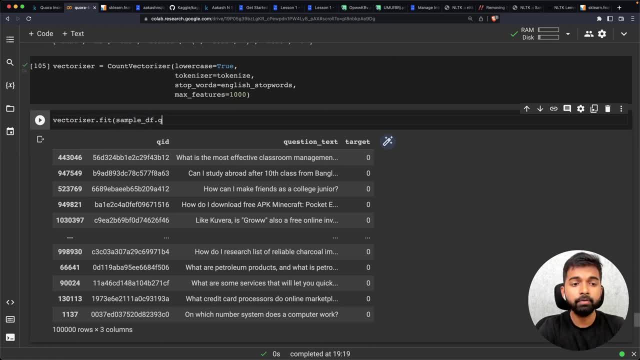 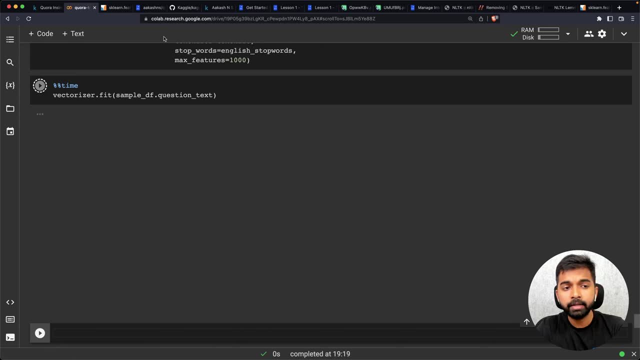 So vectorizer dot fit sample DF dot. question text. Now we're going to learn the vocabulary- vocabulary from the entire sampled D F. I'm going to run that. So whenever I run a command that is going to take some time to execute, I add this: 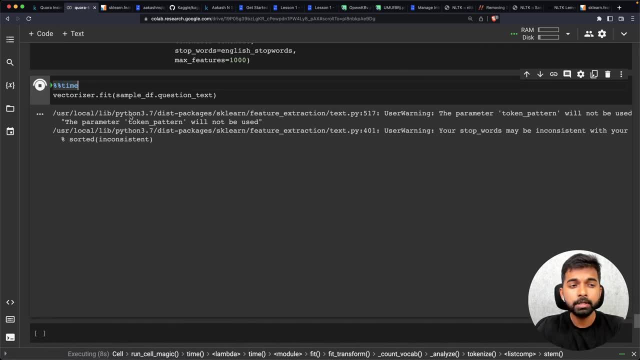 percentage percentage time at the top of it in the Jupiter notebook. So that just prints out the amount of time it took to execute, just for future reference. Now, in this case we've passed sample D F dot question tech into vectorizer, which is: 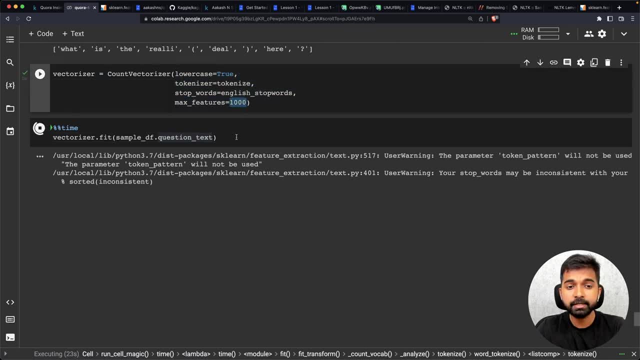 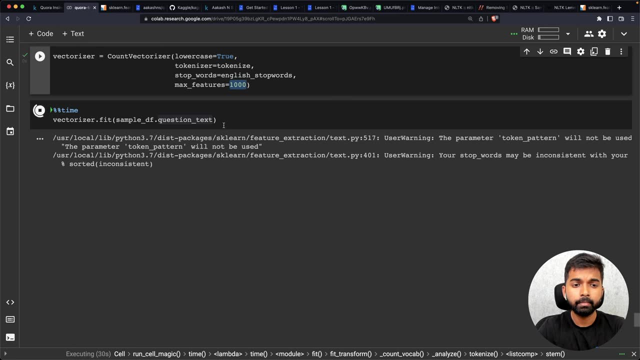 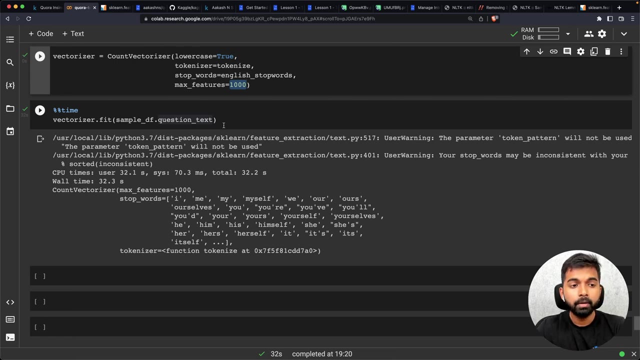 performing all of these pre-processing and is only going to create a vocabulary of size 2000,. and that is going to now learn the vocabulary for us. All right, So it seems to have learned the vocabulary already and we can check the vocabulary. 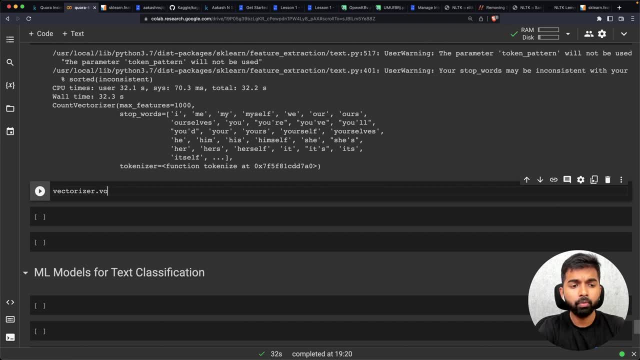 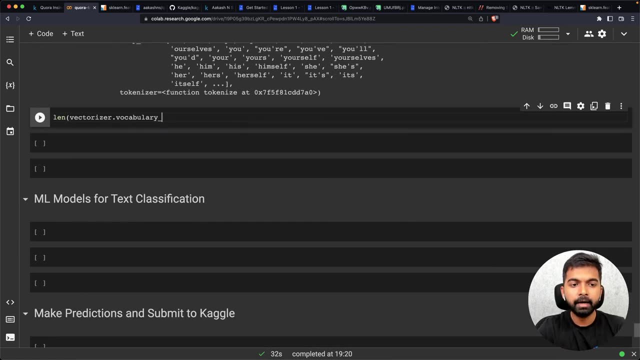 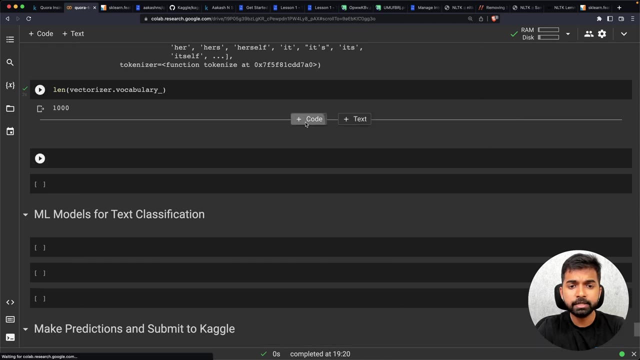 So I can say: vectorizer dot, vocabulary underscore. now I may not want to print the entire vocabulary. I can just check the length of the vocabulary and looks like the vocabulary is of size 1000.. So that's great, That's what I expect. 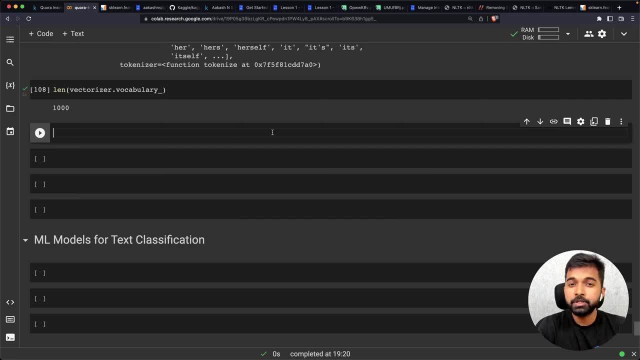 And you can experiment with the values 2000 or 3000.. It's just going to take a little longer. That's why I chose not to do it. We can also look at some of the first few values. So let's say, vectorizer dot, get feature names out. 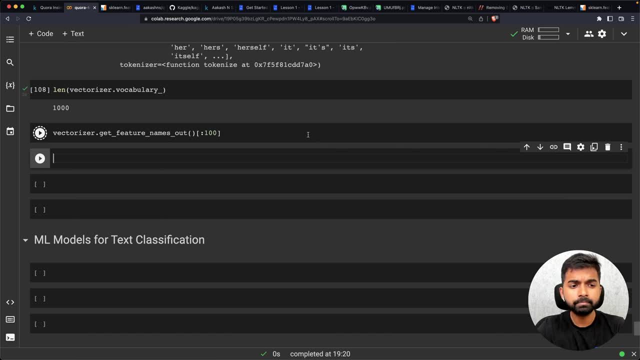 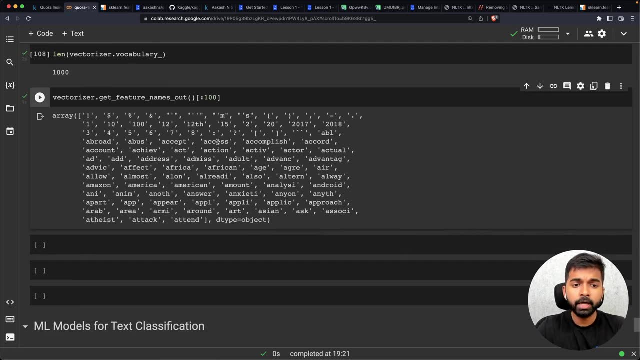 And let's look at maybe the first hundred words. So these are the first hundred words in the vocabulary: a bunch of punctuations followed by a bunch of words. You can see that we have performed stop word removal here. Clearly, we have also stopped word removal and stemming here. just by studying these tokens. 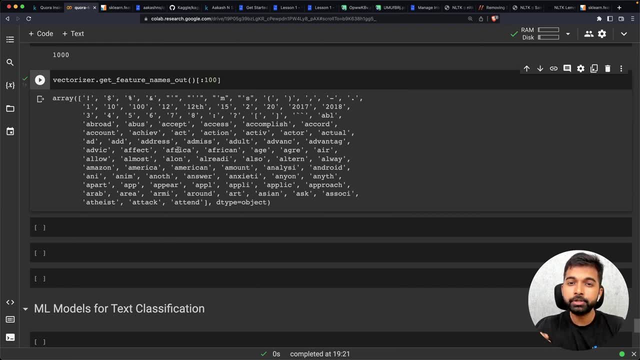 And this is always a good idea: as you are working on a project, make sure to print things out and verify that they're working as expected, because you may have forgotten something somewhere. for example, checking lowercase and things like that. All of those things become clear. 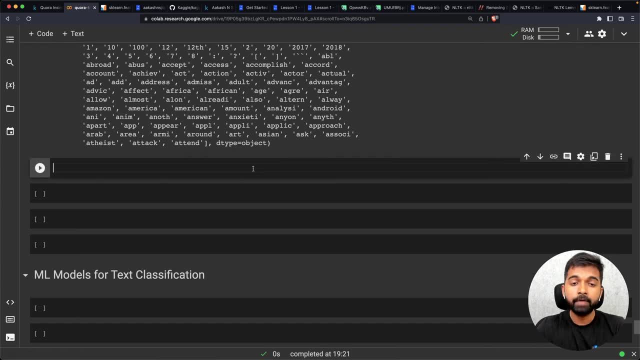 When you print things out. okay, now we are finally ready to actually convert and transform our text questions into vectors. So I'm going to call this inputs, because these are going, these vectors are going to be inputs into a machine learning model. So inputs equals vectorizer, dot transform. and let's give it sample DF, which contains: 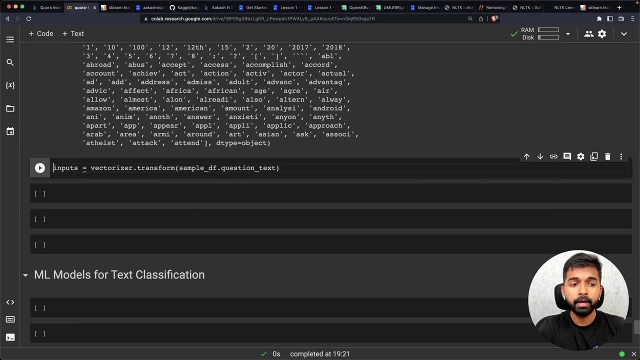 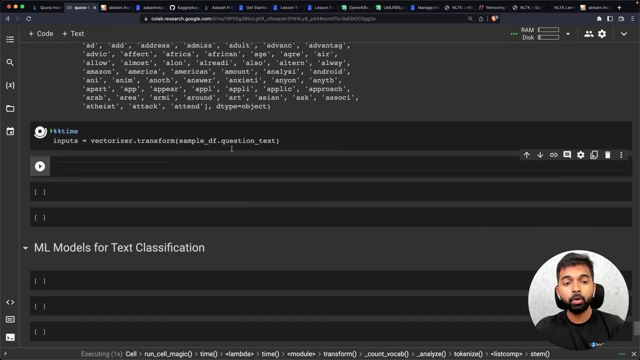 a hundred thousand rules, dot question text And let's also time that. Let's run that. And now that is going to convert all of the hundred thousand questions into vectors. So in about 30 seconds all the hundred thousand questions will have been converted into vectors. 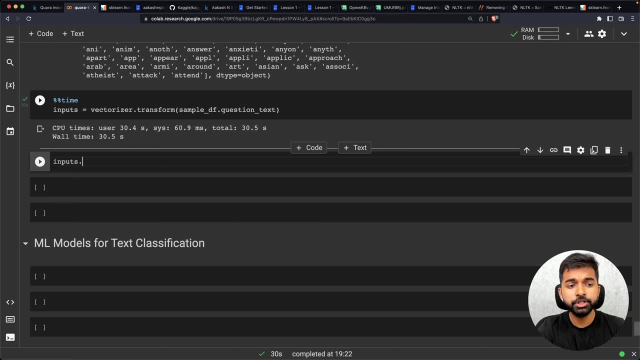 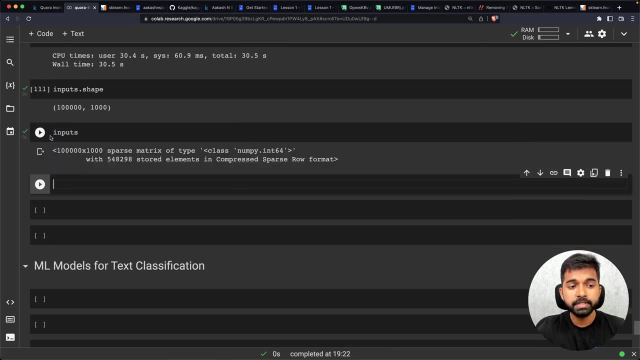 You can see here. it took about 30 seconds. Once again, we can check inputs dot shape. Remember this is going to be a sparse array, So that's why you won't be able to directly print it out. You can see that this is a sparse matrix. 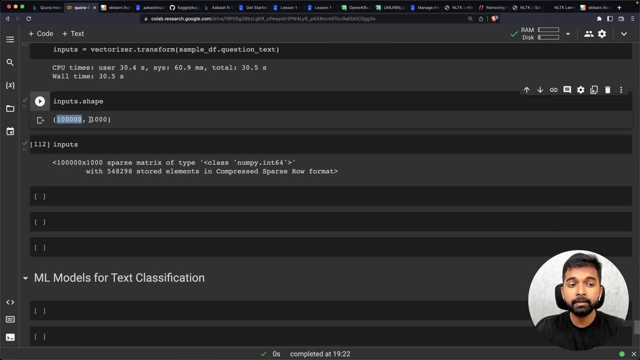 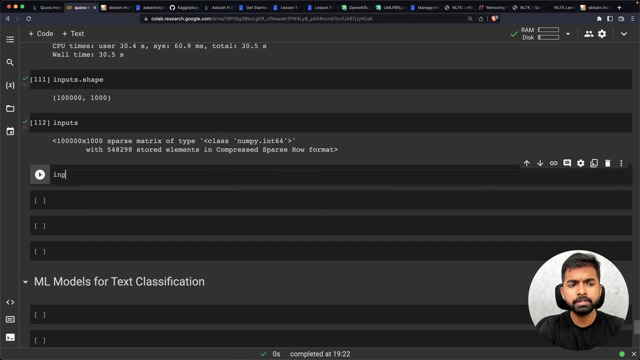 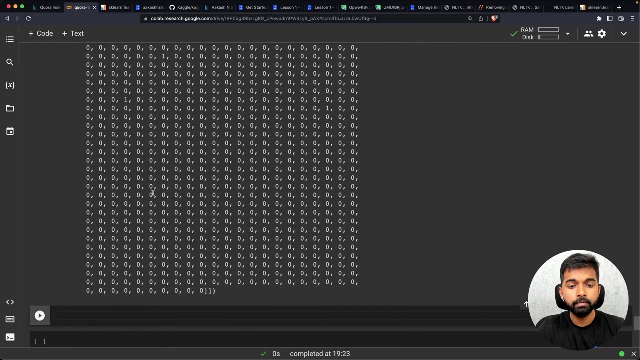 And it contains a hundred thousand entries, Or a hundred thousand rows and a thousand columns, which is basically the vocabulary of size thousand. You can look at the first one. So let's say: inputs zero, Input zero, dot two, array. So this is the very first question. 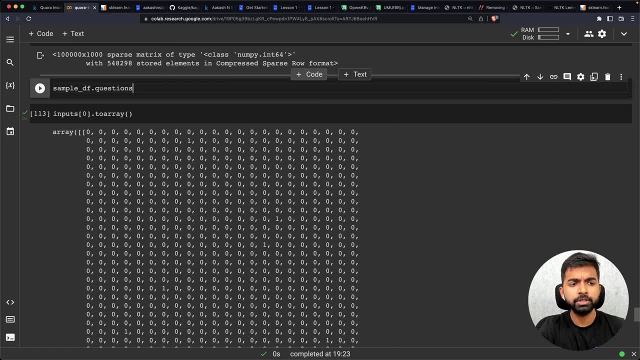 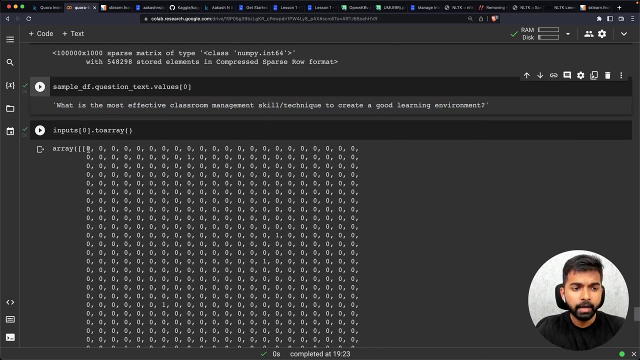 And let's check that question also. Sample DF dot question text: Input zero dot values: zero. So this is the question: What is the most effective classroom management skill? And there are a bunch of zeros, but there seems to be a one somewhere here. 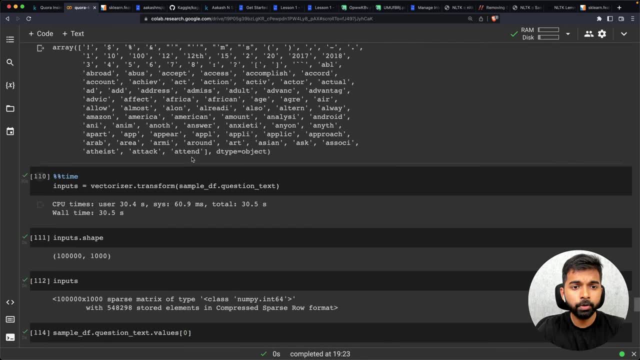 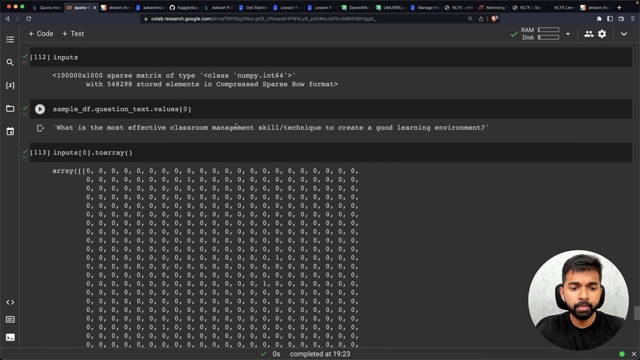 Now this one, I would imagine, might correspond to the question mark, as I can see here. So yeah, it looks like this one corresponds to the question mark And if you keep going you'll find another one. So this is the question mark. 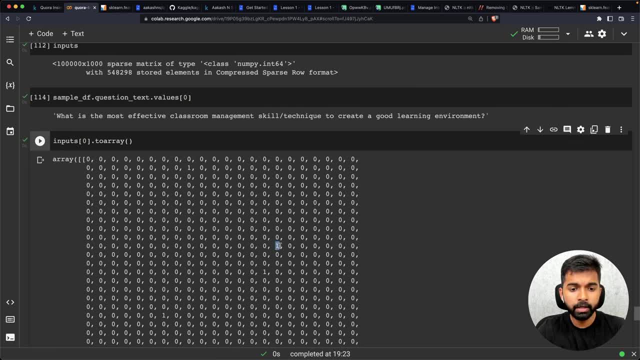 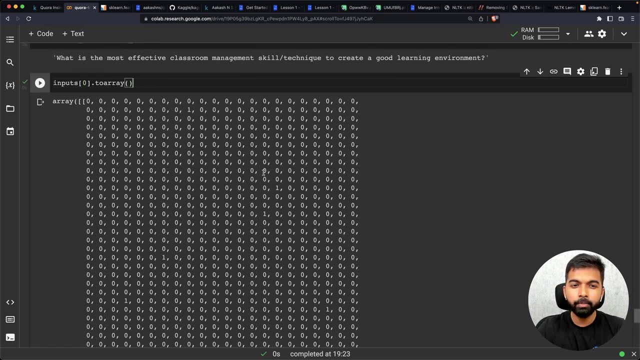 There's another one somewhere, maybe here, And this one, I would imagine, might correspond to classroom. So if you keep going, you might find the word classroom. So these vectors are very hard to interpret directly because you are going to find lots of zeros. 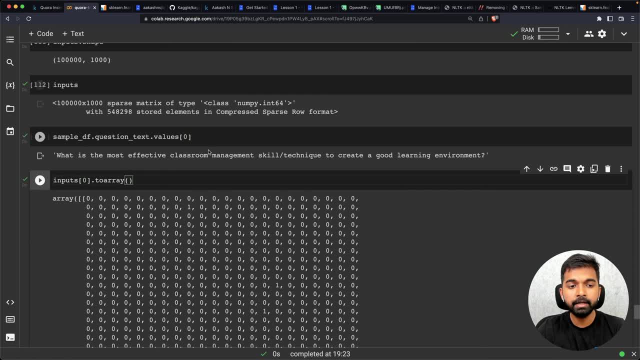 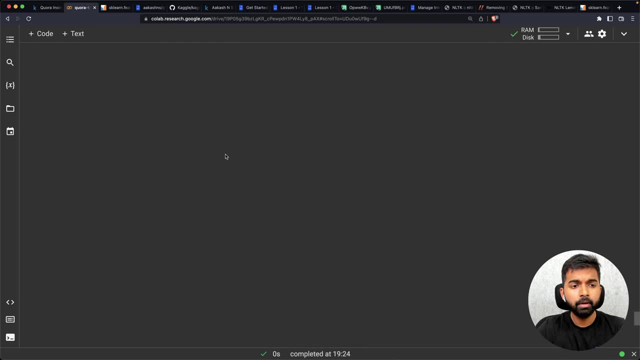 But if you look at the ones and twos and then look them up in the vocabulary, you'll find that they correspond to the words that occur within the question. Okay, So I'm going to remove this, But at this point we have now converted the text that we had. 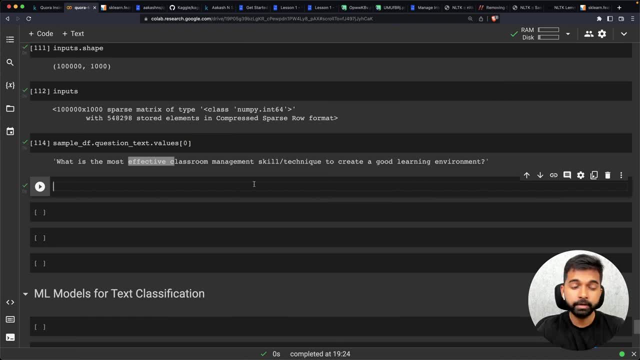 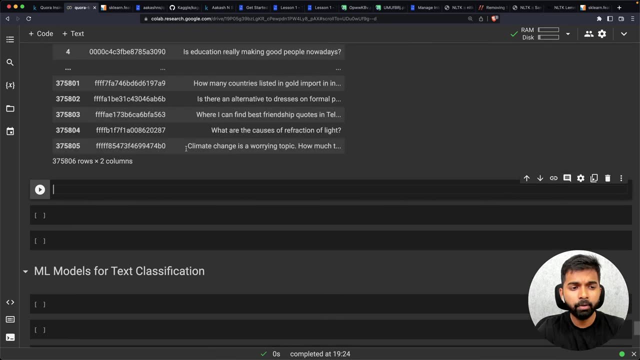 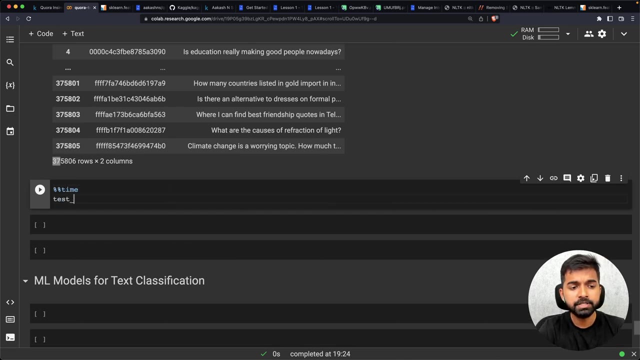 Into a bunch of vectors. Let's also do this for the test data frame. So we have the test data frame. The test data frame contains about 375,000 rows, So we can also go time and test inputs. equals vectorizer, dot, transform, test DF, not question. 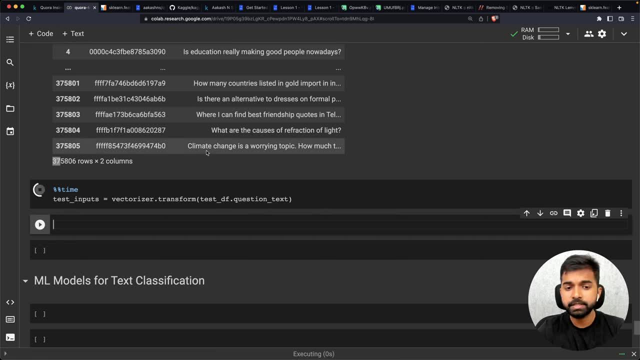 text: Okay. Okay, So we have the test test inputs. Now notice that we did not fit the vectorizer on the test set. This is a very important thing to keep in mind, because when the vectorizer has learned the vocabulary from the training set, it is then going to create vectors for the training. 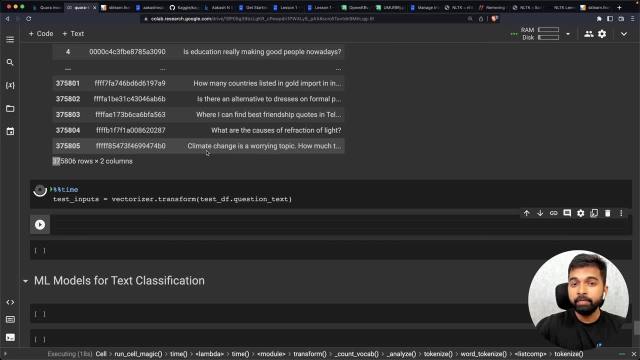 data using that vocabulary. So when we get some new data, either in the real world or when we are testing it on this test data, on this test data set, if we re-learn the vocabulary, the order of words might change or a different set of words might come in. 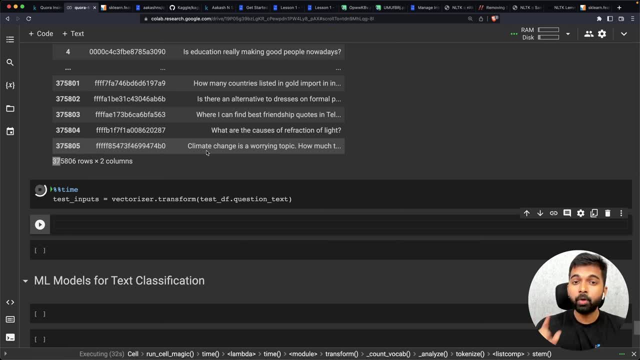 So the new vectors may not make any sense. That is why the vocabulary should be learned only once on the training set. but the transformation can be done separately on the test set And if you have a validation set you can do that on the validation set using the same. 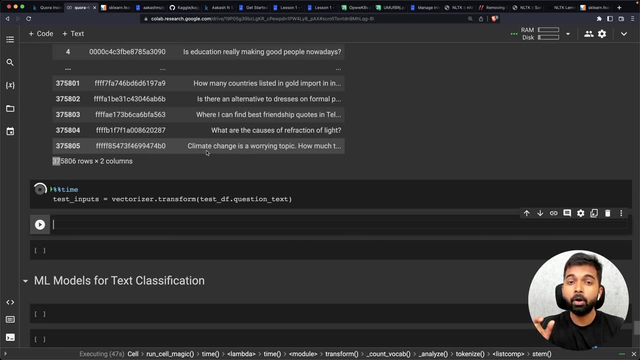 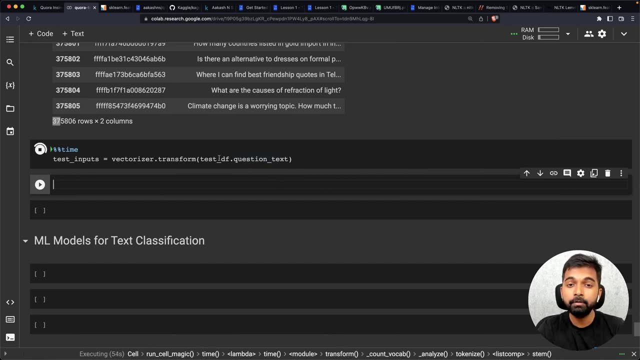 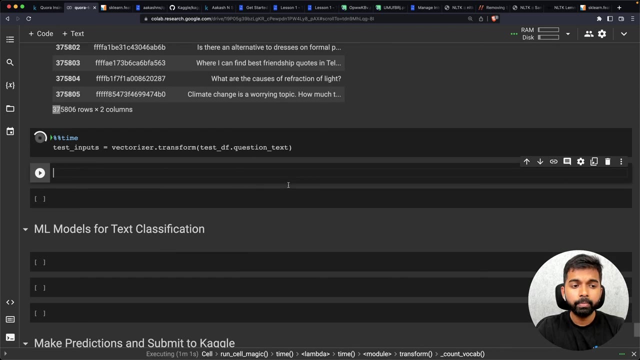 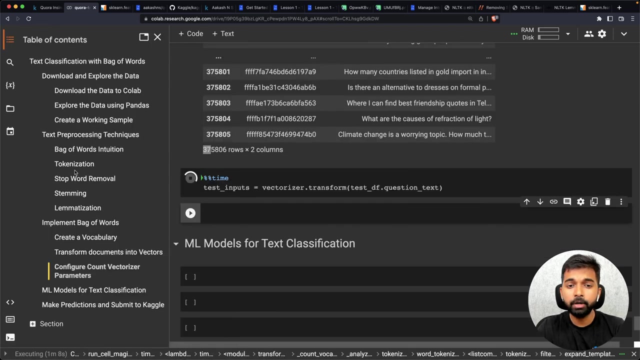 vectorizer that has been trained to learn the vocabulary on the training set. Okay. So keep that important distinction in mind. If you are training a vocabulary using the test set, you are going to get completely meaningless results, Okay. So once the test inputs are completed, we will be done with the second part, or the third. 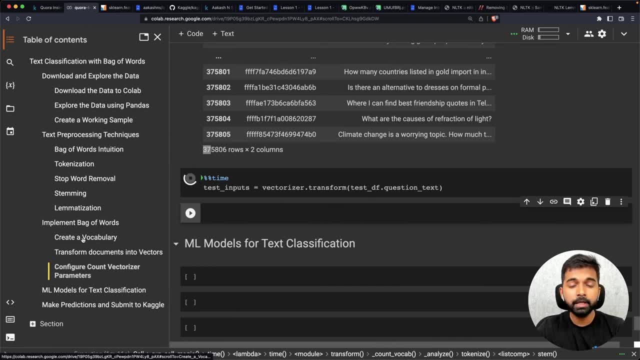 section which was implementing the bag of words model. So here we created a vocabulary using count vectorizer. Then we transformed those documents into vectors by using count vectorizer, dot transform, And finally we configured the parameters of count vectorizer to perform tokenization. 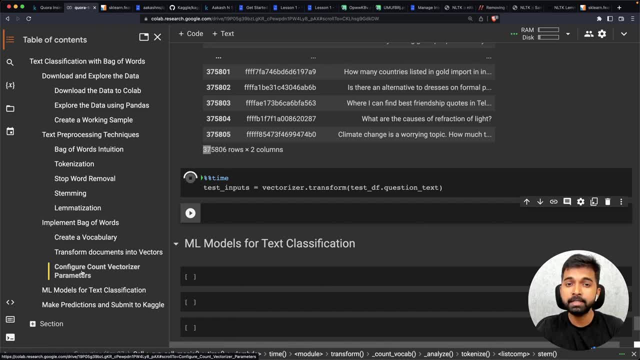 stop word removal, stemming and limiting the vocabulary vocabulary size As per Our convenience. Now you can play with all these parameters. You can check out some of the other parameters as well. The more you experiment, the more you will understand. 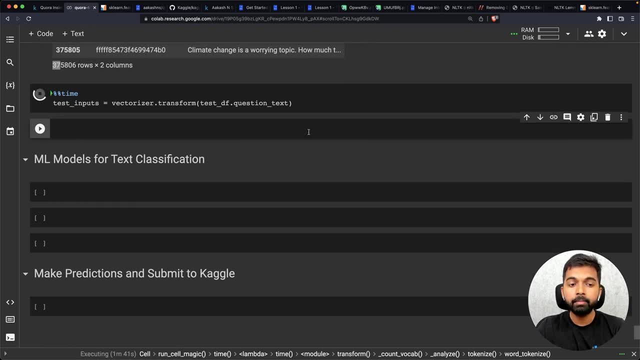 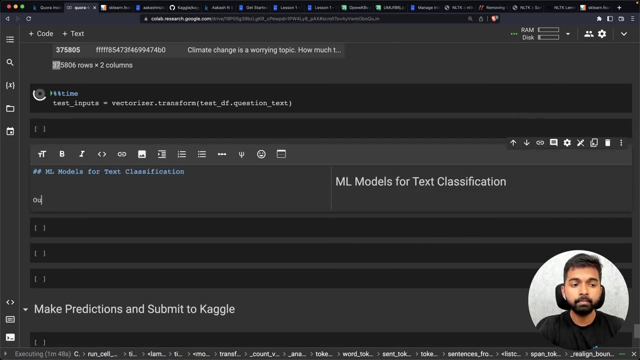 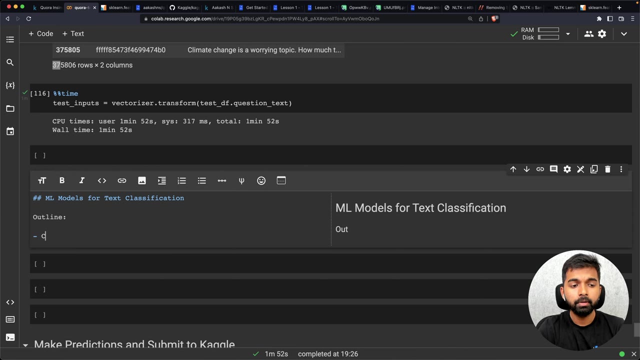 All right. So now we are finally ready to train a machine learning model for text classification. So here's what we're going to do in the machine learning part of this session. So first we are going to create a training and validation model. So here's what we're going to do in the machine learning part of this session. 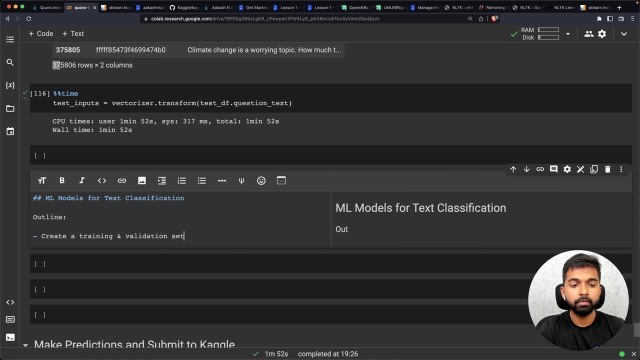 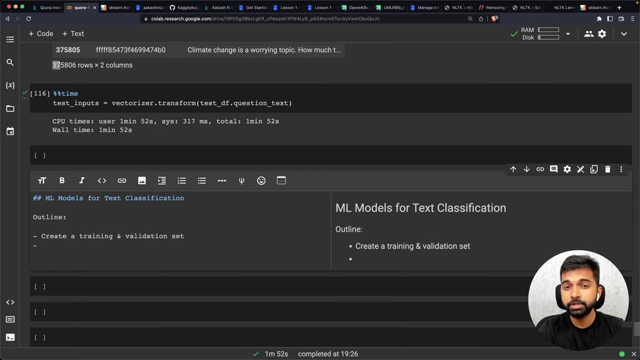 So first we are going to create a training and validation model. So we are going to create a training and validation set. Now, this is more part of machine learning And we have a course on machine learning that you should check out: machine learning with Python: zero to GBMs. 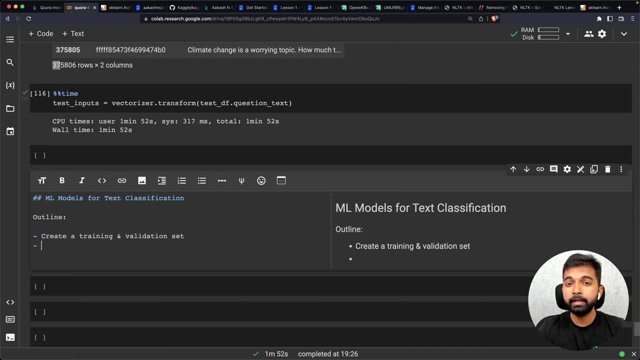 But anytime you're training a machine learning model, you should split the data that you have- the training data- into a training set and a validation set. You should train your models on the training set, but you should evaluate them on the validation set. 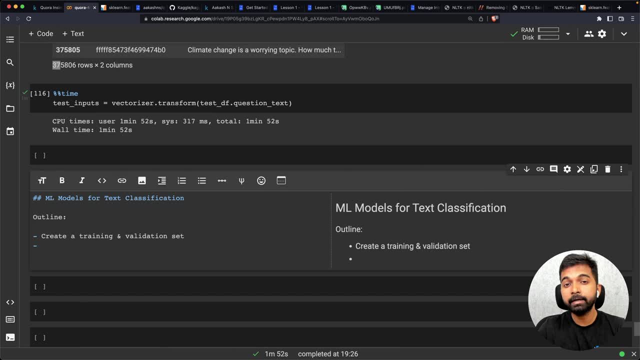 This is because, in the real world, your model is going to see data that it has not already been trained on. So that is why you should evaluate your model using data that it has not been trained on. So we are going to train it. 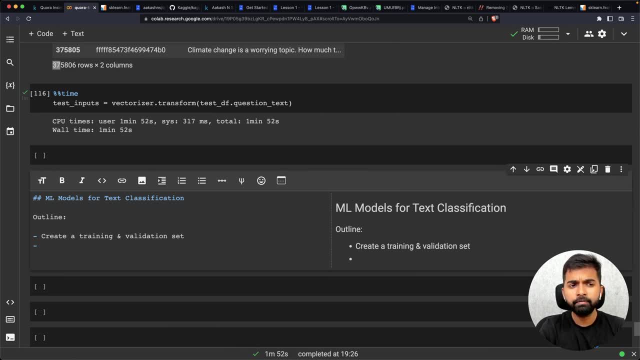 We're going to create a training and validation set from the data that we have, the inputs. Then we are going to train a logistic regression model. Again. also, this is something that is slightly outside the scope of this particular course, but we are trying to perform text classification in supervised learning because we have labels. 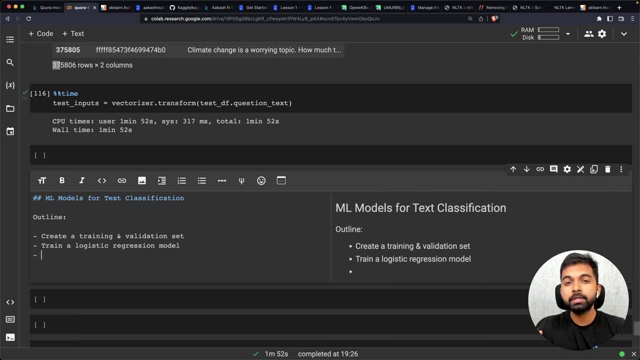 in the training data. Now, logistic regression is the most simple text classification machine learning algorithm, and you can check out our machine learning course to learn more about it. So we train a logistic regression model And then, finally, we are going to make predictions on training, validation and test data. 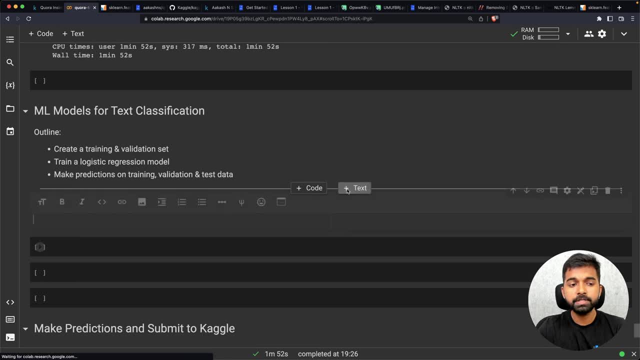 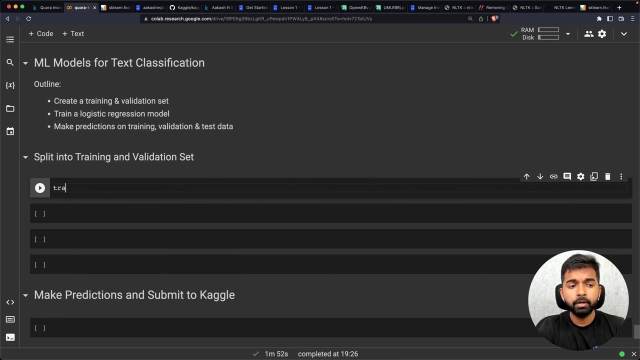 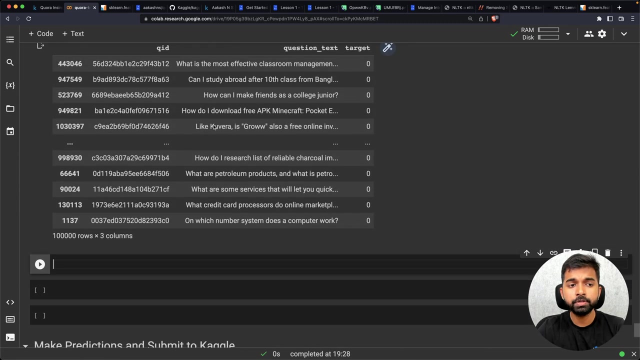 Okay, so let's get started. The first step is to create a training and validation set. All right well, if you look at the sample DF here, it contains 100,000 rows of data And it contains questions and it contains targets. 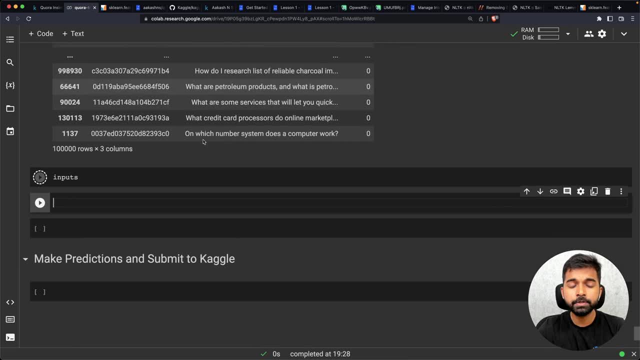 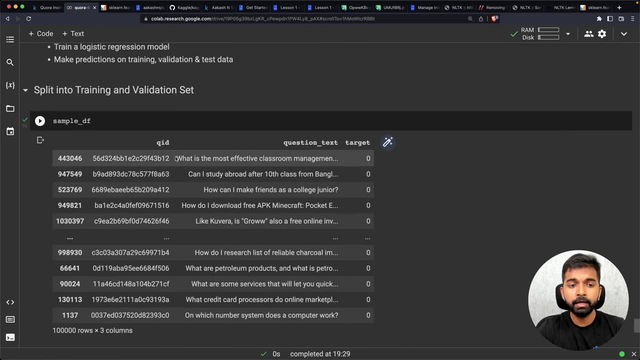 Now the questions have been converted into numbers Already, And that is something that we have stored into inputs. Remember, inputs contains: for each question, it contains a vector of size 1000.. So, because the vocabulary is of size 1000, it contains a vector of size 1000. 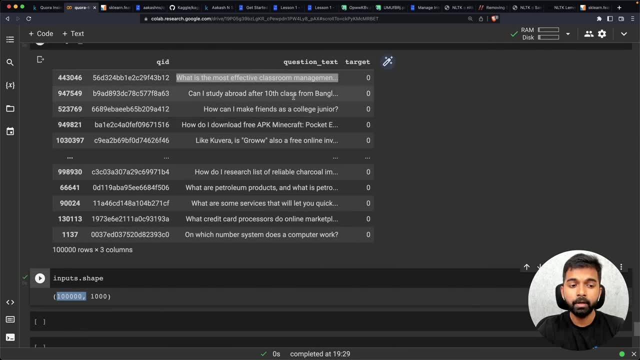 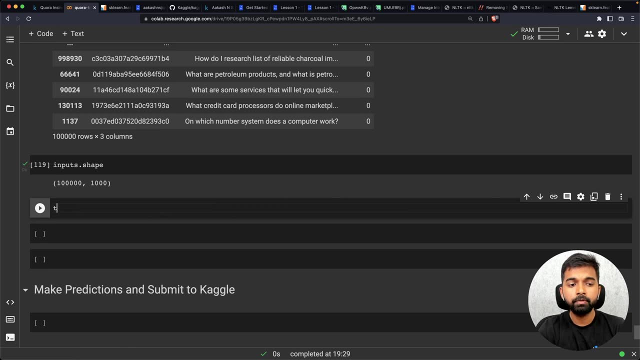 And there are 100,000 such vectors, one for each question, And they're in the same order that we have in the question text. So here's what we need. we need a bunch of rain inputs, a bunch of inputs that will be. 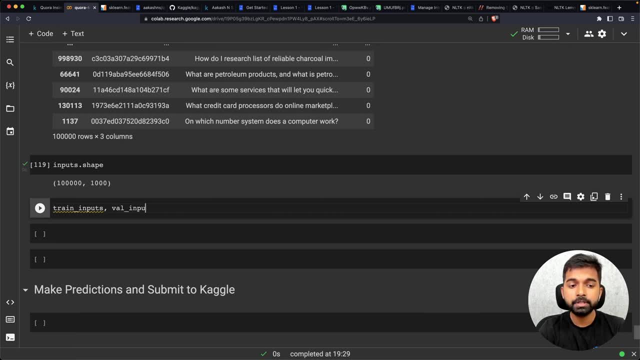 used for training. We need a one bunch of val inputs, a bunch of inputs that will be used for validation. We need a bunch of trained targets, Because when you're training a machine learning model, you also need to provide the targets. it's not enough to just provide the inputs. 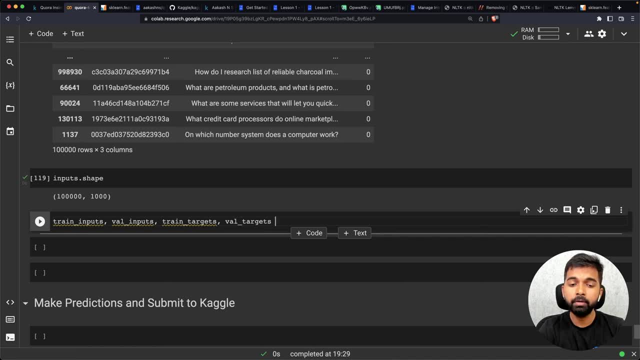 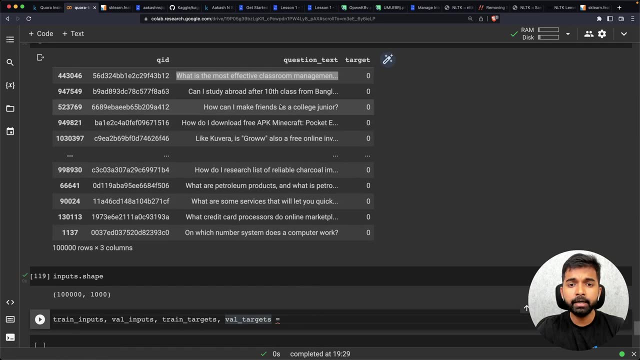 And we need a bunch of validation targets, Because when we are evaluating the model, we are going to compare the predictions of the model with the targets that we have, And the way this is typically done is we take the entire data set and we pick a random. 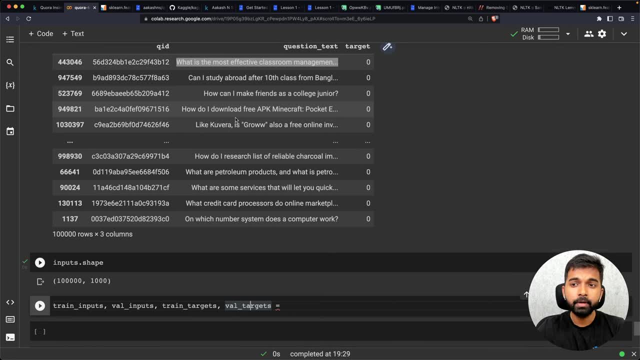 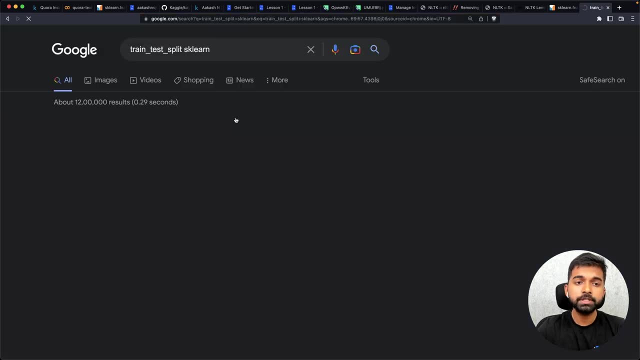 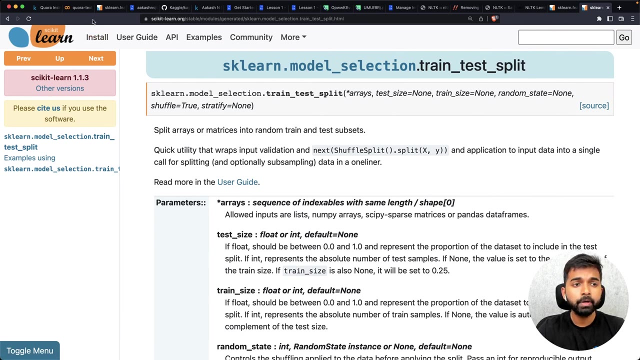 sample of the data set: Okay, And we add as a validation set. So this is done in SQL. on using the train test split function. So if you just search for train test split, you'll find that scikit-learn provides this model selection: train test split module. 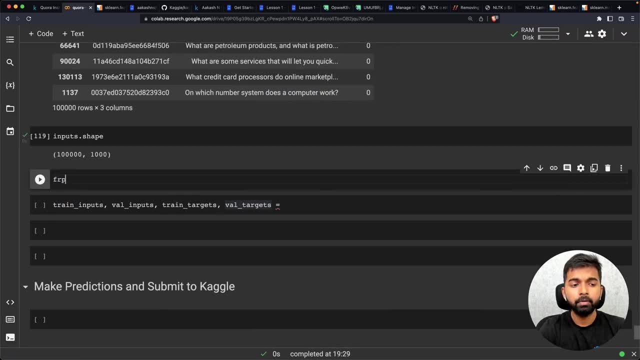 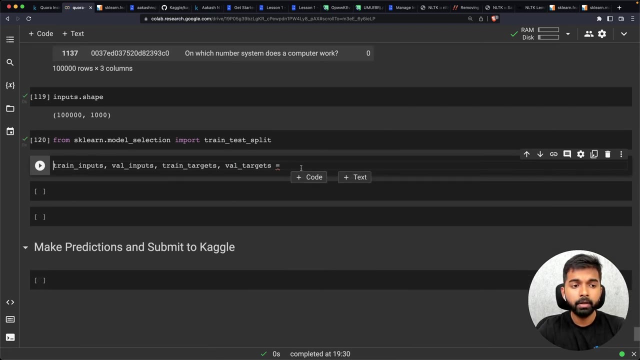 So I'm going to import from SQL on import Train test split And we need to give it- first, we need to give it the set of inputs that we want. So the inputs are going to be simply inputs. Then we are going to, then we need to give it a set of targets that we have the targets. 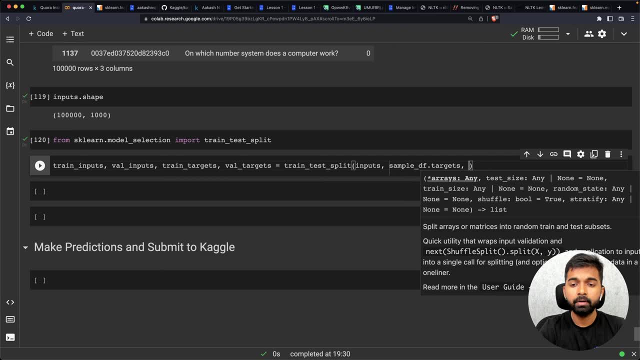 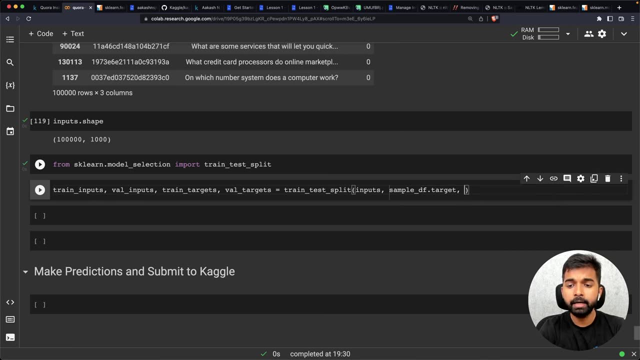 are simply sample DF dot targets. Yeah, sample DF dot targets contains all that own dot target contains all the targets. And then we need to provide, Okay, Test size, which is the validation set in this case, which is called test size. but 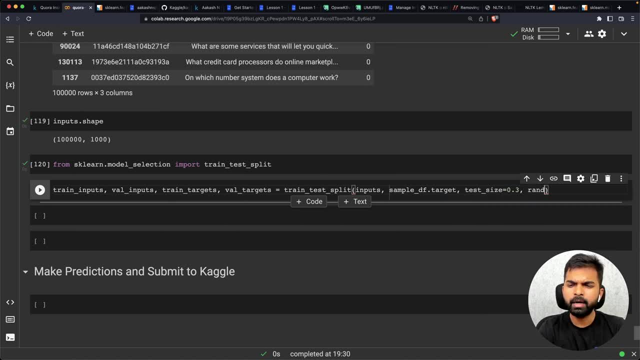 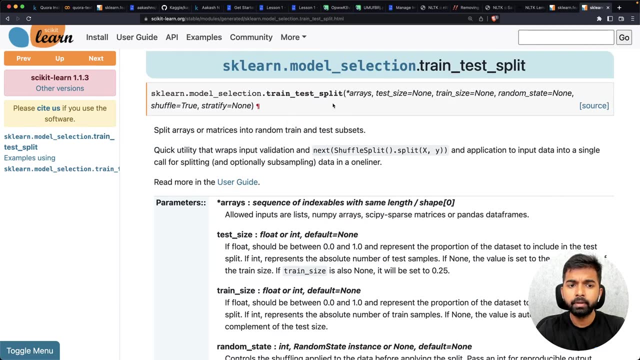 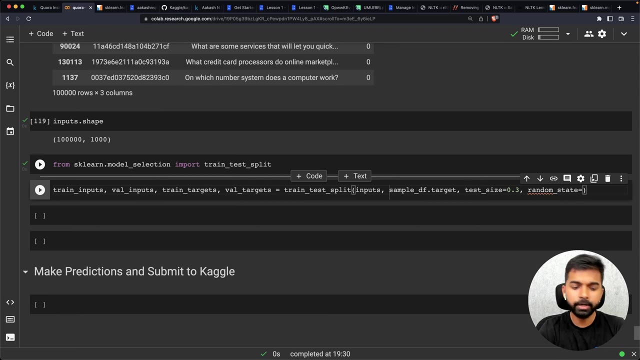 the test size is point three. And finally, we can also provide a random state. I believe Let's see here. Yeah, so we can provide a random state if you want, in case we want to make sure that every time we run this notebook we get the same split. 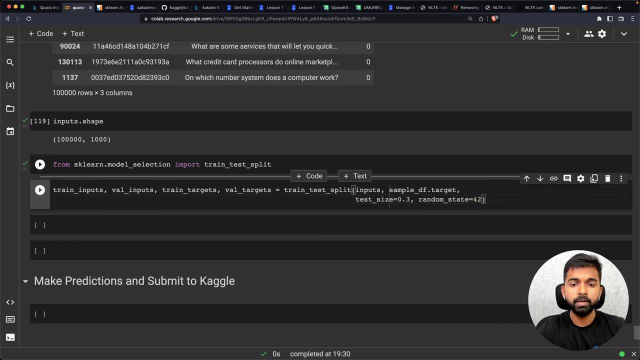 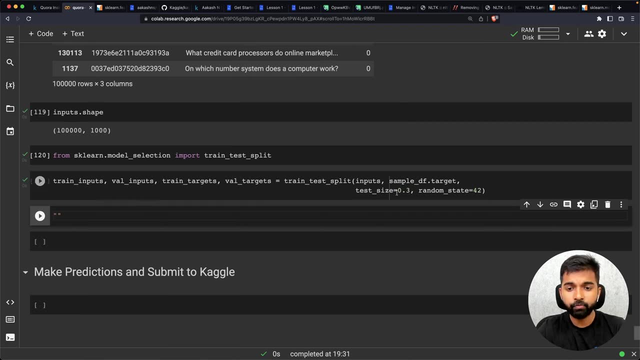 So I'm going to pass a random state of 42.. Okay, So now This is going to take all the training inputs and all the training targets which are provided by sample DF dot target, And it's going to identify a certain percentage of inputs and matching targets to be used. 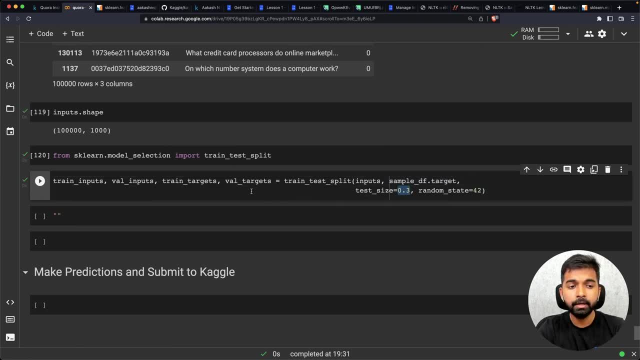 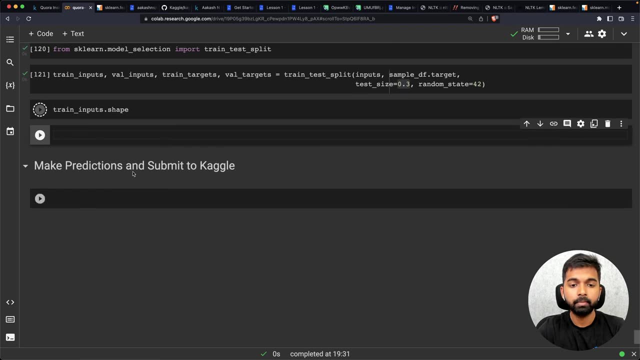 in the validation set, which is 0.3 or 30%, And the remaining 70% is going to form the training set. So now, if you check train inputs dot shape, you'll see now that train inputs dot shape is 70,000.. 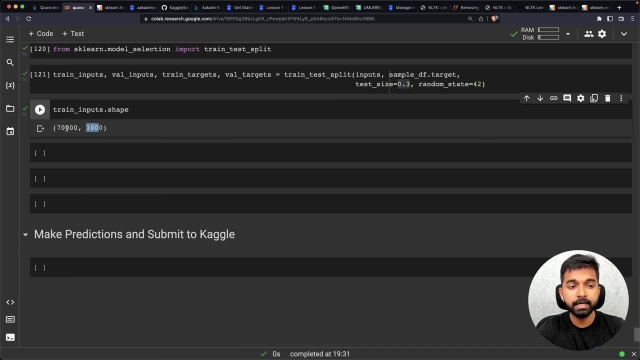 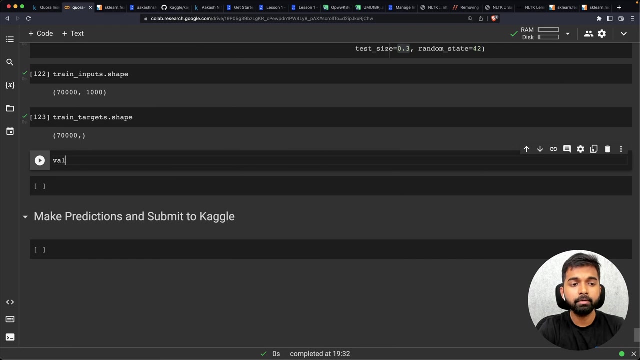 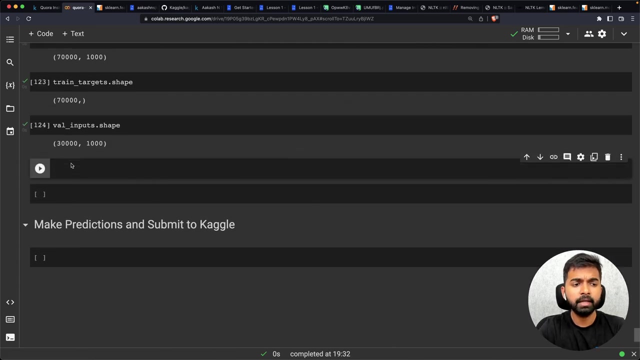 So we have 70,000 questions that have gone into. Okay, The training set 70,000 bag of word vectors and train targets. dot shape: That is simply a list of the corresponding 70,000 targets from sample data frame. Similarly, you can check while inputs or shape: that is 30,000.. 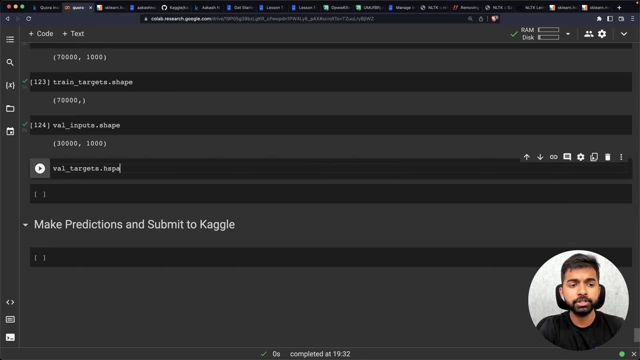 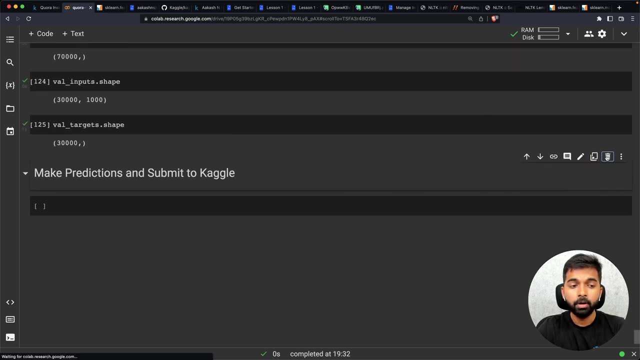 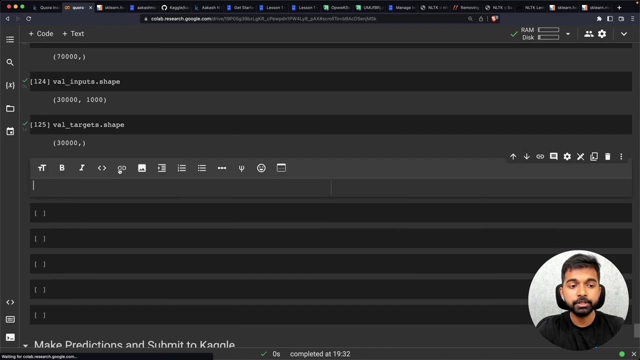 And then we have: well, targets, not shape. These are the corresponding 30,000 targets. Okay, From our data frame. All right, So now we have done the first step, which is creating a training and validation set. Now let's go on to the second step, which is brain logistic regression model. 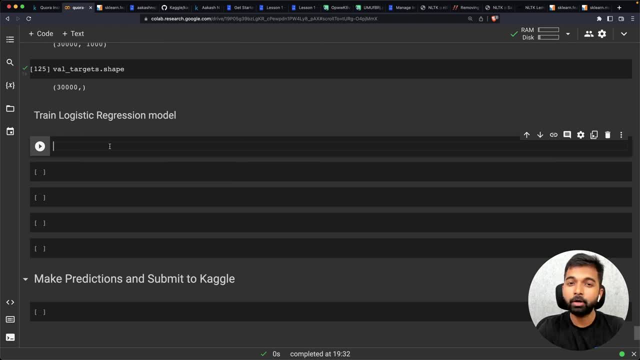 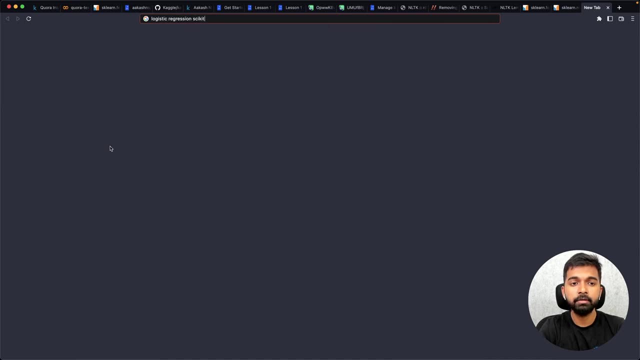 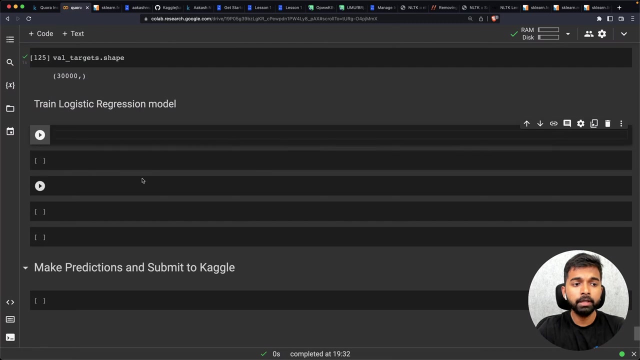 Now we are going to train a very basic model here. We're not going to do any hyper parameter optimization here. So let's search for logistic regression psychic learn. Okay, And this is part of the sklearnlinear model class. So I'm going to go in here and say: from sklearnlinear model import logistic regression rate. 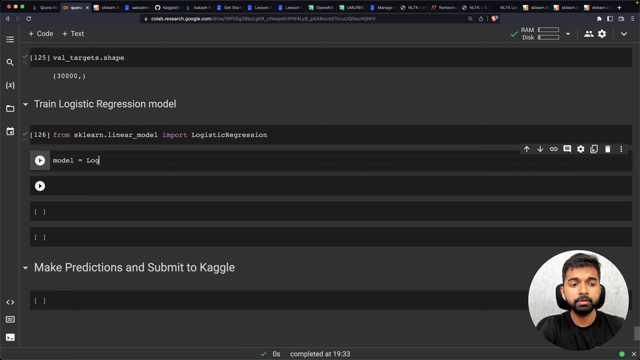 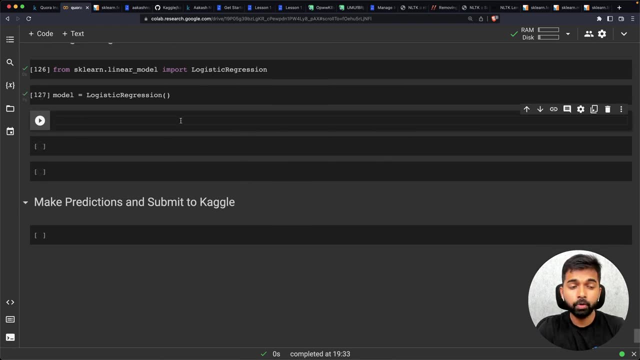 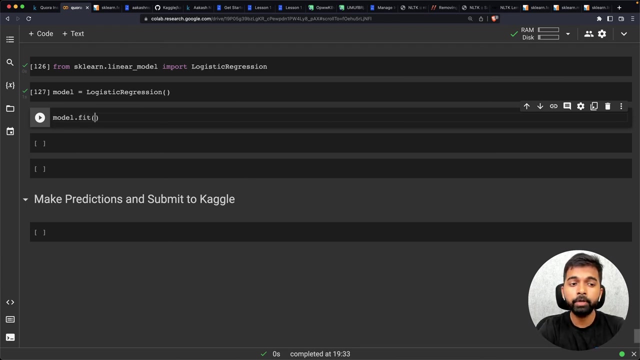 And now let's create a model. So model equals logistic regression. Again, check out our machine learning course on how logistic regression works to learn how logistic regression works And how to use it. And now let us fit the model, which means we are going to give the model the set of. 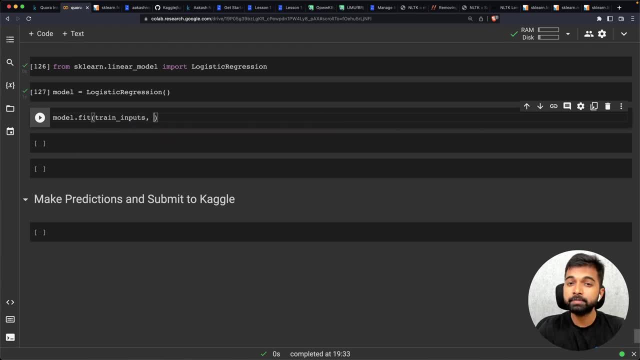 training inputs, which is all the bag of word vectors for the 70,000 samples that we have picked for our training set And we're going to give it the set of targets. the training targets and the model is internally going to first start with some random parameters. 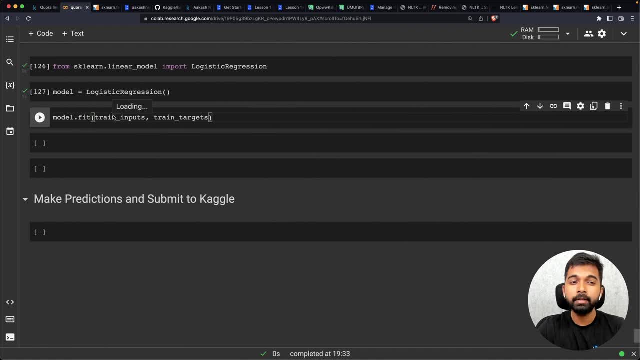 It's going to try to make some predictions on these training inputs, that is going to compare those predictions with the targets- Okay- And it is going to adjust its internal parameters using an optimization algorithm to make sure that the predictions become closer to the targets. 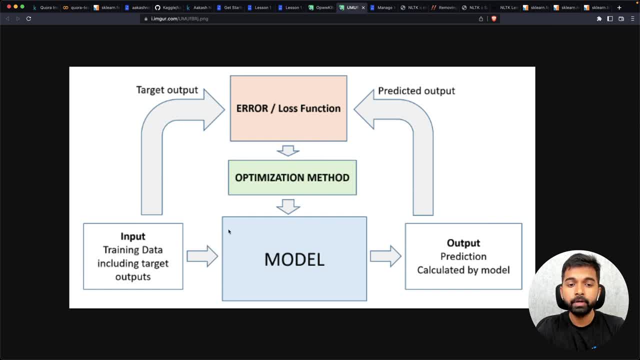 So all of this is part of the machine learning workflow. Here is how machine learning works. You give some input. the input contains some training data and including target outputs. The training data is fed into the model directly And then the target output is then fed into the predictions from the model. 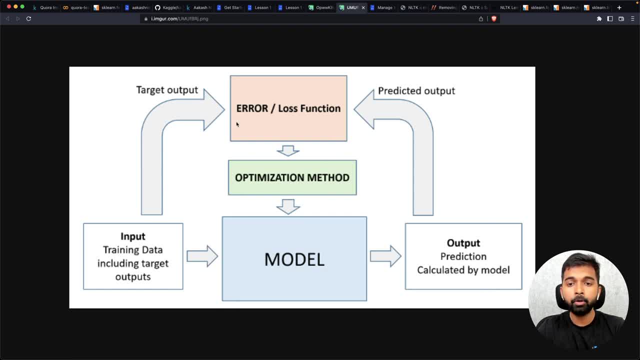 So the model comes up with some predictions. So the target output and the predicted output are compared Using something called a loss function, And then using the loss function, and optimization algorithm is used, And that optimization algorithm then improves the internal parameters of the model. 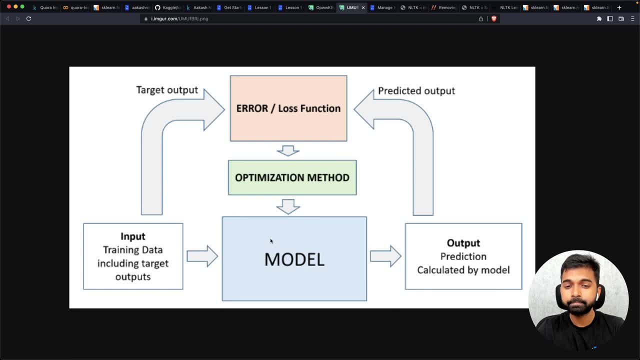 So that now the model makes better predictions on the training data. This optimization algorithm is typically something called stochastic gradient descent, And all of that ultimately means that the model iteratively gets better and better by looking at the training data, Improving its outputs with the targets and then improving its internal parameters to 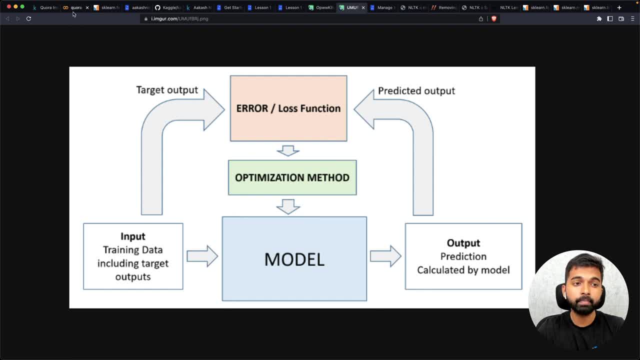 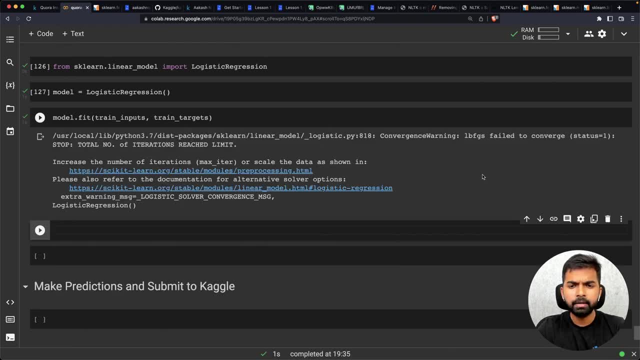 make better predictions that are closer to the outputs. Okay, So let's do that. Let's call model dot fit train inputs, and that's going to take some time, but looks like there is some error here. Lgb, L, B, F, G, S fail to converge. total number of iteration limit reach. 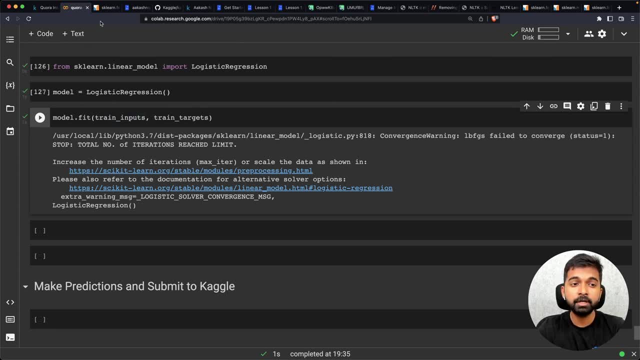 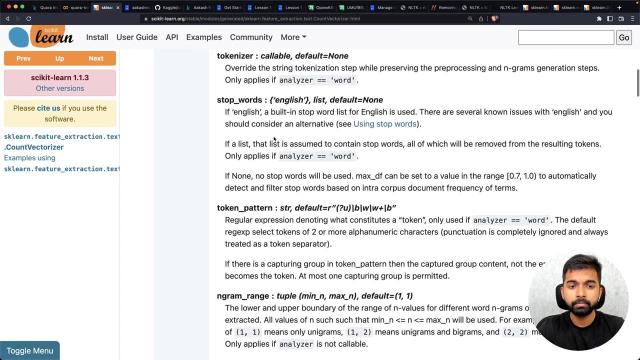 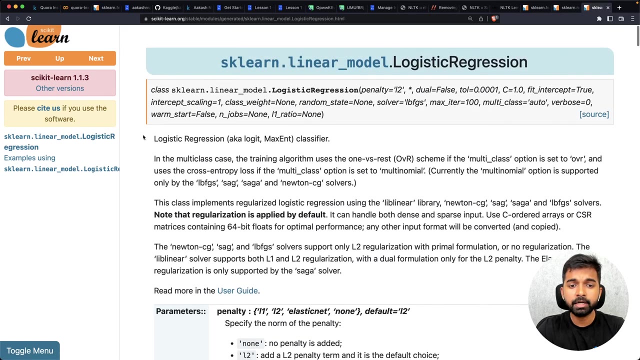 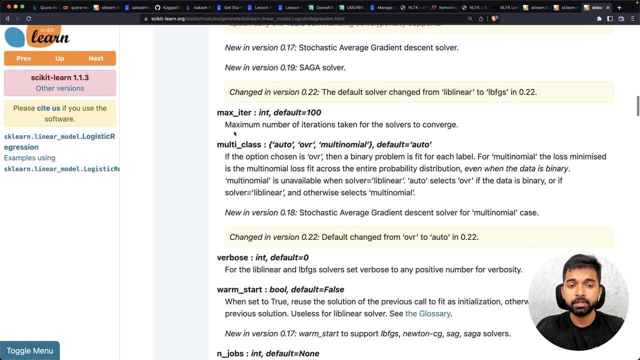 Okay, So this can happen when you're using logistic regression or linear regression. If you check, it has something called a max iteration. Okay, So if you check, logistic regression is something called max iterations configured somewhere, which is how many times it is going to go through this process of optimization. 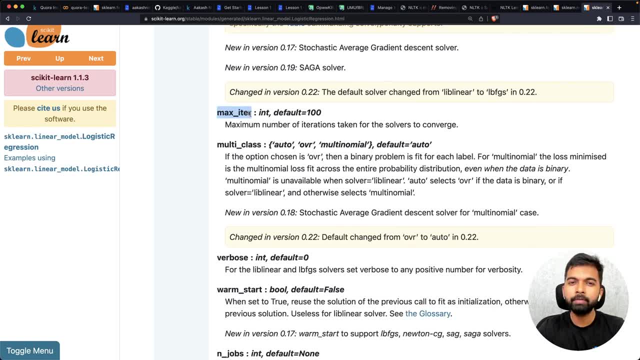 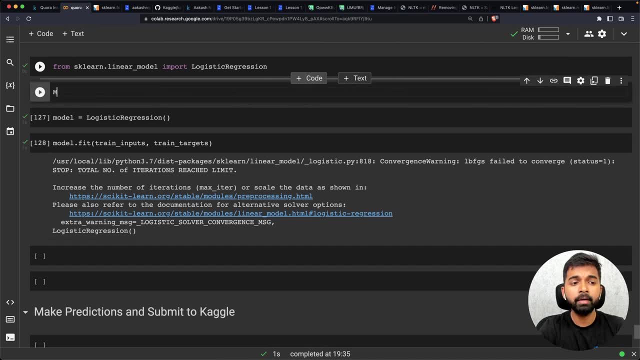 And, by default, the max iteration is set to a hundred, which is a very small number when you're doing, when we're dealing with a dataset containing hundreds of thousands of rows. So once again, I may want to use a bigger max iterations. 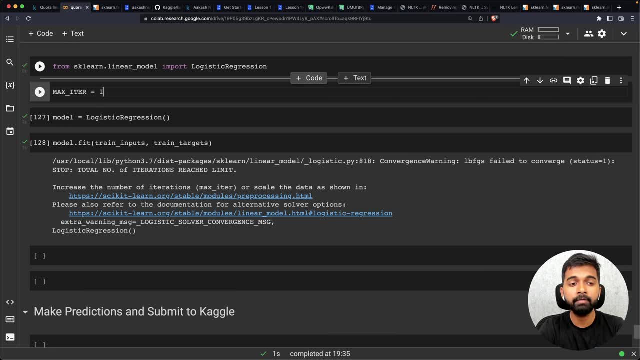 And I'm going to put this in a function, in a variable, so that I can modify it later when I need. I'm going to use thousand iterations right now And let's just say max iter. max iter equals thousand. And another thing that you can configure in the logistic regression model is the solver. 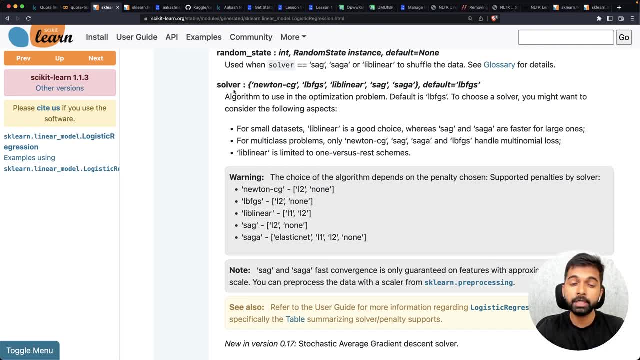 which it is using, or does optimization algorithm which it is using to improve the internal parameters, Okay, And make predictions. So the solver I'm going to use is called SAG, or stochastic gradient descent. It has something else which works better for smaller datasets, but I'm going to use the 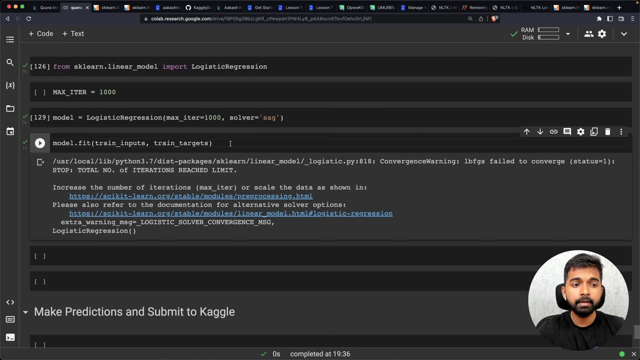 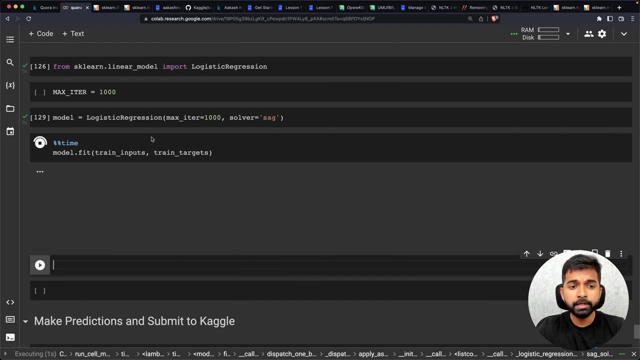 solver, SAG, and let's create that model again and let's fit it again, And I'm also going to time it, Okay. So now what it is doing is it is looking at the input vectors, that the training set vectors. it is then going to make some predictions. 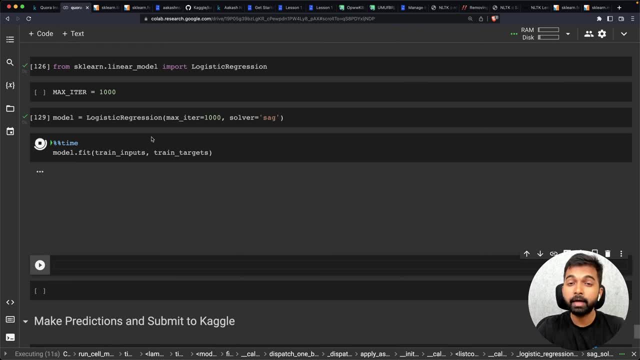 It is going to compare those predictions with the outputs That the targets that have been given here. then it is going to adjust some internal parameters of the model using the stochastic gradient descent or stochastic gradient descent optimization algorithm. Then it's going to make predictions again, compare them with targets again and it's 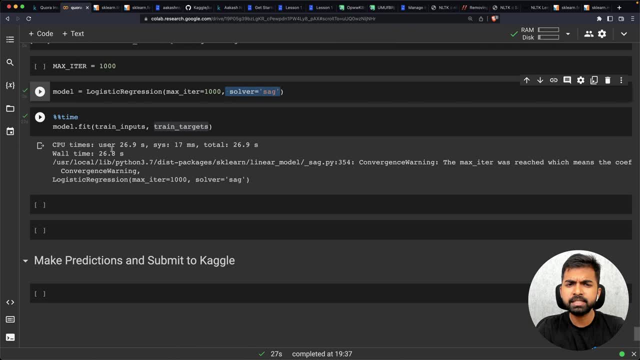 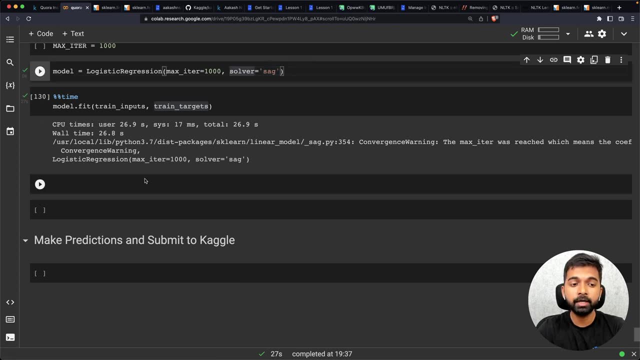 going to repeat this a whole thousand times. That's why it takes about 30 seconds. but now the model has been fitted. Now the model has some understanding of how to make predictions on the data and the way we can verify This. So now we're making predictions. 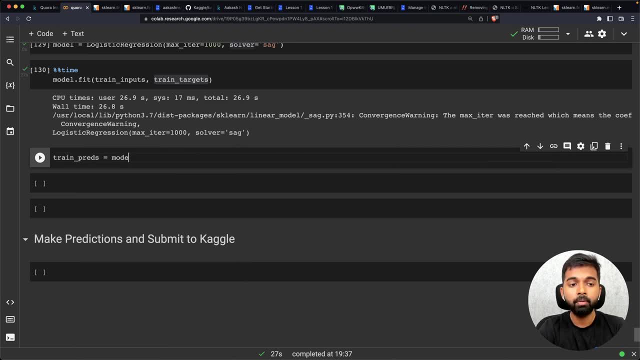 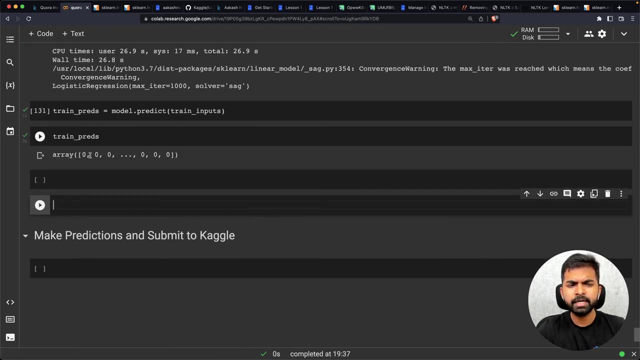 So now we can say: train preds equals model dot predict train inputs. So now, if we give it a set of input bag of word vectors, it can give us a set of predictions. Okay, So let's check train preds and it looks like it's an array containing all zeros. but is 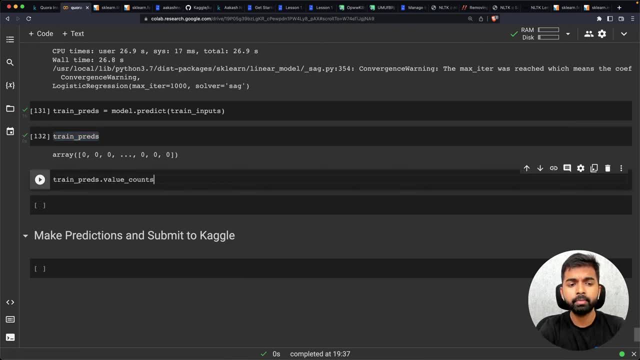 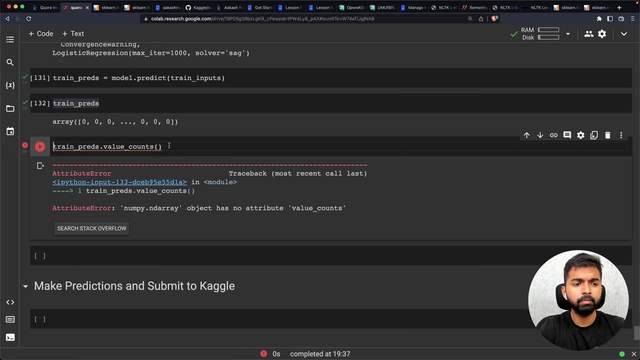 it really all zeros. So let's check train preds dot value counts, Okay, Okay, Okay. So let's convert that into a data frame, into a Panda series, so that I can use value counts. All I'm doing is counting the number of zeros and ones. 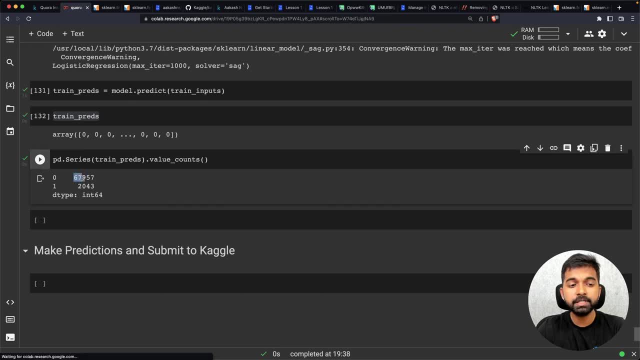 Okay, So it looks like in the train preds. we got about 69,000 or 60 or 68,000. predictions are zero. So this is a prediction obtained from the model. We have given it some inputs and it has come up with some predictions. 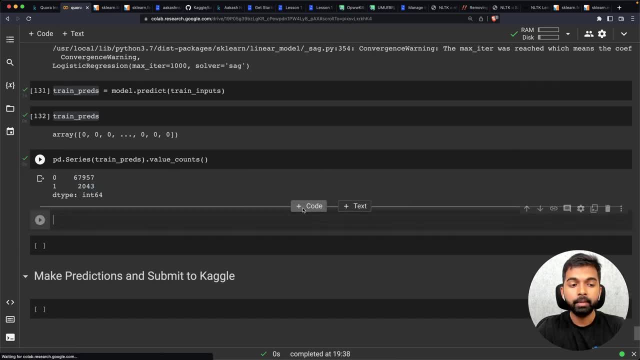 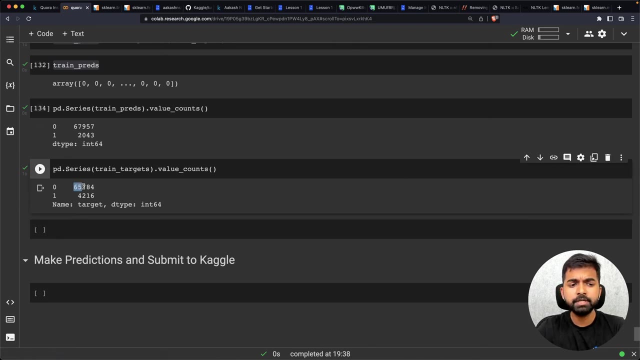 And in 2000 cases it has predicted a one. compared that to the train targets And in this case you can see that in the train targets of there are about 65,000 zeros and 4,000 ones. So obviously the train preds are not the same as train targets, because models are not perfect. 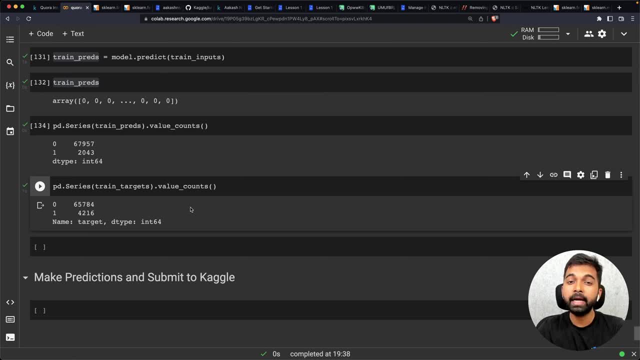 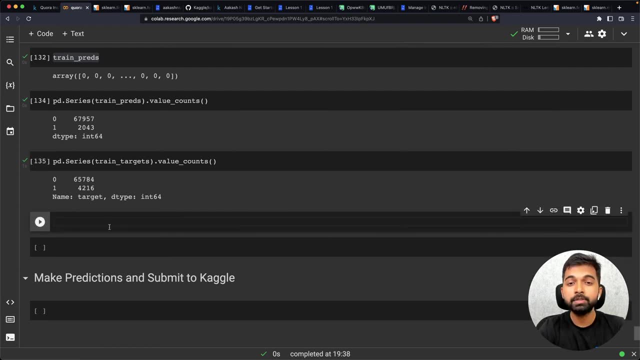 It's just that the more data you give it, the more parameters the model has internally, the better it will get. This is definitely not a perfect model, but how do we understand how good it is? The way we check how good it is is using something called an accuracy score, possibly. 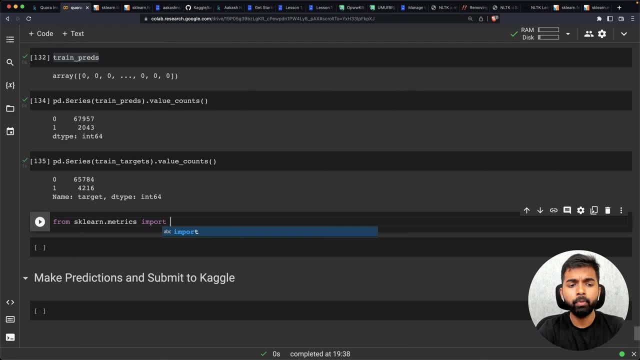 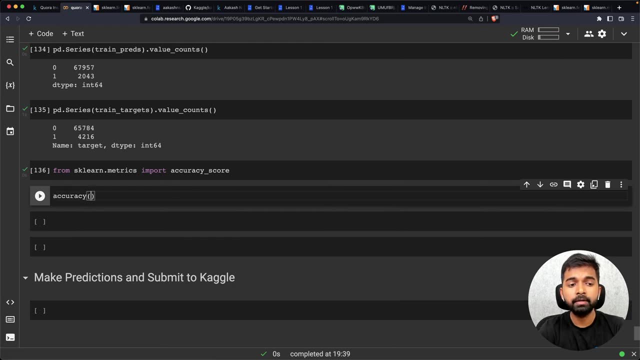 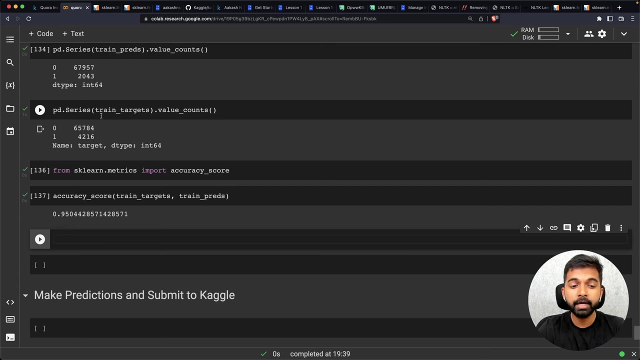 So we can say from sklearnmetrics import accuracy score. Okay, And what's accuracy score going to do? Well, you give it the Train targets, you give it the train preds and then it is going to go through the train targets one by one and it is going to compare the train targets to the train preds. 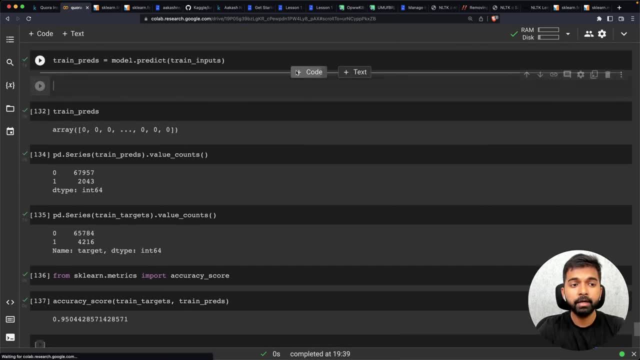 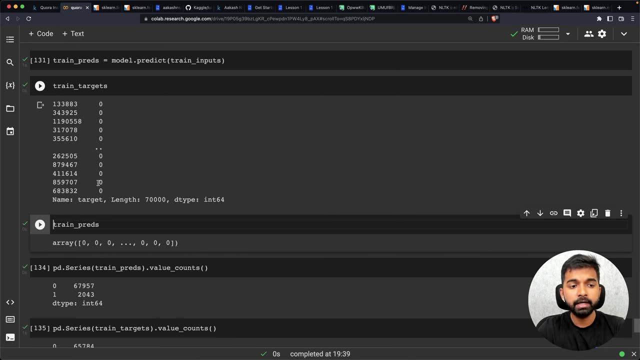 And it's going to search for exact matches. So these are train preds. If I see here train targets, you can see these are train targets and these are train preds. So it's going to compare one by one: zero against zero, zero against zero and one against one. 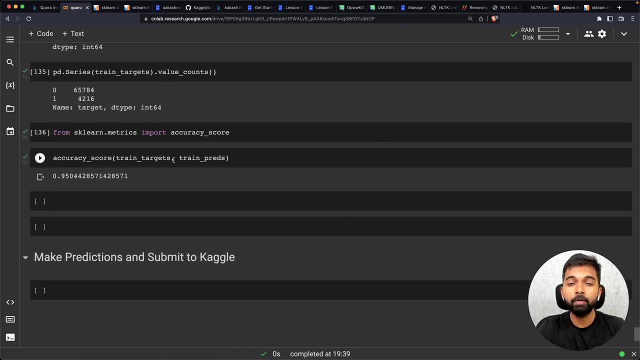 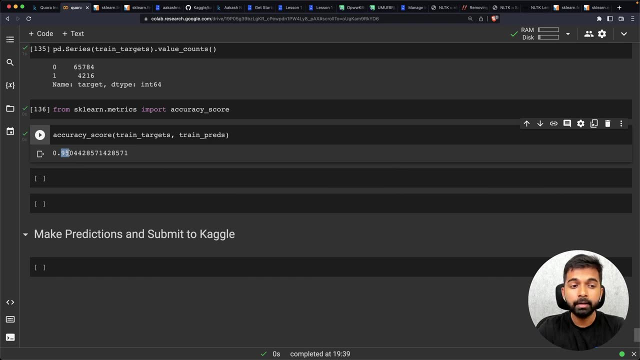 and so on, And then it's going to identify what percentage of these, or what fraction of these, match. So it looks like 95% of the time our model was able to predict the right value. But, as we saw earlier, even if we always just predicted zero, we would still get 94% accuracy. 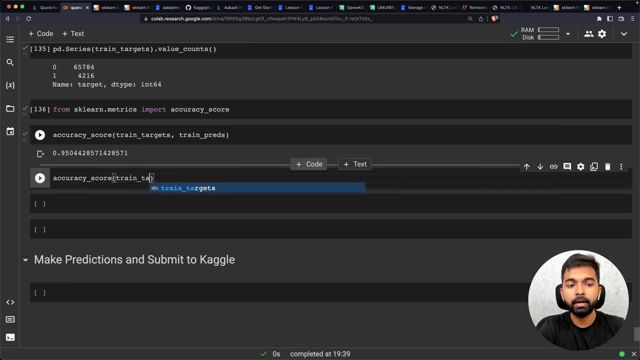 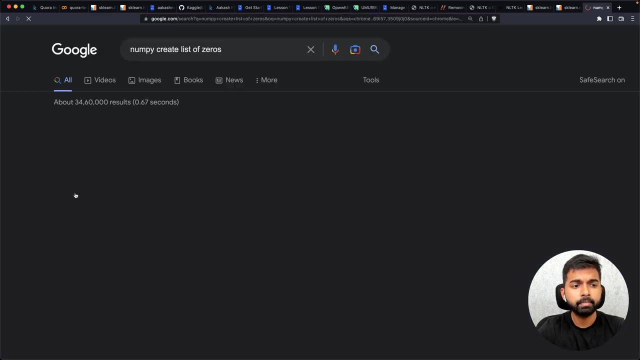 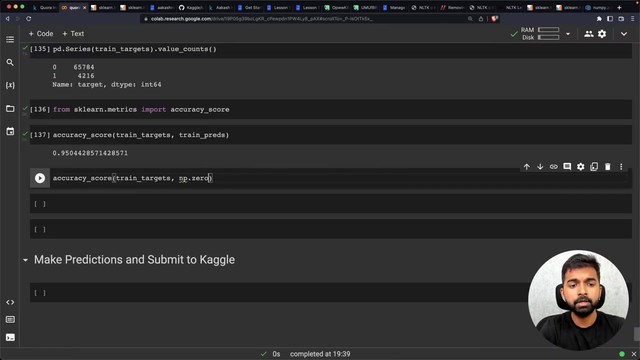 So you can actually check that accuracy score train targets, And we can just say NP dot. Or yeah, let's see NumPy create list of zeros: NP dot zeros. Okay, So I can, if I just do NP dot zeros and I give it the shape Len train targets, let me. 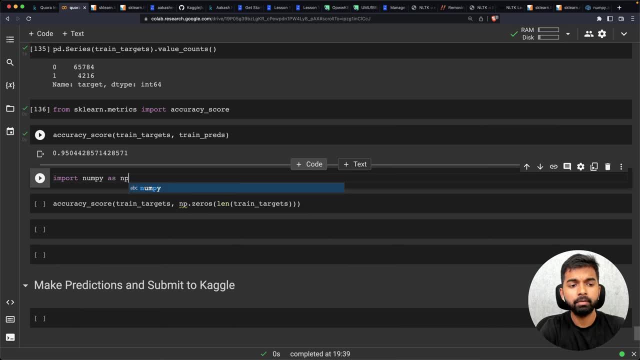 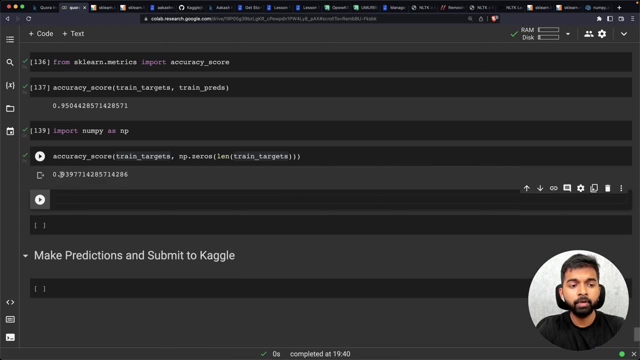 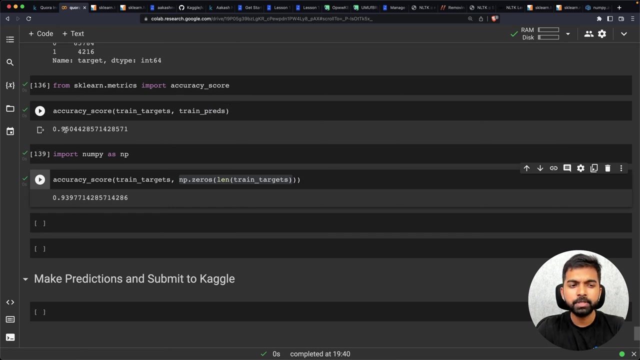 just import NumPy as NP. That would have a 94% accuracy. So just by predicting zeros all the time, you get 94% accuracy, 94,, 93.9%. by predicting by using our machine learning model, which we have trained, we are getting 95% accuracy. 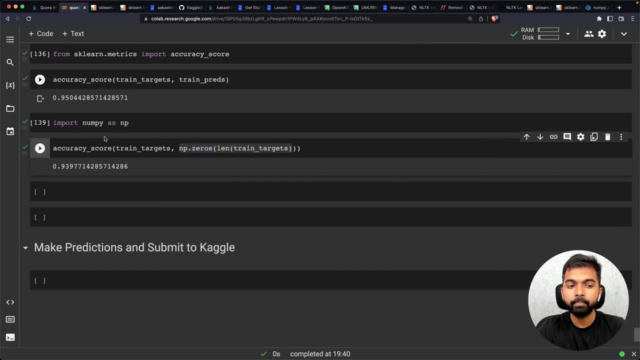 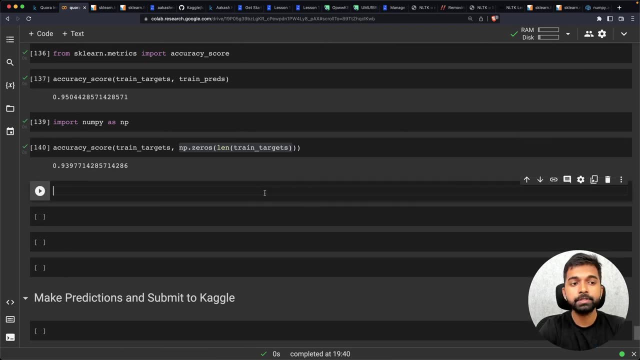 So it's slightly better, but you can't really tell whether it's a great model. The way you can tell whether this model is good or not, Especially when you have imbalanced data sets, It's using something called an F1 score. 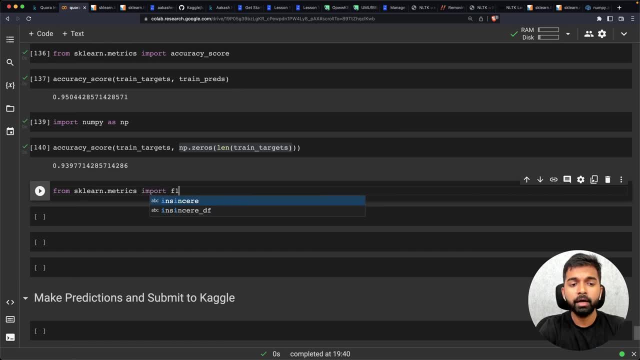 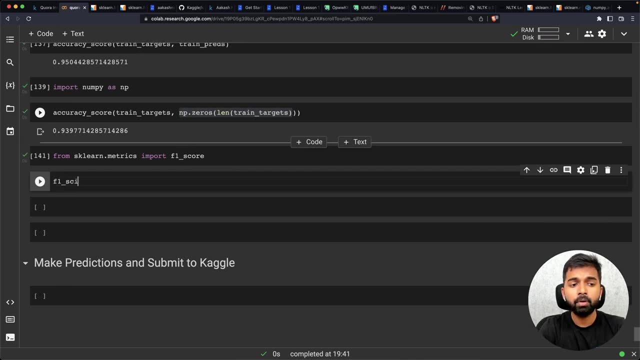 So from sklearnmetrics import F1 score And this is the metric that is also used in the Kaggle competition. And let's check F1 score of train preds or train targets versus train preds. So F1 score of our model on the training side is 0.44.. 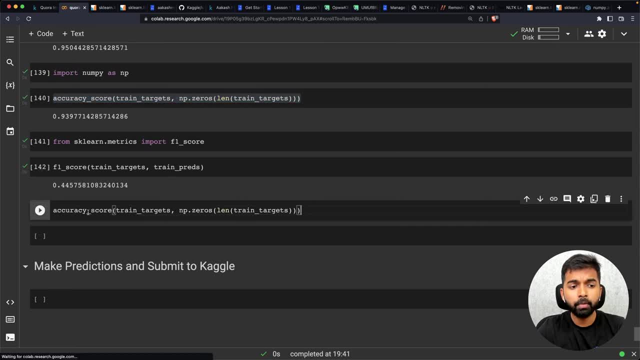 And let's check the F1 score of our model. And let's check the F1 score of our model. And let's check the F1 score of our model. And let's check the F1 score of just random of predictions, where we're always predicting. 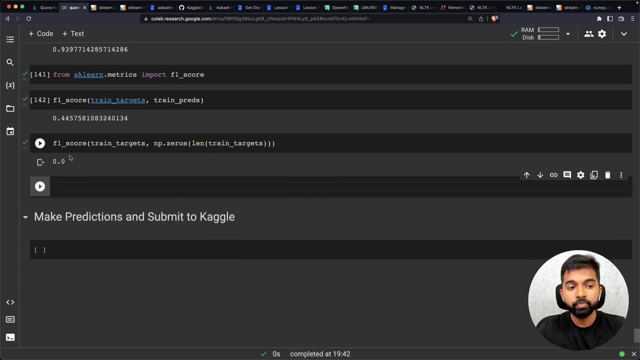 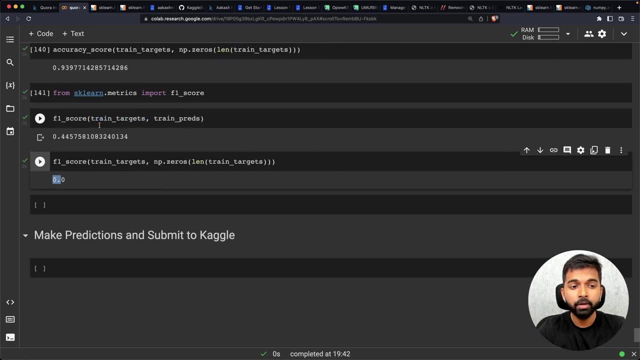 zero. So if we always predict zero, the F1 score is zero. This is because it looks into precision and recall, And one of those will become zero if you're always predicting a fixed value. On the other hand, the F1 score of the logistic regression model is 0.44, which is actually 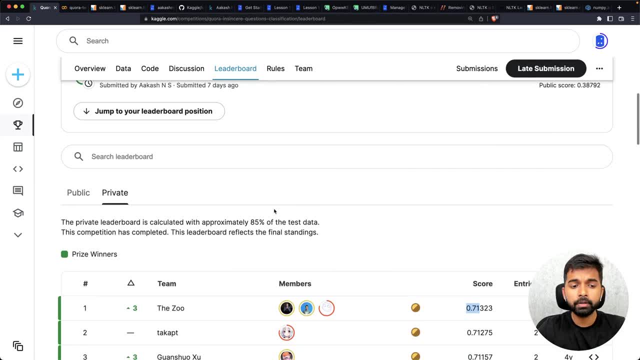 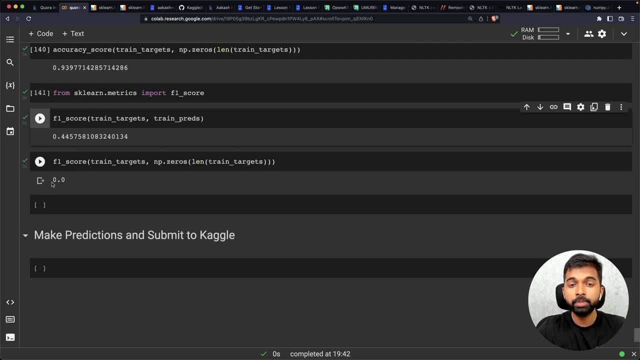 pretty good, considering that in the leaderboard, the top submission is 0.7.. And we have already reached 0.44.. Okay, That is a huge improvement from 0.0,, which is what you get by always predicting a fixed value. 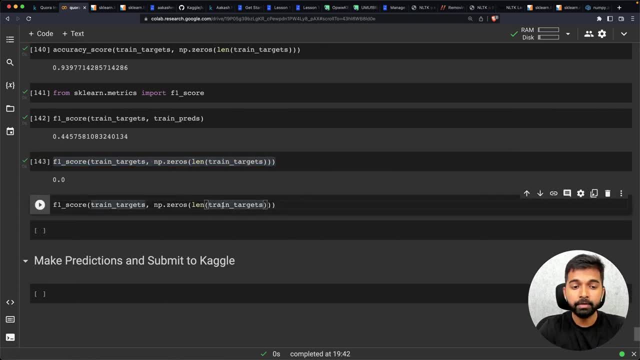 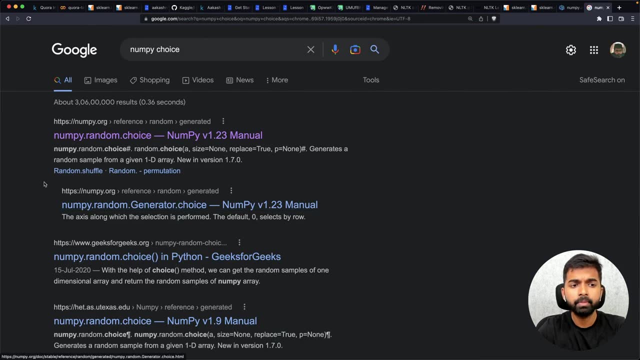 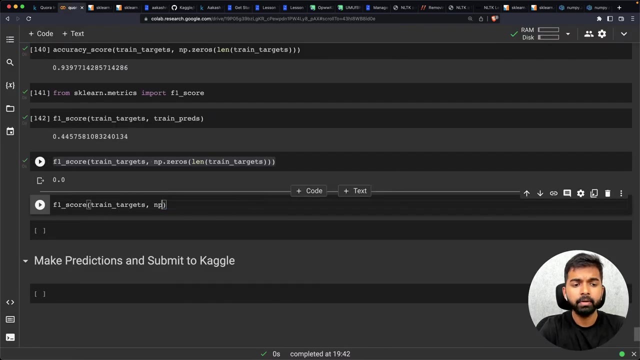 Here's one other thing: you can check What happens if you predict random values. So what happens if you say NP dot? so let's see, numpy choice is a function and p? dot, random dot choice. So let's do that, Let's try, and p? dot random dot choice. 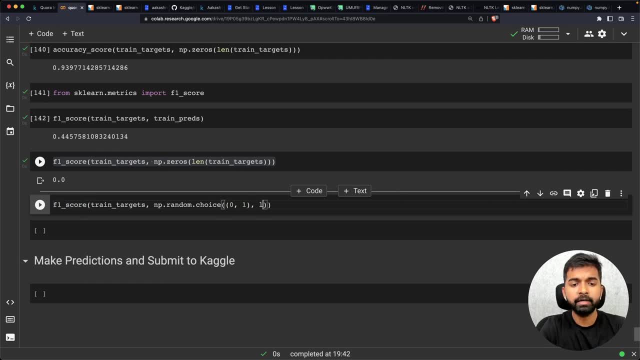 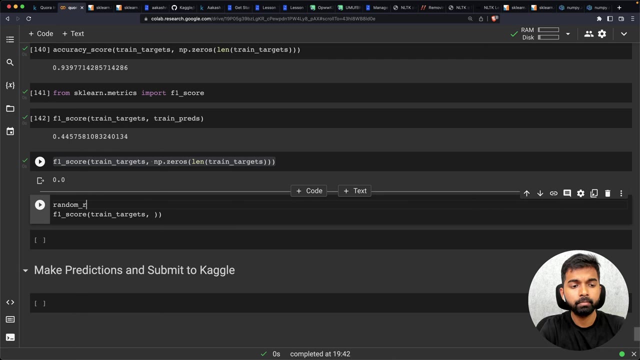 And let's choose from zero and one, And we want a vector of size length train targets. Okay, so these are basically some random predictions. I'm going to just move it out here so that it's easier to read. So all we're doing here is we're saying that let's create a vector of size train targets. 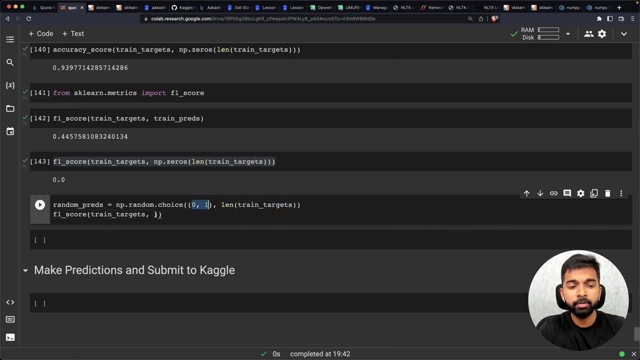 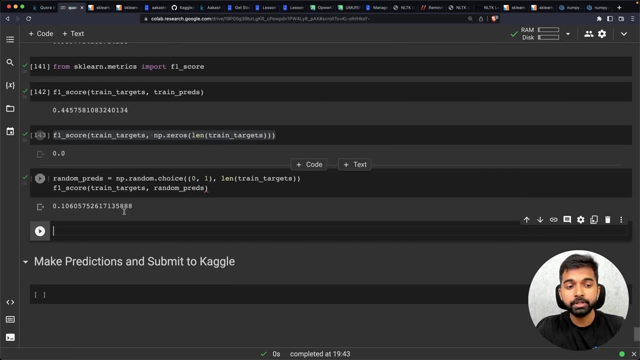 of length train targets, where each value is picked randomly between zero and one. So when you use random predictions, you get the FN score of 0.1.. When you use a fixed prediction of zero, you get an FN score of 0.0. 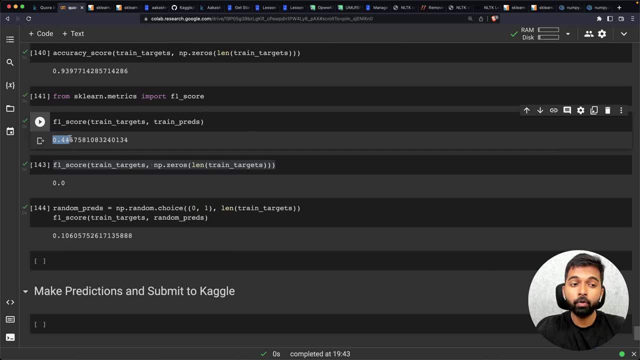 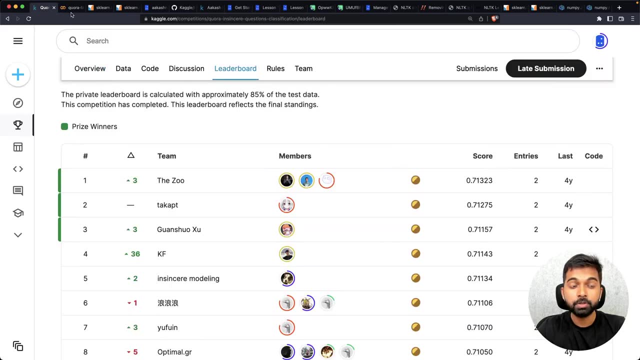 When you train a logistic regression model, you get an FN score of 0.45, almost, That is more than halfway to the best submission, which is 0.71.. So our bag of words model, which is already trained on a very small sample, just a hundred. 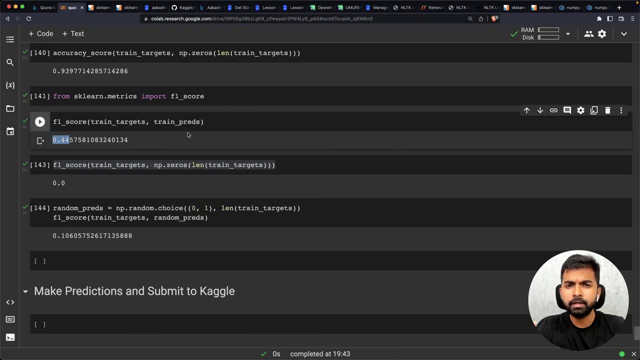 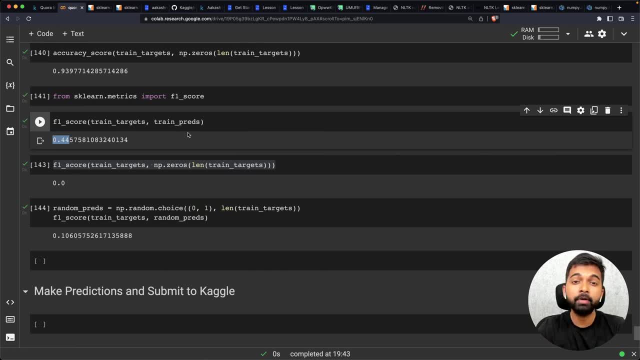 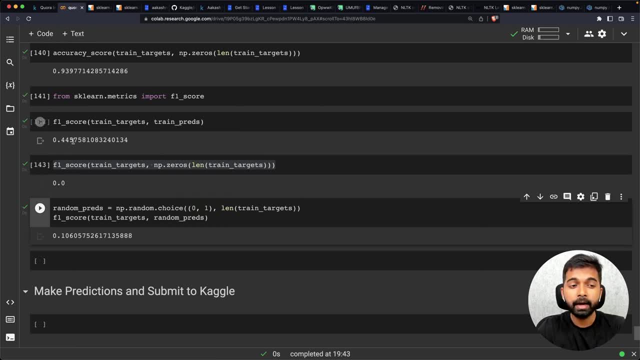 prediction. These are often called baselines or dumb models, and you can use these to identify how well your model is performing. Suppose the FN score that we obtained was very low, let's say 0.05.. Then we could look at this and say maybe we've done something wrong in training the 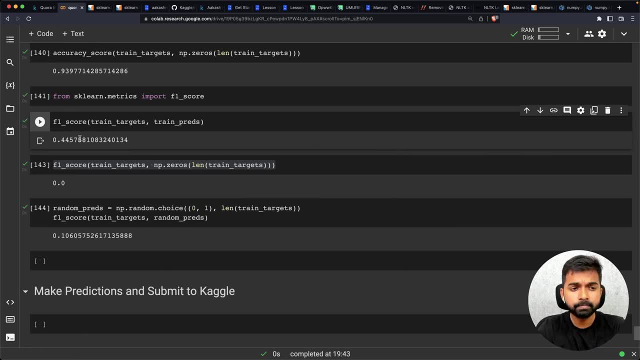 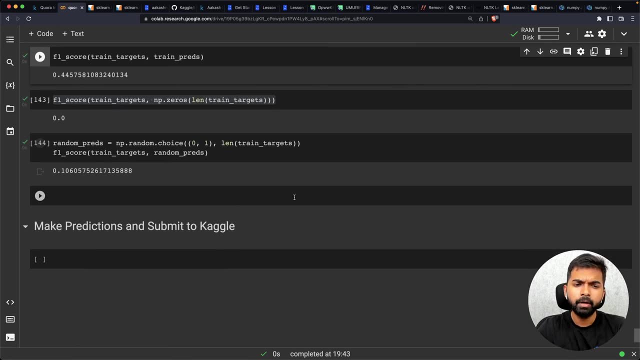 model, or maybe we've not created the bag of words model model properly. So comparing your model to these baseline models is a great way to make sure that you've done everything correctly so far, All right, But all of this prediction was done on the training set and you don't. 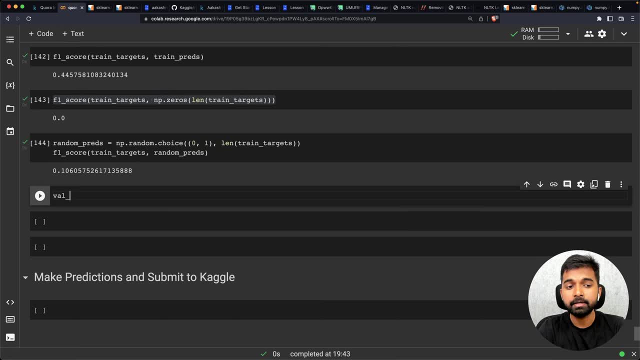 use a model on the training set. You use a model on previously unseen data. So let's make some predictions on the validation set. So let's get valpreds, which is model dot, predict on val inputs, And now we can do again accuracy score. 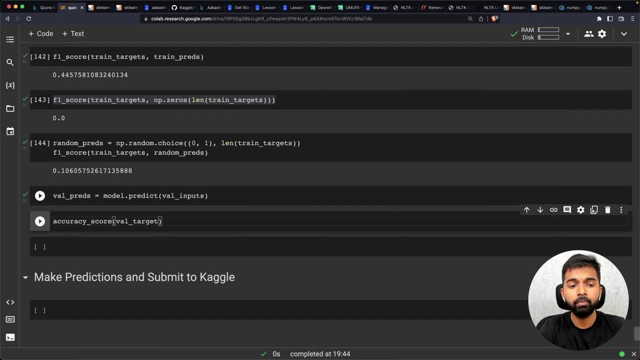 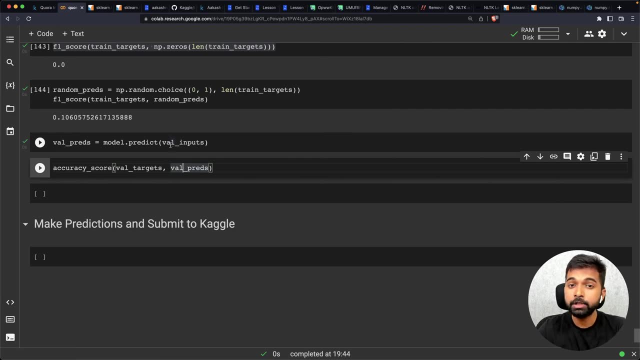 Valpreds or val targets and valpreds. So notice, when we are predicting on the validation set, we are not passing any targets, because the model should never see the validation set targets. The model should only see the training set targets and that it should see. 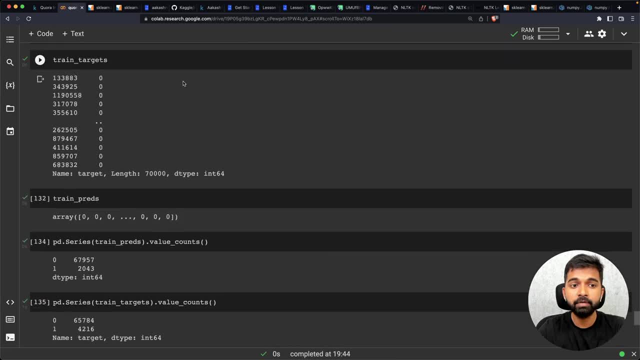 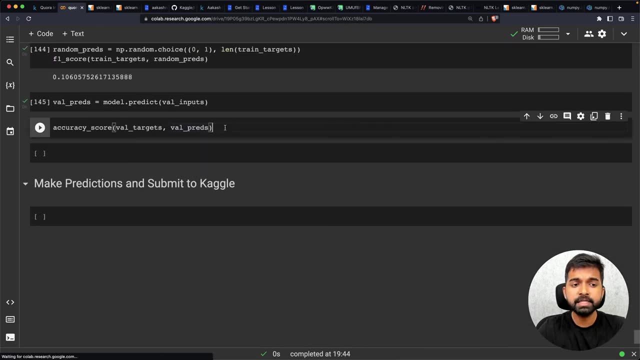 only when you're fitting the model. And, as you can see here, we have fit the model above using the trained targets. but while predicting we never pass the targets. So let's see the accuracy score on the validation targets. Once again, the accuracy score. 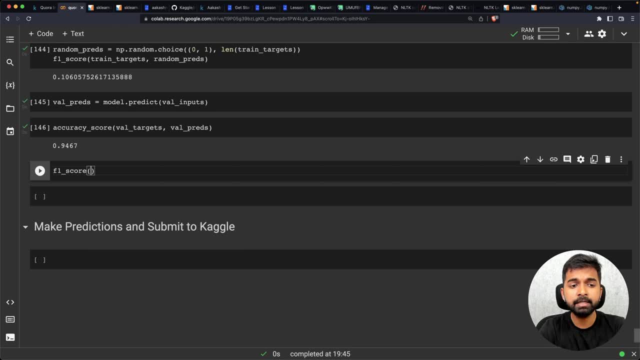 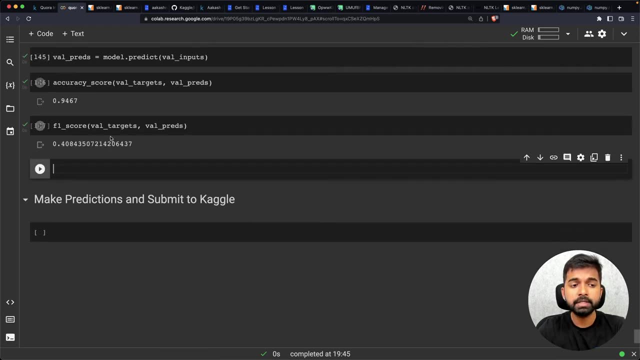 The accuracy score is 94.6, but what we are more interested is in the FML score. So val targets valpreds and the FML score is 0.40.. This is again something you'll notice, that the score generally will be worse. 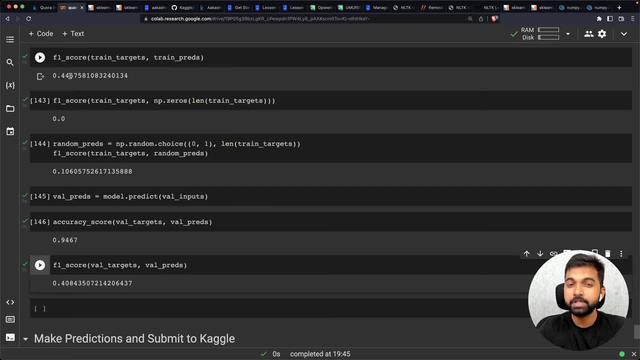 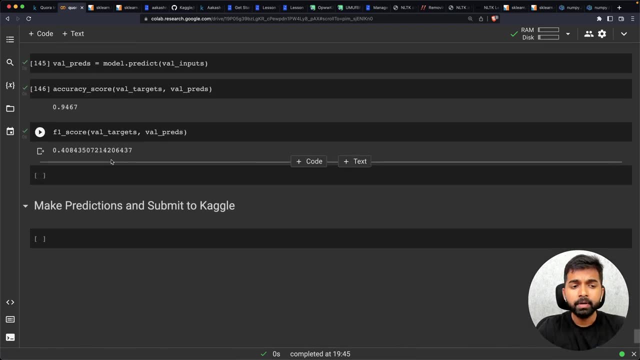 on the validation set because, compared to the training set, because the model has to some extent memorized parts of the training set and that is why we have a validation set in the first place. All right, So now we have done the third part. 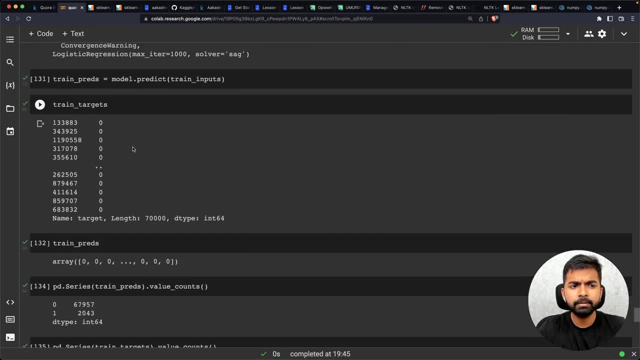 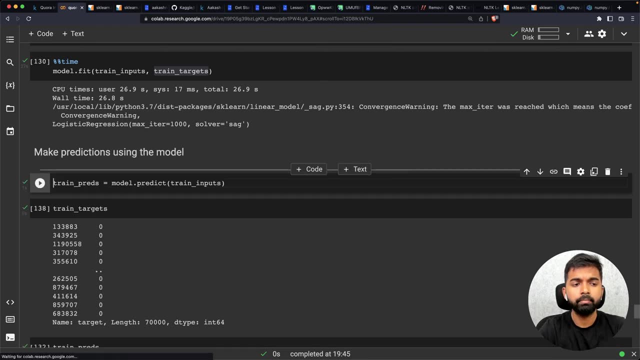 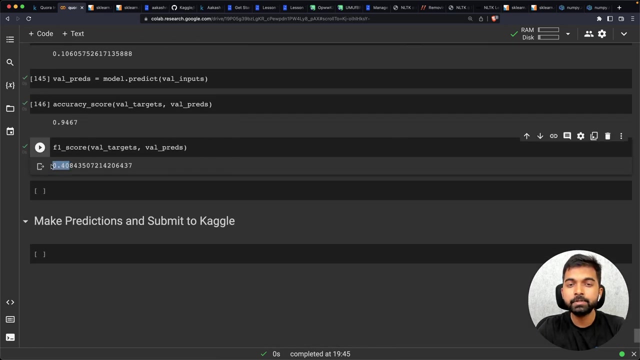 is making predictions using our model. So let's actually create another section here: make predictions using the model And after making those predictions, we have also computed the FML score and looks like the FML score is pretty good. but it also helps to maybe look at some. 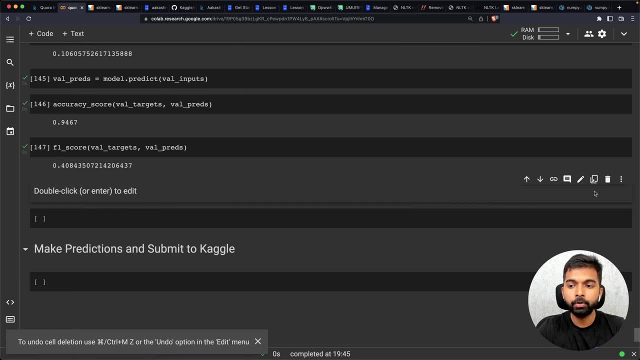 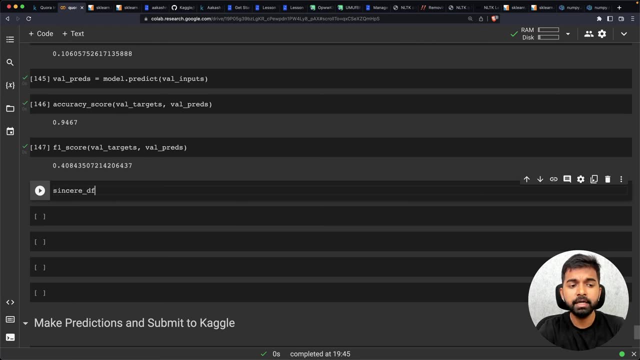 real predictions on some real questions. So here's what I'm going to do: I'm going to pick a few questions from SincereDF, So let's say SincereDFQuestionTextValues, Let's look at 10 questions. 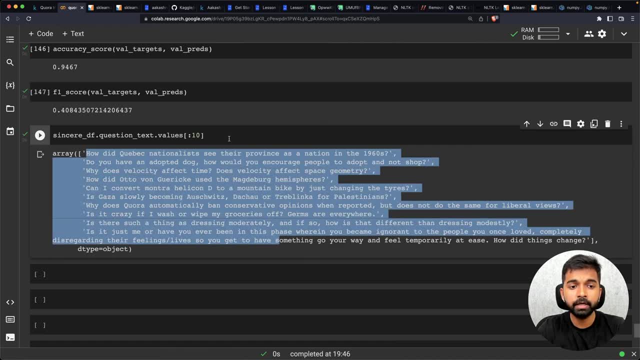 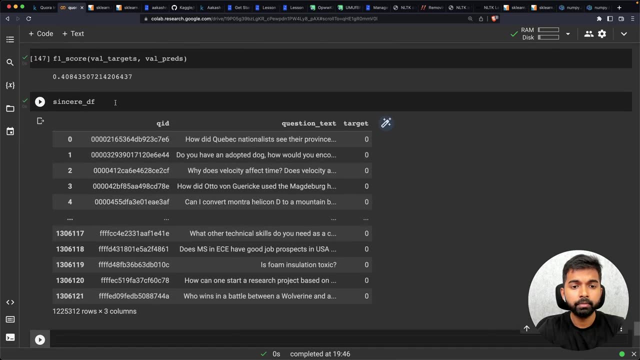 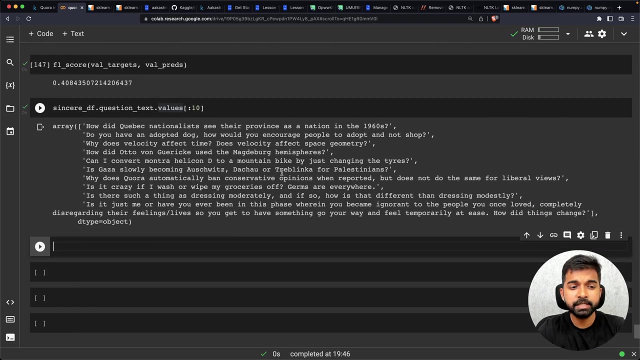 Yeah, So here are 10 sincere questions. Remember, SincereDF only contains sincere questions. All right, So these are all the sincere questions. These are obtained by just checking target zero. All right, So these are all sincere questions. All of these essentially have the target. 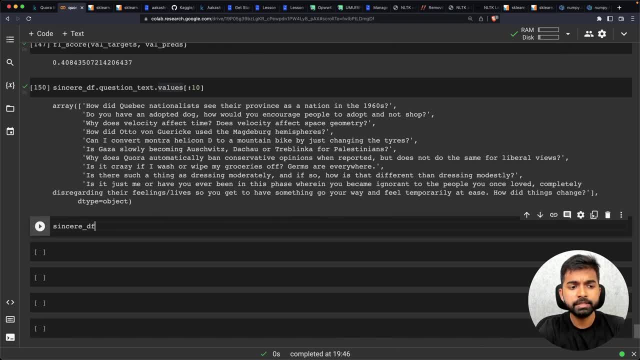 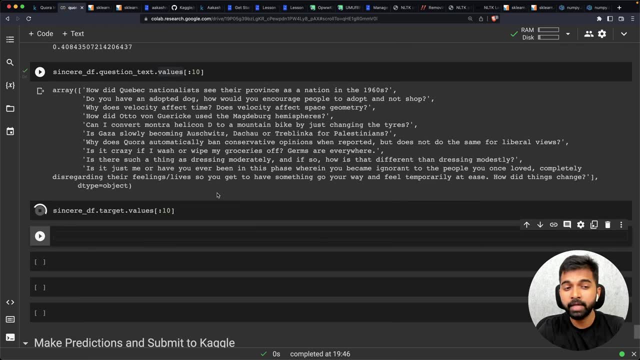 Essentially, all of these have the target one. So let's check SincereDFTargetValues 10.. You can see: all of them have the values. All of them have the target value zero. Now let us make a prediction on these 10 questions using our model. 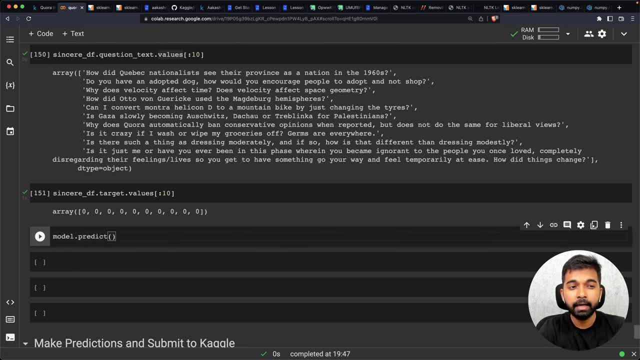 So let's say modelpredict, And we can't give it the question Text directly. So first we have to say vectorizertransform And then we give it SincereDFQuestionTextValues 10. So we are first transforming the first 10 questions of SincereDF into bag of words. 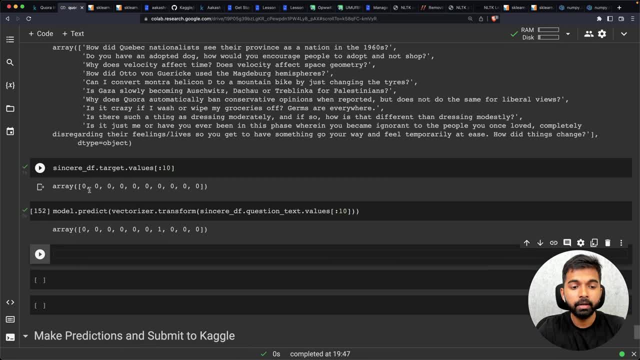 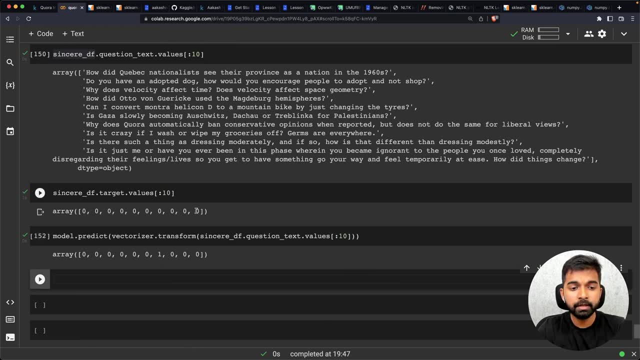 And then we are making predictions using the model, And these are the predictions we get. So it looks like the model got most of these correct, but the model got one of these wrong. Which one is it? It is one, two, three, four. 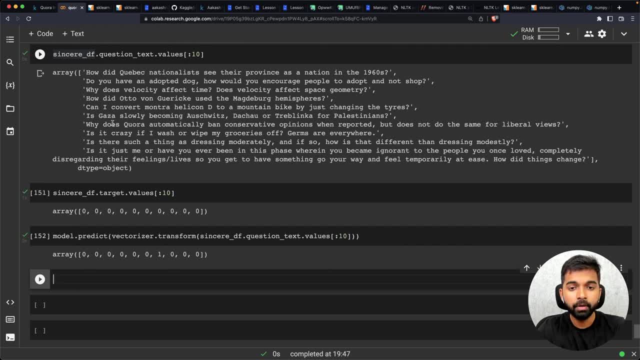 Fourth from the end. So one, two, three, four. Okay, Looks like here. why does Cora automatically ban conservative opinions when reported, but does not do the same for liberal views? Okay, So you can probably guess what's happening here in our target. 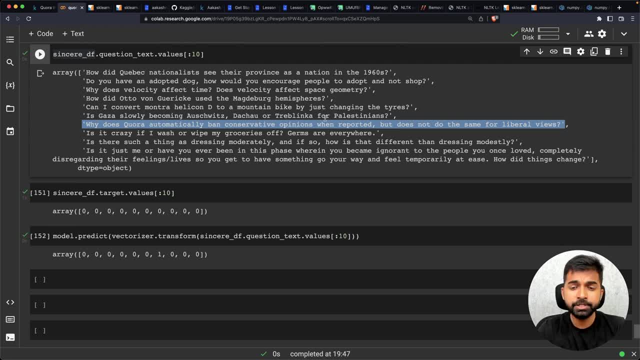 We have the value zero because this is a fairly balanced question. It is not well. it is still somewhere on the boundary possibly, but it is still asking a fair question. It's not offensive, I wouldn't say it is very insincere. 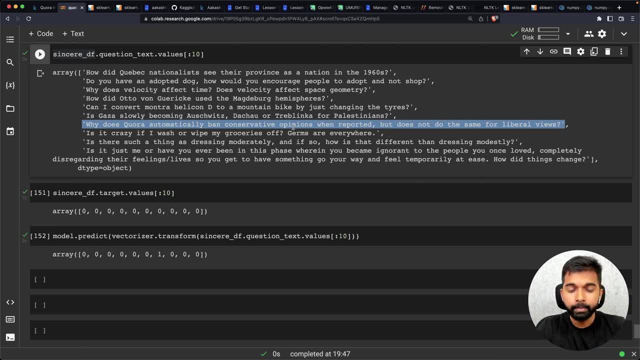 It could be on the boundary, but on the other hand it contains the word liberal and conservative, And those words may be words that may show up, often in insincere questions which are very polarizing, And because our bag of mud model depends largely on frequencies of words and presence of words, 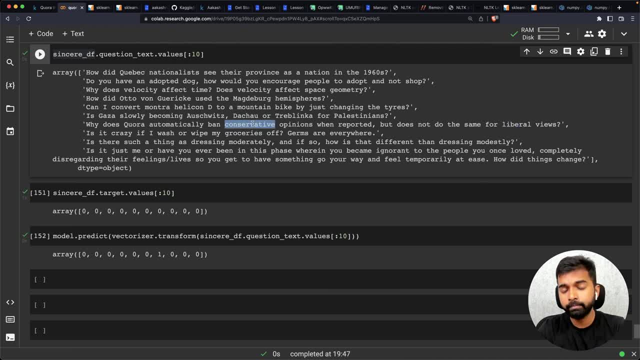 So that's why, by looking at the words liberal and conservative, it may have Okay, By looking at the words liberal and conservative, it may have classified this as a insincere question. So that is the limitation of the bag of words model. 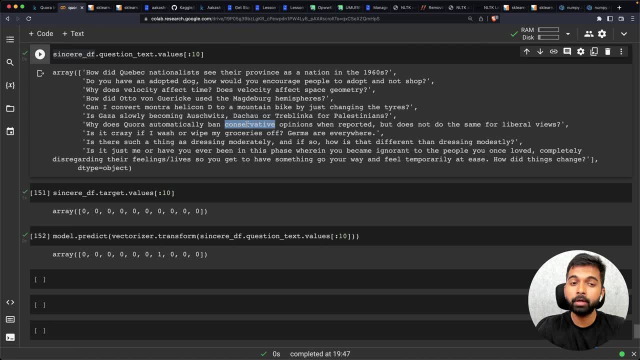 So this is something that you should always do Whenever you train any machine learning model: try to look at some actual predictions. It's all right to look at the metrics, but look at some actual predictions, because that will tell you why things are going wrong where they are. 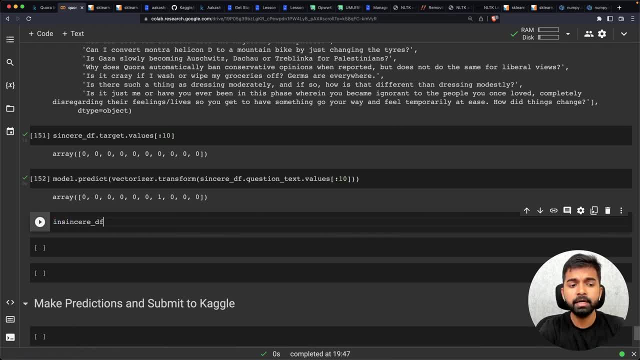 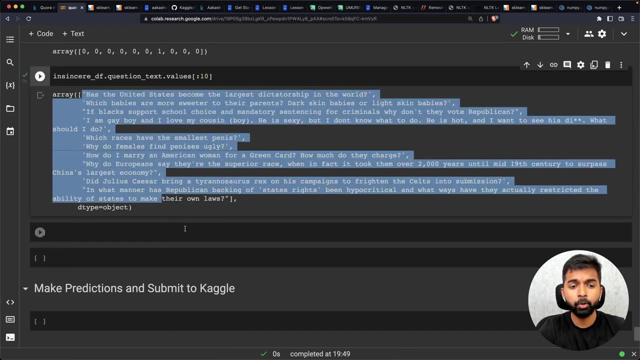 Let's also look at some insincere questions. So let's see insincere DF dot question text: Dot values 10.. So here are some insincere questions. These are clearly all very inappropriate questions to ask. And now let's make predictions. 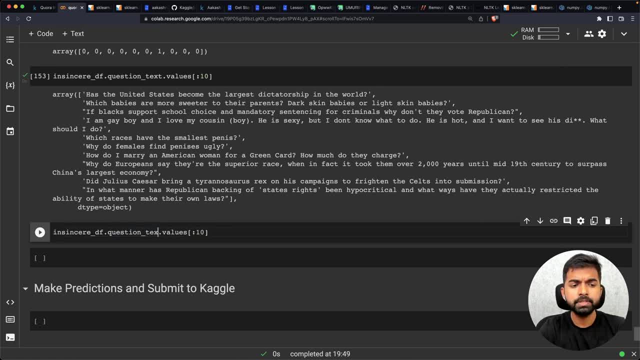 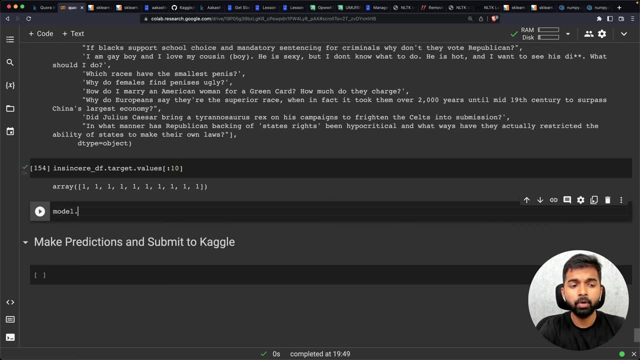 Let's check the targets as well. So insincere DF, dot, target, dot values 10.. So the targets are all one. obviously let's try model dot predict, Vectorizer, dot Transform, Insincere DF and question text 10.. 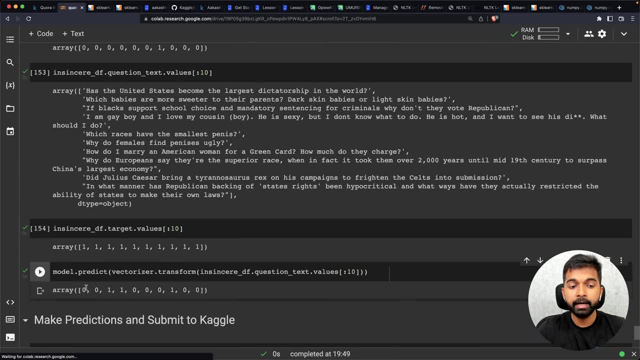 Okay. So now you can see that here it's actually getting them wrong quite often. The first question: has the United States become a largest dictatorship in the world? It got it wrong. It thinks this is a sincere question. The second question, which is something about, uh, related to skin color- it is also not able to classify that as insincere. but the third one: probably it's picking up. 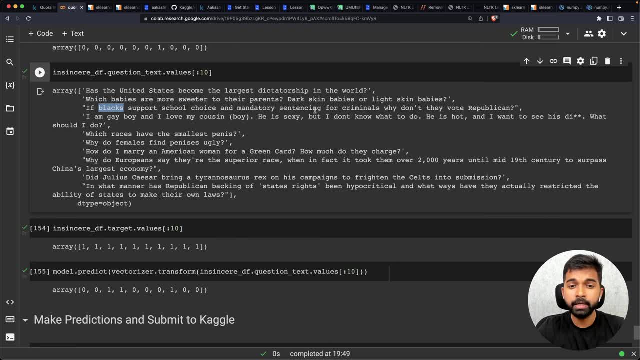 Because of these words, which are possibly more likely to occur in insincere questions. So every model that we create thinks in a certain way. So the bag of word models clearly is thinking about which words occur and how frequently they occur. So you can see why it's making certain predictions. for that reason, 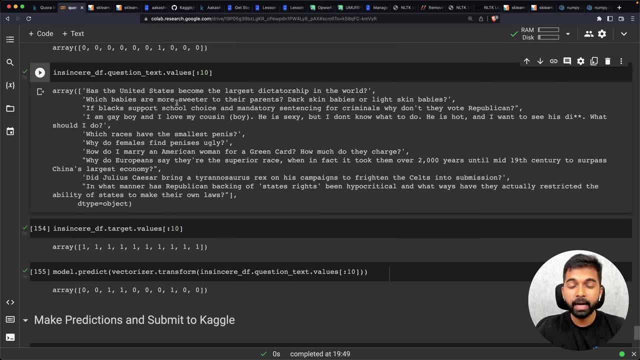 As we study more complex models, we'll understand that bag of words is actually quite simple in its approach. It's not considering the order of words, It's not looking at punctuation, It's not looking at negation Okay, It's dropping things like case. 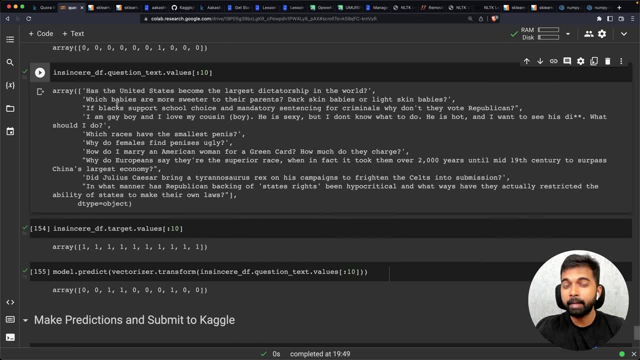 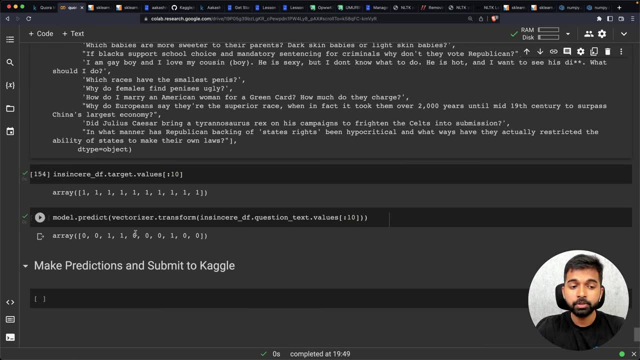 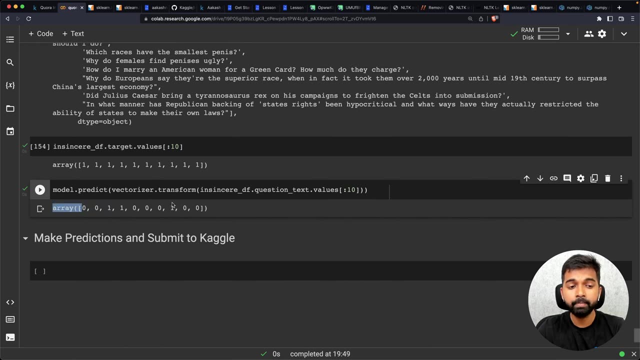 So it's obviously has its issues, and its application should be limited to those cases in which these limitations will not cause a major problem. So because if Cora were to use just a bag of words model, it would be classifying some sincere questions as insincere and they would be classifying certain insincere questions as sincere. 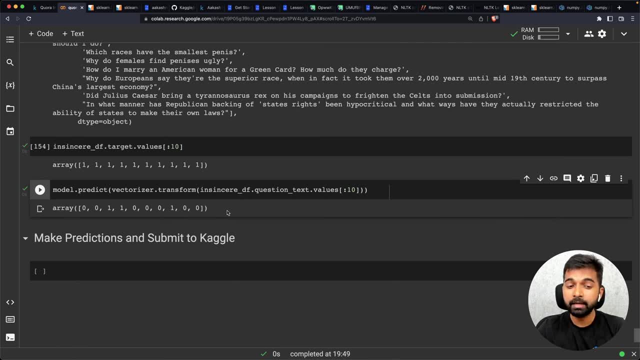 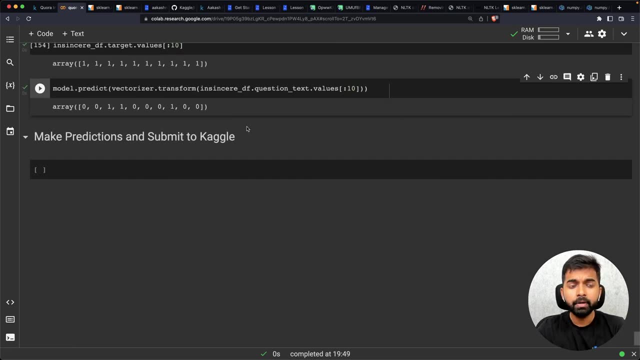 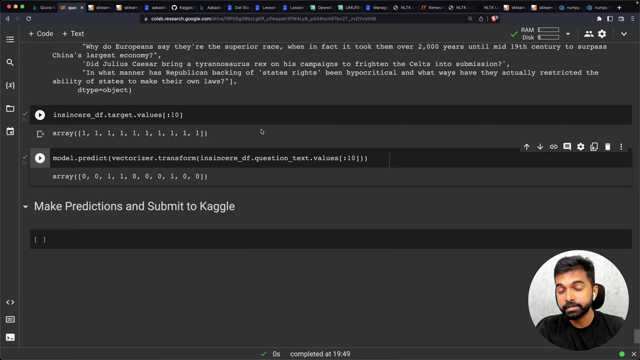 So it may not be the best approach for them, but it's better than nothing And potentially what it could do is serve as A first level of filtering. All right. So that's how you train a bag of words model, And that's how you train a text classification machine learning model, using bag of words vectors, and we've seen it how it's applied to Cora as well. 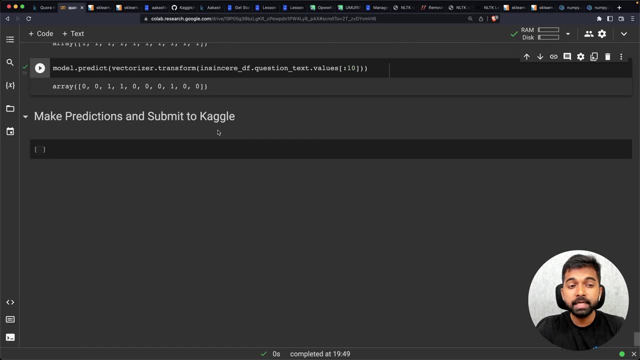 Now one last thing here. we are going to now make some, make some predictions and submit it to Kaggle. Let's look at train inputs and let's look at the train DF. So here is our train DF, or train data frame. 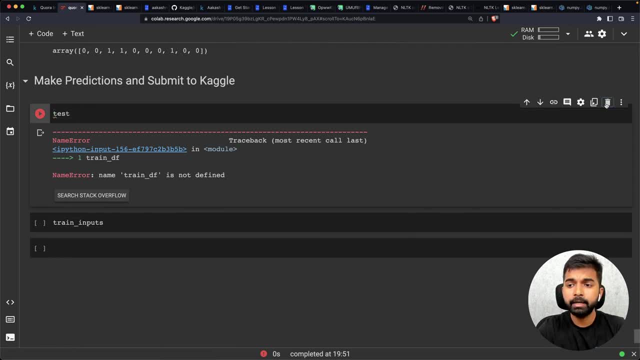 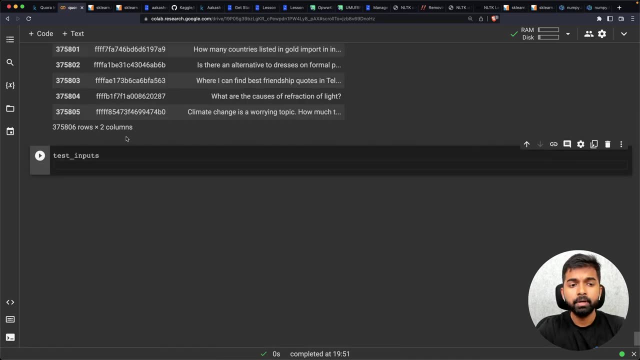 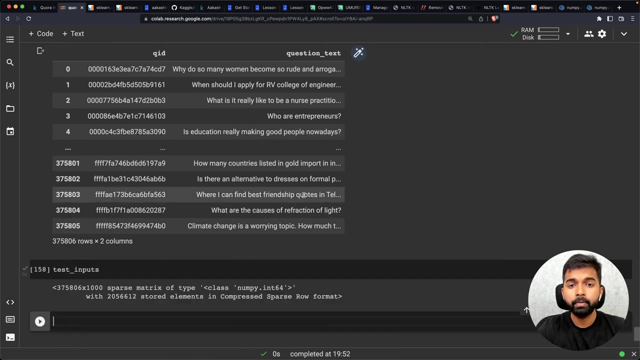 Oh, I'm sorry, Let's look at- let me delete that. Let's look at our test data frame and let's look at our test inputs. So our test data frame only contains question text and these question texts have been converted into test inputs, which is a sparse matrix. 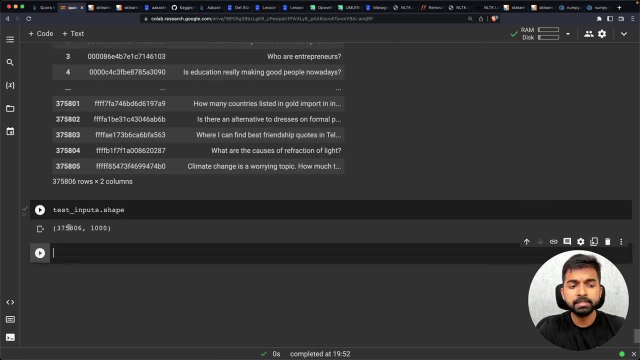 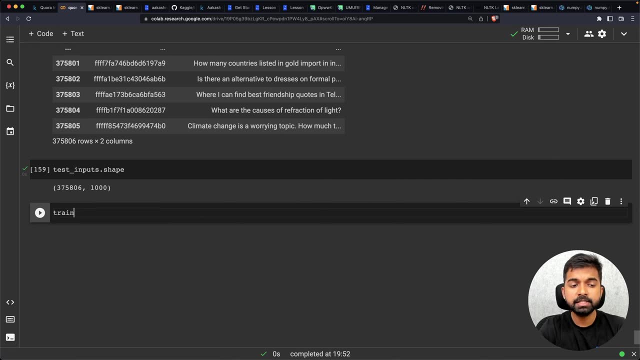 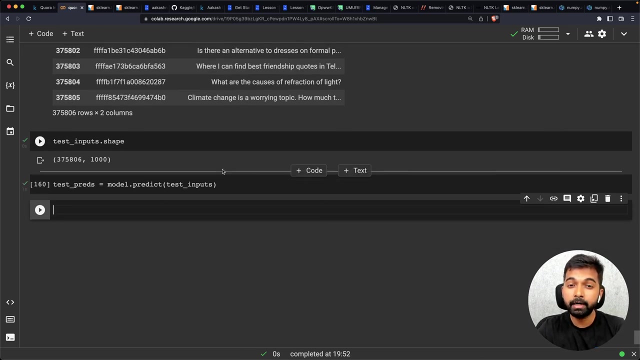 You can check it shape. So it contains 375,000 vectors, each of size thousand. Now we can make Predictions on the test set using the same train model So we can say: test threads equals model dot predict test inputs. And that is going to take all these test bag of word vectors which have been transformed using the vectorizer trained on the training set. 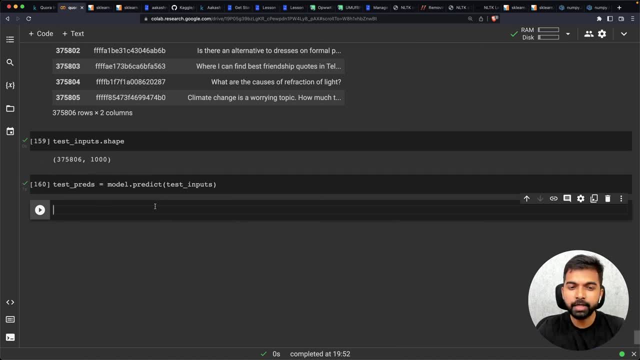 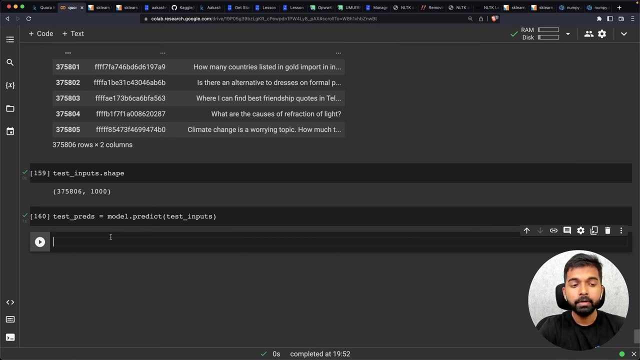 And now we want to check the accuracy of these predictions, but we are not given the predictions for the test set. What we have to do is submit these predictions to Kaggle. So to submit these predictions to Kaggle, We have to create a submission file. 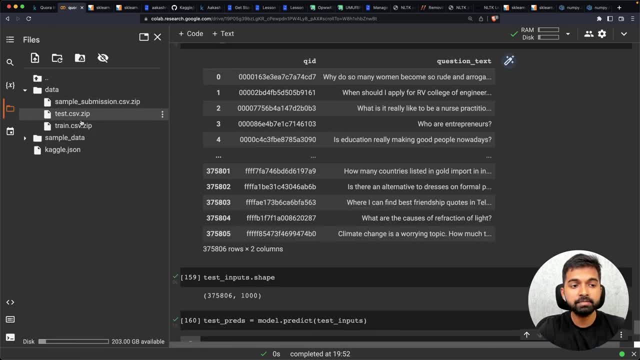 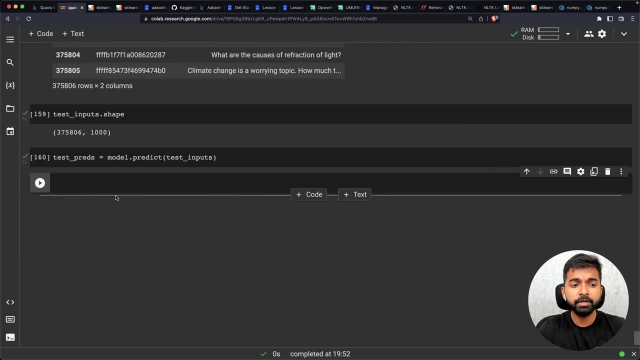 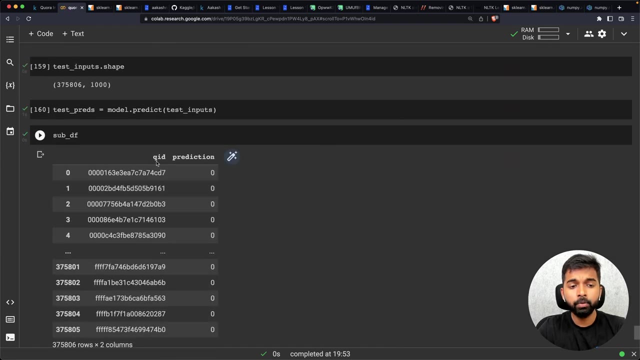 How do we create a submission file? So remember there is the submission dot CSV file that we had submission or CSV dot zip. So we need to load up the submission or CSV dot zip, which we've already done in sub DF, And what we need to do is, against each question ID, we need to make a prediction on the test data. 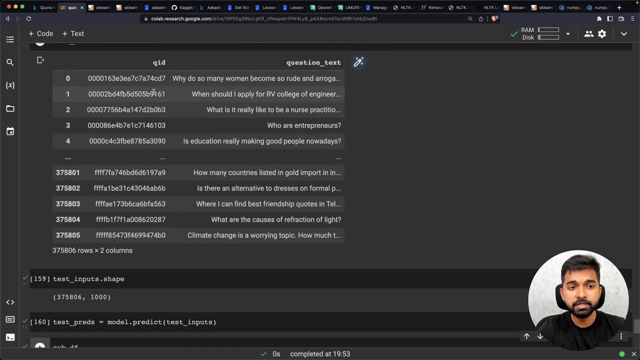 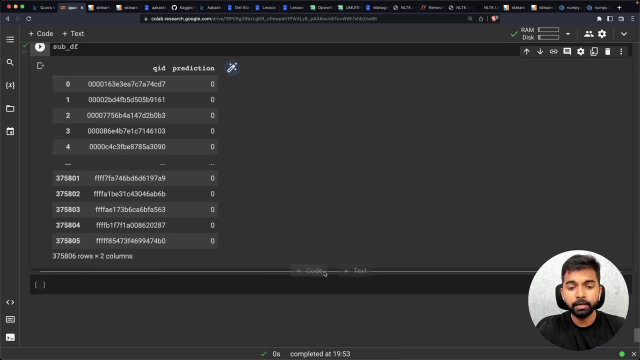 Now these question IDs are in the exact same order as the test data itself. So CD seven one six one, Zero B three. CD seven one six one zero B three. So here's a quick trick that we can use. I can simply say: sub DF dot prediction equals test spreads. 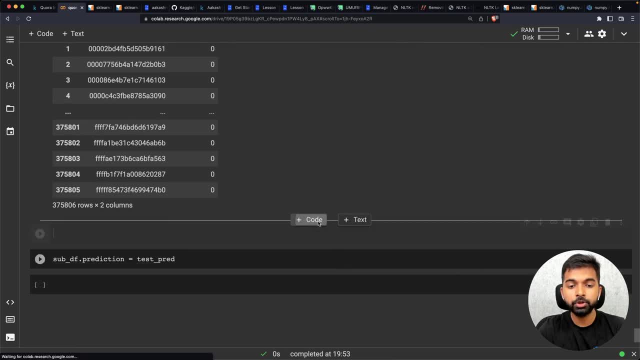 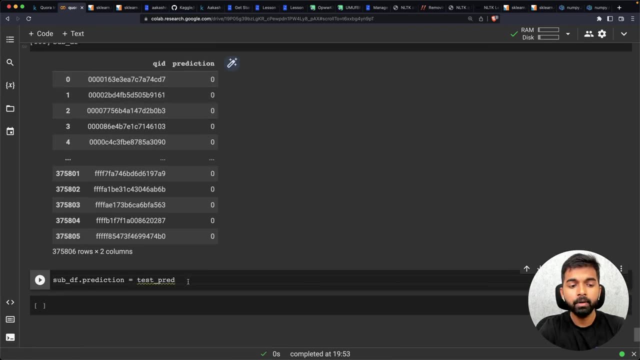 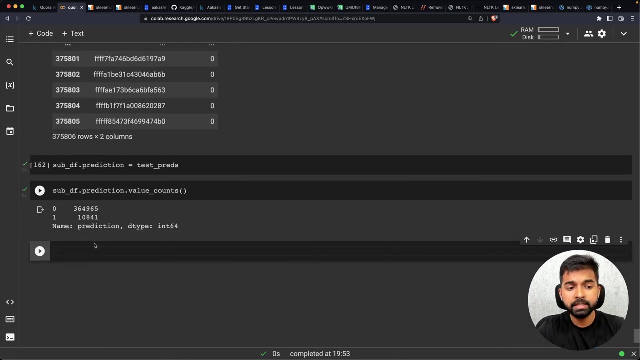 Okay, And before I execute this, I just want to show you what the uh and remember, sub DF only contains all zeros, So sub DF predictions only contains all zeros. but once we do, sub DF, dot prediction equals test brands. Now you can check sub DF dot prediction. dot value counts and it's going to contain some ones as well. 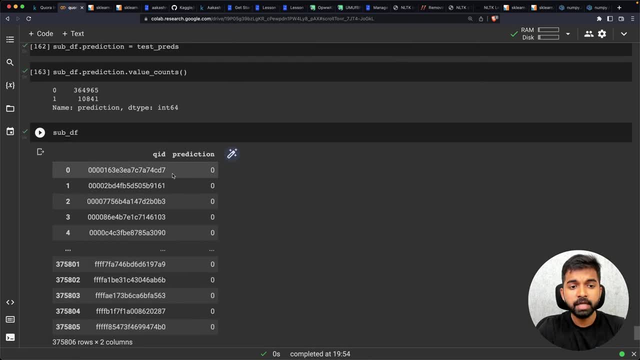 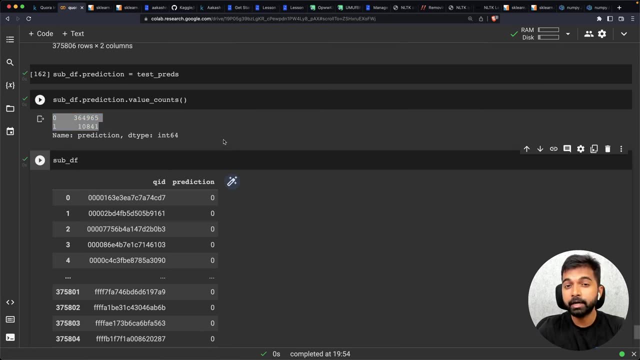 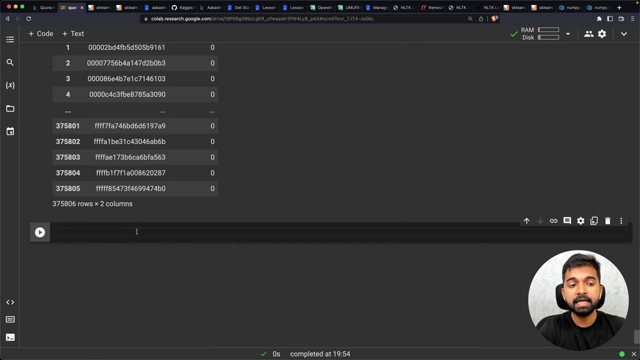 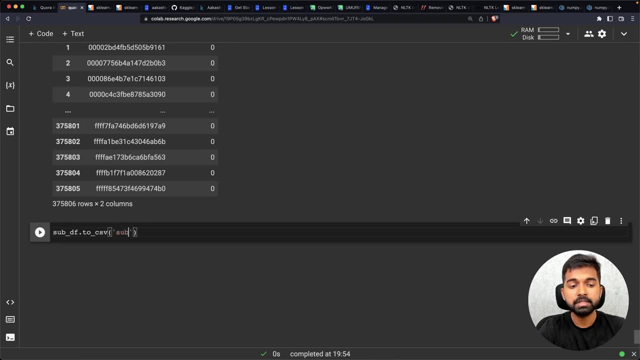 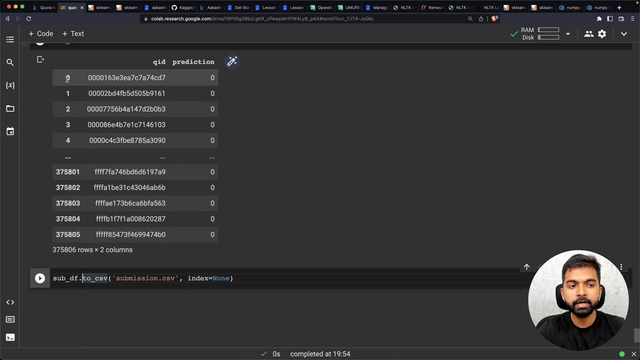 Two CSV: Submission dot CSV, And I'm just going to set index equals none And I let you figure out what this does. but basically, if you don't pass this, then pandas, the two CSV function, is going to add another column called index, where it's going to put these random numbers which I don't want. 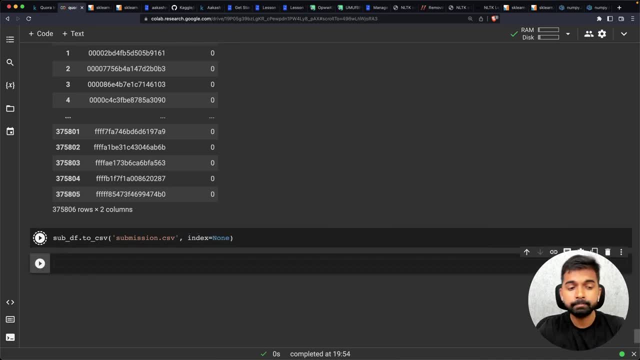 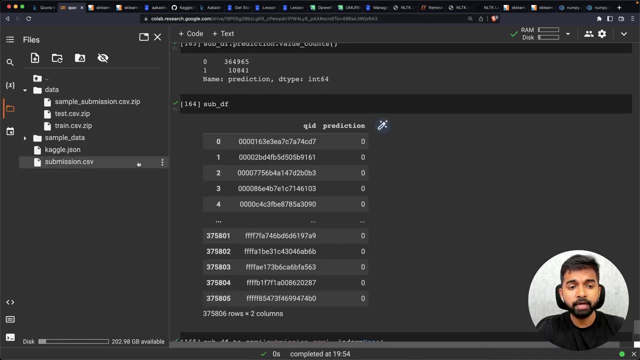 You can experiment with and without and see what the difference in the output file is. All right, So now we've created a submission file. Now if you go into Our files tab here, we should have a submission file and I can click this. so I can. file is too large. 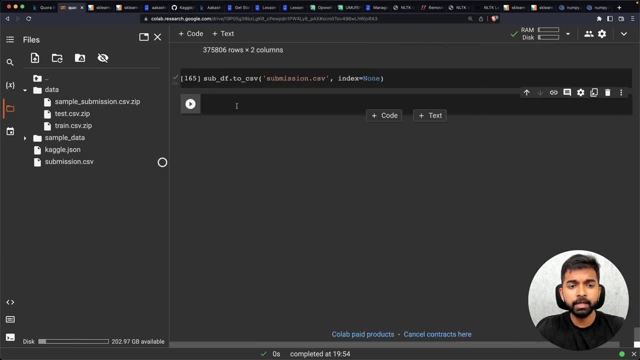 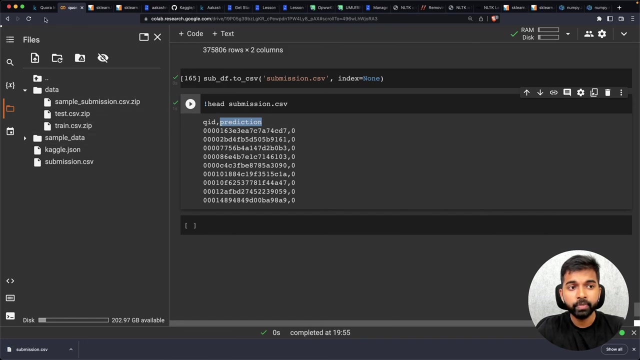 So I can just download this file and I can also display the first few lines of this file. So, using head, you can see that it contains a question ID and it contains a prediction, as I expect, And I download the submission or CSV file and now I can go back into the competition and now I can click. 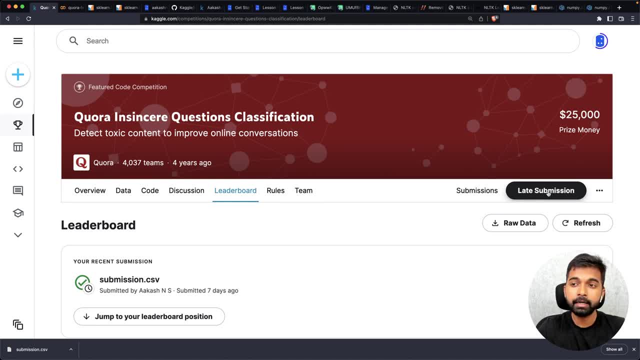 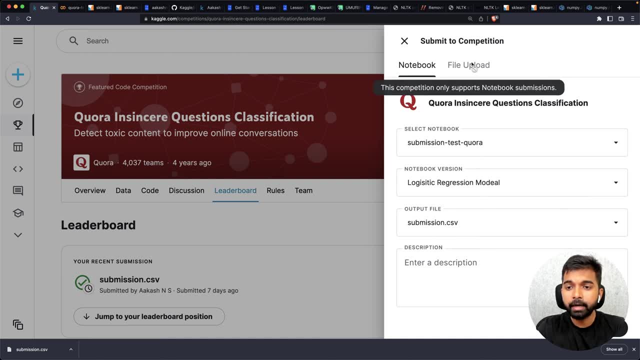 Late submission. Once I've accepted the rules of the competition, I can click late submission and I should be able to upload the file. Oops, Okay, It looks like I can't upload the file here because this particular competition is what's called a colonel's only competition. 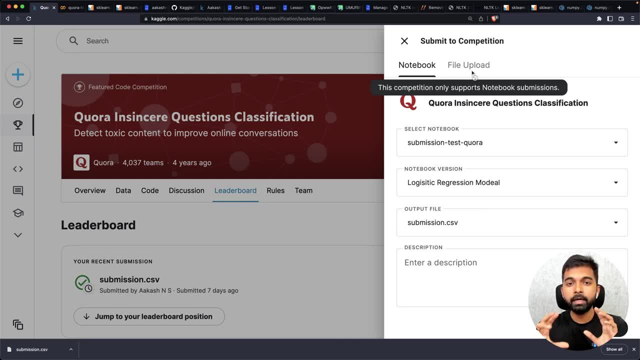 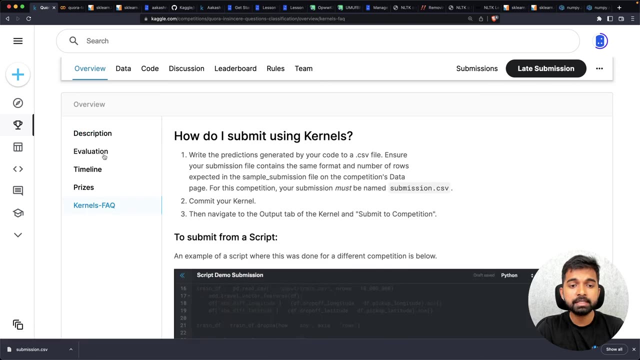 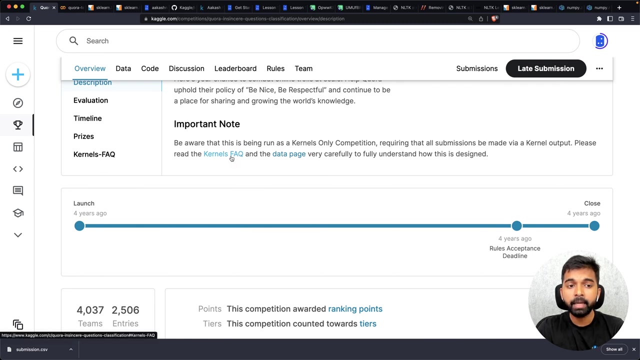 So Kaggle has two kinds of competitions. One is where you can directly submit a set of predictions as a submit, a sub submission or CSV file. That's when this file upload option is open. But in this competition, if you go in here, you will see that this competition is a submission, is a colonel's only competition, which means that you have to make a submission by creating a notebook on Kaggle. 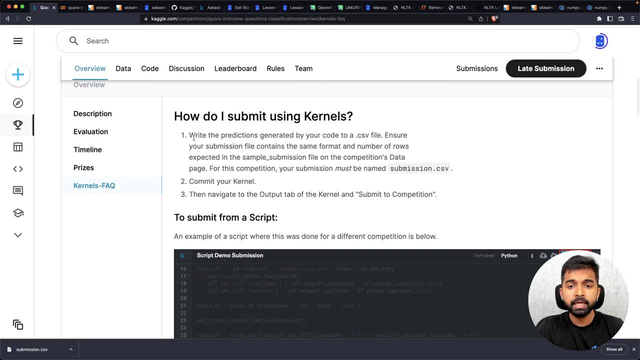 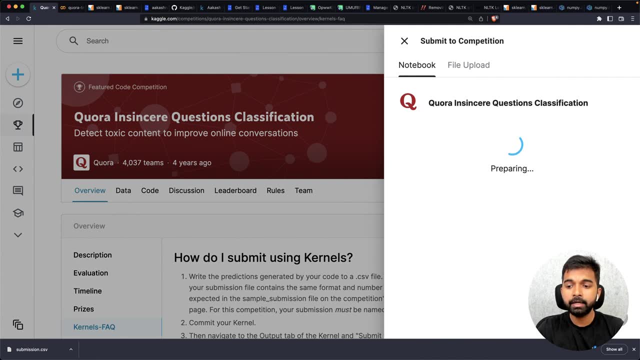 So if you check the colonel's FAQ here, you can see that you have to make a submission by first creating a notebook on Kaggle. And there are a couple of ways in which you can create a notebook on Kaggle. One is by clicking submission and then creating a new notebook here. 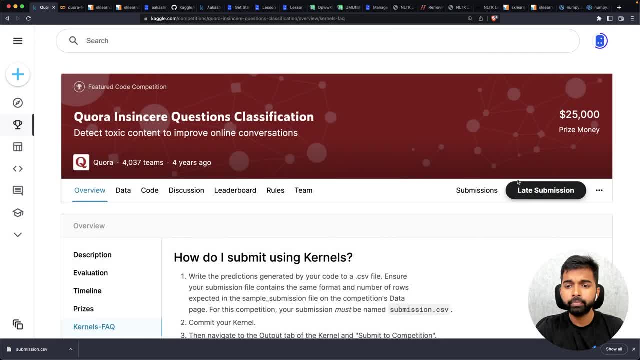 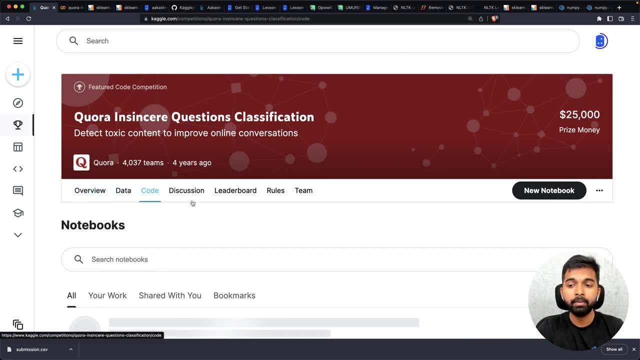 So you can- um, okay, Not here. Well, you can. you can go into the. so there are a couple of ways you can create a notebook on Kaggle. One way you can do it is go into the core tab of the competition and create new notebook. 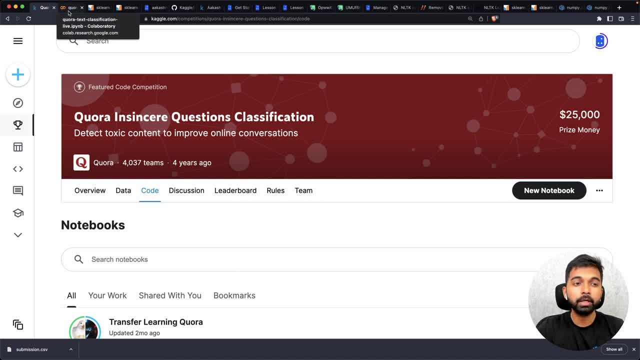 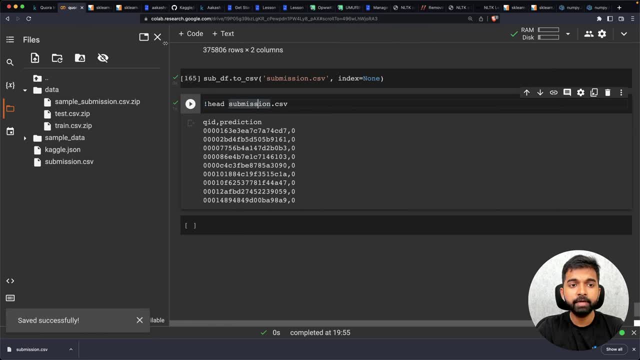 But here's another way I'll show you which is easier to work with: if you're working on your own computer or on Jovian. So let me save this file And once I save it I can come back here and on Jovian. 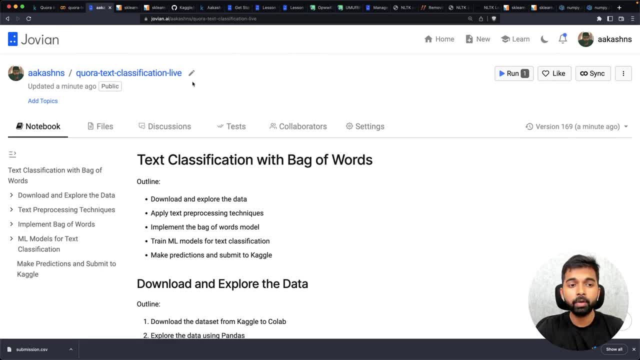 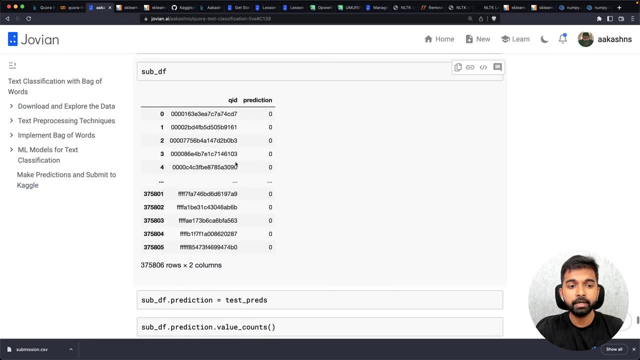 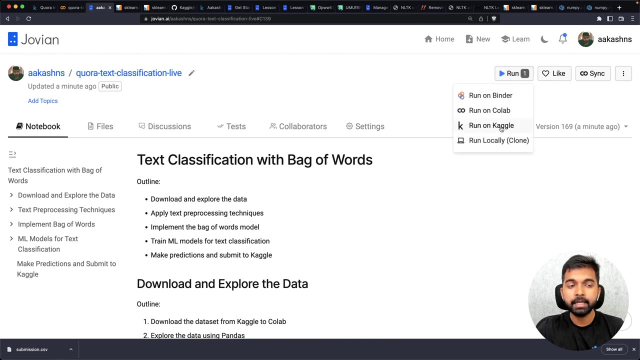 And now this notebook would have been updated on Jovian So you can see Cora text classification. Live has been updated. Okay, It has. download explore data, set, implement, make predictions. All of that is done. Okay, Now I can go up right to the top and click run and select run on Kaggle. 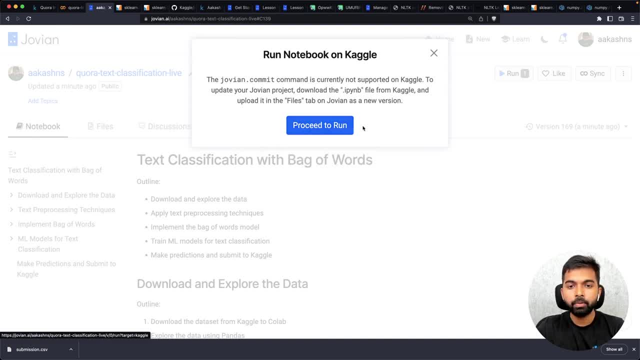 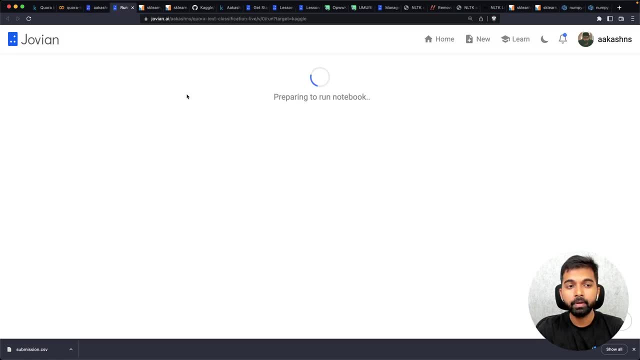 Now, this is a one-way integration at the moment, So work done on Kaggle is not going to get saved back to Jovian, but you can take this Jovian notebook and open it up on Kaggle. So now what we're doing is we are taking this Jovian notebook and we are 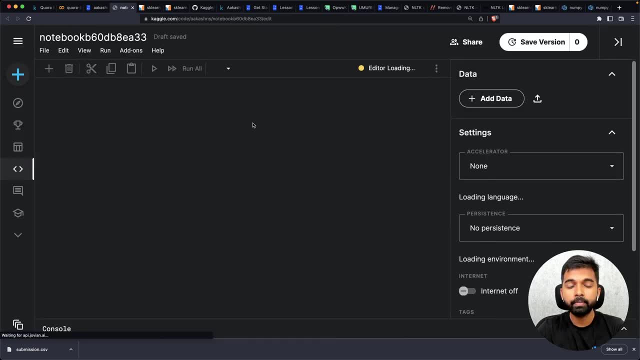 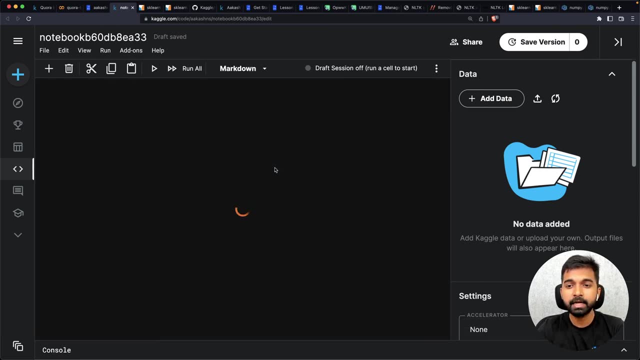 opening it up for you on your Kaggle account. And this is what a notebook on Kaggle looks like. So it is just like Google collab, except that it has a few more bells and whistles. It has a slightly different interface. 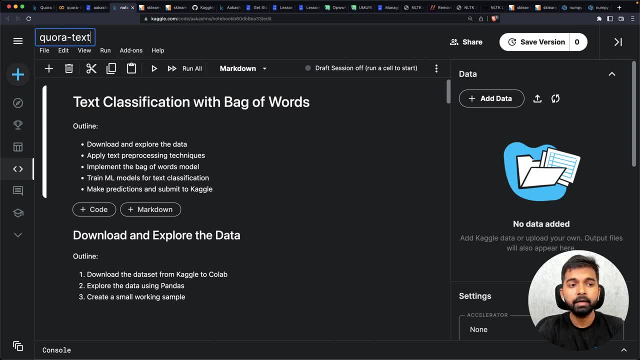 Let me just call it Cora: text classification: live All right. So now my Jupyter notebook, which was earlier on Google collab, was saved to Jovian and then from Jovian it was run on Kaggle. You can see. all the same code is present here. 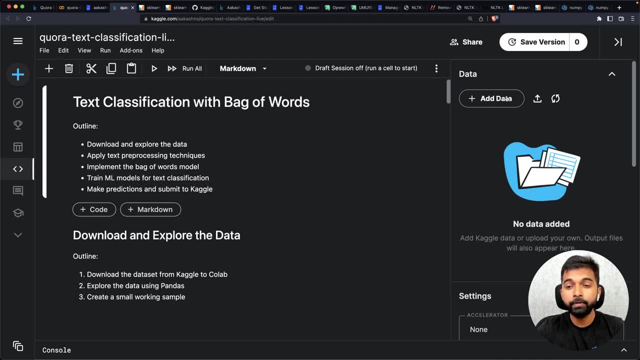 Now here I am going to attach the data set of the competition. So when you're running a notebook within Kaggle, you don't need to download the data set separately. You can attach it from the sidebar. You'll find the sidebar on the top right. 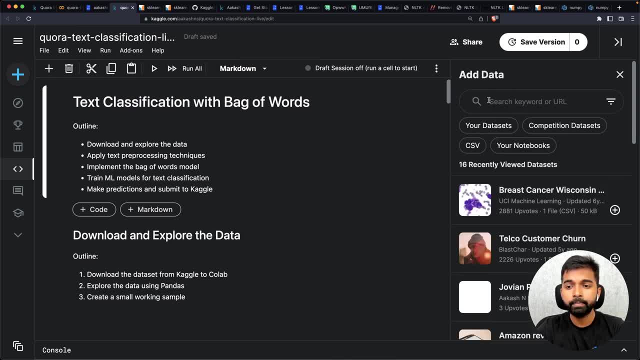 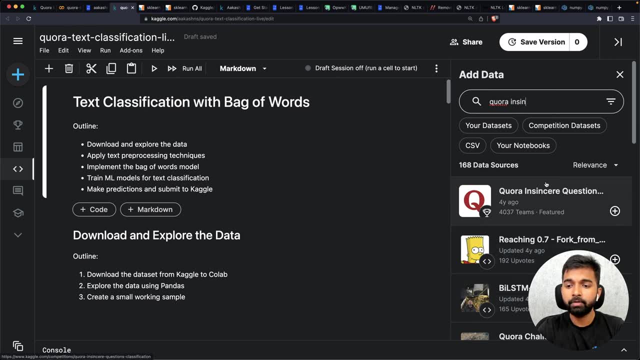 Or you click this button open the sidebar. You can click add data and let's just search for Cora. insincere question classification: Yes, And you can verify that. this is the same competition And I'm going to click plus. And when I click plus, this data gets added as an input. 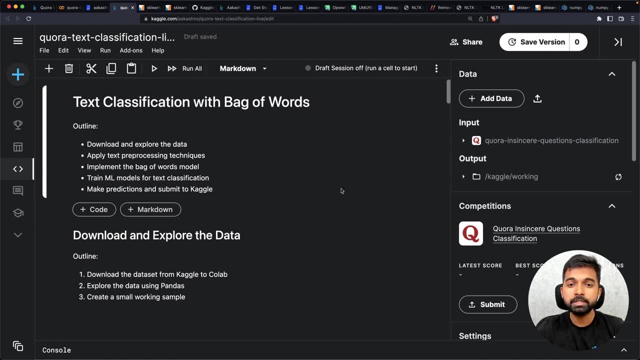 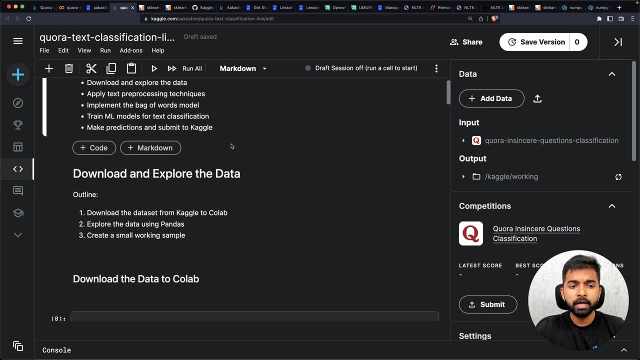 So now we no longer need to use the Kaggle download command, because this data is already added to my Kaggle notebook And in fact I can simply copy the file path here. So now, if I go down here slightly, I may have to make a few changes. 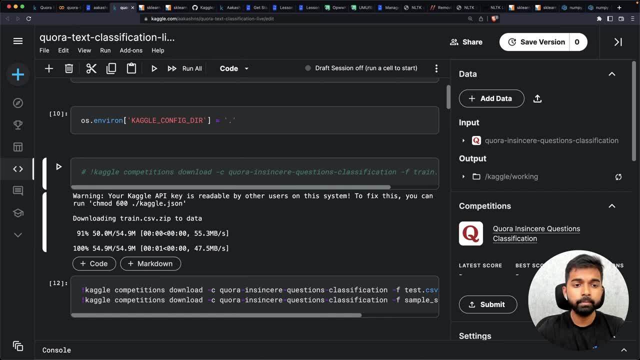 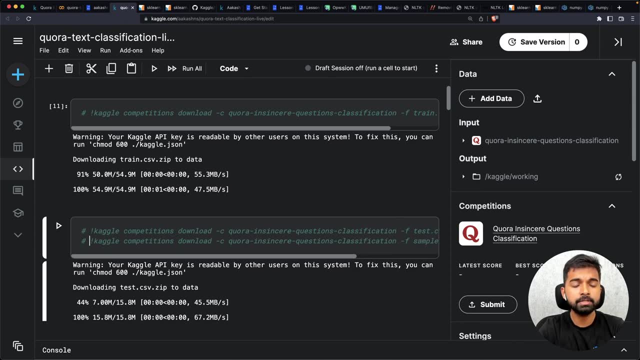 Now I no longer need to do this, so I can comment this out: I no longer need to Set this environment variable. I no longer need to set this. I no longer need to set this. All of this is not required. Here is something that I may need to change. 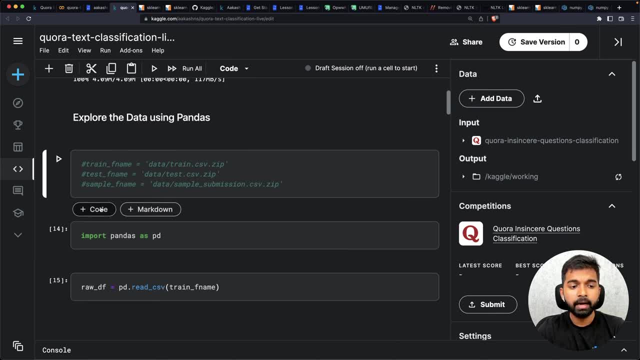 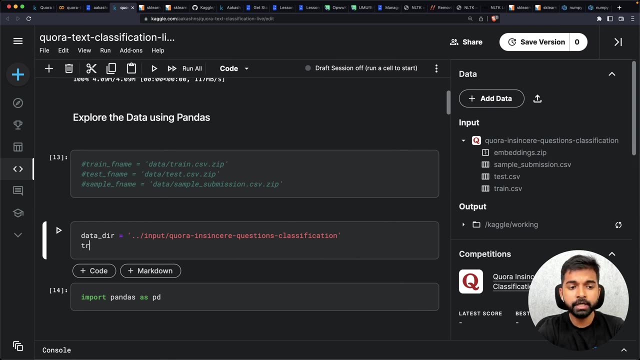 So I may need to just change these, and I'm going to just change it to this. So I'm going to first say: data DIR equals this. So I've simply copied the path of this input directly where all the files are located, and then I'm going to say: train F name equals. 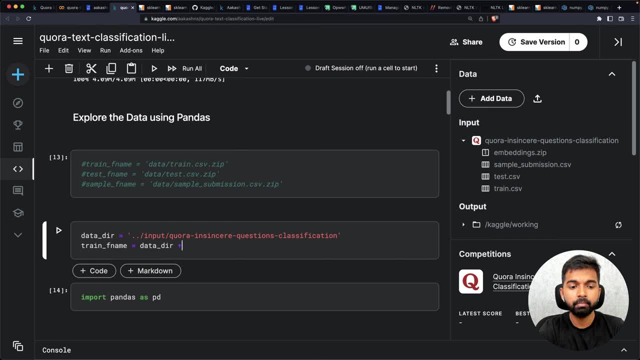 data underscore DIR plus Slash train dot CSV. You can see that here it's not a zip file, It is just a CSV file. Similarly, test F name equals data DIR plus slash test dot CSV. And finally, sub or sample F name equals data DIR plus. 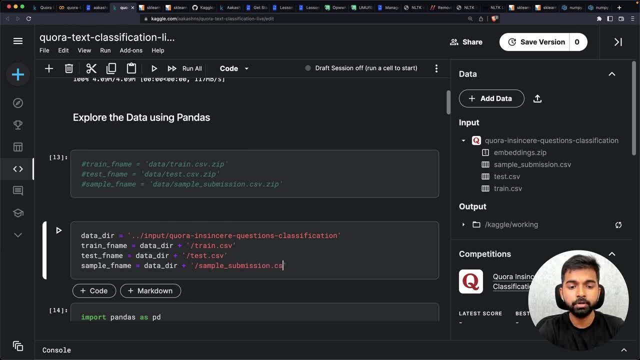 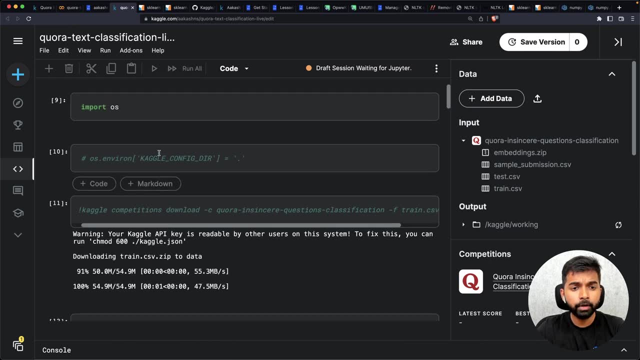 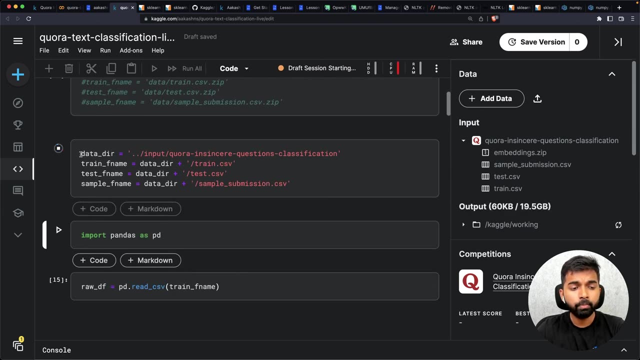 Slash. So all we are doing here is commenting out the code for downloading the data set. We're no longer doing that. Instead of that, we have written some new code, because the data can already be attached And this can take a moment to start, but once it started up, you can see here. 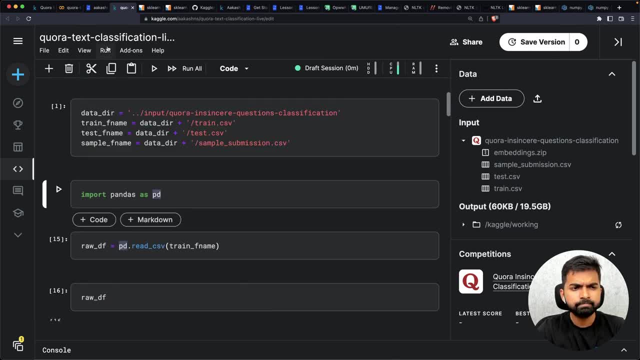 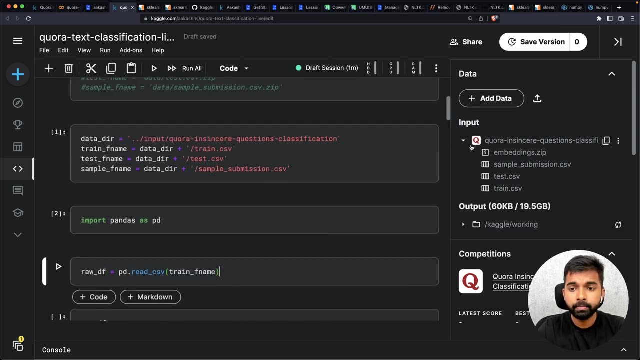 Now we have the data directory set up and I'm going to do restart and clear outputs, just so that all the outputs are clear. and now I am going to import pandas as PD and now when I say pdreadcsv train underscore F name, it is going to use this. 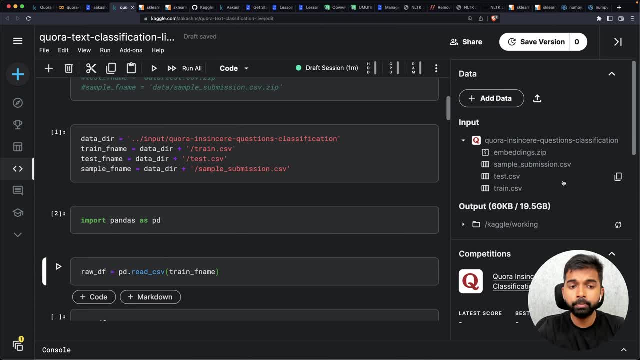 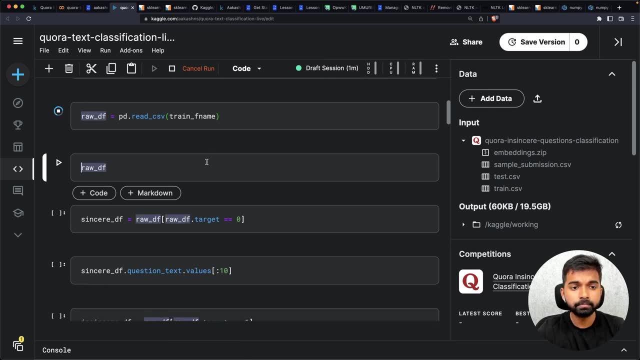 path and a dot dot slash, input slash Cora and sincere questions, classification slash, train dot CSV, and it's going to pick up this data frame and I can check it out And I can run the future cells and I can just make sure that all the data is getting. 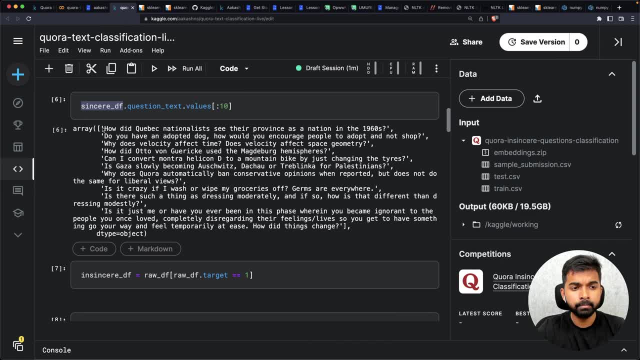 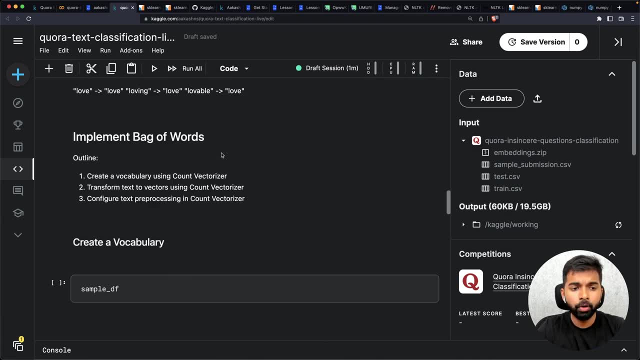 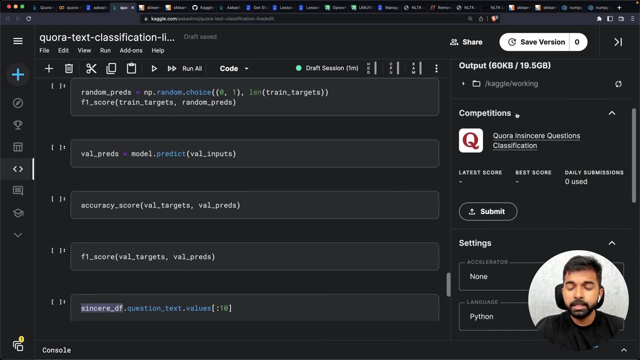 loaded properly. So, indeed, all the data is loaded properly. Great, Now we can go down. We can keep running all the code all the way down, but we don't have to do it As long as we have this notebook. and you scroll down here, you see that. 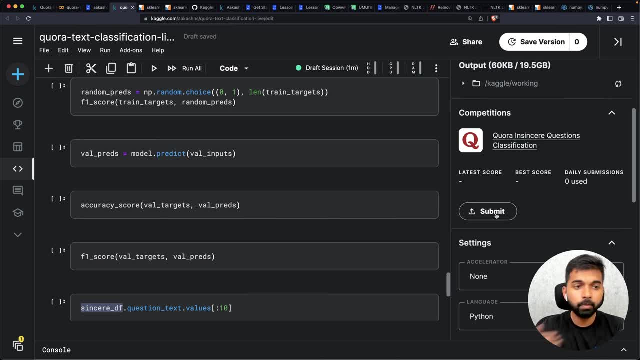 it is connected to this competition. It shows you an option to submit this notebook to the competition. So if you click submit, what's going to happen is Kaggle is going to run this notebook from top to bottom. It is going to generate a submission file, because we have some code at the end to 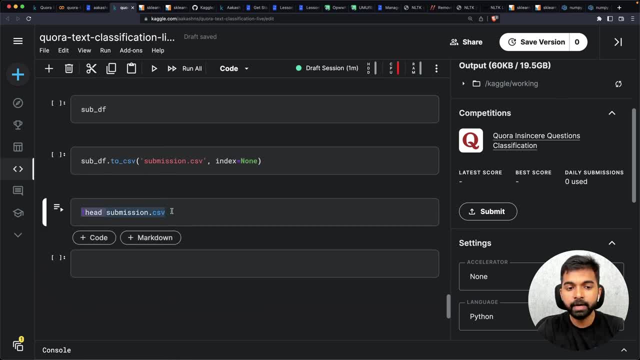 generate a submission file and then it is going to look for that submission file in the generated output and it's going to submit that submission or CSV file directly to the competition. Okay, So before I hit, submit one last thing. if you go down here, you will see that internet. 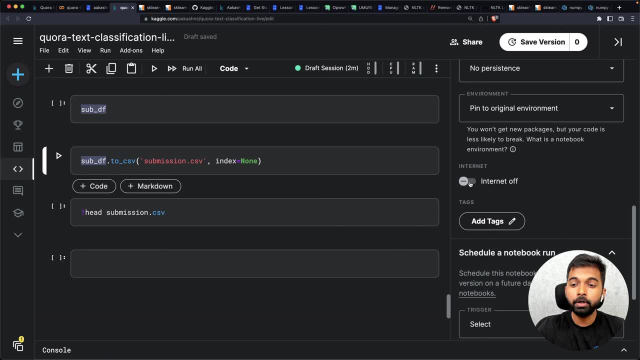 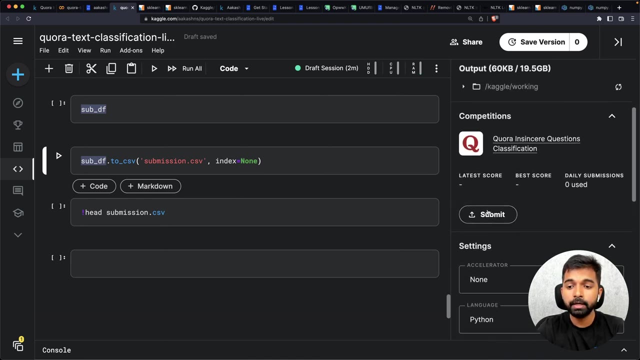 is turned on currently in this notebook, you will have to turn off internet because this competition specifically does not allow Kaggle notebooks which can connect to the internet, because this competition does not allow using any external data. So you need to turn off the internet and then you can go in here and you can click submit. 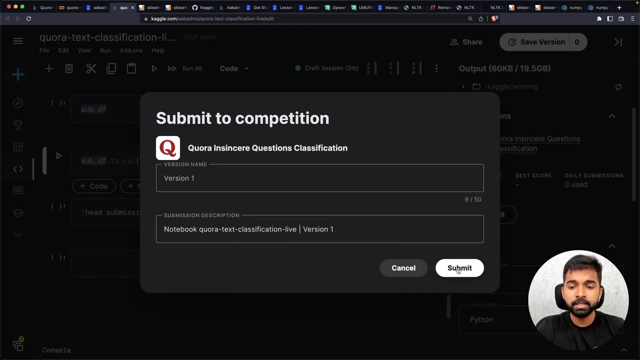 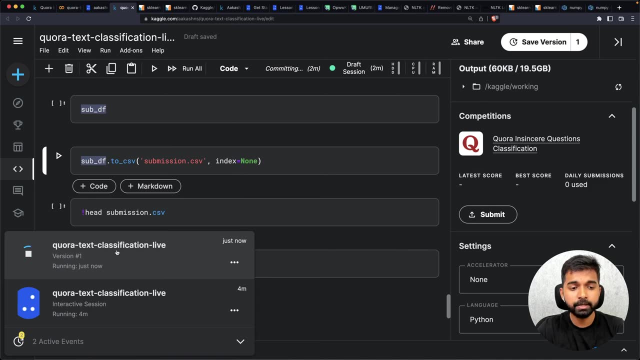 And now we are submitting this competition, Now we are submitting this notebook to the competition So you can actually see the status of the submission, You can actually go in here. Once it starts running, you can go to the next tab so you can open it up in a new tab and you can see. 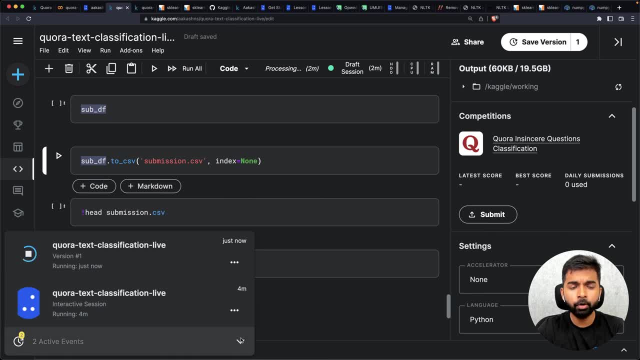 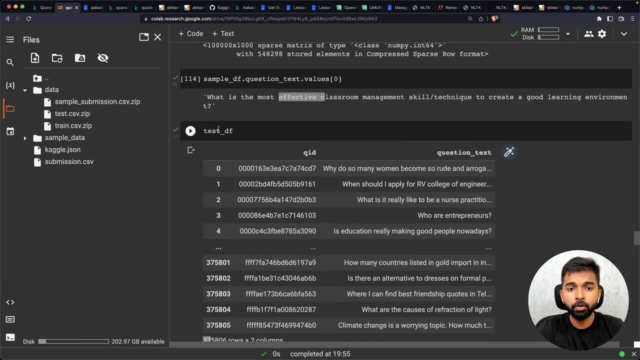 The logs from the execution. Okay, And you can continue to edit the notebook and save new versions and make more submissions. But the idea is just to repeat: you take your notebook, which is present on Colab, You save it so that it comes back to Jovian. 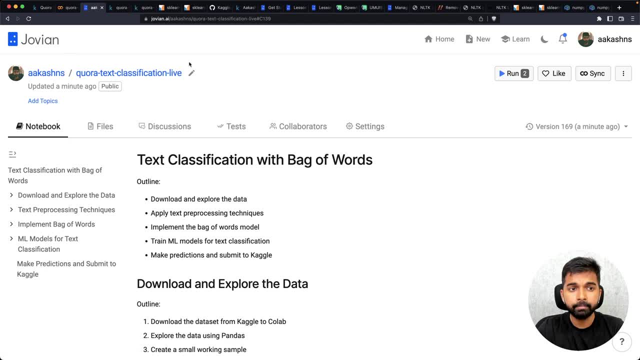 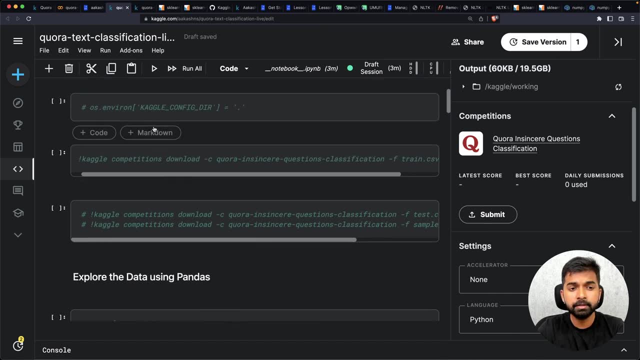 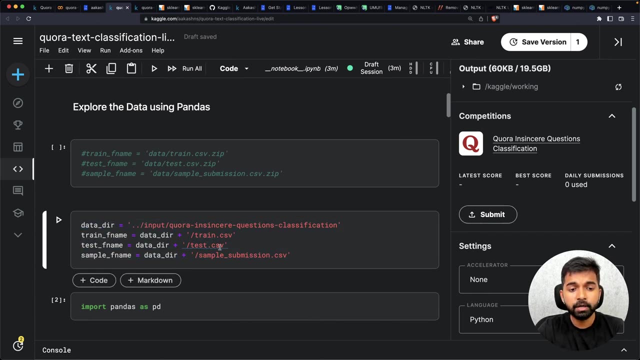 Then you run that notebook on call on Kaggle and on that Kaggle notebook you go ahead and you remove the code which has the data download code And instead you can add some code Which is going to just refer to the right data directory on Kaggle. 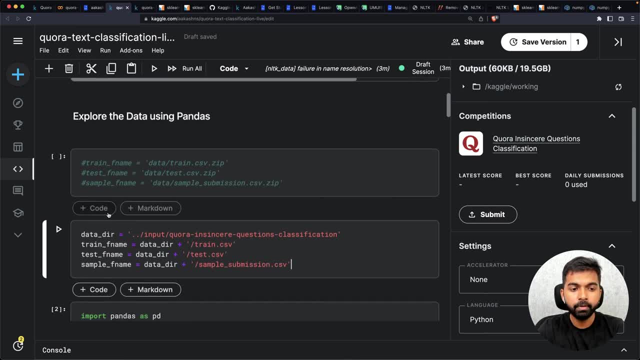 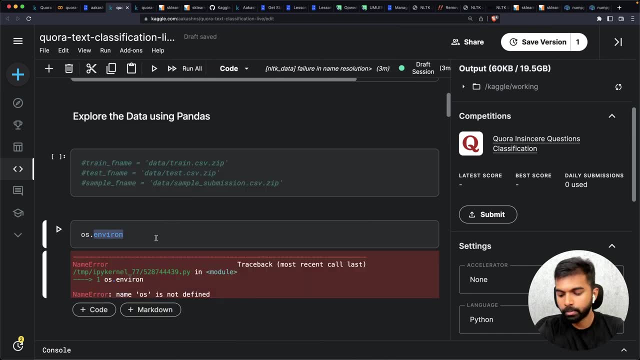 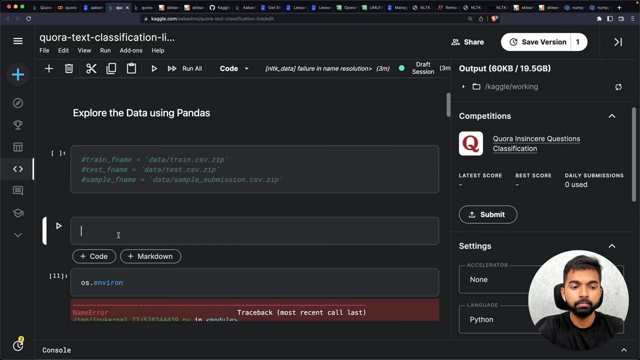 Now I want to show you a quick trick here While our submission is being processed. If you just check osenviron on Kaggle, Okay, I'm just going to import OS as well. Yeah, If you just check osenviron on Kaggle. 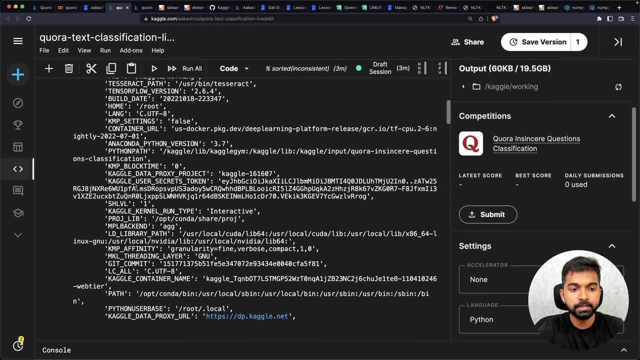 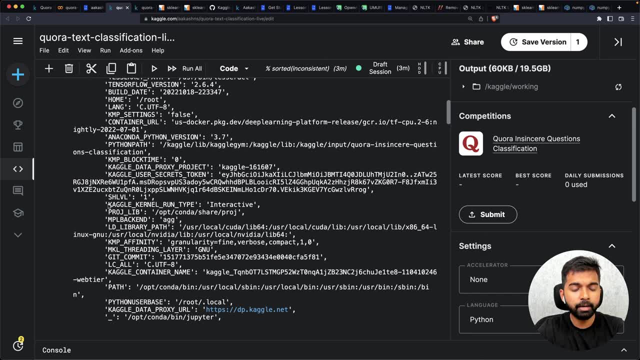 Yeah, If you just check osenviron on Kaggle. Yeah, If you just check osenviron on Kaggle. If you just check osenviron on Kaggle, It has certain Kaggle specific environment variables. For example, let's see Kaggle kernel run type. right, 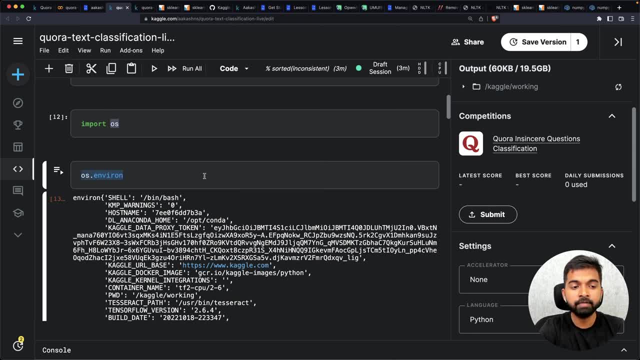 So it has this environment variable. So you can check for the presence of this environment variable, to check if you are currently within a Kaggle dashboard or not. So you can say something like: is Kaggle equals Kaggle kernel run type in osenviron. 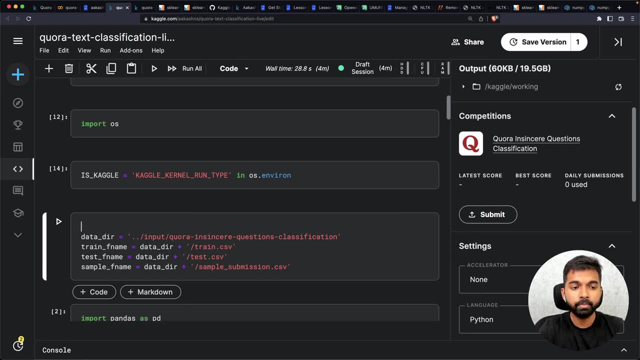 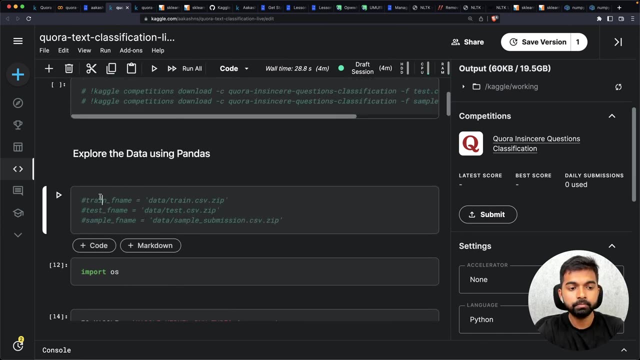 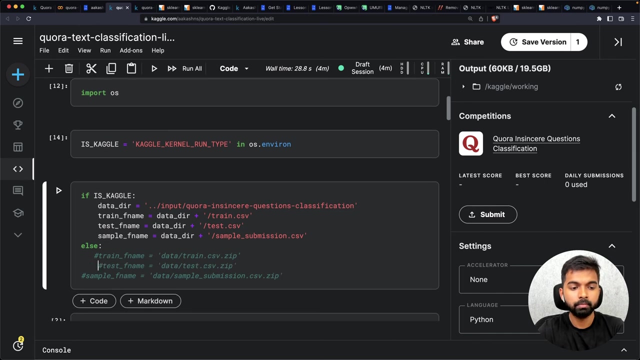 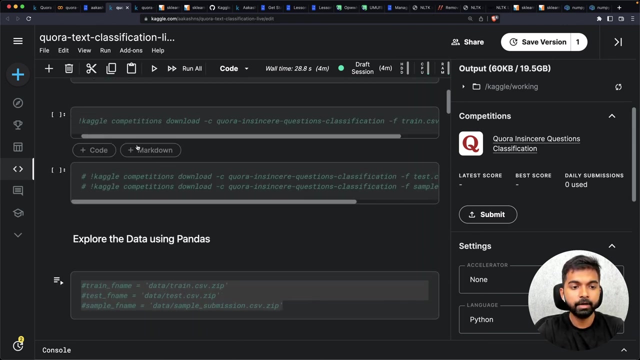 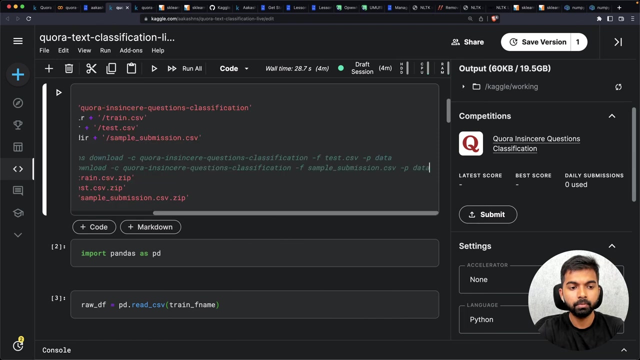 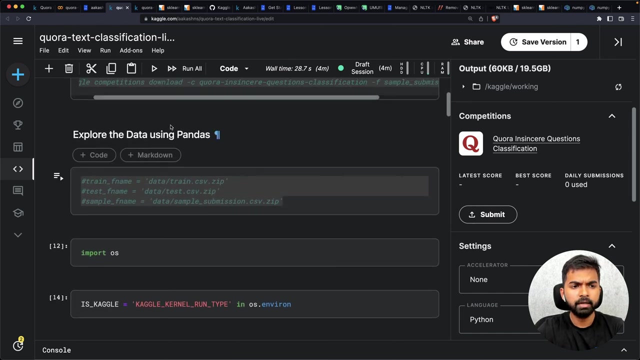 All right, And then you can do something like this. You can say: If is Kaggle and do all this else, let's get all this code, Let's get all this data download code as well, And let's get this last data download piece of code as well. 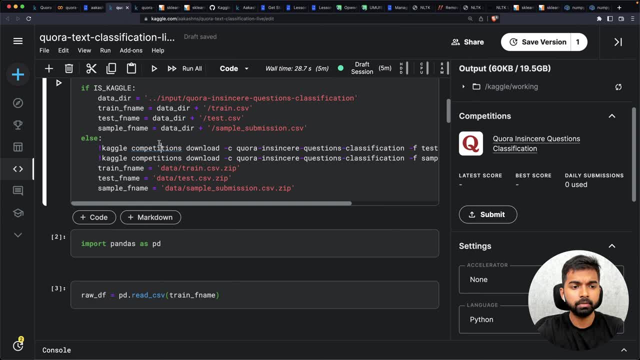 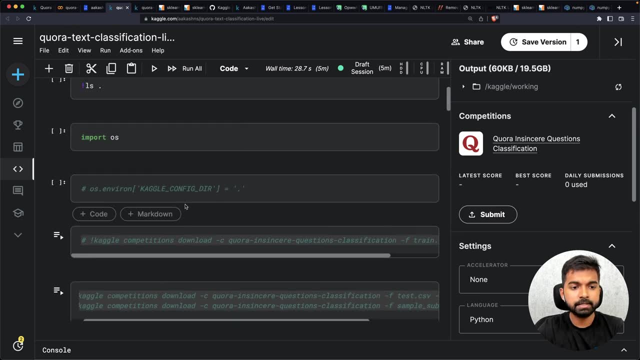 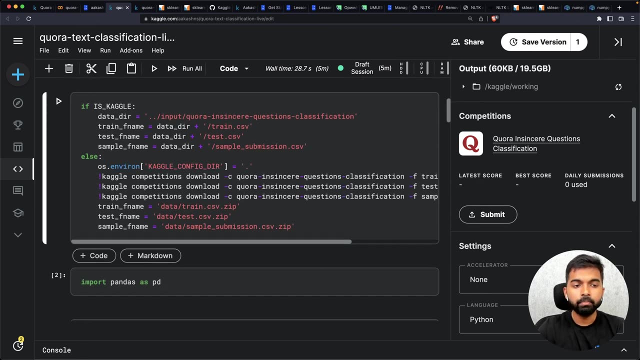 And I believe we also need this last cell where we configure the Kaggle conf director, And I believe we also need this last cell where we configure the Agile conf directory. So, just with this one line of code, or this one cell of code, we are checking whether 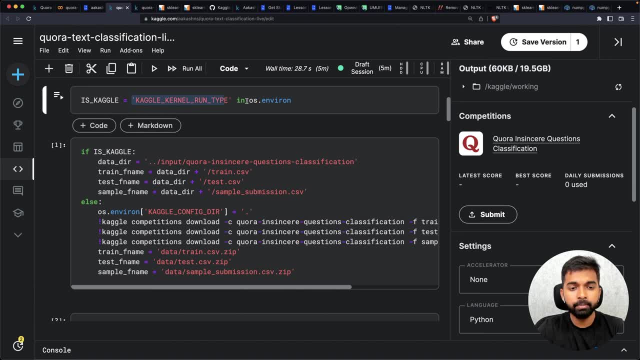 we are currently in Kaggle, by checking Kaggle kernel run type whether that environment variable is present in osenviron. If it is, then we are in Kaggle notebooks, If not, then we are in Colab or wherever else, And if we are in Kaggle, then we simply set the data directory. 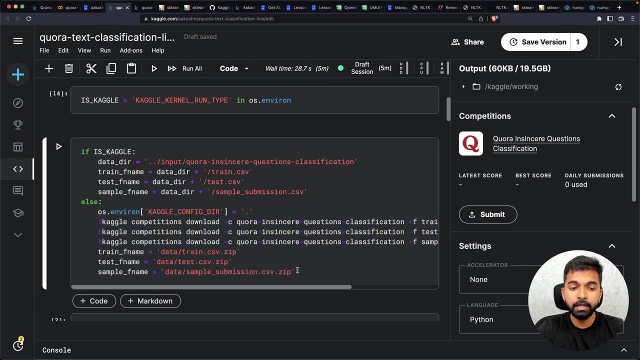 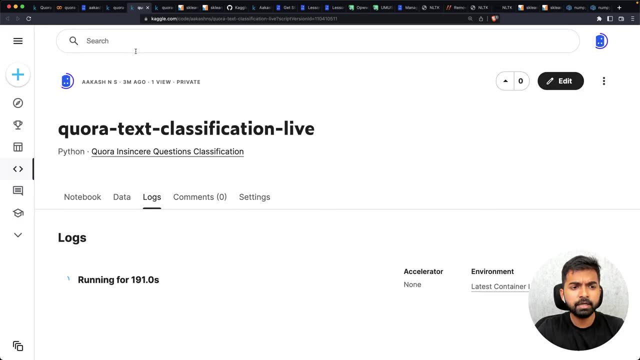 If you're not in Kaggle, then we first download the data and then we go ahead and work with it. So that's one quick trick that I wanted to show you. but let's see, this notebook is still running. Let's see if it has run. 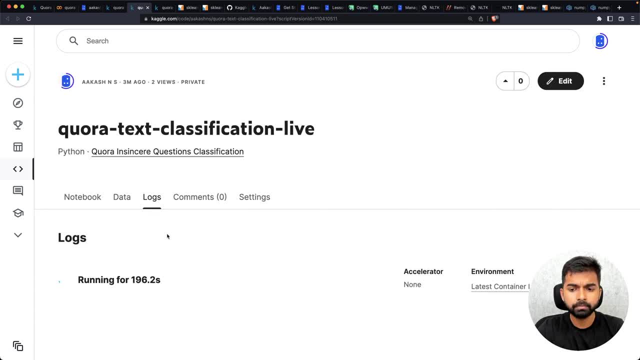 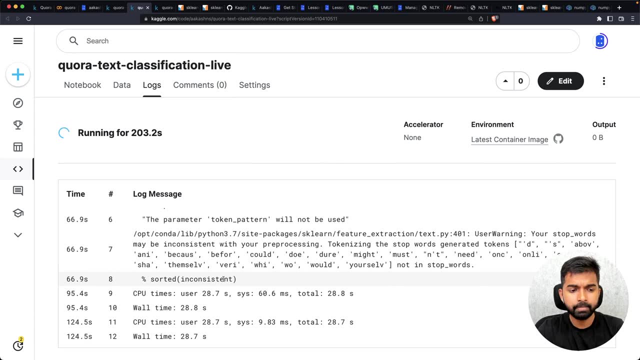 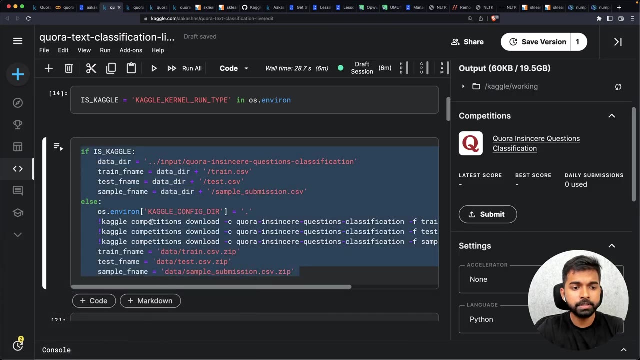 Let's see if there are any logs for us to review. Yeah, So there are a bunch of logs, but it looks like it's still running. So, in the meantime, here's one last thing that I'm going to do. I'm just going to take all this code and put it back into my Colab notebook right at the 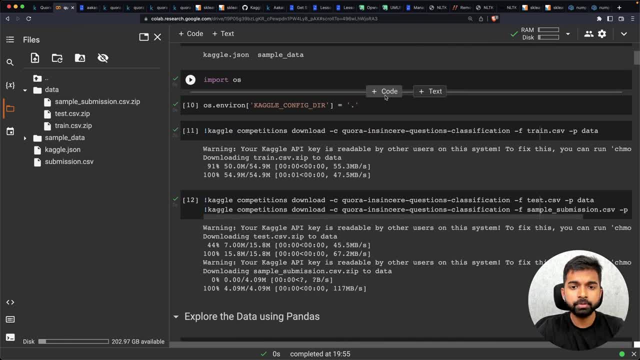 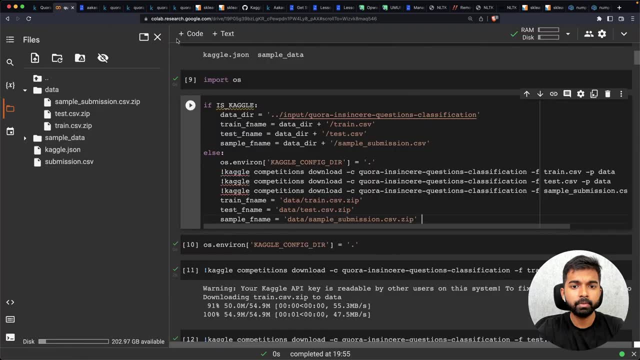 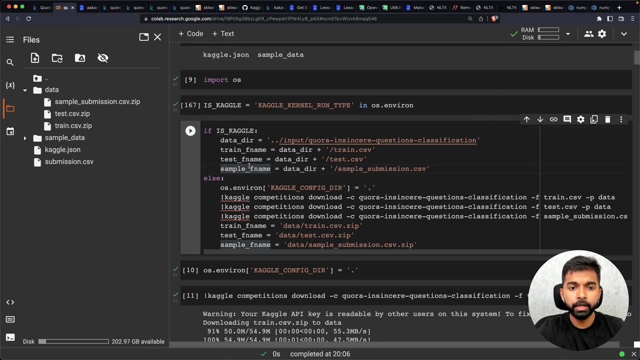 top. So I am just going to put in here that and I'm also going to put in this. So now I have this code is Kaggle, And then I have this code for downloading from the data directory and I can try running it again, just to make sure that it runs fine. 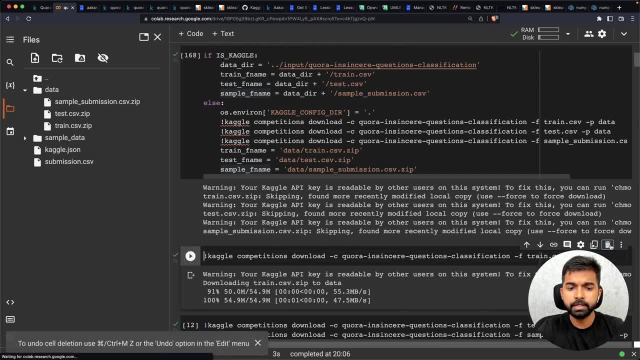 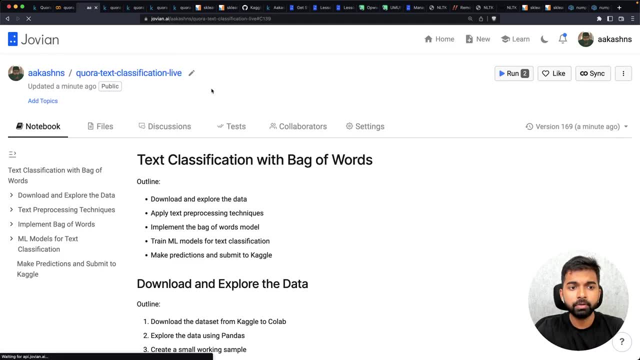 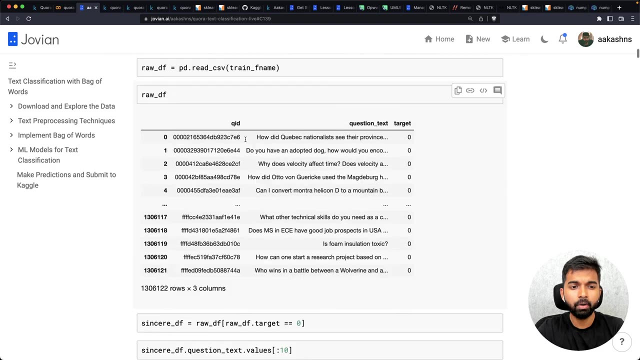 Yeah, it looks like it runs fine. So then I can get rid of all these. Okay, Okay, And once I save it, So the data is going to come back here on Jovian as well. Yeah, So now you can see here our code contains all the Kaggle related changes as well. 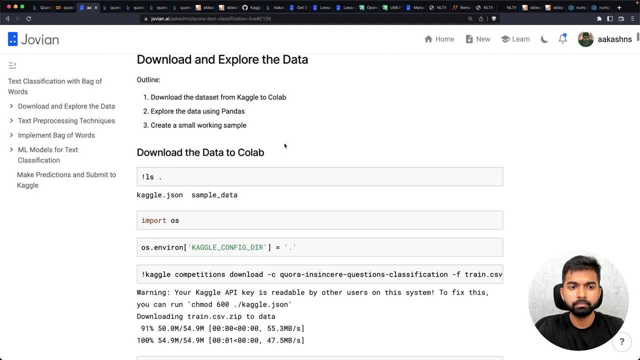 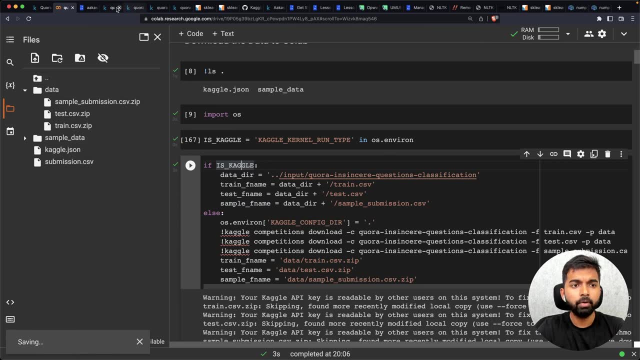 Okay, Not yet. Maybe the next time we save it. okay, Let's see if this notebook is executed. It's still running. Maybe it's still going to take a little more time. Okay, Let's see if we can run it again. 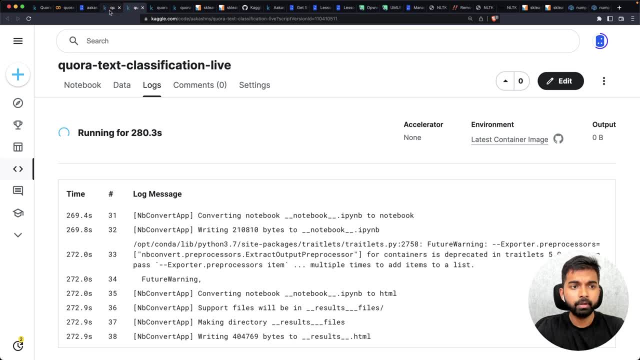 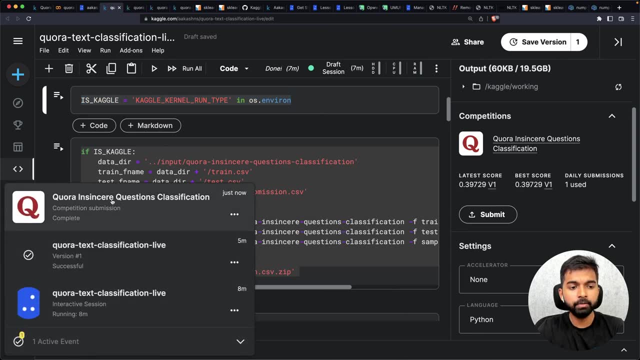 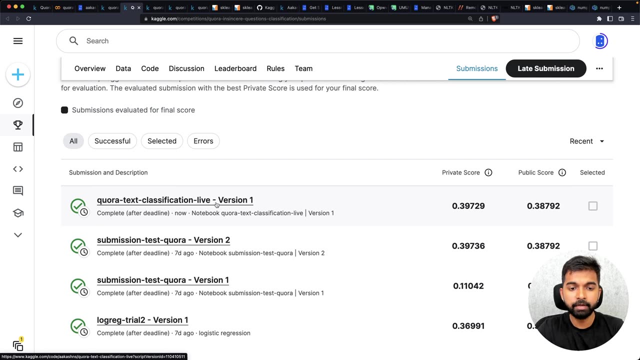 Yeah, It looks like the results are almost out. So when you yeah, so now it says save and run complete, you can see that it's now submitting to this competition. You can click to check the submission. So now this submission was made. Cora text classification live version one, and I've 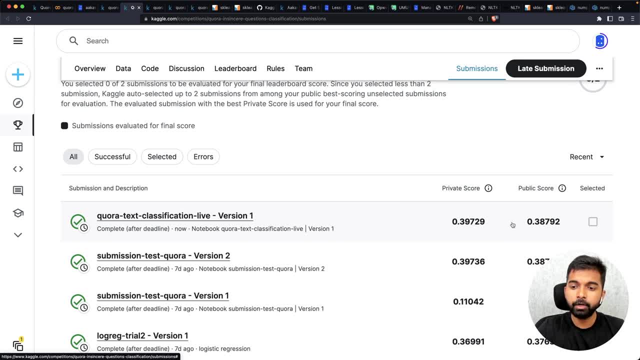 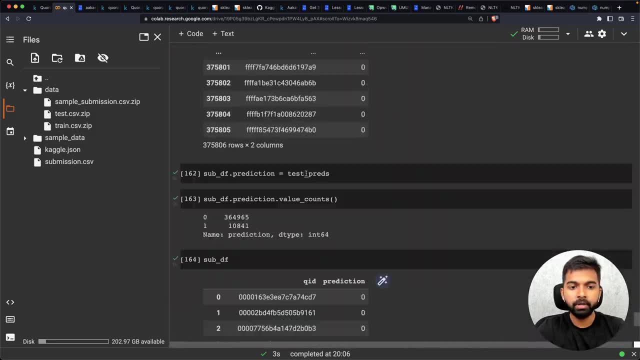 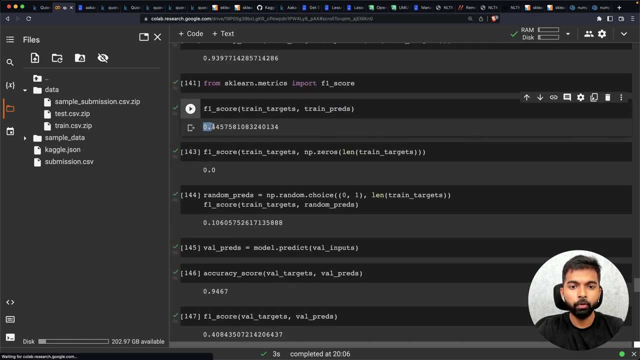 made some submissions before as well, but you can see that this submission led to a score of 0.3729.. So, coming back to my notebook, Remember here, on the training set, the score was 0.44.. On the validation set, the FN score was 0.40. 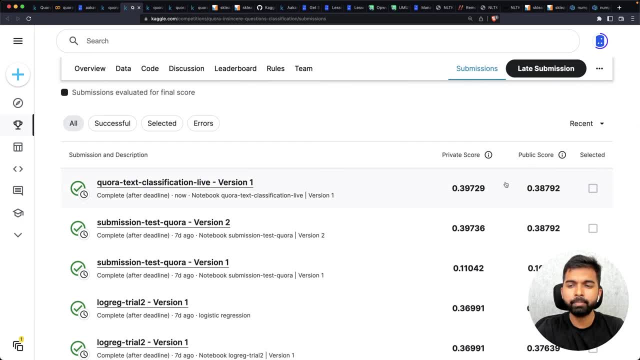 And on the test set. finally, when we made it made a submission, So there's a private leaderboard and publicly the board. the test set itself is split across a private and public. but on the test set, my score is 0.39. 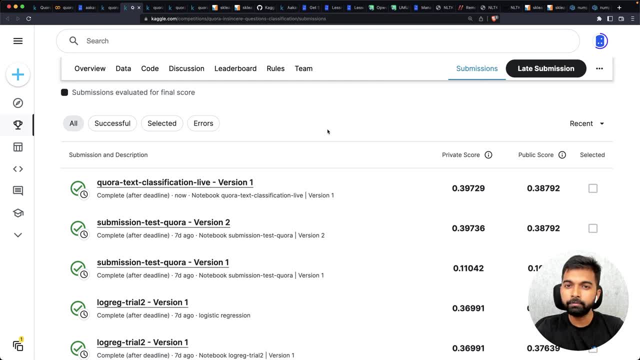 Well, so these three scores are not too far off 0.39.. 0.44 is higher than 0.40.. That is expected, because you have training data, You have some overfitting, you have some memorization of data. 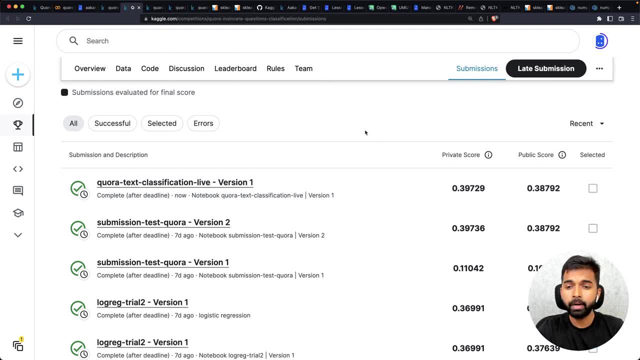 Then you have the test data set- 0.39, which is slightly worse than the validation set, but it's close. This is something that you should ensure before you try to build more advanced models: that your validation set and test set have similar scores roughly. 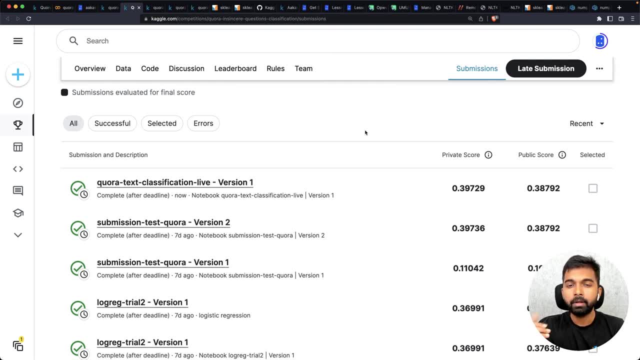 And your validation set is slightly worse than your training set. Now how much worse your validation set is compared to your training set. It can help you determine how much overfitting there is and how much hyperparameter tuning you may need to do. So all of those things are things that you'll have to keep in mind when you train a proper 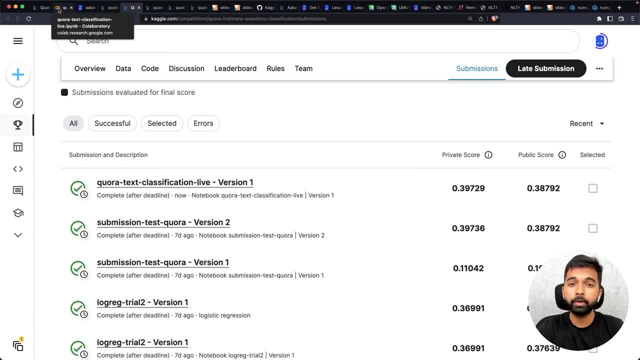 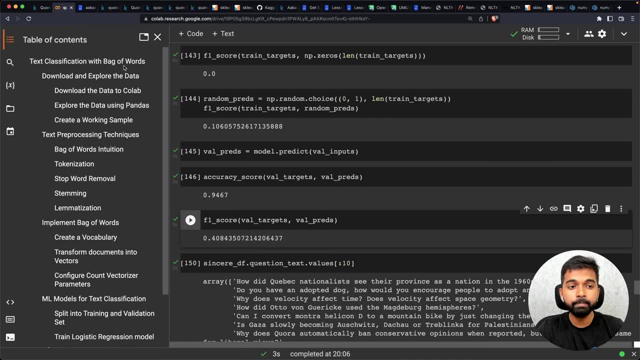 machine learning model for a real world dataset, And that is something that we'll continue to look at in future tutorials. Now just to recap everything that we've done today and everything that we've done today. So we looked at text classification with bag of words and we looked at that by looking 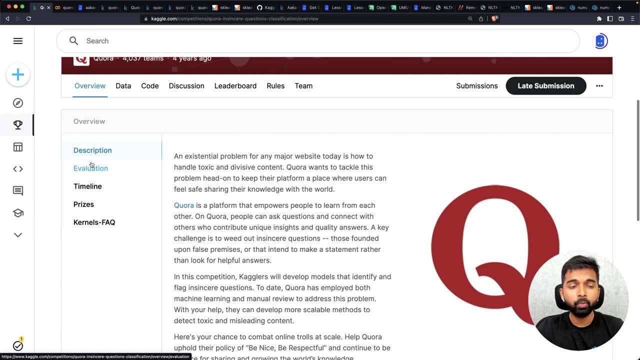 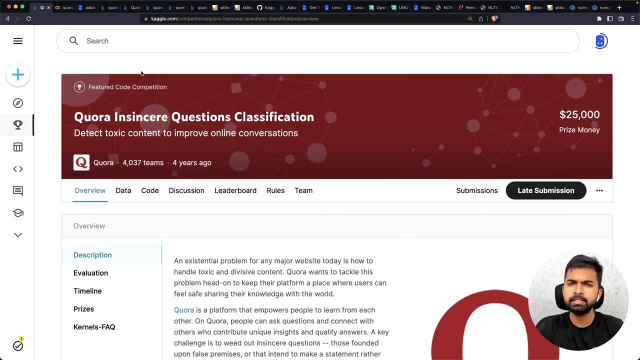 at the Cora insincere question classification Where, Where? So we are given questions. We are given 1.3 million questions and they are given labels zero or one zero meaning sincere and one meaning insincere. about 94% of them have the value zero, which is that. 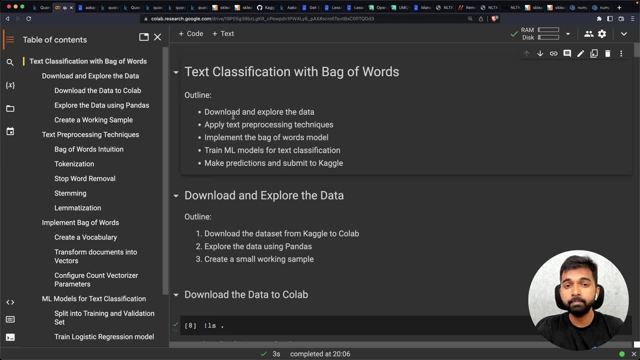 94% of them are sincere and about 6% are insincere. We have to train a model which can automatically classify questions at sincere and insincere, And we are given a test set on which we have to make predictions and submit it to Kaggle. 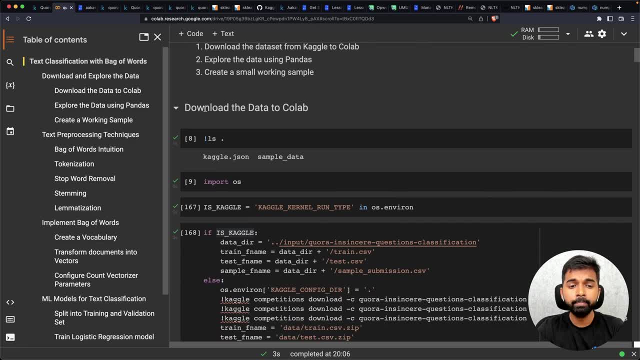 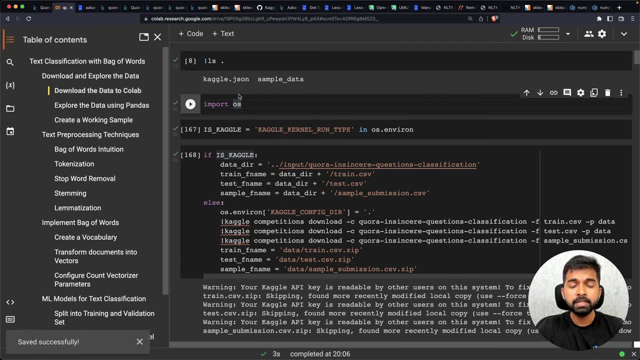 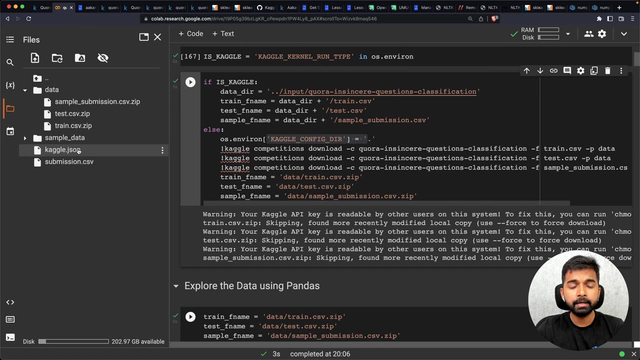 So the way we did this is by starting to Download and explore the data. now, on Google Colab, The way we downloaded the data was by simply setting this Kaggle config directory, adding that Kagglejson file in our Google Colab by uploading it. 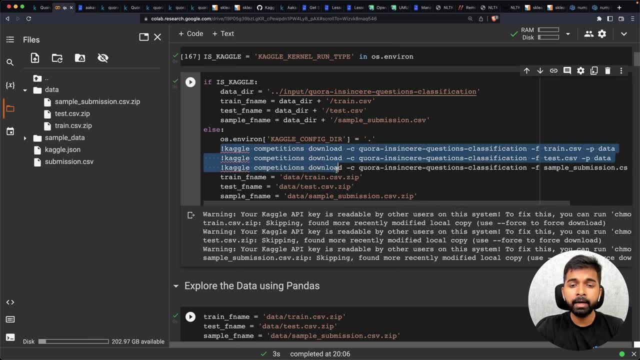 It is downloaded from our Kaggle account, Then using the Kaggle command line tool to download the train files- test file and sample submission file- And then finally creating these file name variables that we could use later. Then, after these files were downloaded, we loaded them up using pandas. 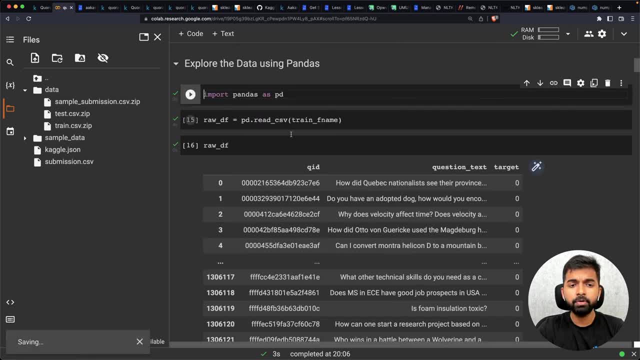 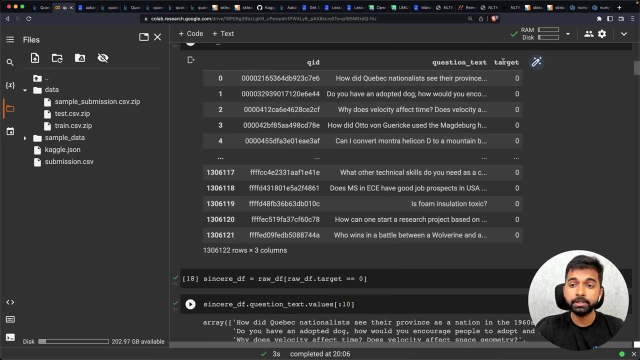 So we loaded up these files. I think this is not required anymore. So we loaded up these files using pandas And we saw that there were 1.3 million rows and we had three columns: QID, question text and target. 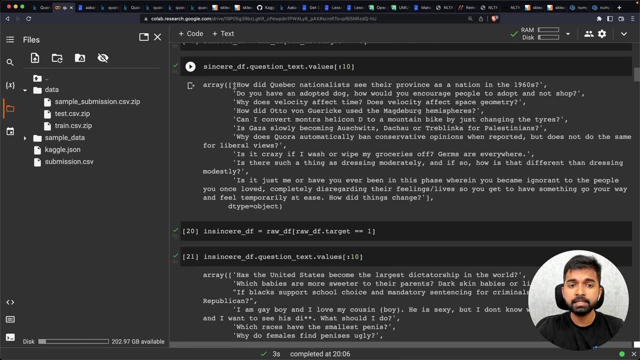 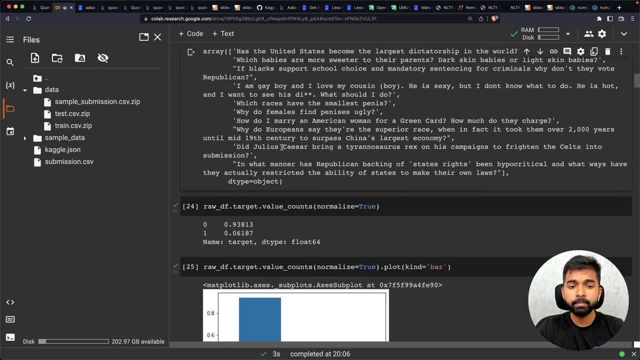 The targets could be zero or one zero, indicating insincere. And these are some sincere questions. Questions look good. These are some insincere questions, clearly questions with a lot of problems, And we saw that about 94% of them were sincere. 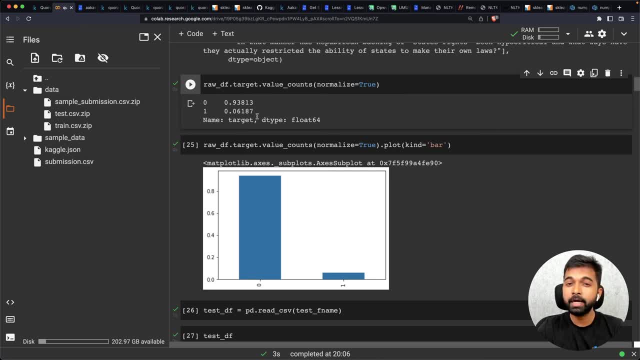 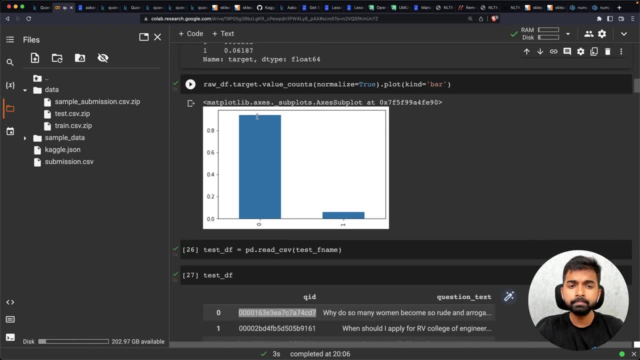 94% of questions are sincere and 6% are insincere. That is why accuracy may not make sense as a metric, because you can get 94% accuracy just by predicting, predicting zero all the time. And then we looked at the test data frame, which contains about 375,000 questions, which 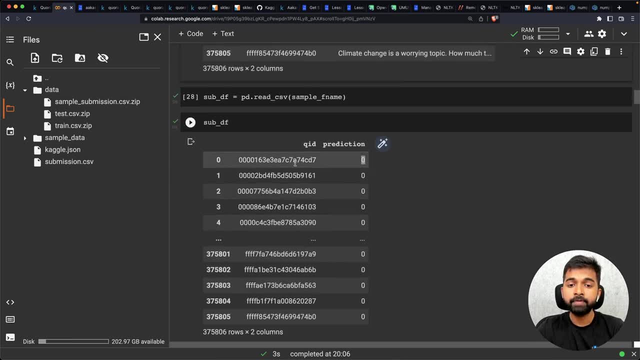 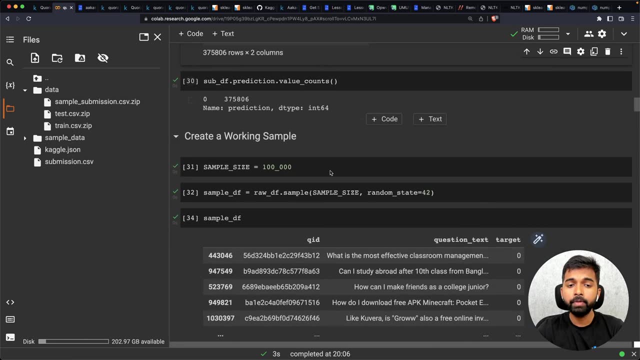 do not have any labels. So we have to create a submission file where we put in predictions for each of the questions in the test set And then we have to submit that prediction to Kaggle. The way we do that is well. first we created a working sample. 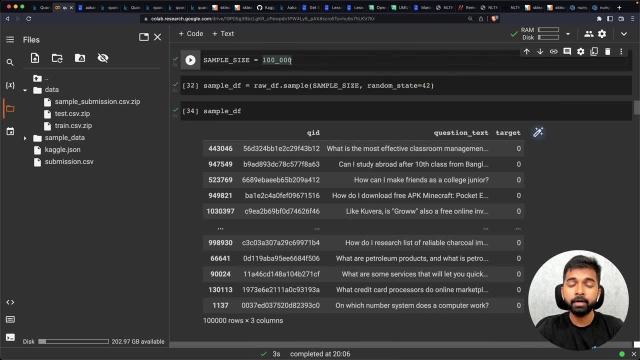 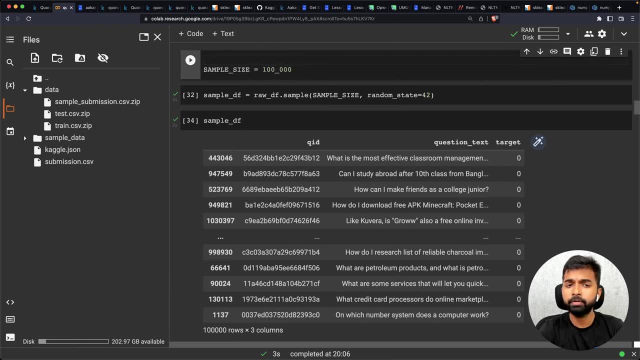 From the raw training data frame. we picked a sample of a hundred thousand. Now one thing you may choose to do is, while submitting to Kaggle, change this working sample size to maybe 1 million or the full data set. So you could do something like: if is Kaggle. 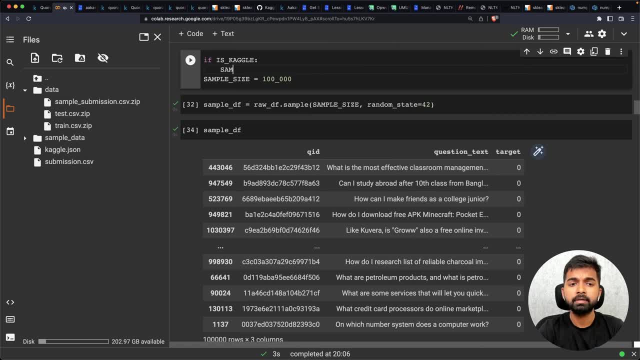 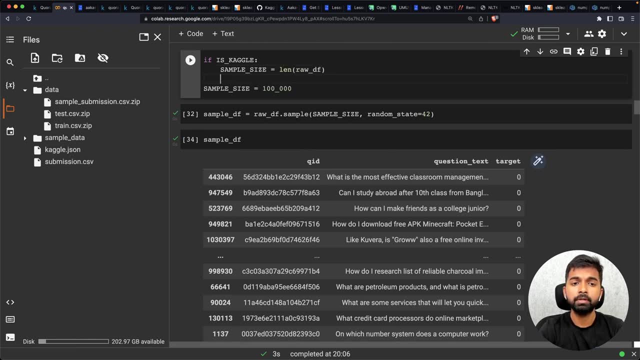 Then you could say: Sample size equals len RawDF, which is just the full thing. else, Just use the entire time. I just wonder how it will work this way. use a hundred thousand. So that's something that I'll leave to you if you want to try that out. 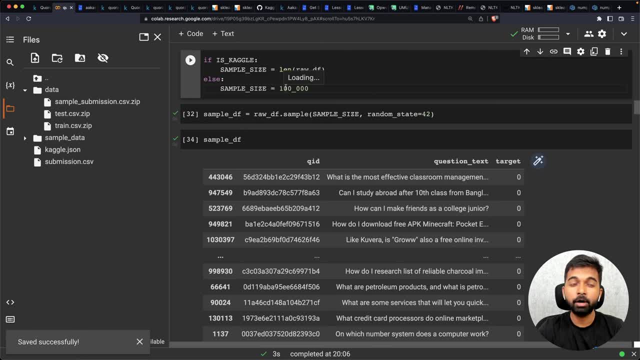 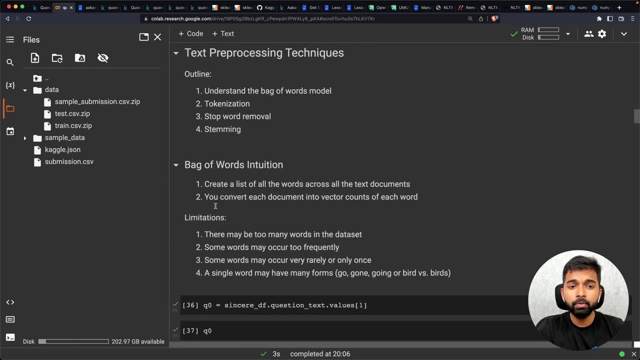 And one thing I encourage you to do is run it on the entire data set and see how much better the result gets. Now in the sample data frame we have picked a hundred thousand rows, And the way we are going to use the sample data frame is going to create bag of words vectors. Now the way bag. 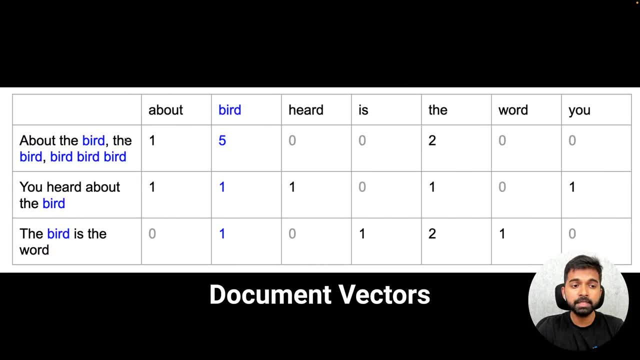 of words works is by creating a list of all the words across all the text documents. So if these are the documents, we create a list of all the unique words and then we turn each document into a vector using the counts of each word in that document. The limitations that are. 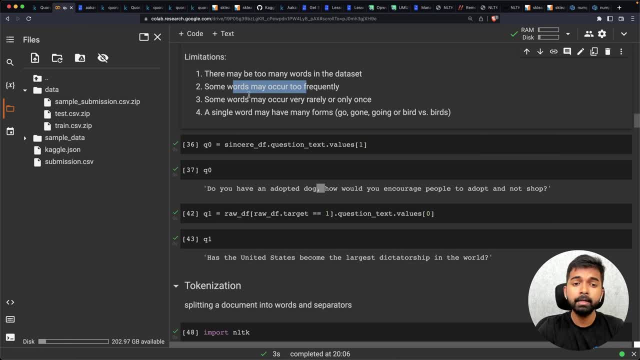 there may be too many words in the data set, Some words may occur too frequently, Some words may occur too rarely, and a single word may have many forms. So all of these make it a little impractical to use bag of words directly. That's why we perform a bit of 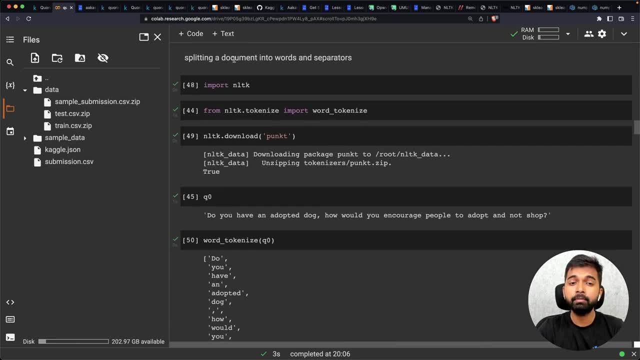 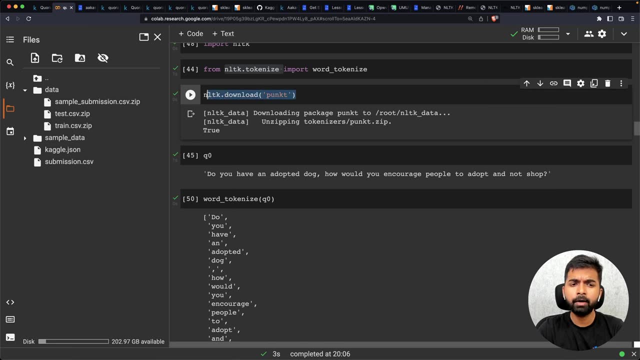 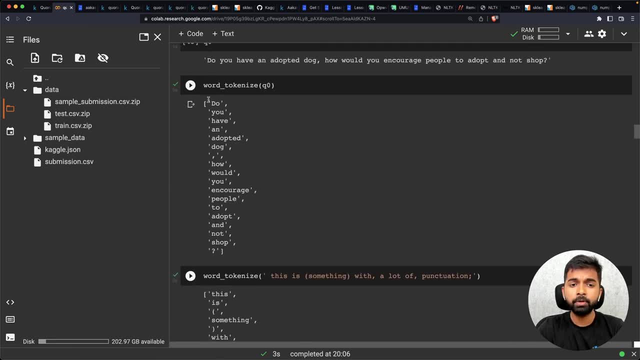 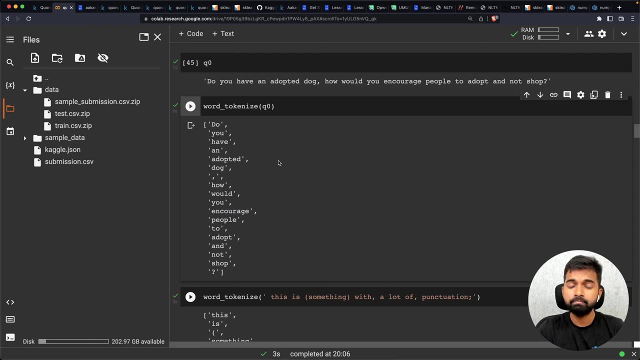 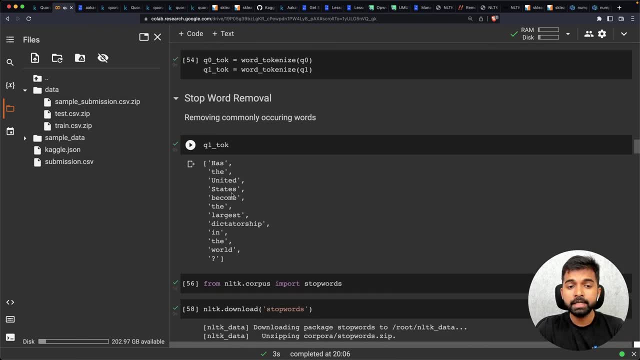 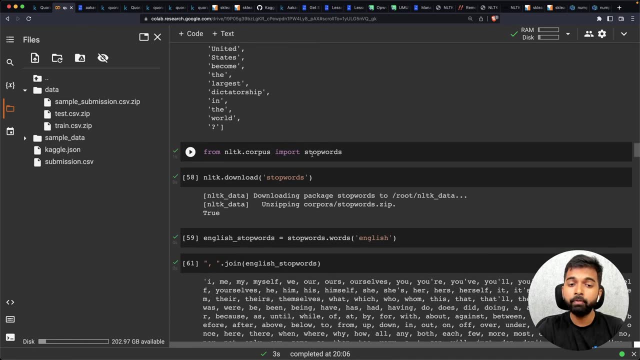 And this is an example. After doing tokenization, one thing that we do is we remove commonly occurring words like a and the not, et cetera. So for this we use the stop words corpus from NLTK. Specifically, we use the English stop words corpus. Now, keep in mind that the English 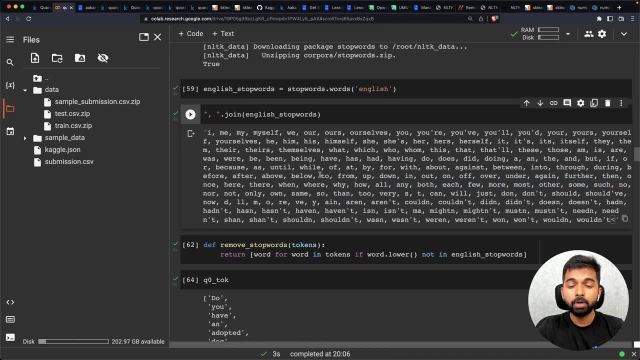 stop words corpus can contain a bunch of stop words that you may want to keep, things like not, haven't, hasn't, et cetera, especially for things like sentiment analysis, where those words can convey a sentiment. In this case they don't matter too much for us, but you can try with and. 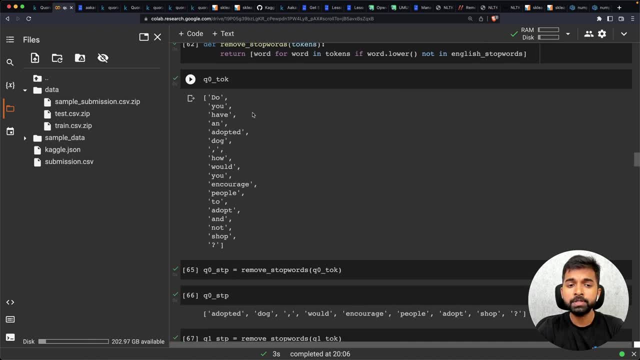 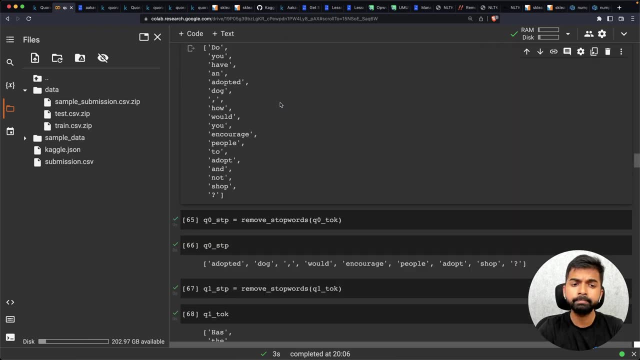 without some of these stop words, And after removing stop words, a lot of the words go away. We may have to be careful that we lowercase the words before we remove stop words, So that's why we have a helper function here. And then we do another thing called stemming, where we take the 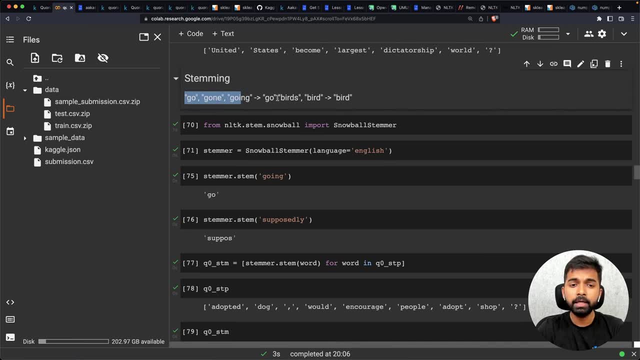 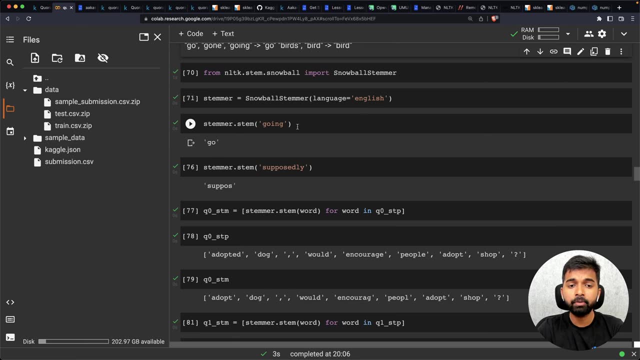 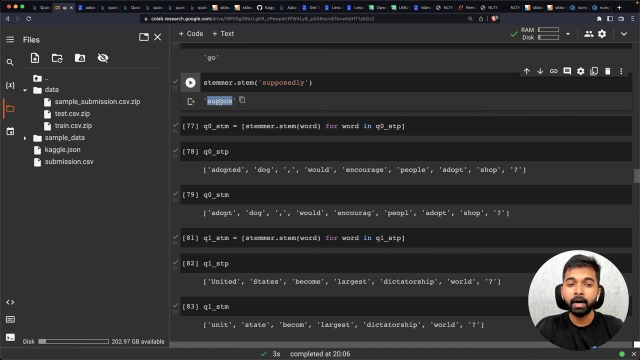 words like go, gone, going, and we reduce them to their root form, like go or birds. bird can be reduced to bird, So we use the snowball stemmer for the English language, and this is how it works. Now notice that stemming does not always create sensible words, because it is based on a hard coded. 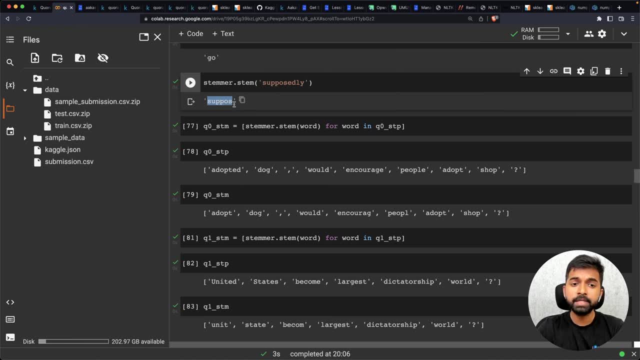 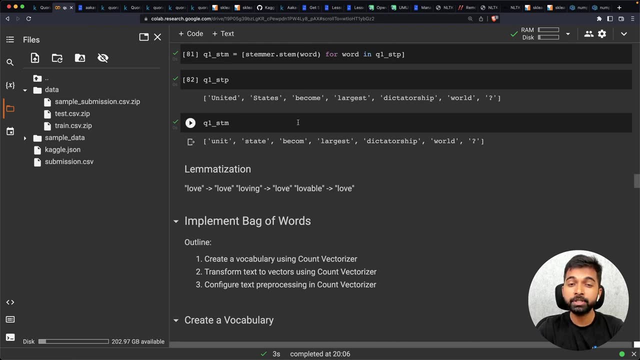 algorithm. It is not looking up a dictionary, but that is what makes it really fast. On the other hand, there is another technique called lemmatization, which will give you meaningful words from the dictionary, but that is very slow And something that you may want to avoid for a large dataset. So here are some stemmed examples. 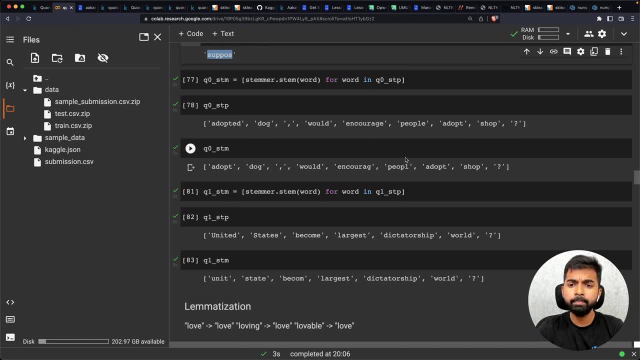 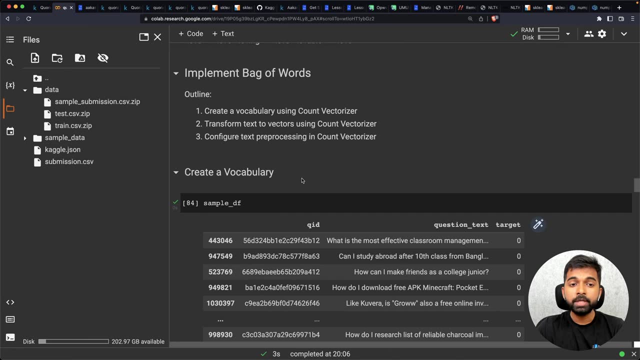 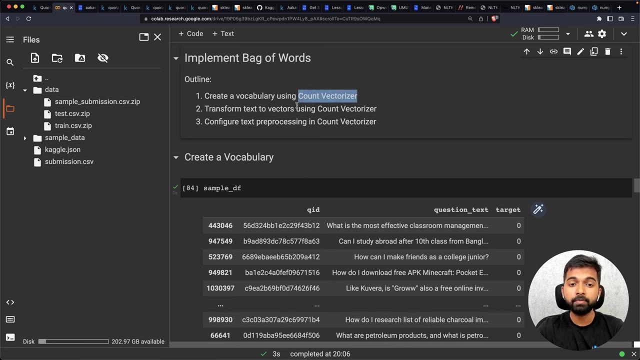 Adopted becomes adopt, encourage becomes encourage without an E. And similarly, let's see states become state. Now, once we have all these reprocessing techniques understood, we can then implement bag of words using the count vectorizer class from scikit-learn. So first we created a sample of just five. 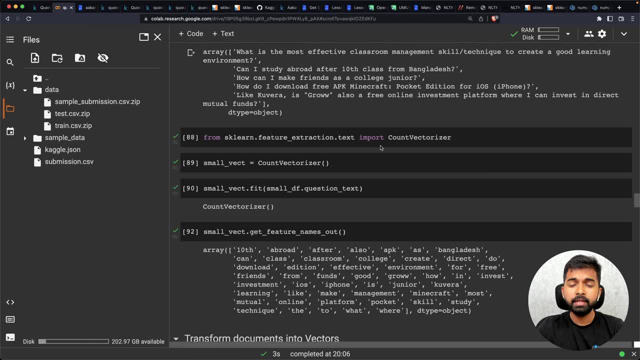 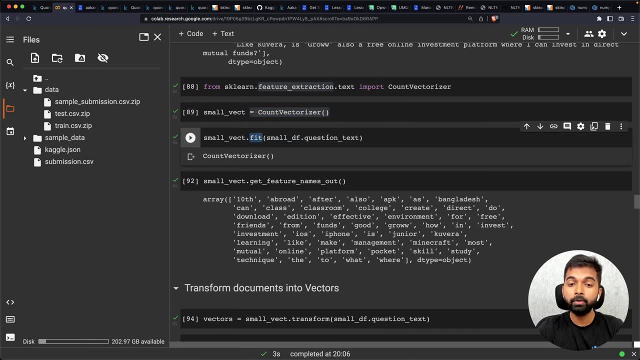 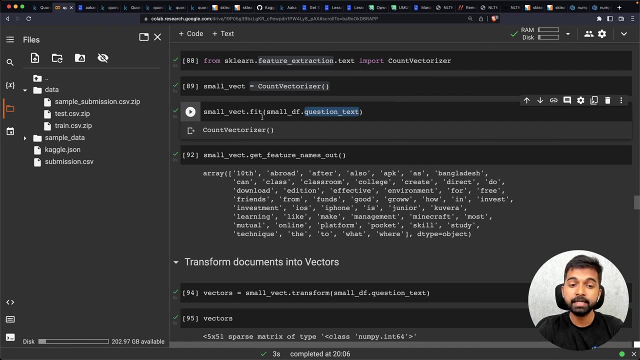 questions. These are the five questions we took a sample of. Let's write down, Then we load them to our So we took our first question, then we imported count vectorizer from S K: learn 수가. that feature extraction or text. 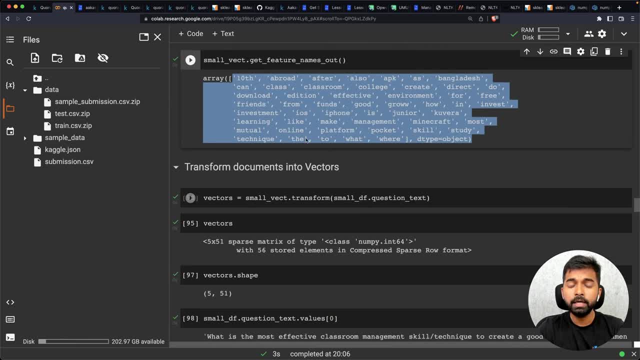 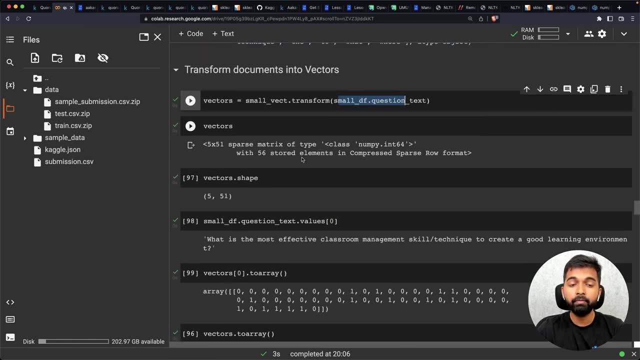 We created the concrete riser and then we fitted it to the question texts. by fitting, We simply find out the list of all the words that are present in the vocabulary, in the entire data set, And I'd give us a vocabulary. Then we use the. 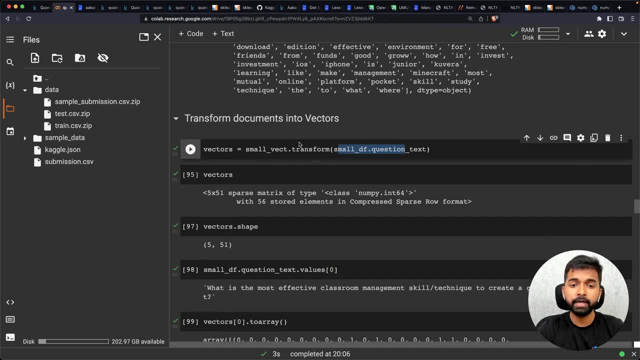 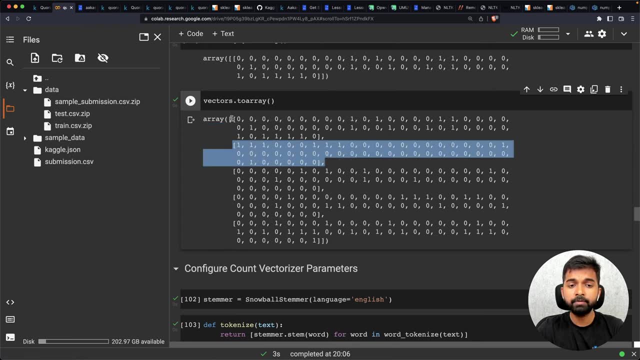 fitted model, The fitted count vectorizer, That way or not vector, that is done by using a small vec, dot transform, And that gives us vectors for each of the five questions. And these vectors are of the same length as the vocabulary and the numbers in. 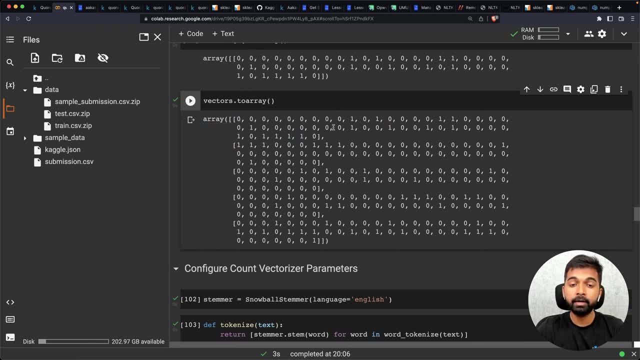 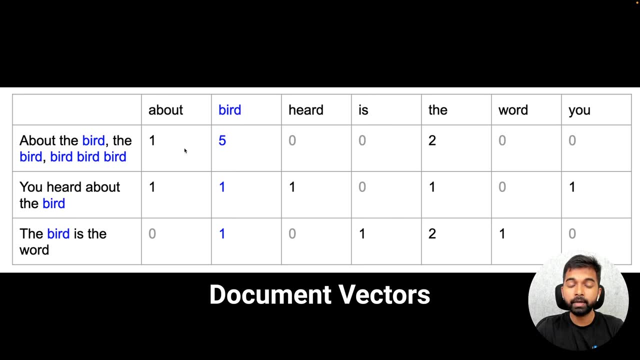 these vectors indicate how many times the words in the vocabulary occur in this particular text. Now remember that bag of words is not reversible. going from this to this is possible using count vectorizer, but given just this, you cannot recover the original sentence. 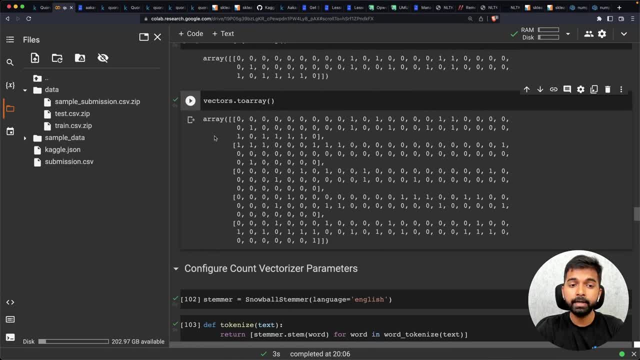 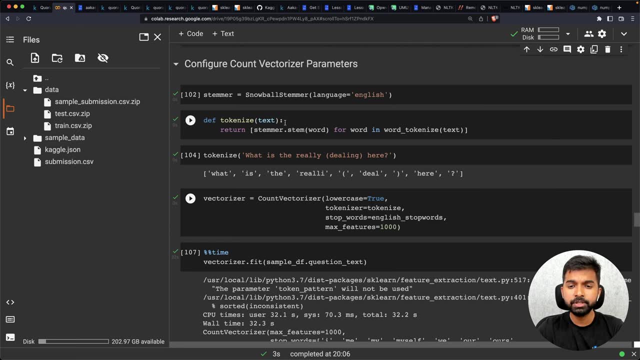 So keep that in mind, that it is a destructive operation. It's not completely reversible. Next, having understood how to use count vectorizer, we added stemming tokenization and stop word removal. So it contains its own tokenizer, but we defined a custom tokenizer. 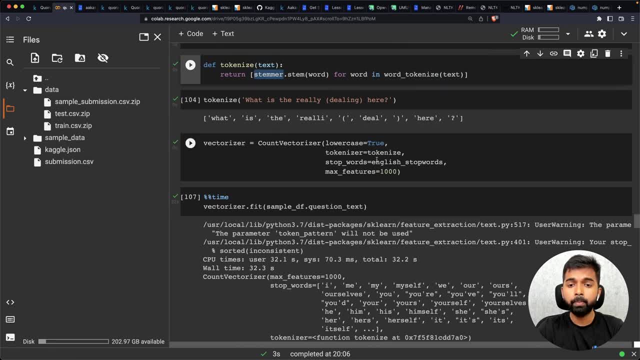 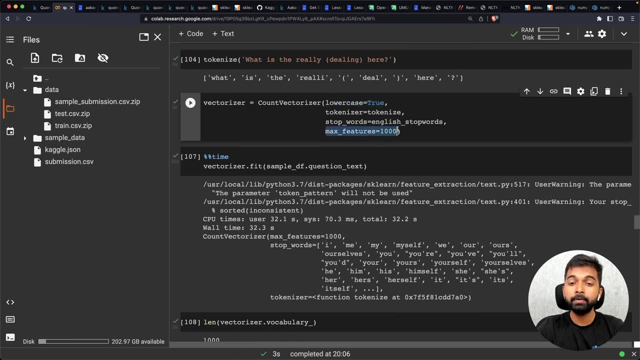 that also performs stemming. And then we also pasted a list of custom stop words And we also said that we want to lowercase the text And we also said that we want to limit the vocabulary to the thousand most commonly occurring words. Then we said: vectorizer dot. fit, sample df dot. question text. 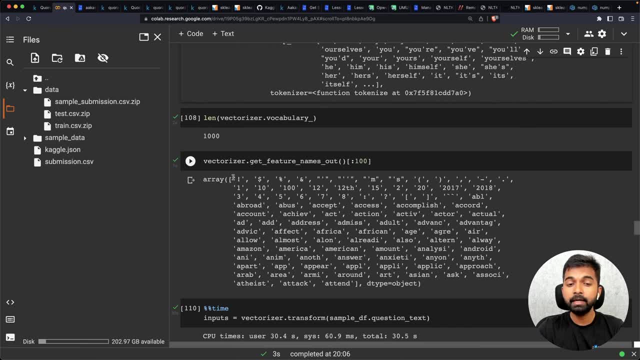 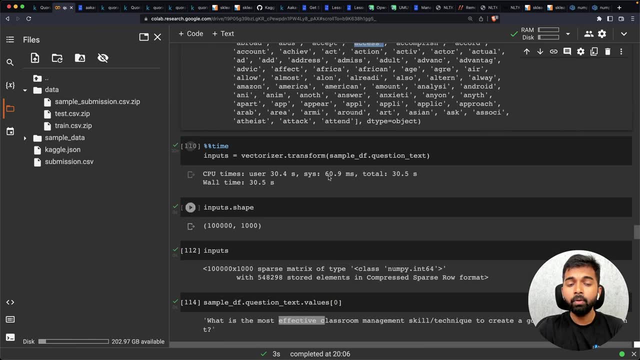 And that created a vocabulary of size thousand containing the thousand most frequently occurring tokens, And all these tokens are also stemmed and stop words have been removed. Now, using the vocabulary, using the trained vectorizer, we can take the entire sample dataset, which is about a hundred thousand questions and 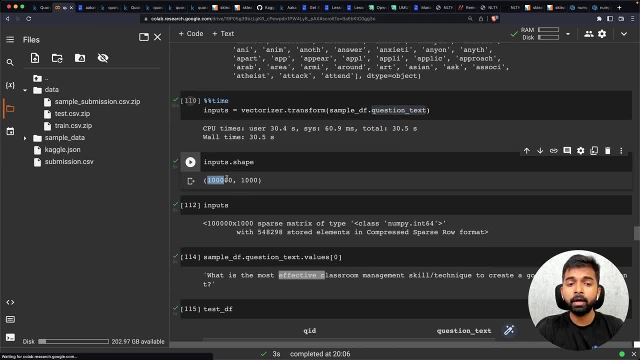 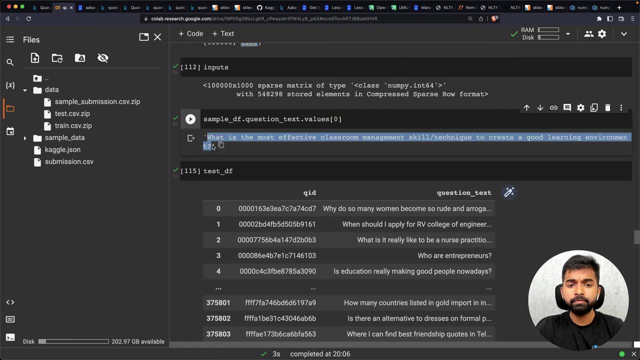 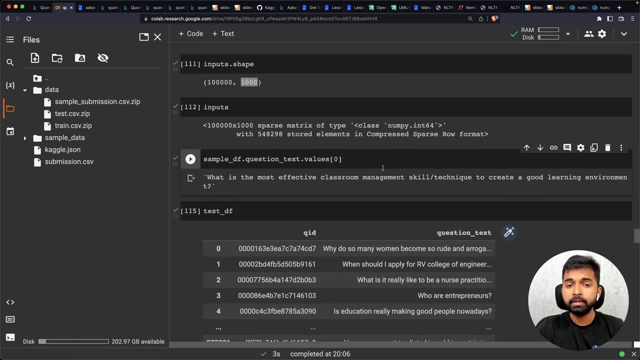 convert all the questions into vectors. So now we got a hundred thousand vectors of shape thousand. Now we could also look at specific vectors here. So this is the first question: What is the most effective classroom management skill? And when we convert that into a vector we can see that that vector 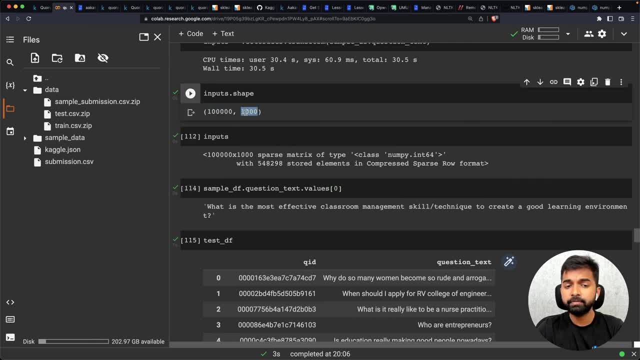 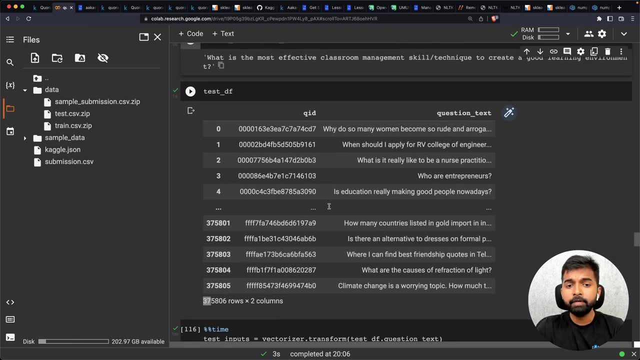 contains a lot of zeros because it's of vectors of length thousand, but a few ones in the places where these words occur. in the same way that we did for the training set, we can also do this for the test data frame, but remember that we should use the same vectorizer. 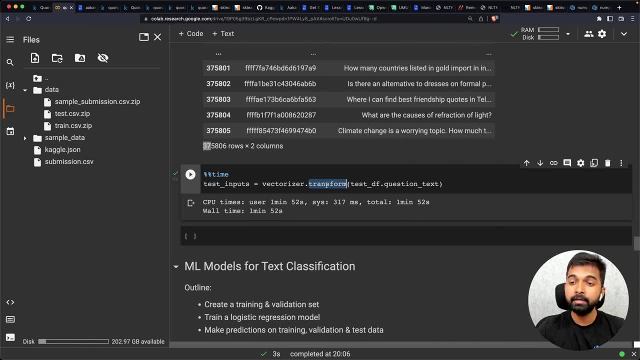 We should not fit the vectorizer on the test data frame, because then the vectors will no longer make sense. So any model trained on the Training inputs will not be able to make meaningful predictions on the test inputs. This is a very subtle but important point. 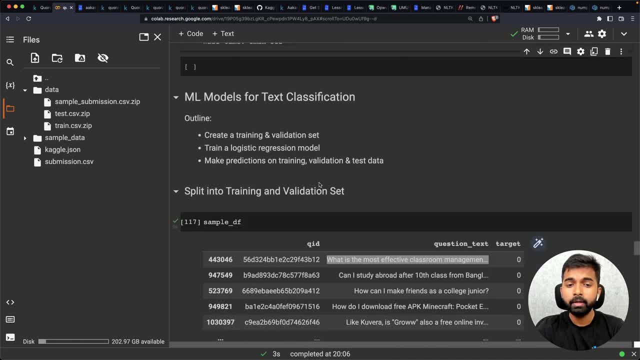 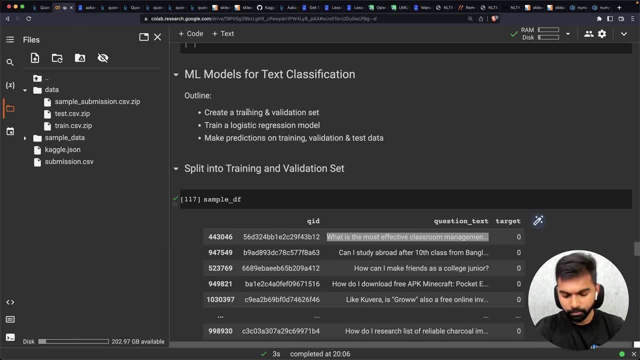 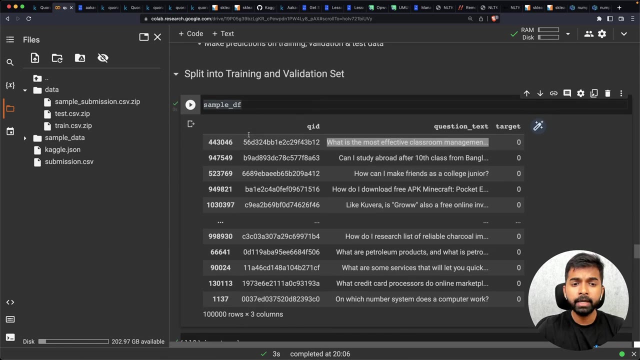 So think about it and convince yourself why this is important. Then we looked at how to train ML models for text classification. So the way we did that was first to create a training and validation set. So we took the sample data frame with a hundred thousand rows and we converted it into a, so we took the input. 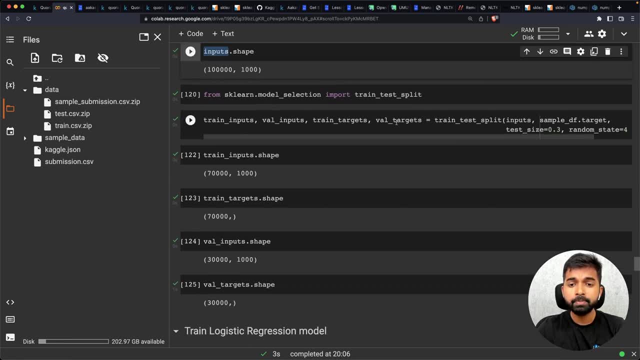 And we took the targets, which are simply the target column, and we split it into a 70% training set and a 30% validation set using train test split, to which we provided the set of input vectors, we provided the targets and we 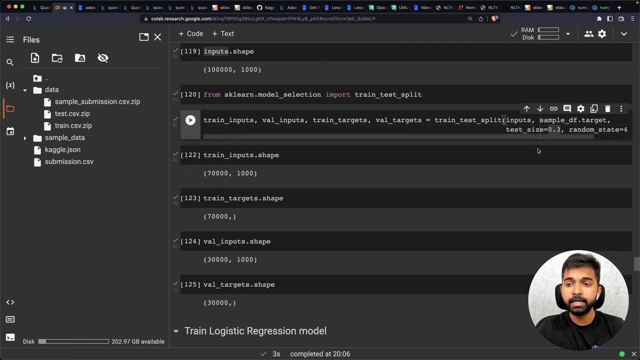 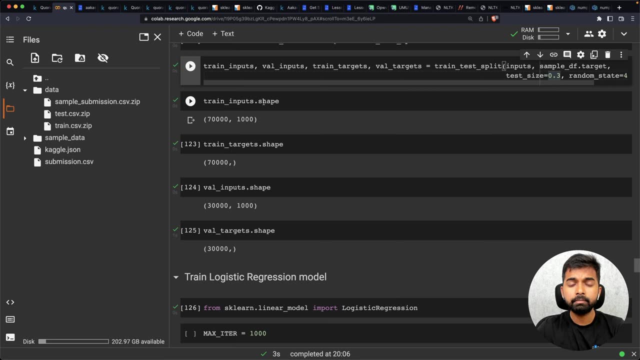 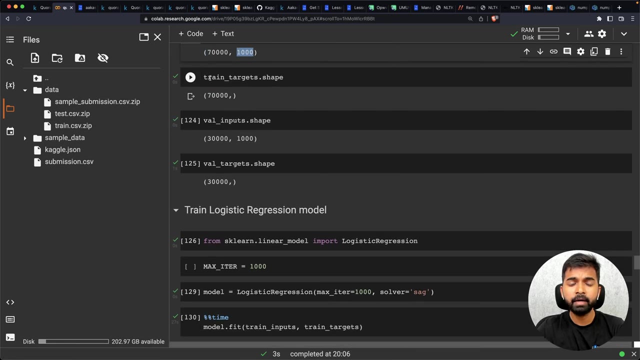 provided the percentage of values to be used as the validation set and a random state to just make sure we always get the same validation set when we run this notebook. Then we got a training set, or training inputs, containing 70,000 vectors of size thousand each and a training targets containing the corresponding 70,000 targets from the sample DF. 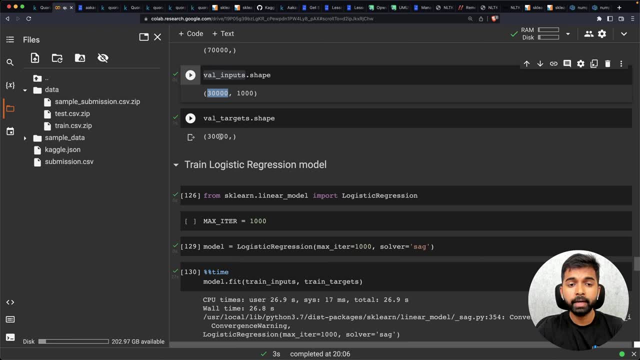 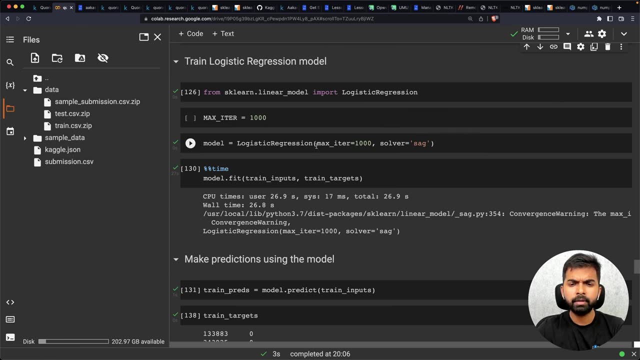 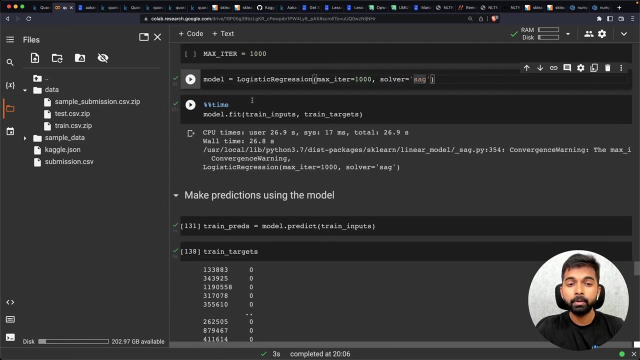 Similarly for the validation inputs. we got 30,000 input vectors and 30,000 targets. Then we trained a logistic regression model. We trained a logistic regression model with a max iterations of thousand and a solver stochastic gradient descent, because these are better suited for the kind of model that we are training. 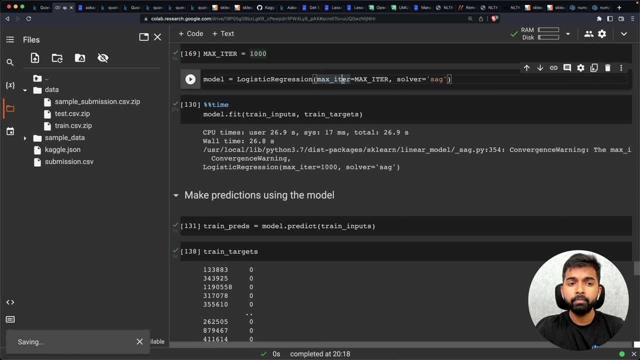 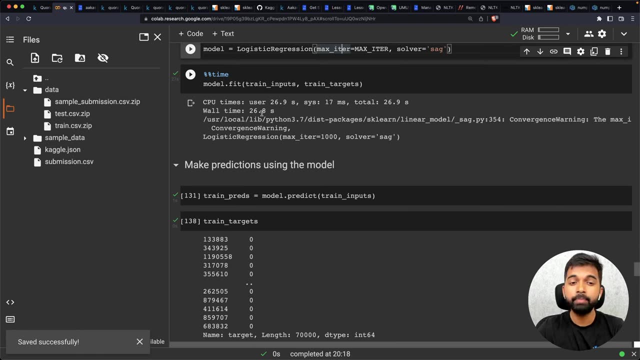 Let me just update that small typo there, Because we have a large data set, So we need more iterations and we need a better solver. and we fit it. It took about 30 seconds. It's the simplest possible model And we made some predictions using the model. 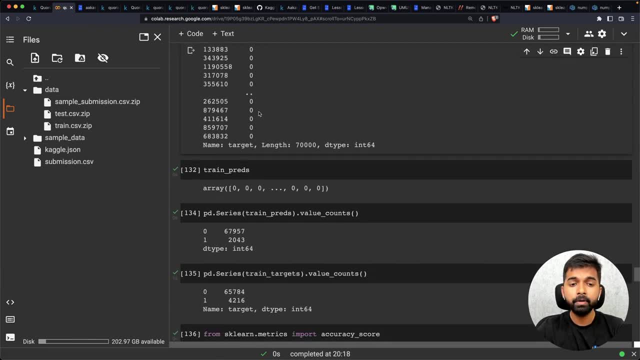 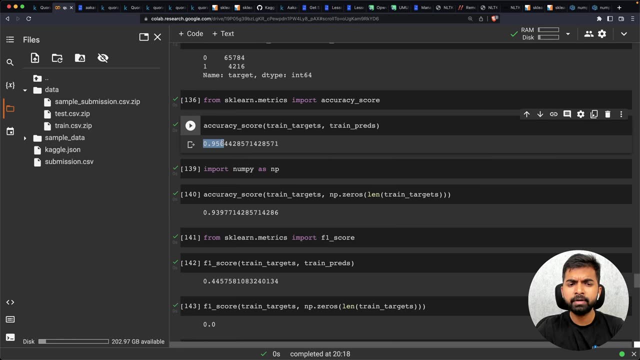 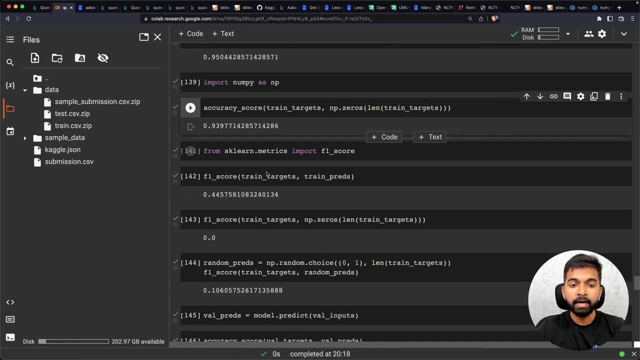 So we called model dot predict on train inputs. We got some targets. We compared those targets to the predictions using accuracy score and we got a 94%- 95% accuracy. but we realized that we can get a 94% accuracy just by always predicting zero, and we can. 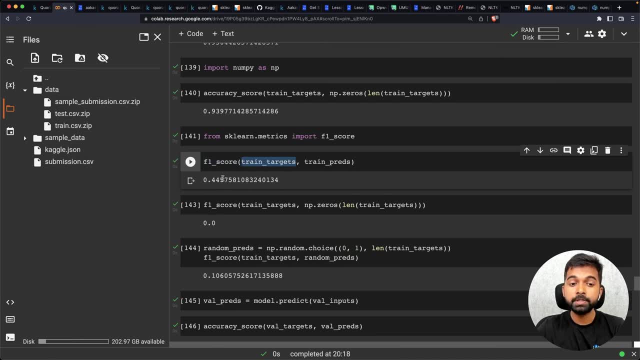 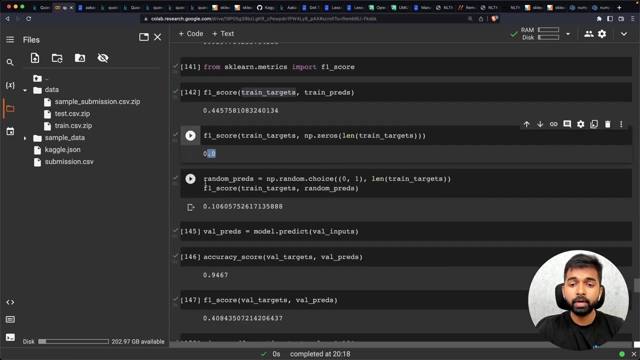 Uh, so that's why we looked at the F1. Score and the F1 score was 0.44, which is not bad considering the F1 score for the uh. always predicting zero is completely zero and F1 score for always making random predictions is 0.1. 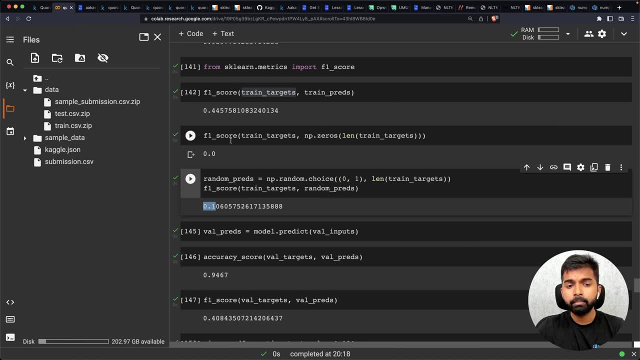 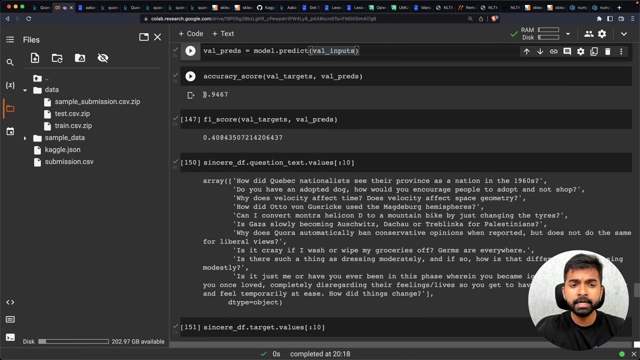 This is something that you should always do. You should always make uh, random predictions and fixed predictions and see whether your score from your model is better than that. If not, you've made some mistake in the modeling process, All right, well then, we make predictions on the validation set and we check the accuracy in the validation set. 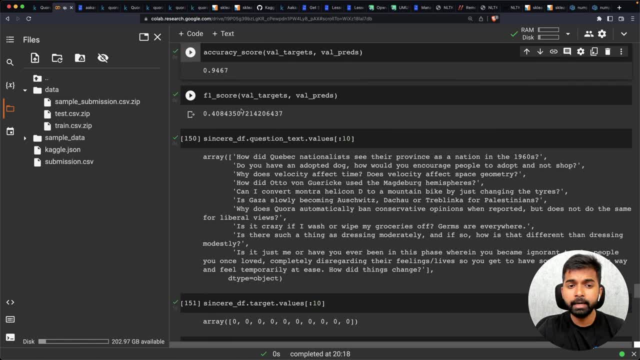 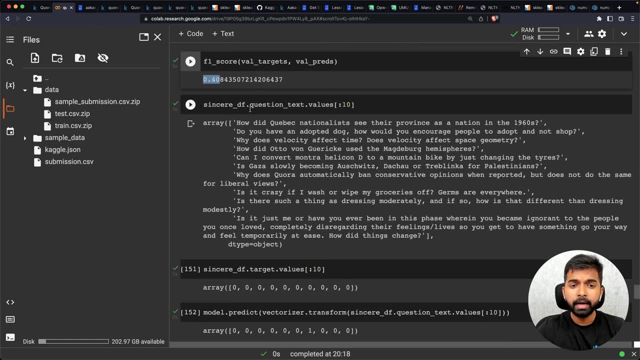 It is 94.6, but it's not very useful again. So we check the FN score. It is 0.40, which is lower than the FN score on the test set, but it's still not bad. And, more importantly probably, we also looked at some sincere questions and we tried to make some predictions on the 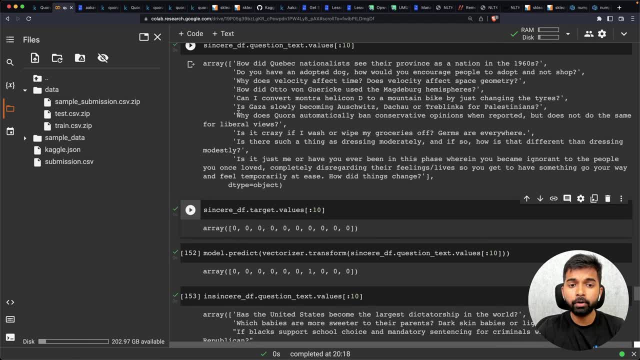 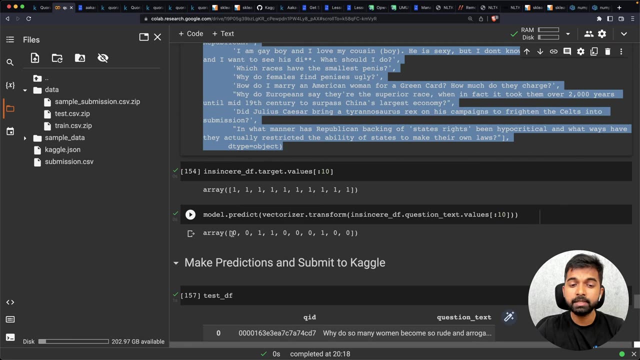 sincere questions, we saw where it got it wrong. So here The model got it wrong because it has probably picked up words like conservative and liberal, which is typically part of insincere questions, And similarly, we looked at some insincere questions and we saw that in this case, the model is really 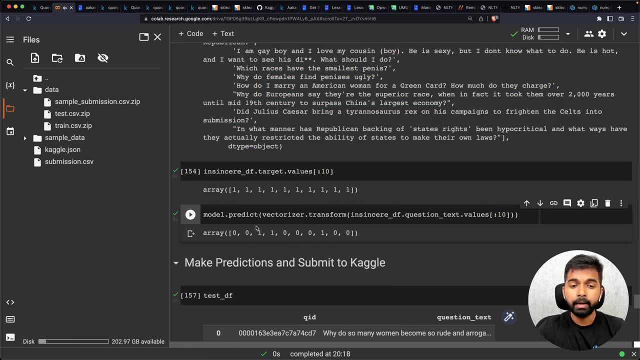 getting them wrong quite often, And that gives us some input in terms of what we might need to do. If the model is not good at detecting insincere questions, it's probably because they're not enough insincere questions, So we may need to do some class imbalance handling using class weights, something like that. 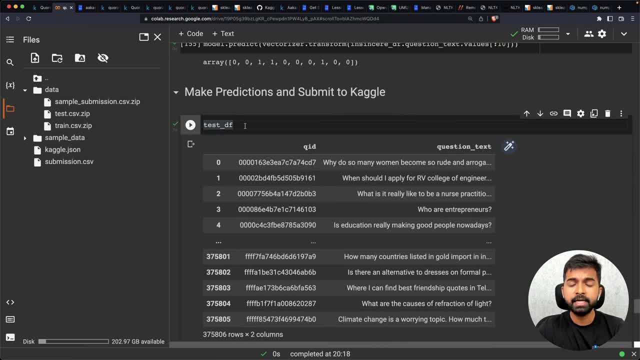 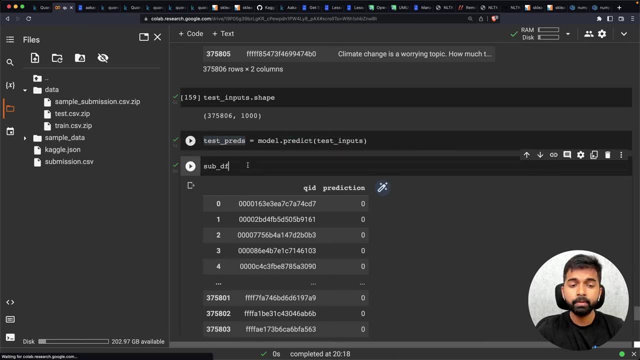 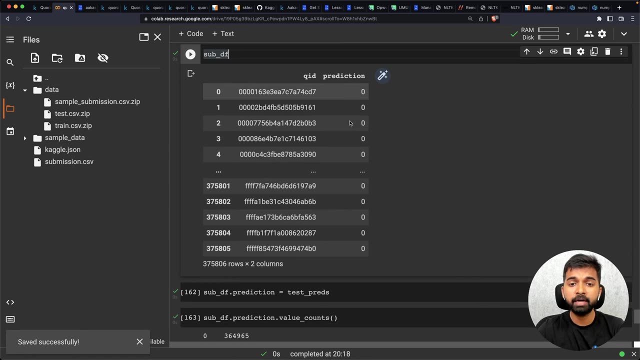 Now to make predictions on the test set. we got the test inputs and we got. we put the test inputs into the model and we got some test predictions And then, using those press predictions, we added the test predictions into the submission data frame that we loaded from the sample submission file. 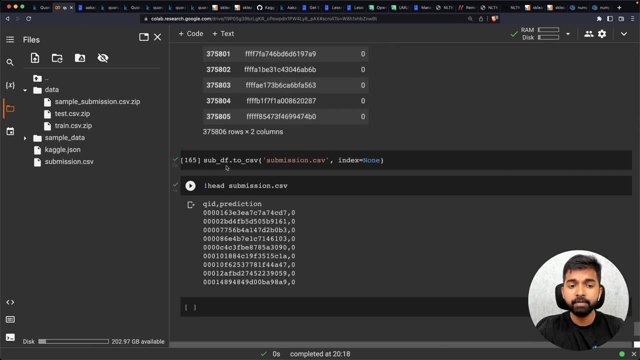 And then, finally, we took that sample submission file and we saved it to a file- submission or CSV- and we checked out the submission or CSV file And remember: this index equals zero. This equals none. This is something that will create issues if you don't put it in. 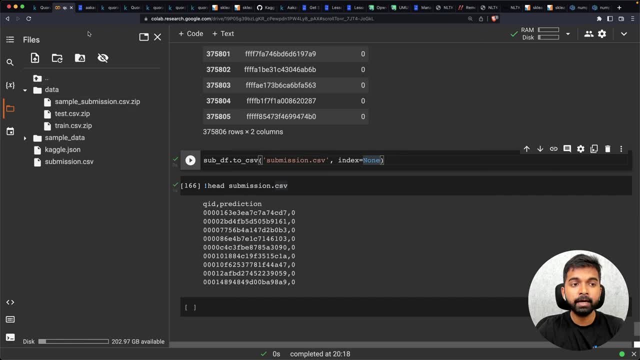 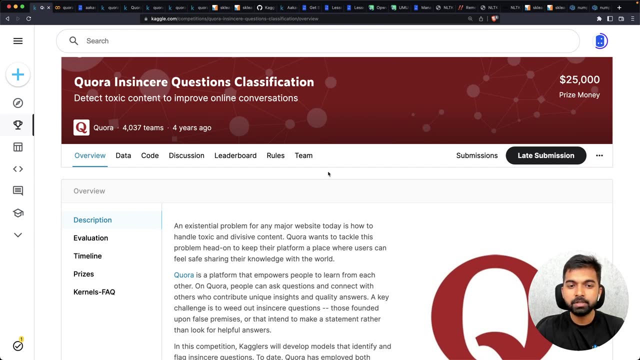 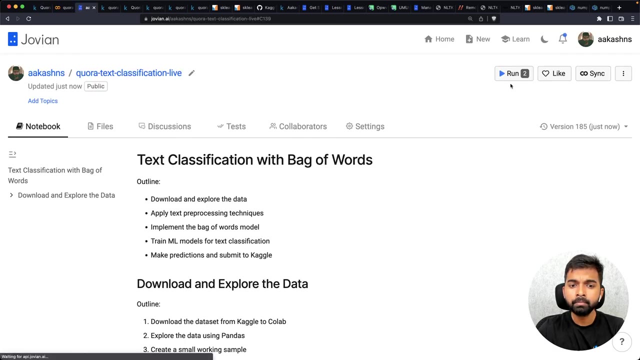 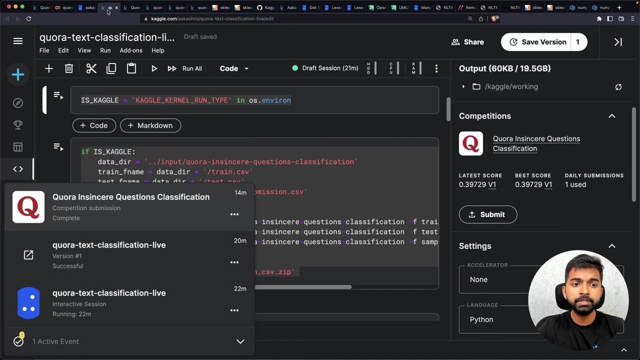 Now the thing was we cannot submission, We cannot take the submission or CSV file and directly uploaded on Kaggle because this is a notebooks or kernels only competition. Now, a lot of Kaggle competitions allow submitting submission or CSV files directly, But in this case what we had to do was we had to take this notebook and we had to run this notebook on Kaggle and we had to do some code modifications in this. 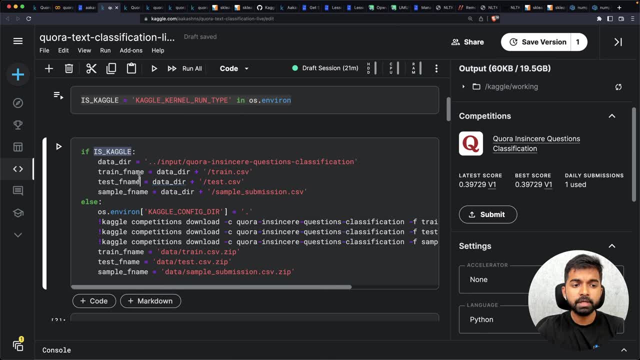 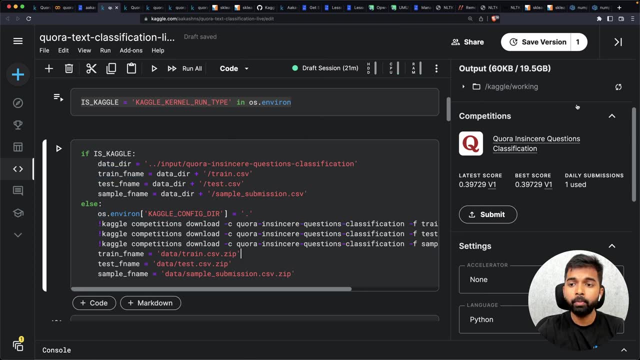 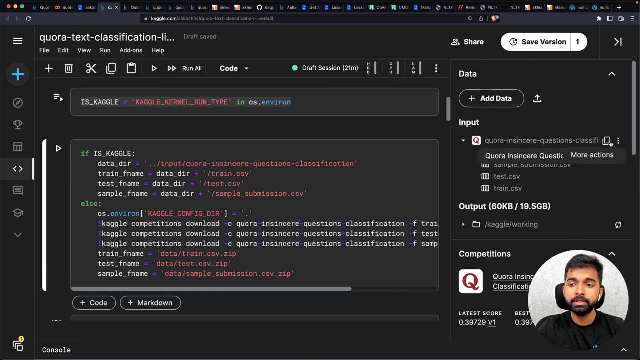 notebook. So we had to just account for the fact that if we are in Kaggle, we don't need to download the dataset from Kaggle. We simply can connect the competition here. so we can go into the data section and connect a competition and then simply use that competition data, which 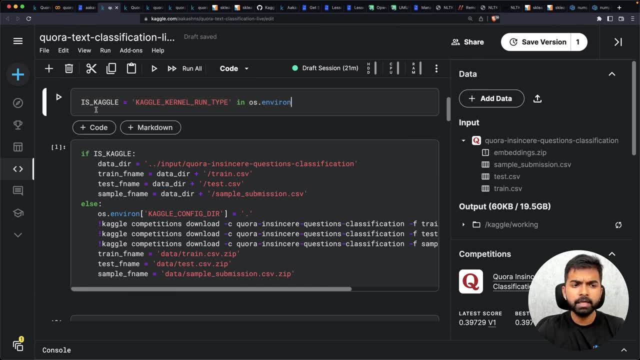 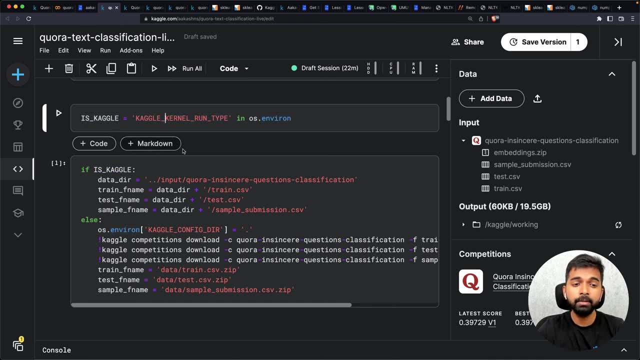 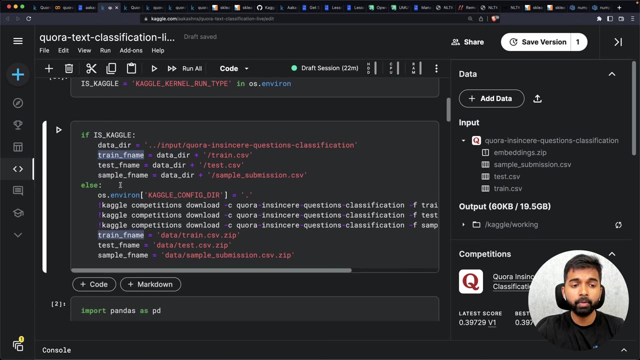 is loaded up as a local directory. So that's where we define this variable- is Kaggle, which simply checks the runtime type and which checks the presence of an environment variable and informs us that we're currently inside Kaggle. So if you're in Kaggle, then we simply use the data directory that is provided here by. 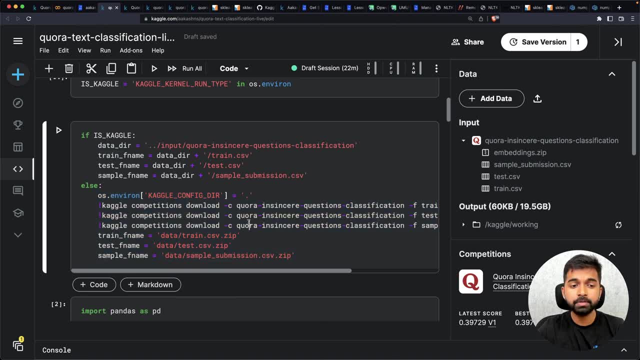 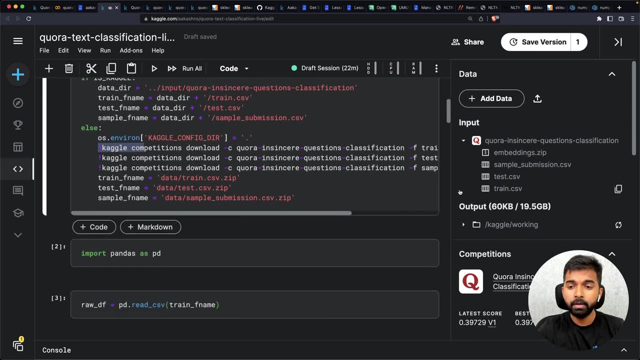 connecting. Otherwise, we use we download the dataset using the Kaggle command line tool And of course we will need the Kagglejson file next to the notebook to make this work. And the rest of the code is the same. And we just went down here and we had to turn off internet for the specific competition. 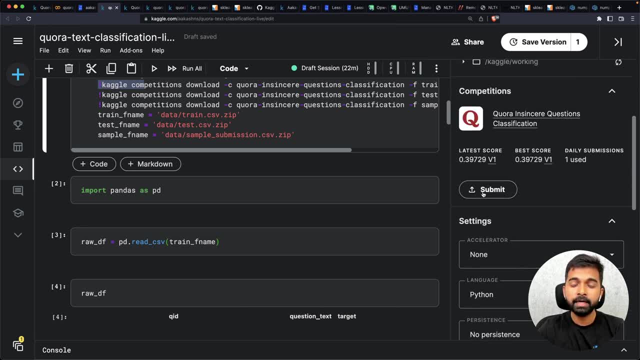 This may not be required for every competition, for this one it is. but then we click submit And what it did was it ran this entire code, which means it was created the bag of words model, Then it trained the logistic regression model, Then it made predictions on the test set. 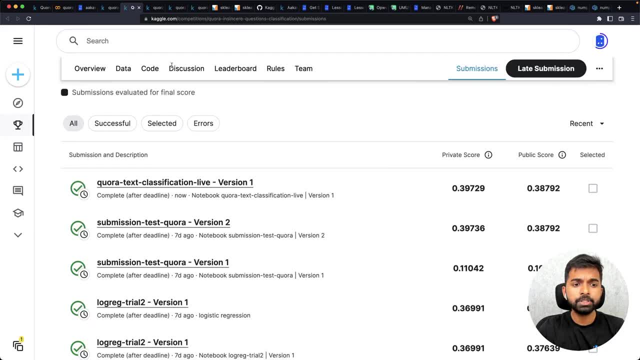 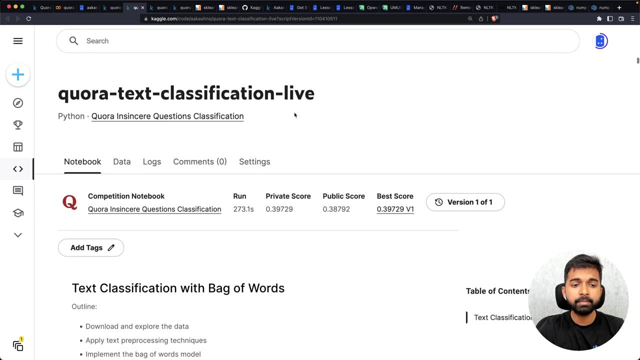 Then it created some submission or CSV file and that submission or CSV file, So you can in fact see the output of that here. You can also check it on your Kaggle profile, So that submission or CSV file which you can verify here, that submission or CSV file. 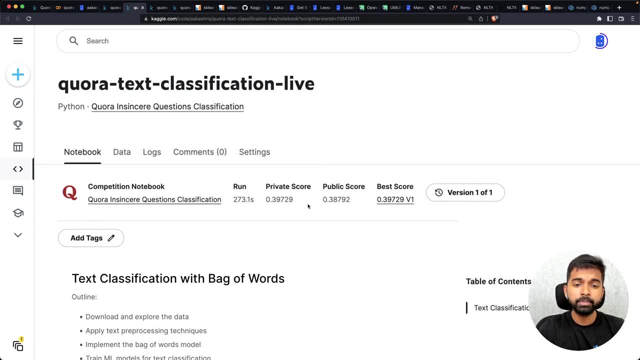 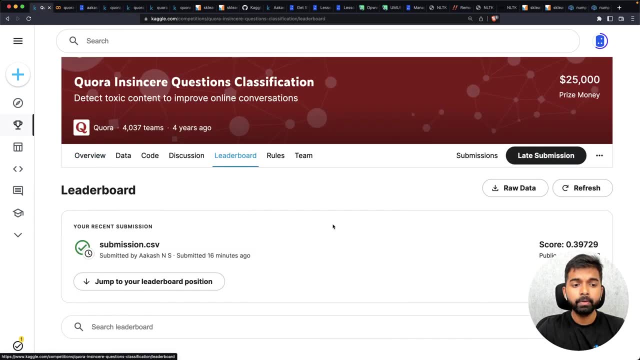 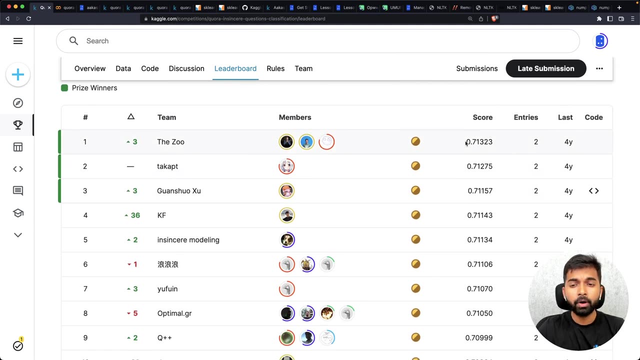 was automatically submitted to the competition and on submission to the competition It gave a score of 0.397.. Now if you go back to the leaderboard here, you can see that 0.397 is close to 0.4.. And that is actually not very far from the best score, which is 0.7.. 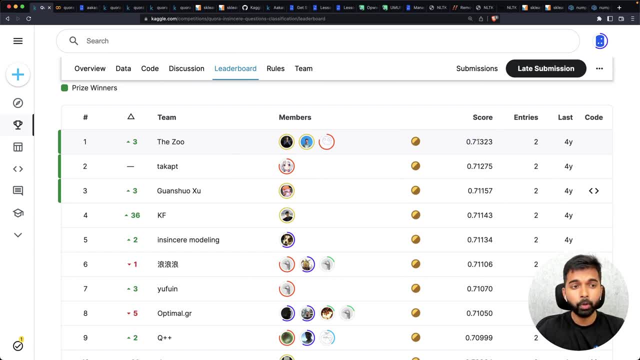 It's, in fact, much better than 0.1.. So we are halfway there. 0.1 was what you would get if you made a random submission. 0.4 is what we're getting with bag of words. So we're halfway there. 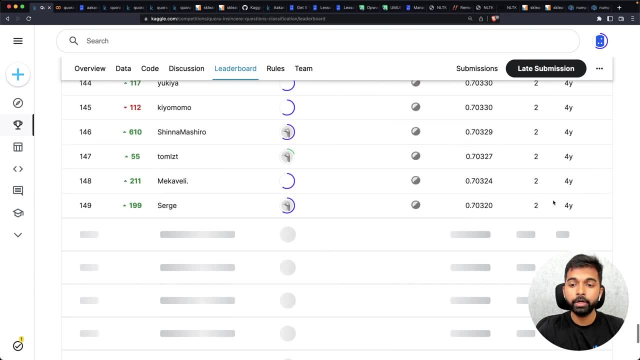 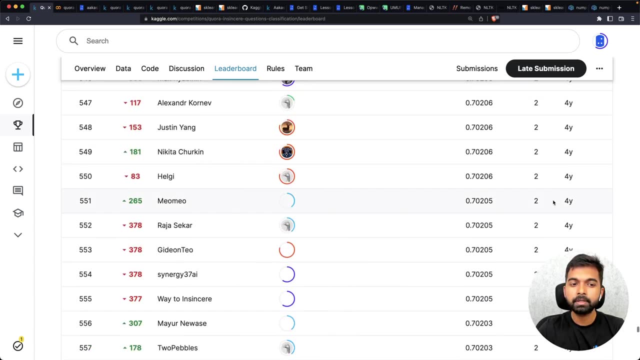 But if you scroll down in the leaderboard and try to find the position at which you have 0.4.. You'll see that it is very low because bag of words is a very simple model And there are many much better models that you can use that we will look at over the. 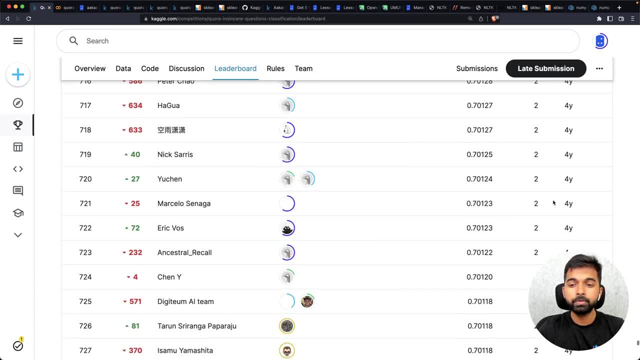 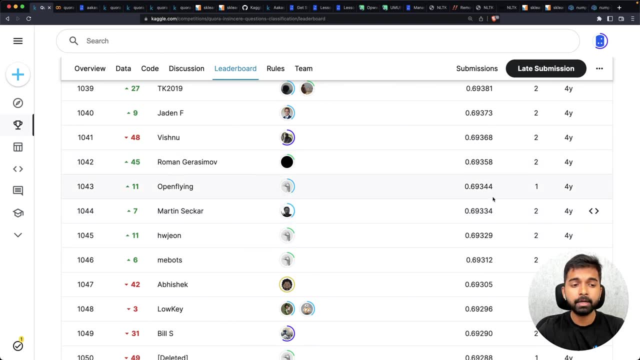 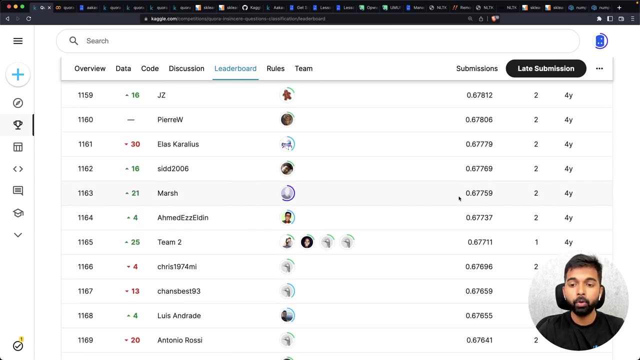 course of the next few tutorials, And most people have used a lot better models. That's where you'll see that 0.7 is actually about. the first thousand submissions are all 0.7 and above, but that should not stop you from rightly interpreting the score as something. 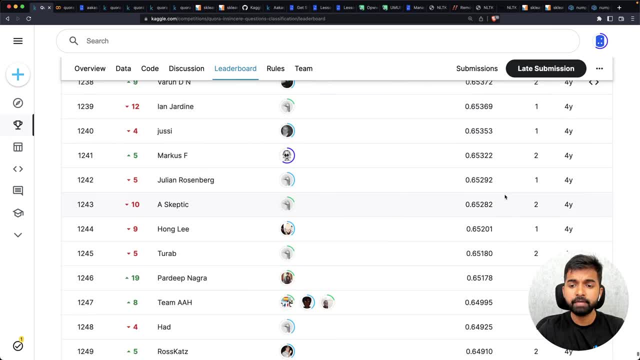 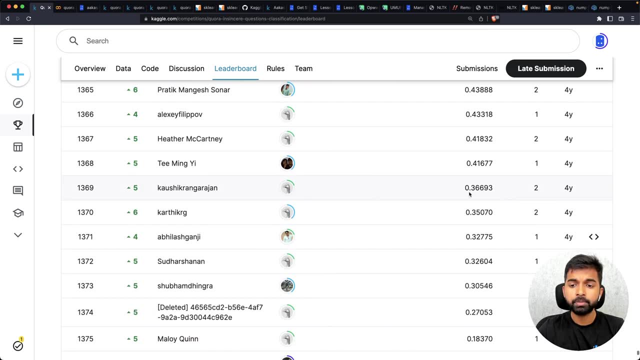 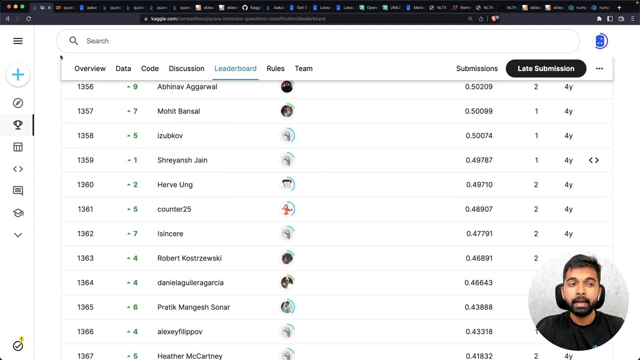 useful Right. So, even though point 7.4, so 0.4 is roughly about, yeah, so 0.4 is roughly about 1367 out of 1396.. So about 1350 out of 1400.. 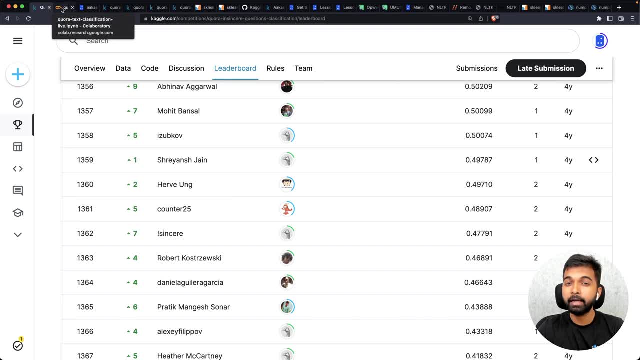 And, of course, we are using a very small fraction of the data. We should be using the entire data set. We should be using a larger vocabulary. We should be training a more complex model. We should possibly be experimenting with some of the bag of words: parameters, some of the 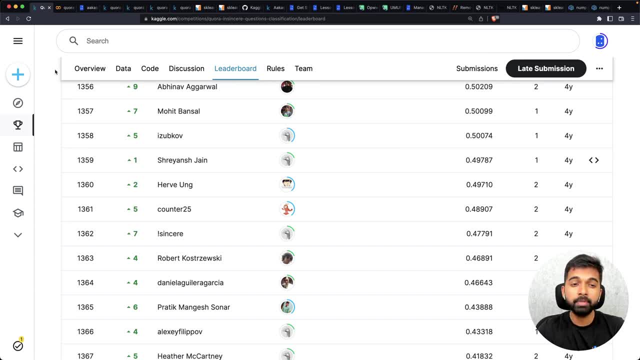 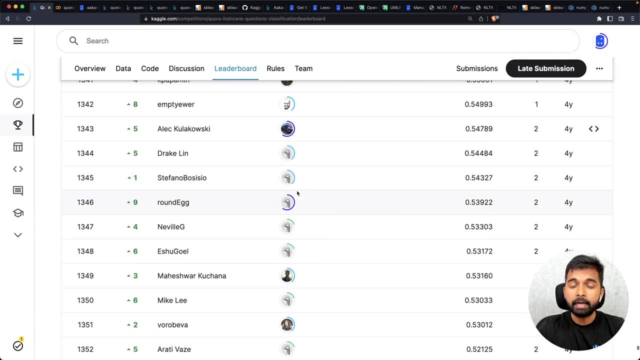 count vectorizer parameters. So we should be doing a lot more research. Okay, We should be doing more experiments, maybe using tree based models, and we'll get a much better result, And I encourage you to try that out when you're working through this tutorial. but try to. 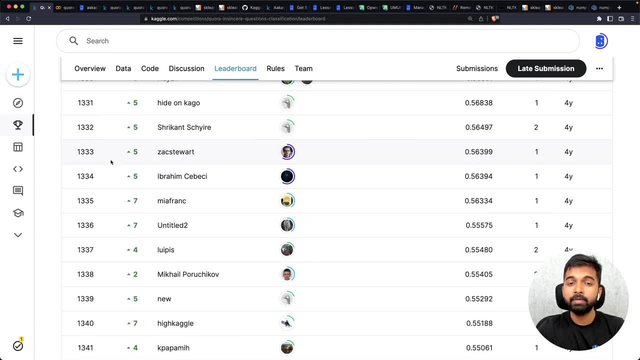 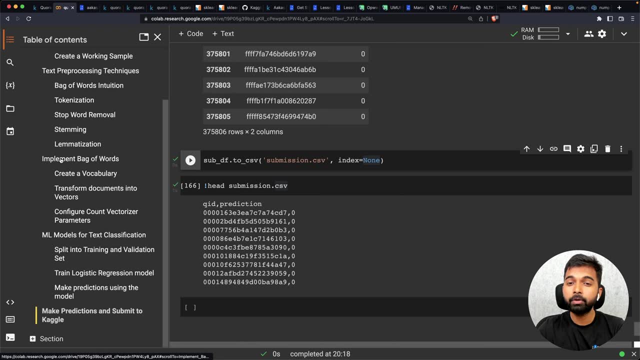 understand that the bag of words is just the beginning And over time, we will train more models, but the only thing that will really change is this portion: instead of implementing bag of words, we're going to implement something else. The rest of the pipeline is going to remain the same, which is loading the data, exploring. 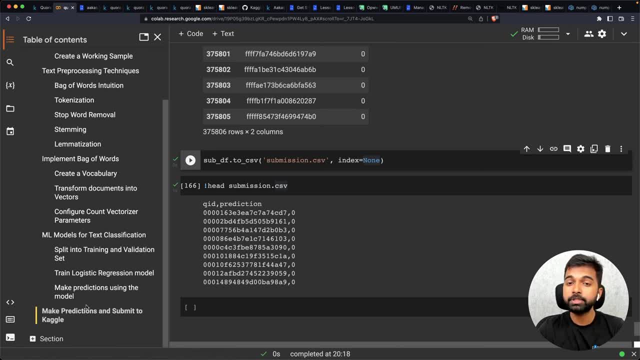 the data and then creating machine learning models and making submissions to Kaggle. So understanding this machine learning pipeline, making submissions to Kaggle- Okay- And making sure that everything is working properly is very important, so that then we can experiment with each strategy on the same real world data set. 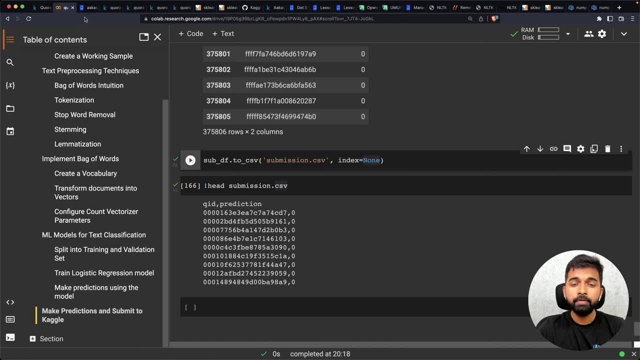 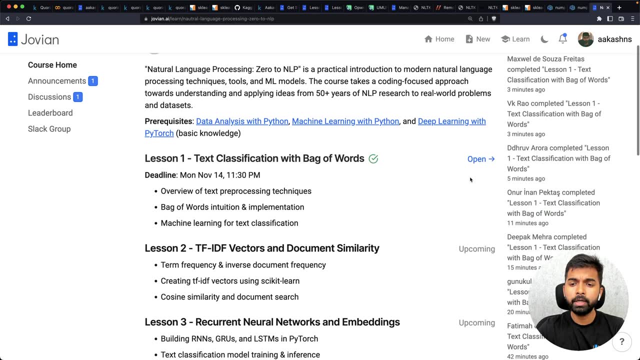 So let's come back and work on that next time. Now, if you haven't done so already, you should head over to 02nlpcom and you should enroll in the course and you can go into this lesson and you can mark this lesson as completed. 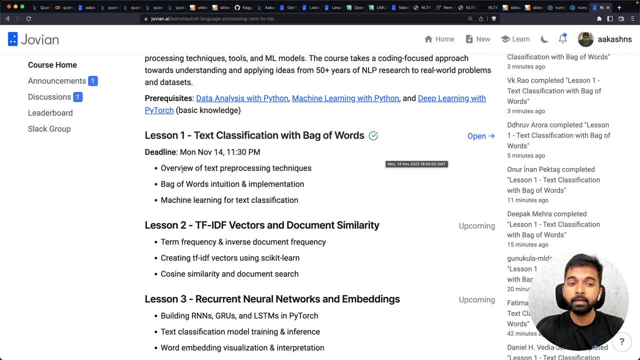 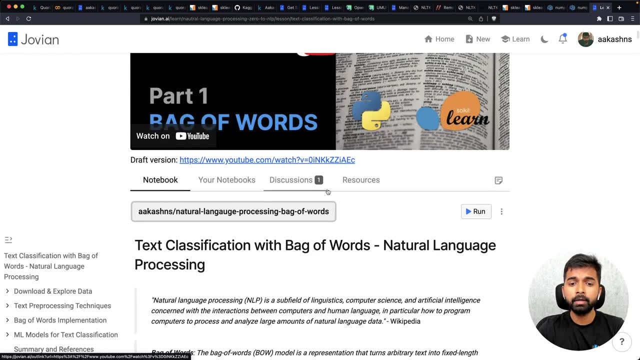 We will have an assignment, a bunch of assignments, and we will also have a project to stay tuned for the announcements And if you have any questions at any point, Okay, You can go to a lesson and go under discussions and post your question, or you can also go. 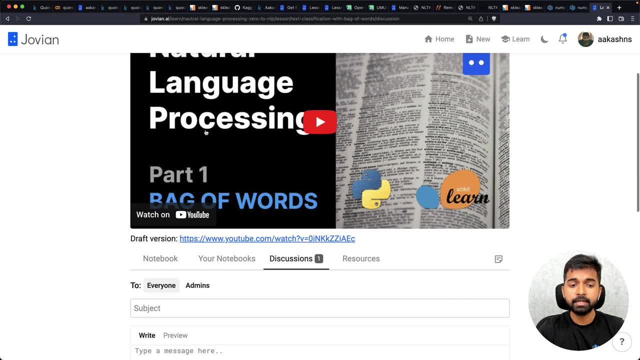 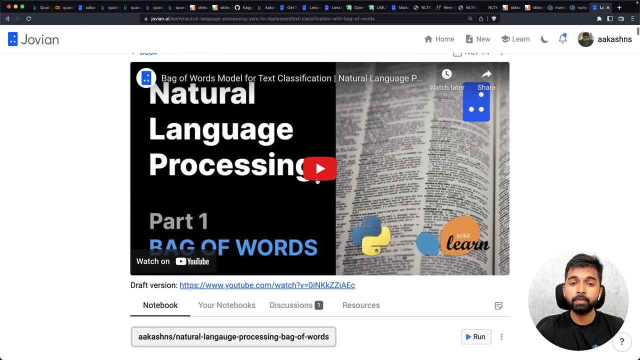 back and you can post a discussion on the course page itself. Now the entire code will be available here so you can go in and check the code. The entire recording is also available here. You can view the recording here and all the resources, all the links that we've used. 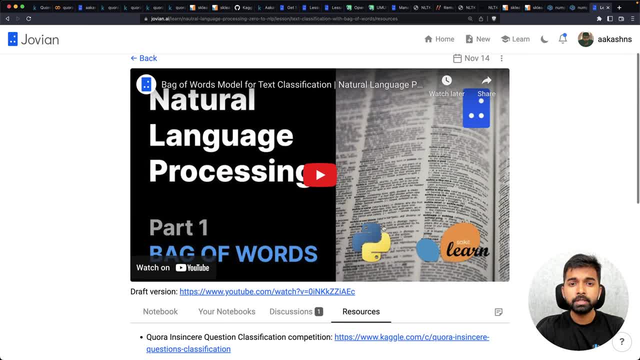 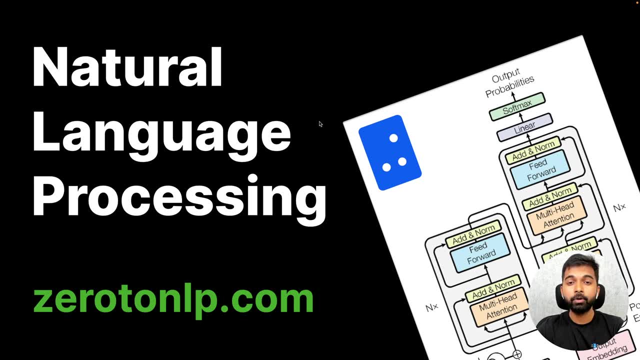 all the resources also available here. So with that we reached the end of this lesson on bag of words. This is natural language processing 02nlpcom. I'll see you next time. Thank you, and have a good day or good night.